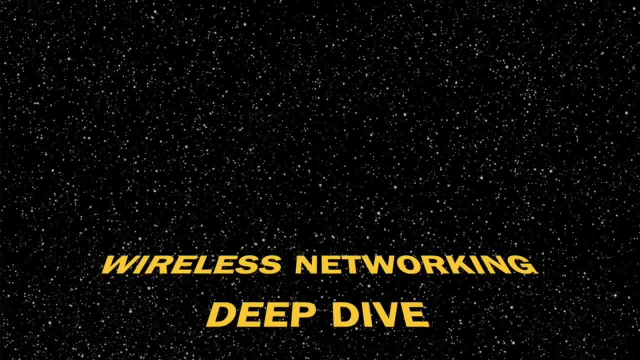 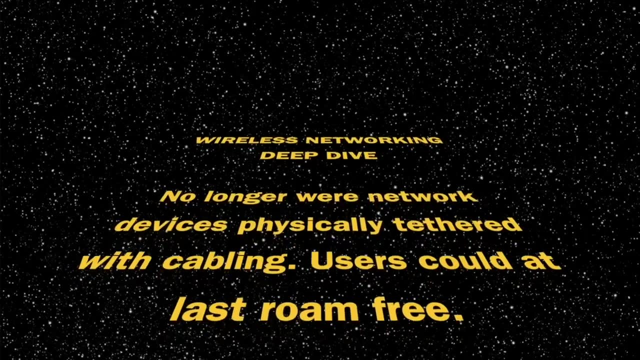 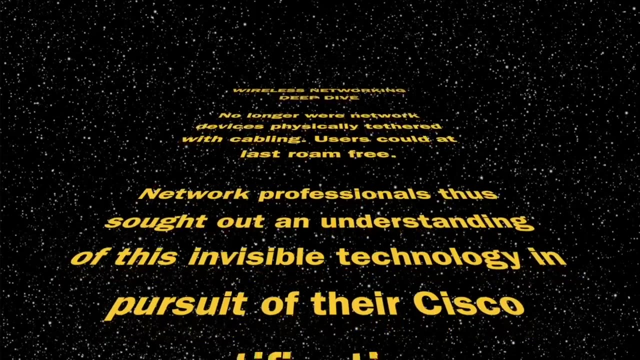 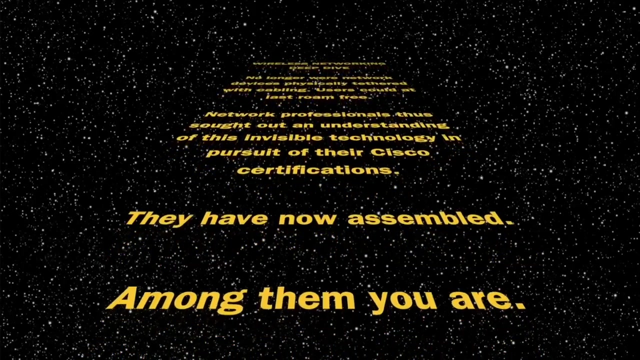 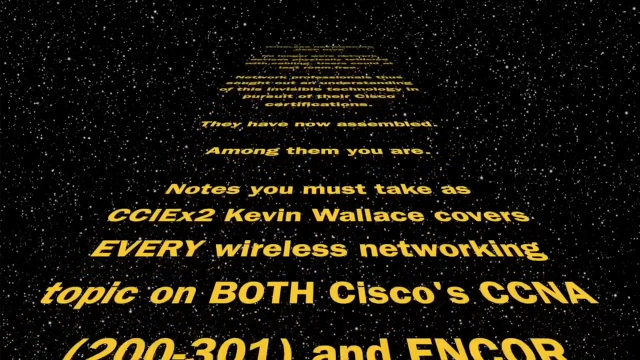 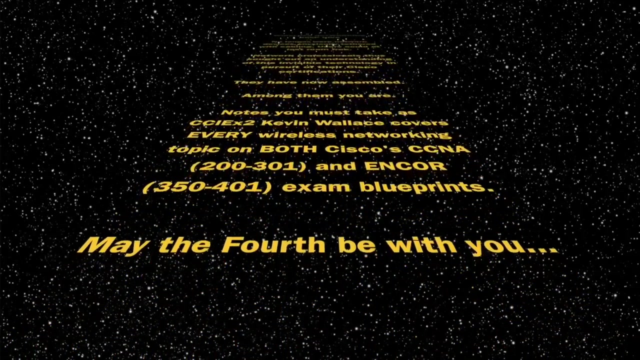 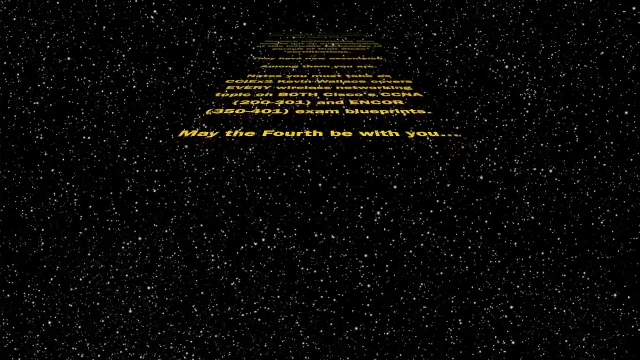 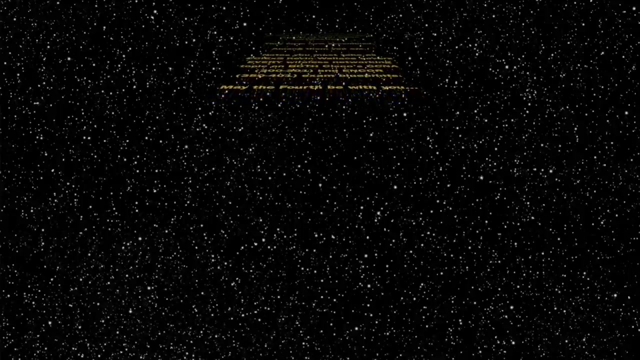 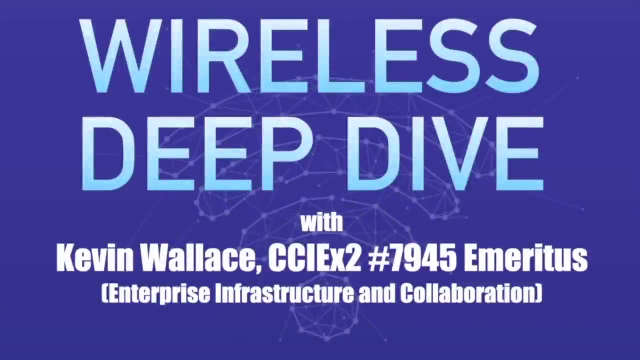 Thank you for watching. Hey, welcome everyone to our Wireless Networking Deep Dive. And for those of you who are new to the channel watching this on a replay, just be aware that we're recording this live on May, the 4th Star Wars Day, hence some of the Star Wars theming. Basic goal is we're going to be covering. 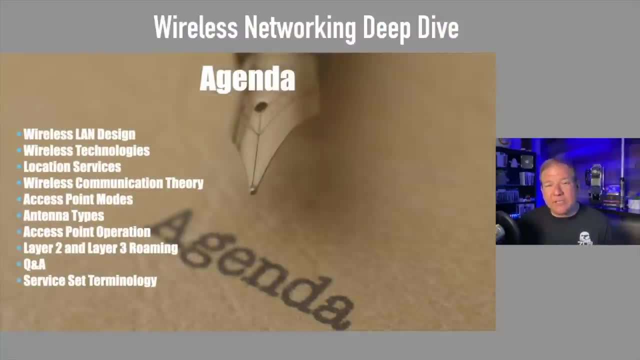 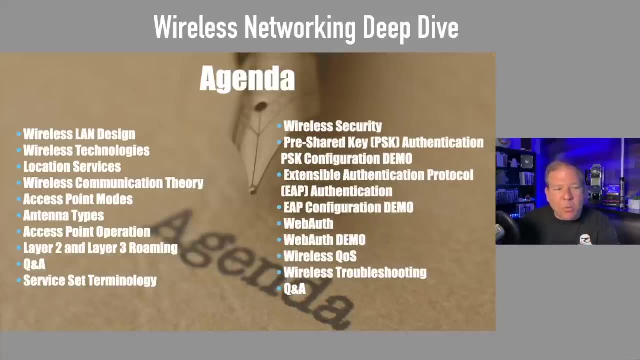 all the topics, wireless related topics on the CCNA and Encore exams, And you see those listed here. It's kind of interesting when Cisco came out with the new version of their certifications two or three years ago, instead of being route switch focus for CCNA and route switch focus. 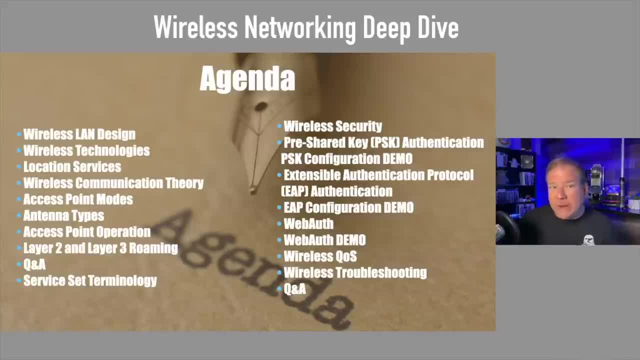 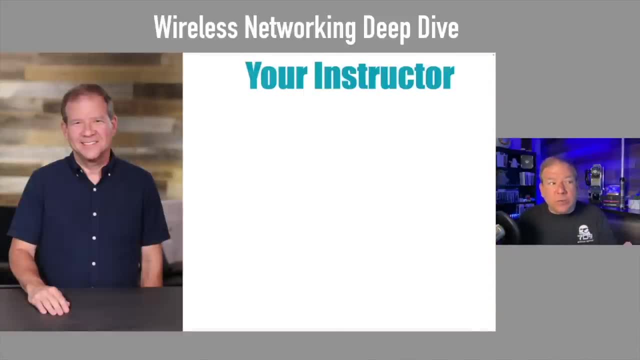 for CCNP. they changed it to enterprise, And enterprise implies things like wireless and cloud and more security, So it's not just so route switch focus like it used to be. So I thought this would be a great opportunity to do a deep dive into wireless specifically, And for those 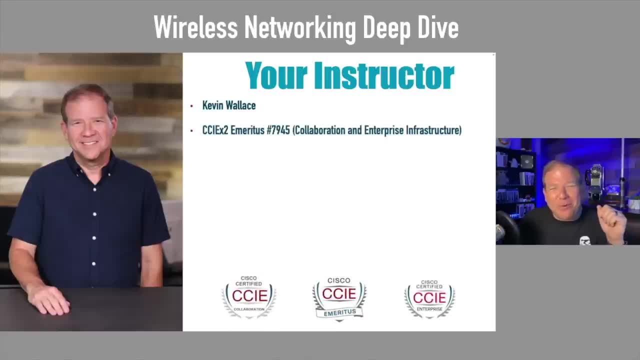 of you not familiar with me, here's my super quick bio. My name is Kevin Wallace. I've got a couple of CCIEs. I've been doing this for a long time, working with Cisco Gear since the late 80s. 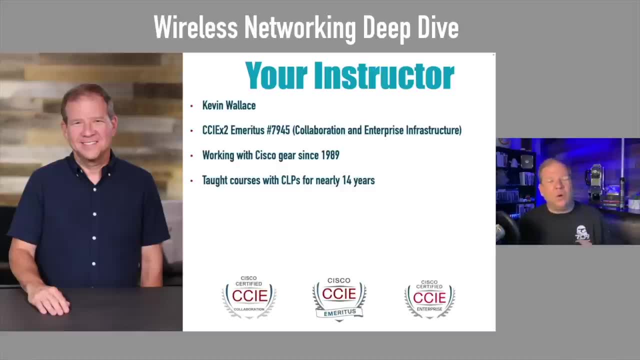 Very first router, the EGS Plus. Working with Cisco Learning Partners for 14 years Been doing my own training company- about eight years now. Really the best job I had in corporate America, though, was I was a network designer at Walt Disney World out in Florida. My family and I- 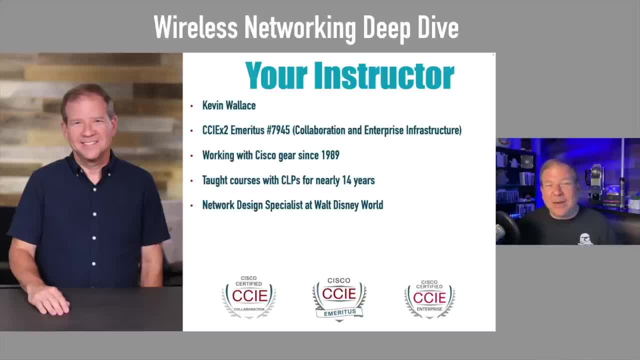 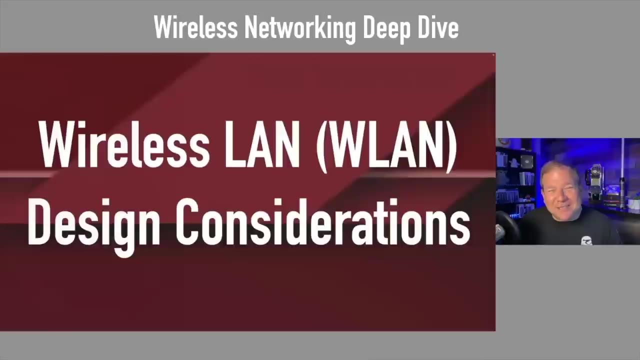 we are huge Disney fans- Actually going to Disney tomorrow. Written a bunch of books for Cisco Press and done a bunch of videos for them, Taught at Cisco Live a couple of times, Got the Distinguished Speaker Award. Bottom line is: I love this stuff and I cannot wait to get into this wireless topic with you. 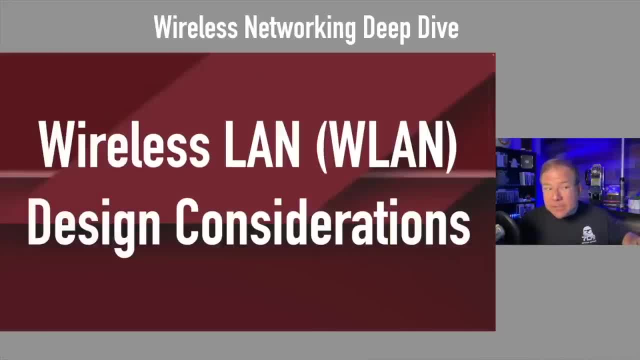 And we're going to get. we're going to start at the basics. So if you're brand new to wireless, no problem. If you're experienced with wireless, I think you're going to learn some things as well, because we're going to be talking about security. I'm going to be getting into electromagnetic field. 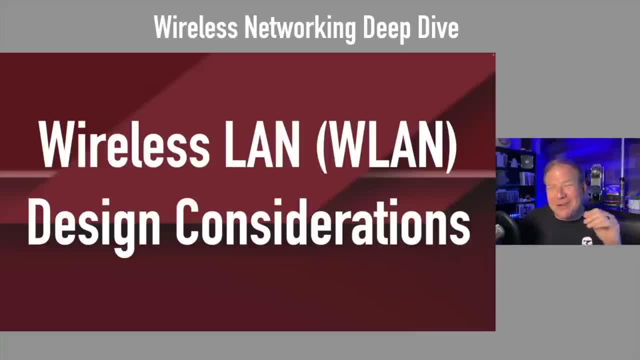 theory a little bit. I'll even mention Maxwell's equations along the way. I think you'll enjoy that one. And we just want to start out really basic though, by talking about some different wireless LAN considerations, One of the most basic considerations or design decisions we have to. 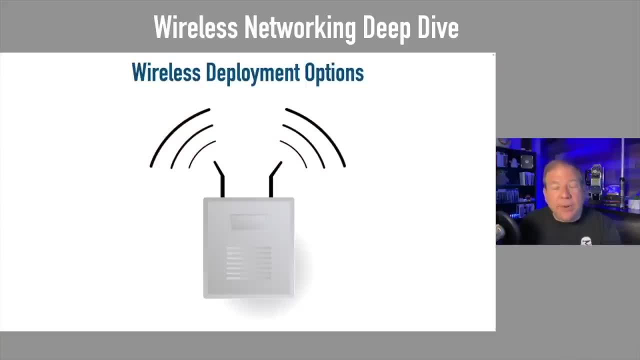 make is: what kind of wireless LAN are we going to have? We've got two main options and I really encourage you to take, really encourage you to take some notes on this, because we're going to be giving you lots of stuff to take notes on today, But one of the basic design decisions is: 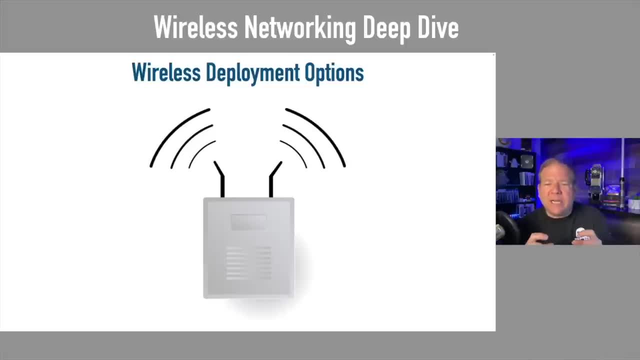 do I want to have a bunch of individual wireless access points and manage them independently, Or do I want to have one central point of control, a wireless LAN controller, and just do all my configuration there, And then I'm going to push that configuration out to all the different access points throughout my environment? 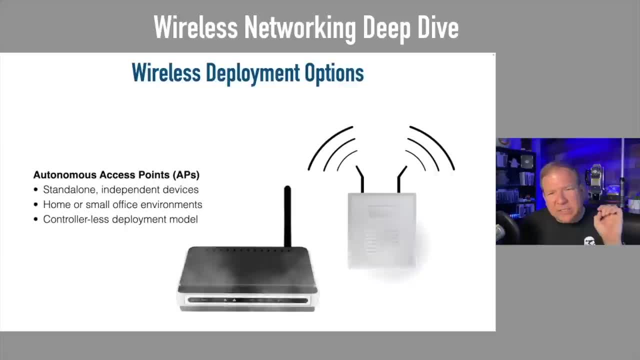 The first option is called an autonomous access point, And this is what you might have in a small office or maybe, maybe in your home, For example here's- we might refer to this as a wireless router. This is something that you might get. 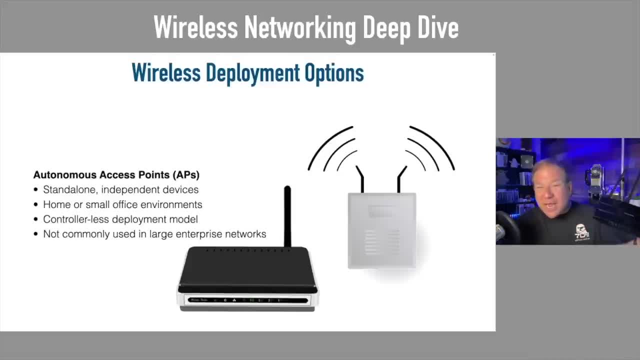 down at your local big box store and you would plug into your cable modem coming into your home. And even though we call this a wireless router typically because it is routing, it's routing between your home network and your internet service provider. It's routing between. 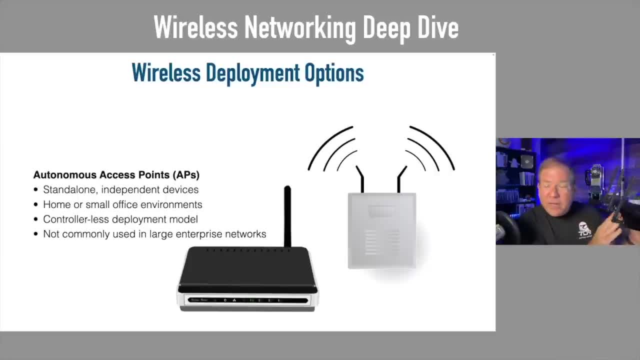 your network and the internet, in other words. But it really is. in addition to being a router, it is an access point, Because an access point is simply a device that's going to allow a wireless device like my iPhone to communicate wirelessly and then transfer that into a wired. 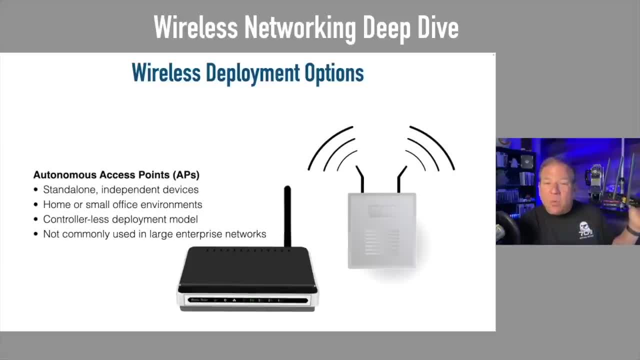 communication So I can come out of this and get into a wired network. Now, this is also a switch. It's got four switch ports on the back, So really, this thing that we call a wireless router. I would argue that yeah, it's a router, it's a switch and it's a wireless access point. But 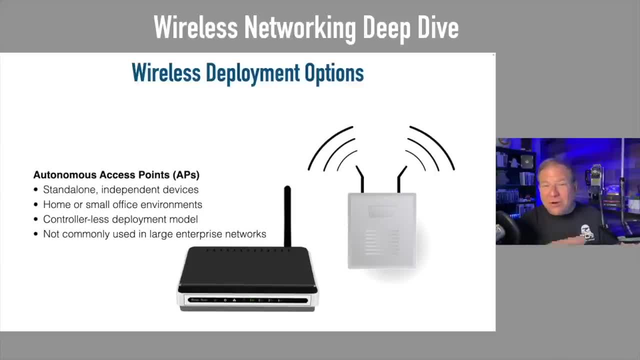 if I start to have a bunch of these to give me coverage in a large enterprise network? that's not going to scale very well. What if I had a large area to cover and I just had one of these? That's not going to do it. The range isn't going to be far enough. 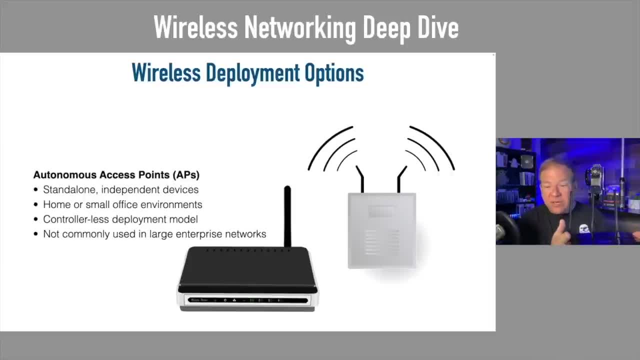 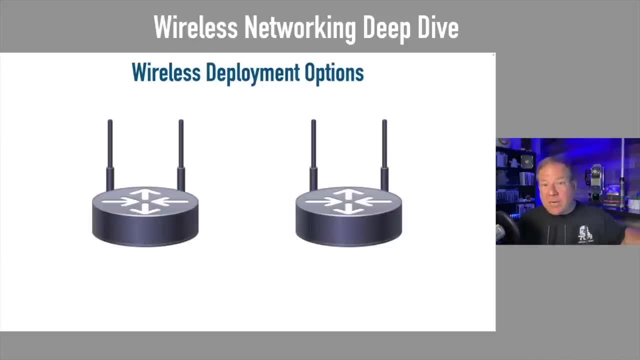 Could I have more than one of these autonomous access points that I administer individually? Yeah, I sure could. In fact, I used to do that. I take care of the network at my local church And I remember, before we did a big expansion, I had four wireless access points scattered. 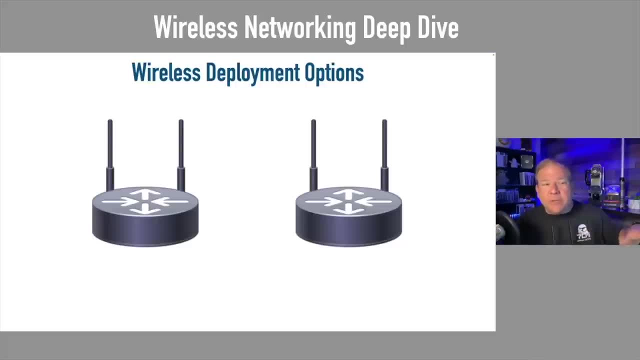 around the different areas of the church. to give complete coverage And in order to be able to take your device and roam from location to location within the building, we needed to be able to have the same configuration on all the different access points. So let's say it was called like: 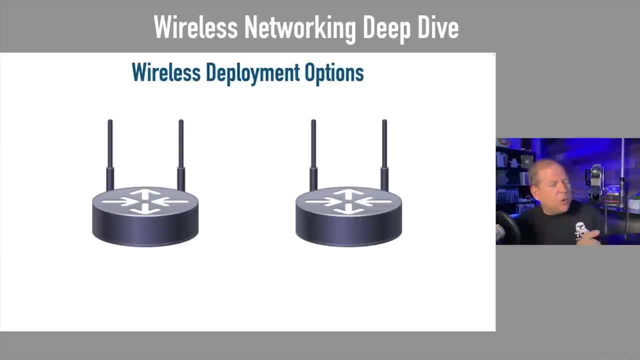 ECC- It's like Eastside Community Church, So ECC might've been the wireless name. I had to configure the same password, the same network name, the same SSIDs. we're going to be learning on every single device And that way I could roam from location to location And yeah. 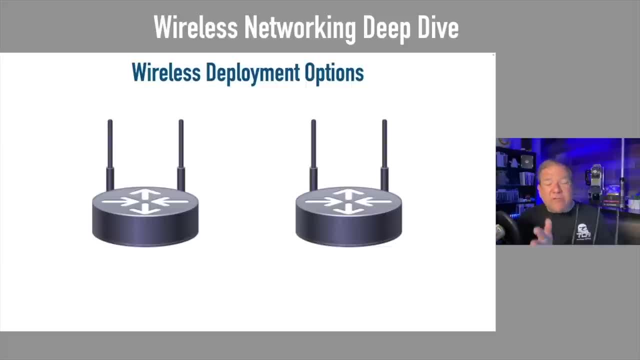 it seems like I never left the network, So that works. You can have multiple instances of autonomous access points and get wide coverage. However, it doesn't scale well. Imagine I was noticing somebody in the chats- I think it was Ken- saying that. 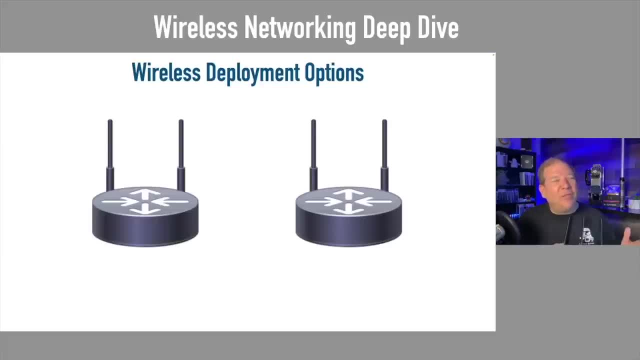 Ken just got a job and they have something like 3000, I think he might've said- or maybe he said more than that- but thousands of access points. You don't want to have to configure individually thousands of access points, because if you do you've got to have an IP address for each one. It's just not. 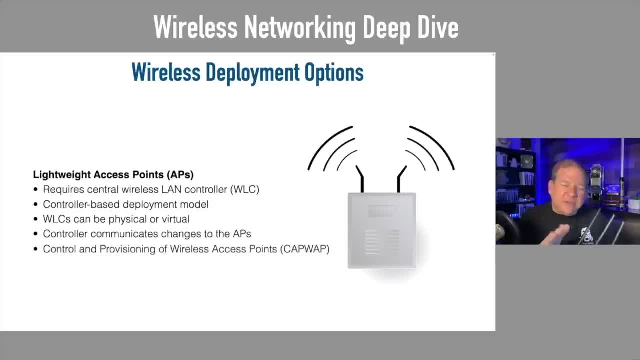 going to scale. So what's the alternative? The alternative to an autonomous access point where we manage things one by one individually, the alternative is to have a lightweight access point. Now, when I hear the term lightweight, it almost makes me feel like it's not as robust. I mean it's lightweight. Is it less robust than an? 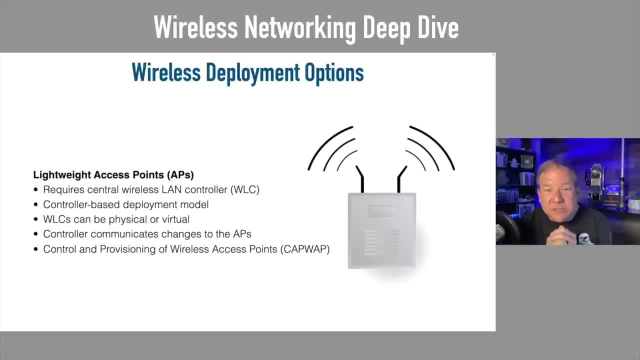 autonomous access point. No, the access points themselves are lightweight because we don't have to do a lot of configuration on them, The brains of the operation, if you will. that happens inside of a controller, a WLC for your notes, a wireless LAN controller. Here's an example of 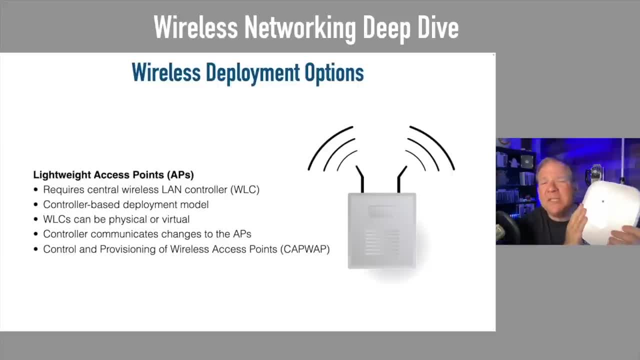 a Cisco access point, And the Cisco access point can be a lightweight access point, And we could have hundreds or thousands of these and they could all be configured simultaneously from one location, from a wireless LAN controller. And I want you to jot down in your notes: 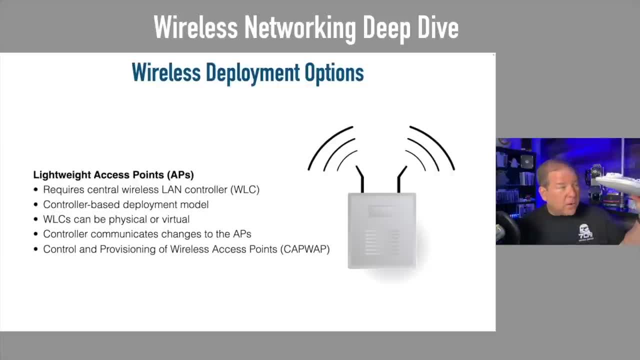 the protocol that's used to talk from a controller out to these potentially thousands of access points in a large enterprise environment. The, the old protocol that we used to use, that we don't see much anymore, was called LWAPP, the lightweight access point protocol. I predict you won't see that today Instead. 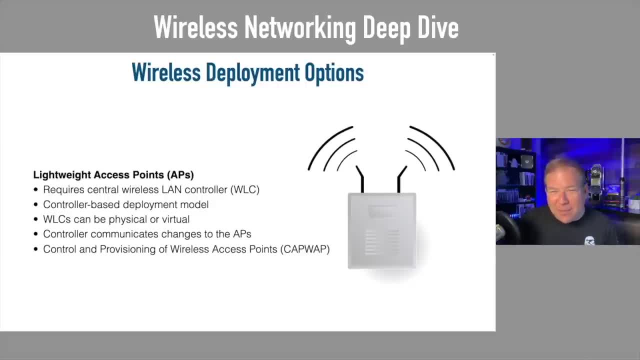 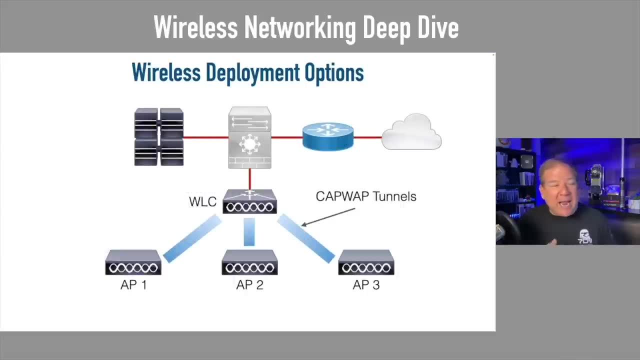 you're going to see something called CAPWAP C-A-P-W-A-P. That's control and provisioning of wireless access points. So that is that's probably what you're going to be seeing today, And here's what happens. logically, You've got all these access points, like you see on screen. 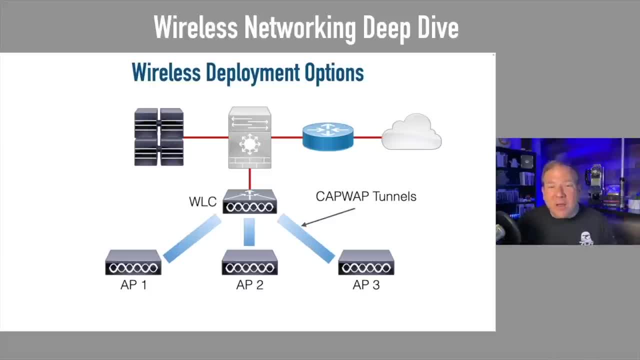 access points one, two and three Communicating with the wireless LAN controller, And they're doing that through a protected CAPWAP tunnel. Now here's what's not obvious And what I'm about to say. I know some of you 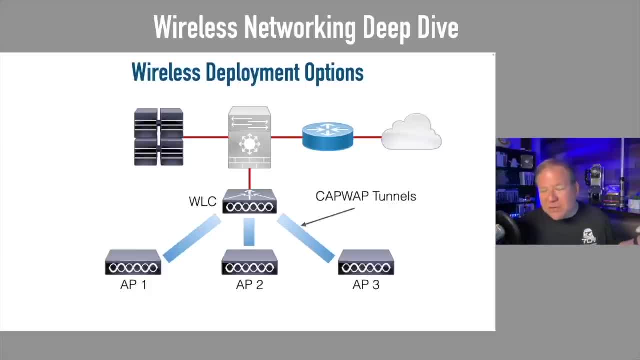 are going to say: no, Kevin, there's an exception to that. Yes, there's, there's an exception to what I'm about to say And we'll talk about that exception. But in general, when you're talking from an access point up to your wireless LAN controller, it's not just the control traffic. 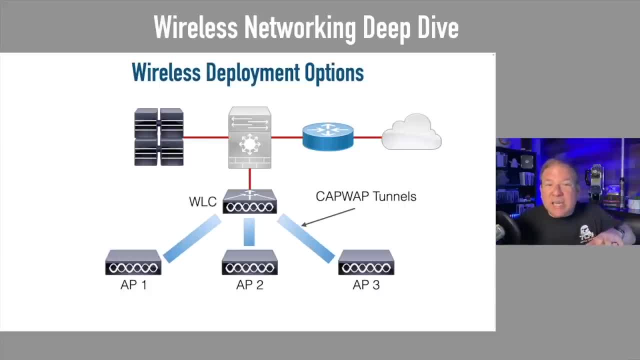 that's going to be communicating with the wireless LAN controller. It's going to be communicating over that CAPWAP tunnel. It's the actual user data. So if you're talking from one access point to another access point, yes, there are exceptions, But in general, your data and your control traffic. 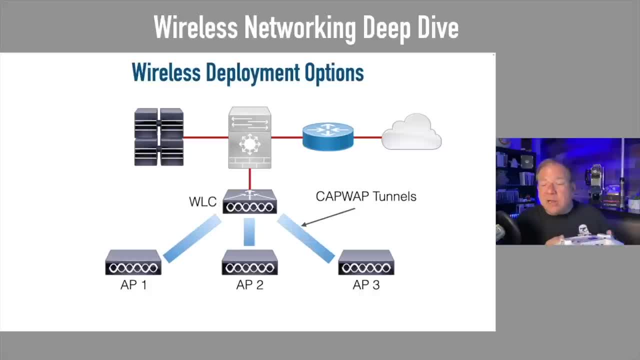 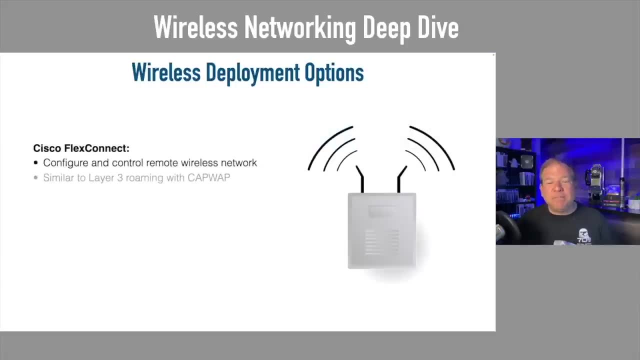 is going to be going over that CAPWAP tunnel up to your wireless LAN controller and then back out to the destination access point if you're going between access points. So let's think about some different ways of deploying these. Now I mentioned there was an exception or multiple exceptions. 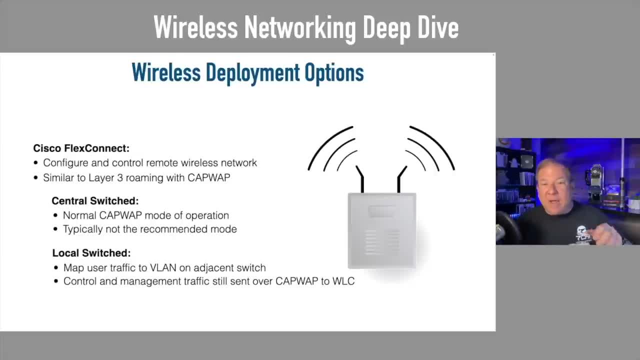 Let me give you one. Let's say that we have our wireless LAN controller at a remote office. we've got a wide area network and we've got the central office, the main headquarters of the company, And then we've got these remote sites, geographically dispersed, And we all are part of. 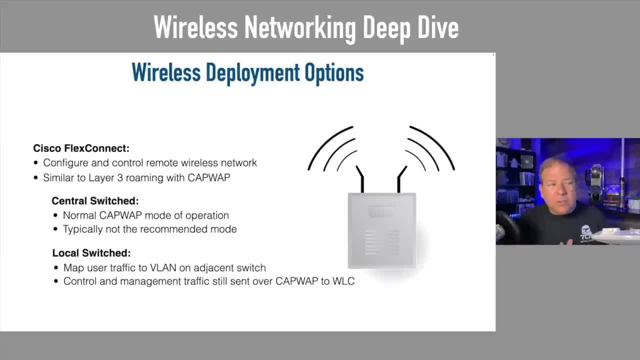 the same wireless network. Do we really want, do we really want, every access point at all those remote locations going over those WAN connections Back to the headquarters to send the data through the wireless LAN controller? Probably not. That's a lot of extra traffic on the WAN, especially if we're just going from one access point to 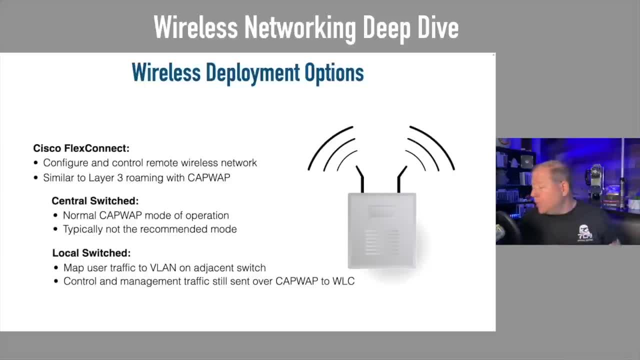 another access point within the same wireless location. So Cisco does us a favor. They have a feature called FlexConnect And that's something I would want you to know for the Encore exam, by the way. They have a feature called FlexConnect and that is going to allow. 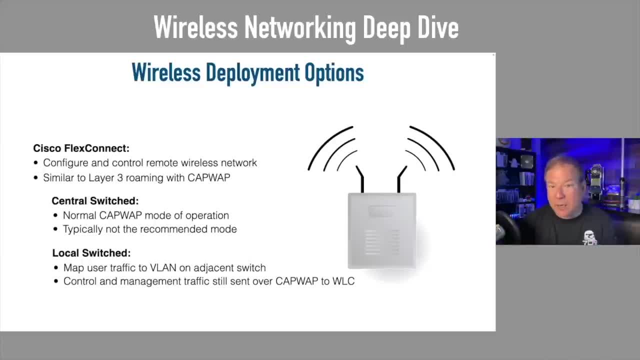 us to keep the local data local at those remote sites. And we're going to be talking, we're going to be talking back to the wireless LAN controller just for control traffic. So please hear me on that. Get that one in your notes. FlexConnect says: if you've got remote site A and you've 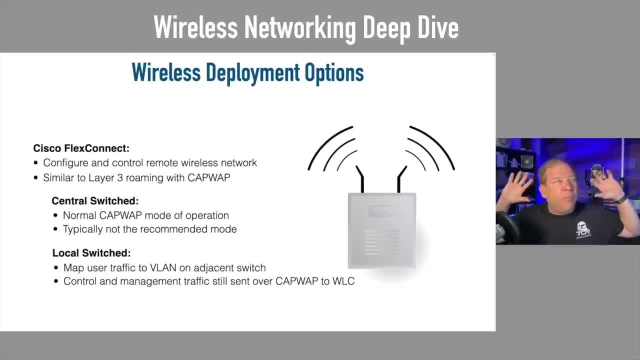 got a couple of access points and those access points need to communicate with between one another at their they're at a remote site. there's no need to send the data back to the headquarters and type WAN traffic, because really it's it's sending the same data twice over. that. 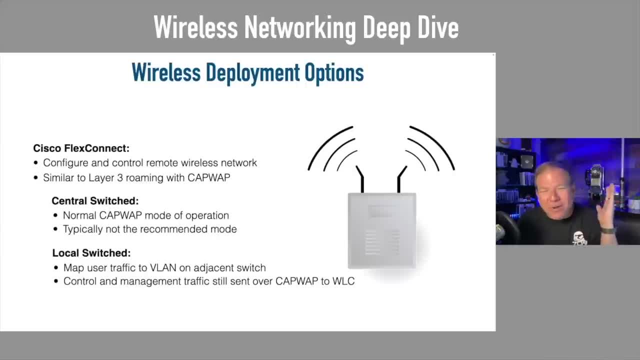 link. It's going back to the headquarters and then coming back. We probably don't want that, So that's called the local switched option of FlexConnect. Now you can set it up where- yeah, it's called central switched, as you see on screen- You can make all the data go back to. 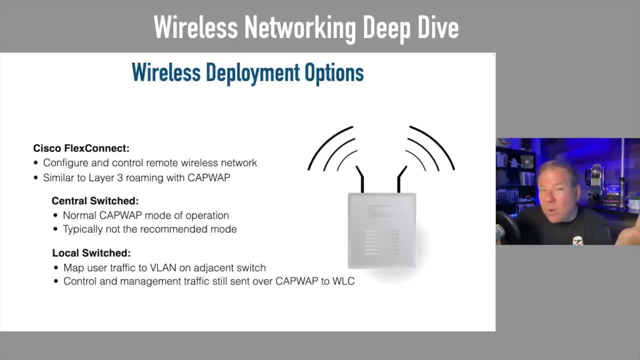 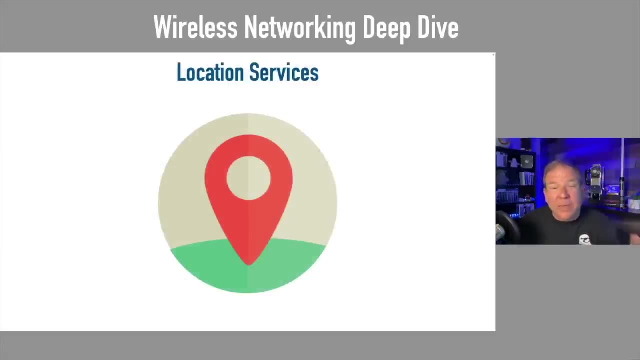 the headquarters. Maybe you want to run it through some sort of a security appliance. I'm not sure why you would do that. I mean that might be a reason, but in general you want to keep your local traffic local. It's going to save on bandwidth And besides just transmitting data, something else- our 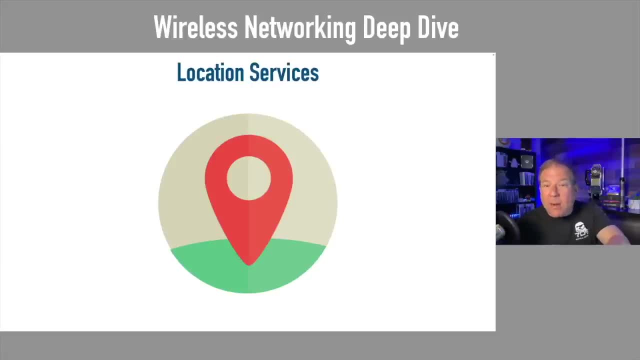 wireless networks will do for us is locate a wireless device. In fact, I was talking about Disney. I'm going to go to Disney tomorrow and we get to do that Guardians of the Galaxy ride that I was telling you about. Well, Disney tracks you based on your 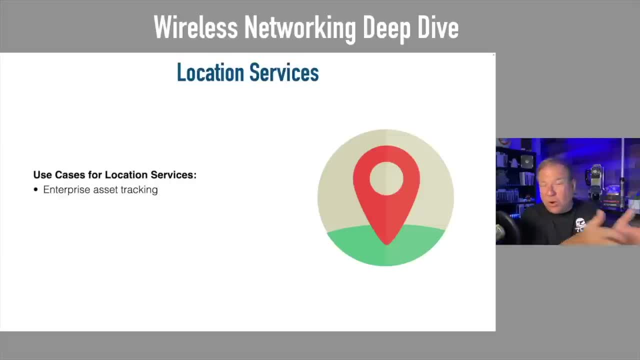 the people that wear the little magic bands. they can see where you are. So if there's a lost child, for example, they can locate that lost child If that child is wearing a magic band because it's able to do location services. same thing here We can have our wireless devices. 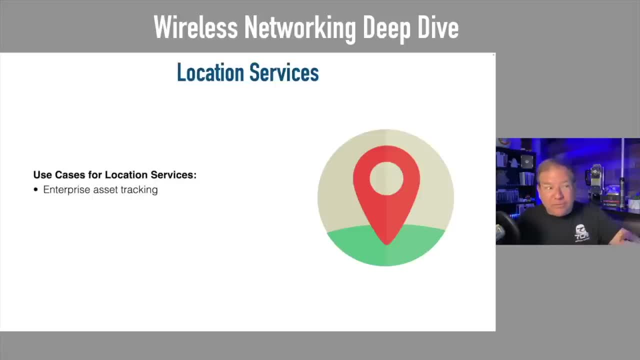 show up on a map and we can locate them with very high accuracy. This is good for asset tracking in an enterprise I know. I used to work for a company where one of the things I had to do was inventory. That was one of my least favorite jobs. I could not stand to do inventory because I 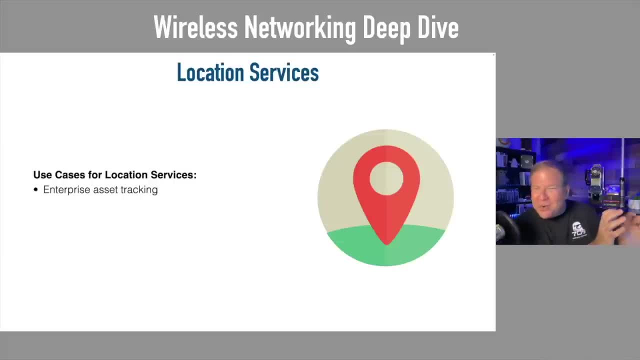 had to go to these offices and try to find the inventory ID tag on all these computers and printers. Well now, if they're wireless, I could just see them on a map and see that they're there. They're just going to show up And you might see this in a shopping area. This happened to me not. 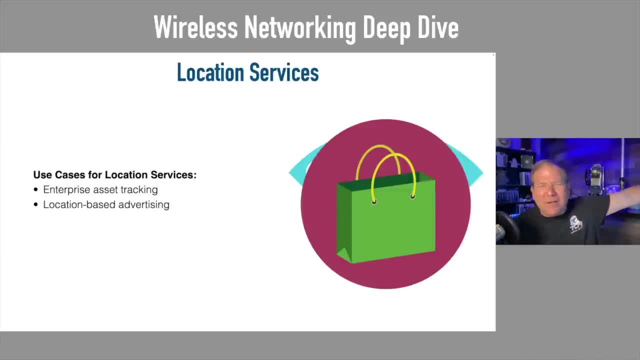 too long ago. I'm walking past the front of a store, maybe in a shopping mall, And I get this push notification on my phone about some sort of discount coupon that I had for that store that I happen to be in front of. 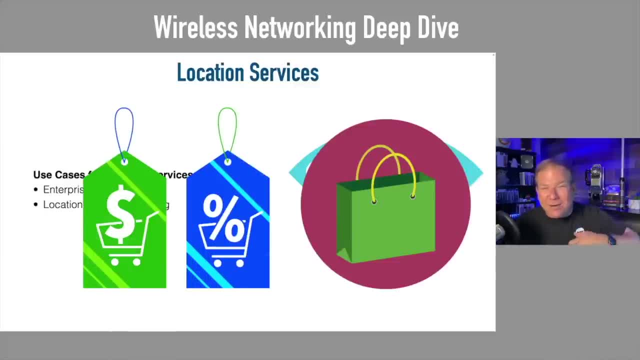 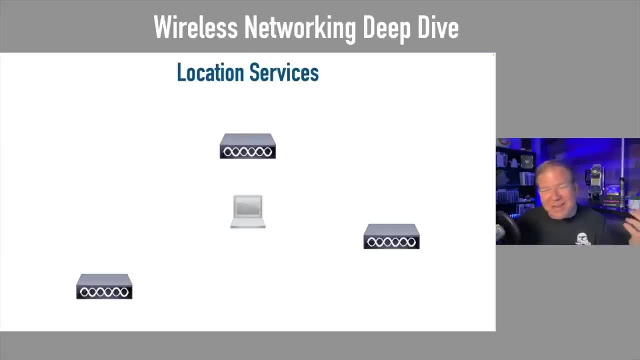 because maybe I joined that shopping mall's wireless LAN, So, based on my location in the mall, they could send me marketing messages. That's kind of interesting. Now there's a big misconception about how location services work, And I want you to be clear on this because you 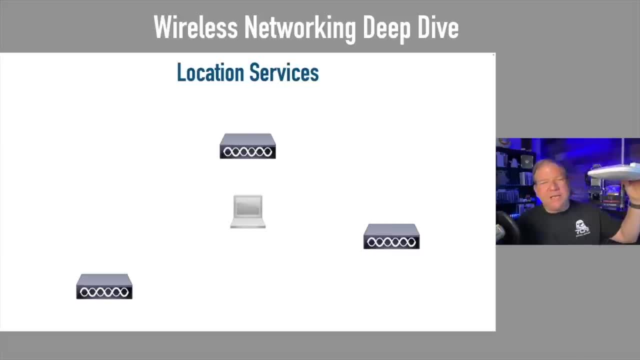 might think: okay, my phone is attached, I'm actually connected with access point and there's all these other access points around me, but I'm closest to access point one. So a lot of people think, and this is wrong. but a lot of people think, oh, it's going to say that. 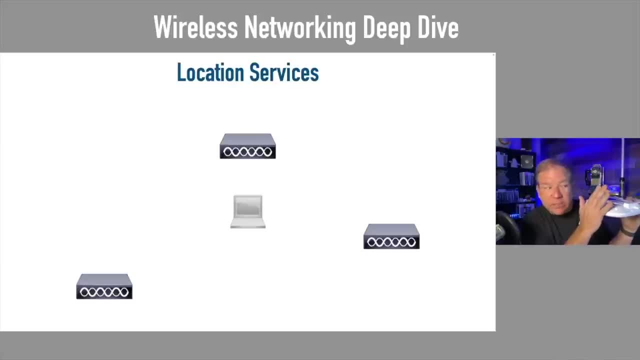 I'm somewhere close to access point one And it's going to be whatever that coverage area is, I'm somewhere in that area. Oh no, it's much more specific than that. Even though I'm associated with access point one, access point two still sees me. Access point three can still see me. 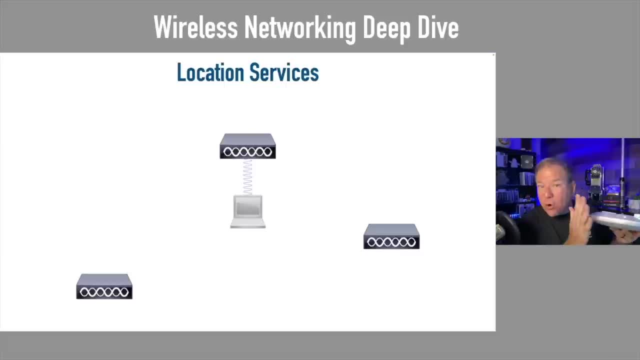 I'm not associated with them because I have a stronger connection with access point one And we can get mathematical here and we can determine with very high accuracy where I'm located. We can look at my signal strength. It's called the RSS, the received signal strength. 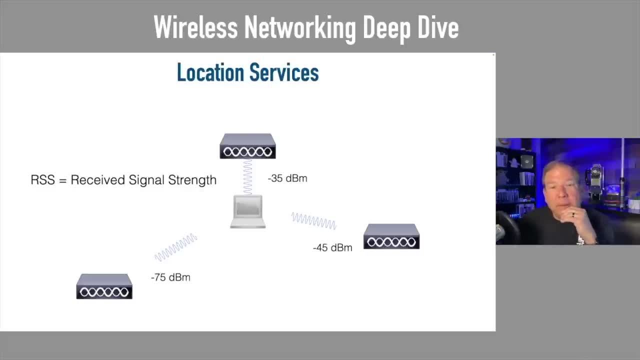 And we can determine how close I am to all these different access points. And it's just like if we were doing this in a geometry class, we would take our little compass and we would draw an arc out from each of these access points, saying: 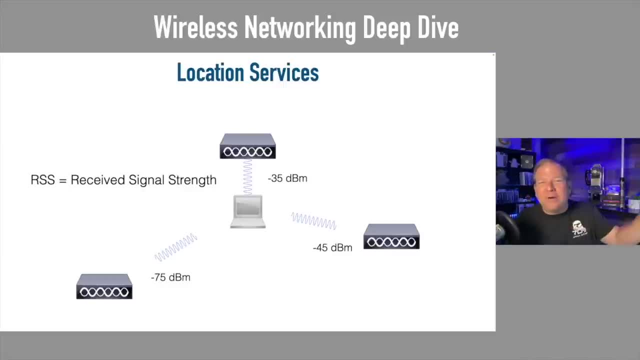 here's the negative 75 dBm coverage area And here's the negative 45. And here's the negative 35. And where those arcs intersected, that's where our device would be. Yeah, triangulation, as one of our students is saying on screen and are in the chats Now. location services. 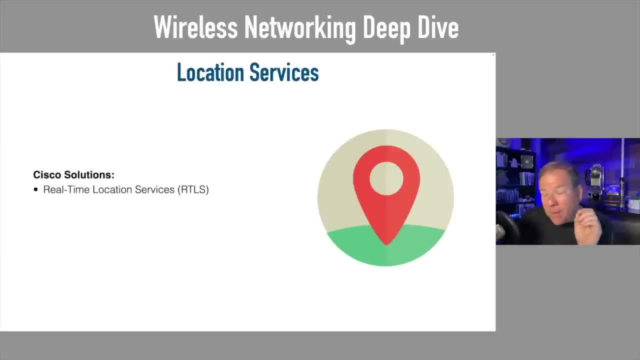 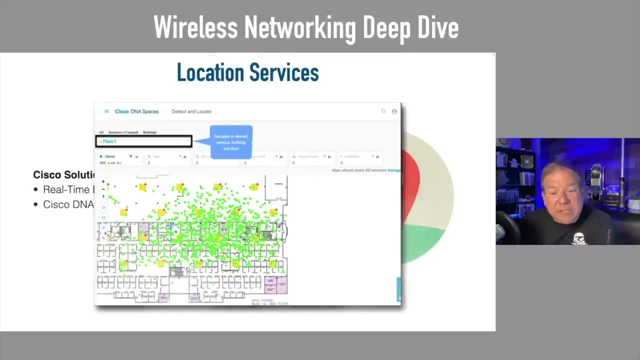 what does Cisco specifically offer us? Well, they've got a couple solutions. They've got more of a high-end massive enterprise solution and more of the mid-size solution. They have the Meraki solution. But at the high end large enterprise they have something called DNA spaces, And here's a. 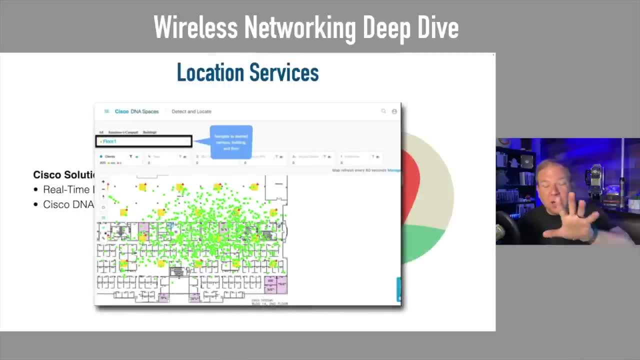 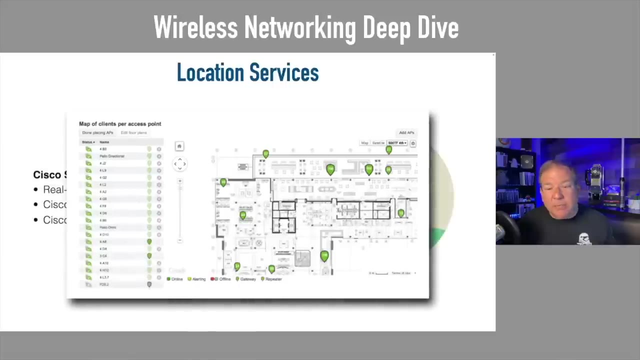 snapshot of what that would look like. You can see devices superimposed on a floor plan of a building, so you know where all of your different devices are going to be located. Now for the medium-sized solution, they have the Meraki platform. It does something very similar. You. 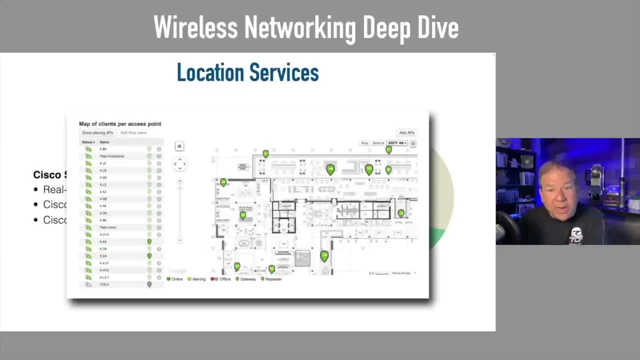 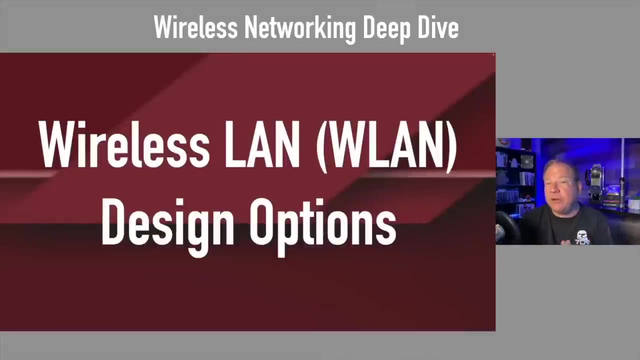 still got your floor plan. You can still see what devices are located on a floor of a building. So location services- that's going to give us an extra feature besides just the flexibility of roaming around with our device. Now we've got some different design options as to how we position. 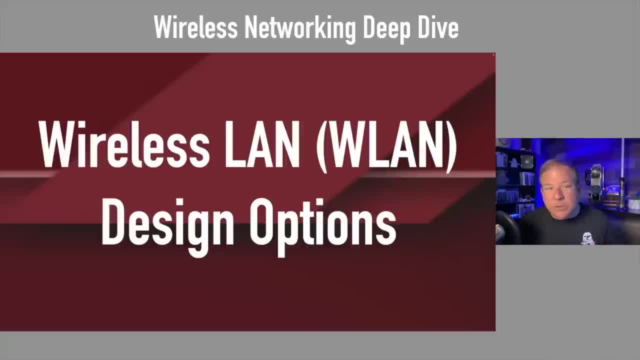 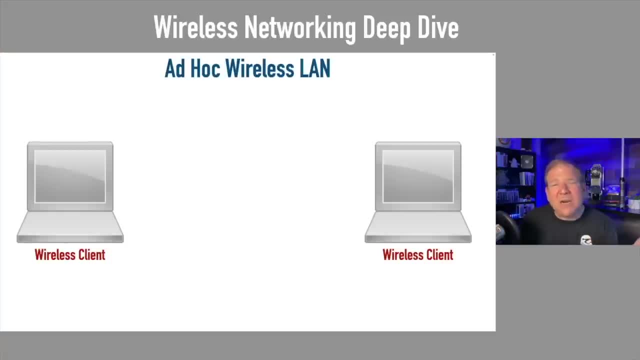 and locate these different access points, or do we even need an access point at all? Let's talk about some of those. One does not even involve an access point. Let's say that I've got here's an iPhone, And let's say: 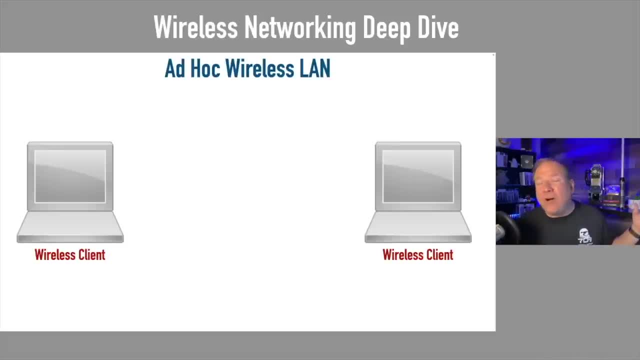 that I had another iPhone, I can be far, far away from an access point or any kind of a network. I could be out in a field somewhere. In fact, I remember one time we were on vacation and we were on a boat And I was trying to airdrop some files, some pictures from my wife. We just visited Notre. 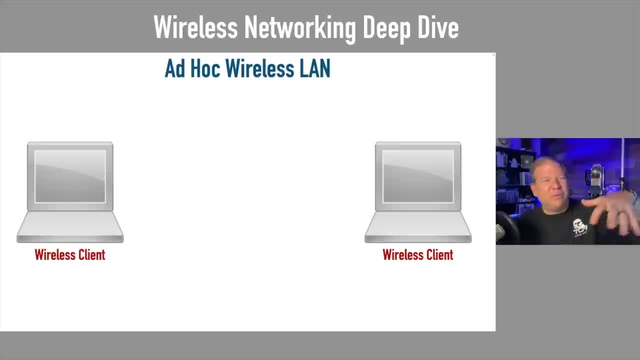 Dame And I had some pictures And we're on the River Seine out there And I'm trying to drop her some files And I thought: is this going to work? I'm nowhere near an access point. Yeah, we're just. 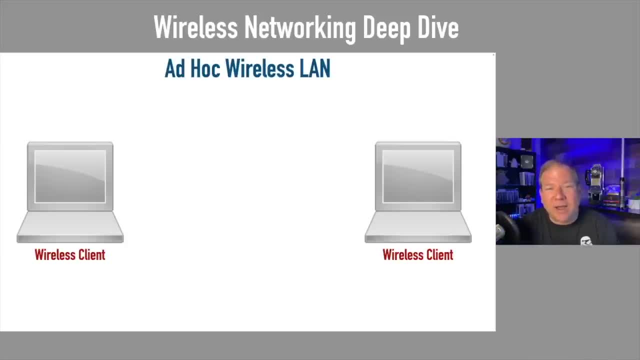 fine, That was called ad hoc networking. Ad hoc networking is where you have one wireless device talk directly to another wireless device without any infrastructure at all. Now, obviously that's not going to scale. That's just for the occasional, the ad hoc. 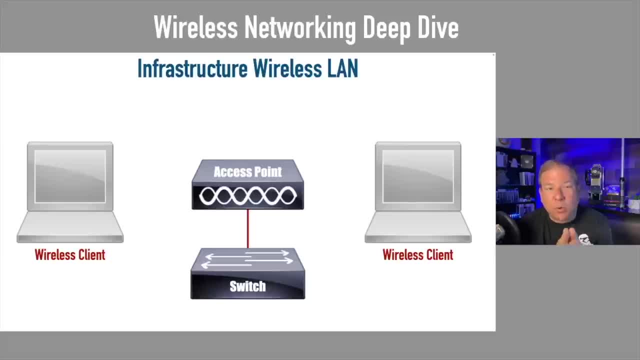 Connection that you might want to make. What we see much more traditionally in a home and in an enterprise is this: an infrastructure wireless LAN. With an infrastructure wireless LAN, you've got your access point And it's got an Ethernet port on it And it has a wired connection. 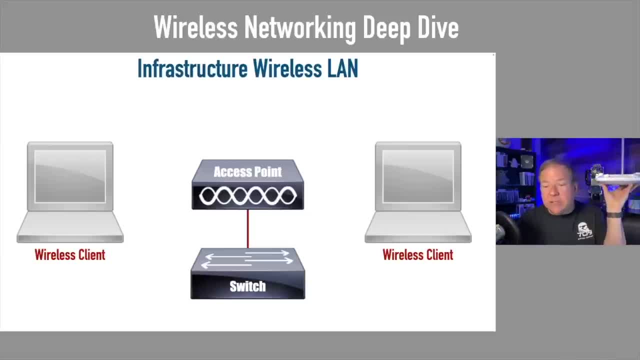 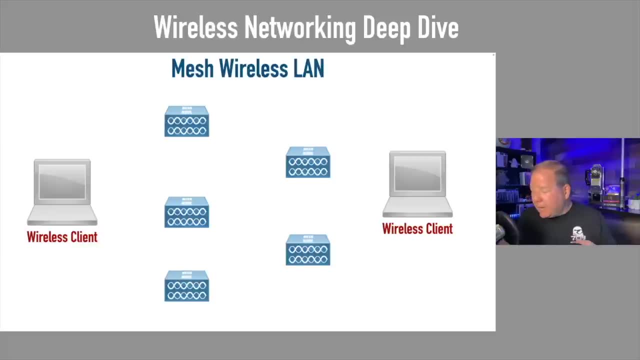 going to an Ethernet switch which gives you connectivity out to the rest of the world. So your wireless devices, they communicate with the access point, The access point communicates with the switch. Now, that's not going to scale. That's not going to scale, That's not going to. 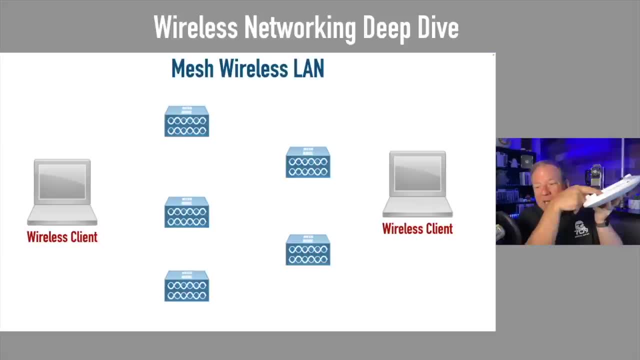 work, And that assumes that you're going to be able to take this Ethernet port in your access point and get it to an Ethernet switch. Sometimes we're not in close proximity to an Ethernet switch, So what do we do then? If I don't have a switch to plug it into, maybe I'm out in the middle of. 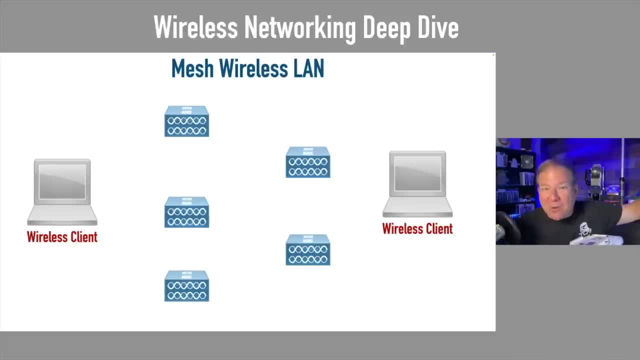 a parking lot somewhere And I want the guard shack out on a parking lot to have wireless connectivity And maybe the parking lot itself we want it to have wireless connectivity. I don't have Ethernet running to the parking lot. What am I supposed to do? 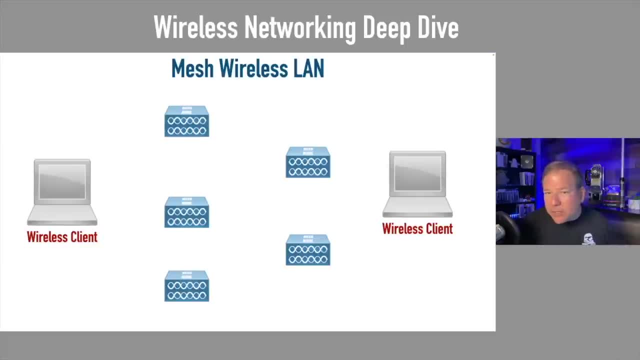 Well, we could use something called a mesh topology. With a mesh topology, as long as you can get power to this, and we could do that through just a power brick, a transformer. we could get power to this guy by just plugging it in And it would receive data from an access point, maybe back. 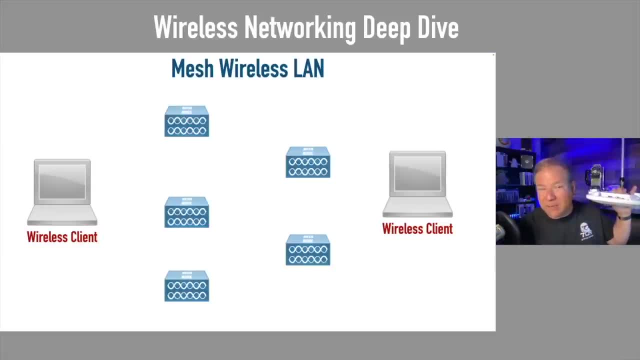 at the main building, Then it could run the data from the main building, And then it could run the data from the main building, And then it could run the data from the main building And then it could regenerate that signal and send it out, giving us coverage around that parking lot and giving 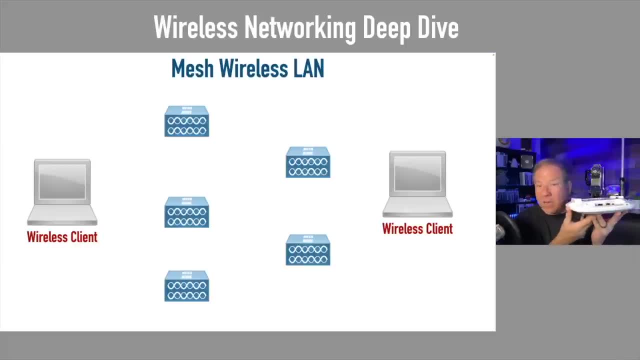 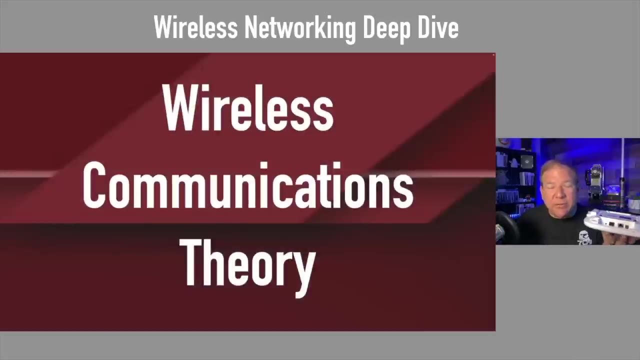 coverage to the guard shack. So if we're not necessarily close to an Ethernet port, but if we can receive a signal coming from another access point, we can regenerate that. So with a mesh network we're not necessarily connected in to an Ethernet network. Now we're going to get a little. 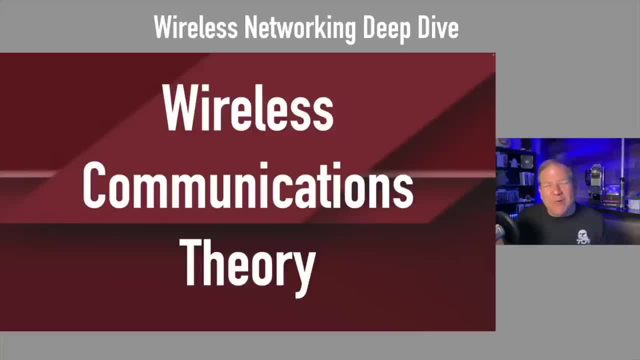 bit technical here. I saw somebody before saying: yeah, I want to go deep here. I don't want to go deep here. I don't want any lightweight stuff, No milk. I think they said They wanted to get into some of the meat. Well, one of the things we like to do here at KW Train is, however, complicated. 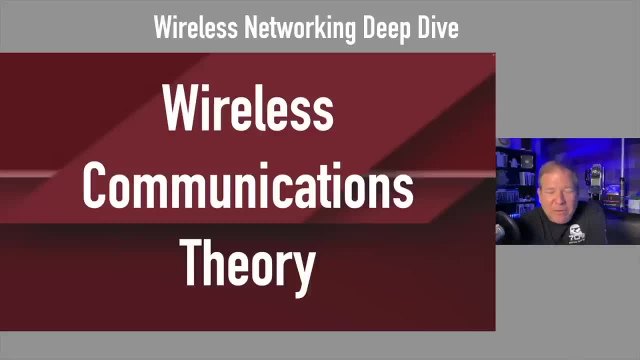 something is: we're big on simplification. So I'm going to do my best to simplify for you some wireless communication theory, And I'm not just doing this because I geek out about this stuff, which I do, by the way. By the way, my degree it's in electrical engineering. 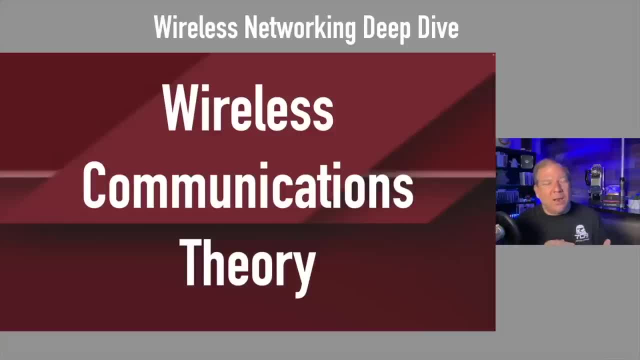 and I spent two semesters going through electromagnetic fields and waves and I geek out about all this stuff. But I realize we're not going to be doing calculus here. You don't need to do that for the exam, So I'm going to do my 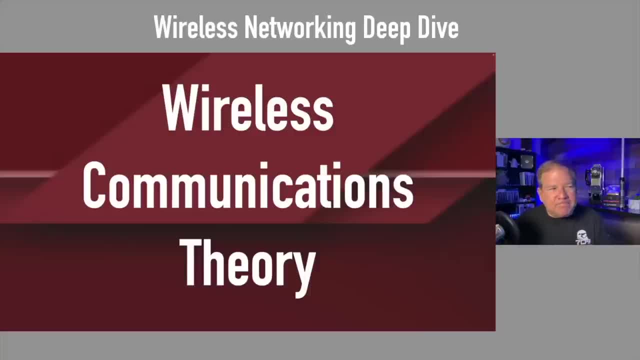 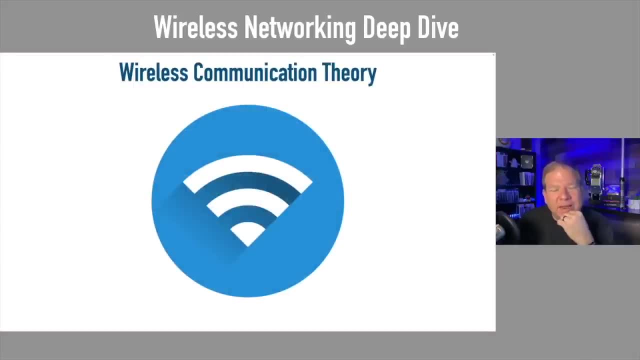 best to simplify some of these theories for you and have it make sense to somebody That's not an engineering candidate. So let's talk about wireless communication theory and how we actually radiate data out of an antenna like this, In fact, let me take, let me unscrew. 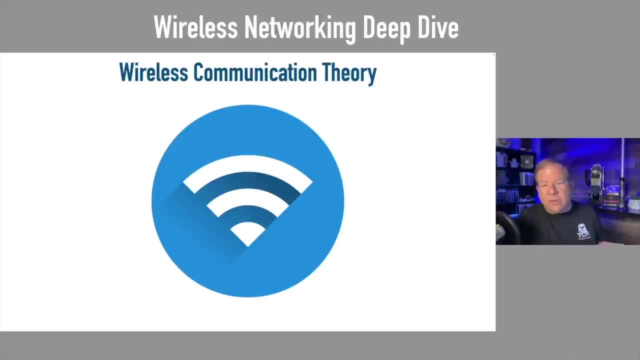 this little antenna so we can use that as a visual aid. But the first thing I want you to think about is this term that we hear all the time, called the electromagnetic spectrum, or we talk about EMI, electromagnetic interference, or electromagnetic waves. Why do we say electromagnetic? 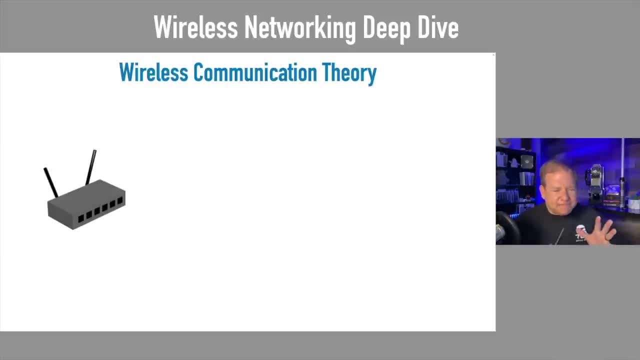 Because there is a tight relationship between electricity and electromagnetic waves. So we're talking about electricity and magnetism. It was back in the- I think it was back in the 1830s- Michael Faraday, he came up with this, with this discovery that proved this close relationship. 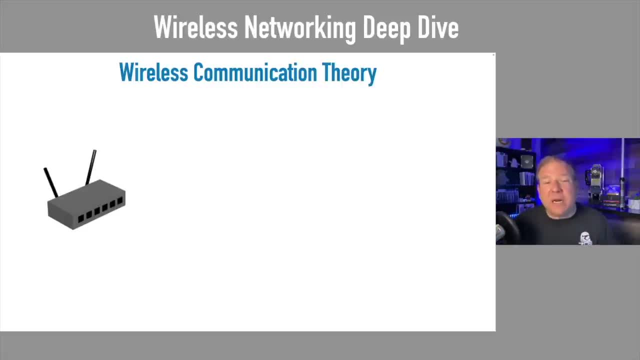 with electricity and magnetism. Have you ever done this on the science class? Have you ever had like a metal? this is a pen. but if you had, like a metal nail and you rolled a bunch of wire around it and you applied a battery to each end of the wire and you rolled a bunch of wire around it, 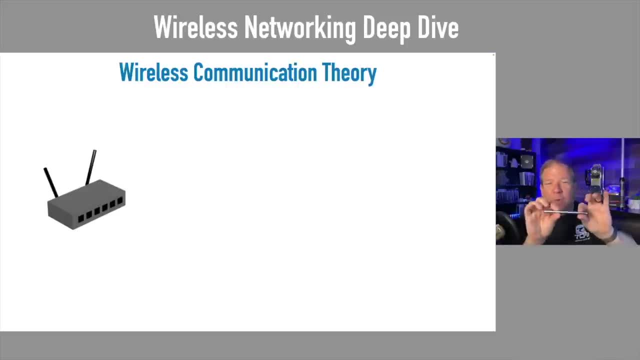 or tell me in the chat what does that do. If I put a coil of wire around a metallic object, like a nail, and I apply voltage to that coil of wire, what does that nail become when I do that? Go ahead and chat that in, if you would. Yeah, exactly, It's going to turn into. it's not a Faraday gauge. 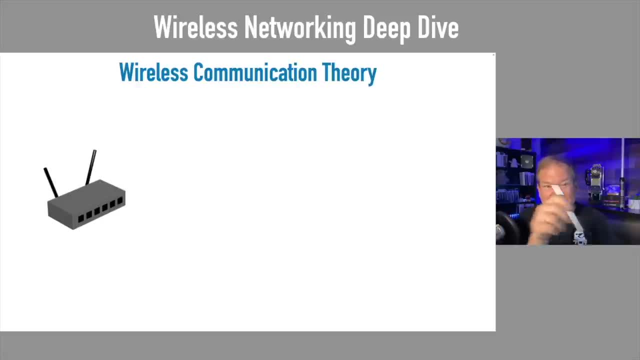 it's going to turn into an electromagnet where you can actually pick things up with it. Or if you've got a bar magnet with a north pole charge and a south pole charge and you run this bar magnet back and forth through a coil of wire, that's going to create current in the wire. So 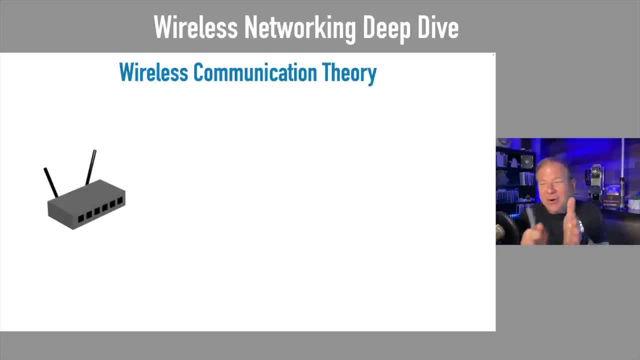 magnetism creates electricity. electricity creates, creates, creates magnetism. So there's this tight correlation. In fact, when we send a radio wave out of one of these antennas, we're going to be sending an electric field. think of it going vertically. 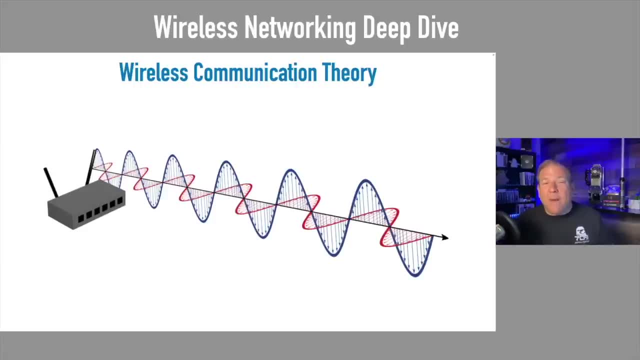 kind of like a sinusoidal vertical wave, but orthogonal. Now here's the term we're going to be using in the wireless network: orthogonal- You might've heard that in high school. That means at right angles too. So if I have an arm that's vertical and I put my other arm like this: 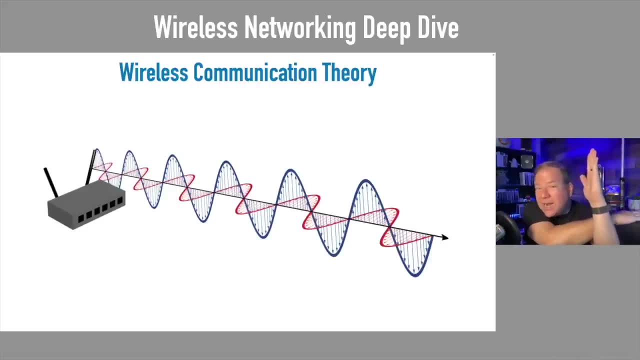 my arms are now orthogonal, They're at 90 degrees in relationship to one another. And that's what the magnetic field is. The electric field it's going up and down. the magnetic field It's going back and forth. One produces the other and we're going to have this electromagnetic. 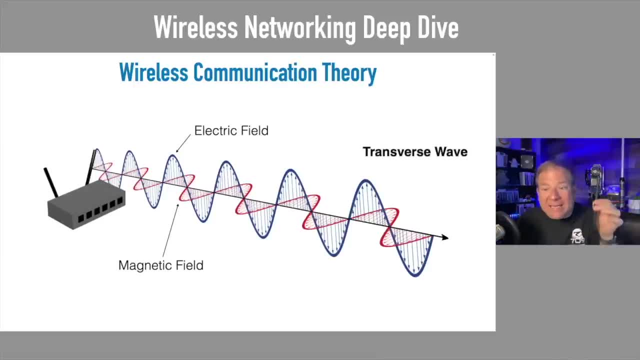 radiation coming out of an antenna to create a transverse wave. Now this brings up a huge question. And that is okay, I've got. I've got electricity running down a wire in my home for electricity. Is that an antenna? Not a very good one? The question is: what makes this electromagnetic wave be? 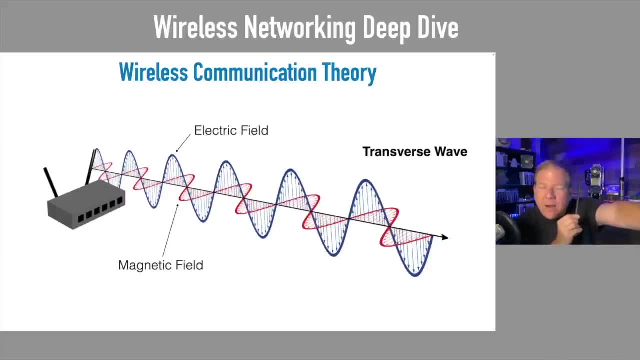 transmitted outside of the wire. Huh, There was a gentleman. I think it was 1887, Heinrich Hertz demonstrated this: how you could actually transmit electromagnetic waves out of an antenna. And here's one way that it works- Antenna theory, by the way, when I was in college, 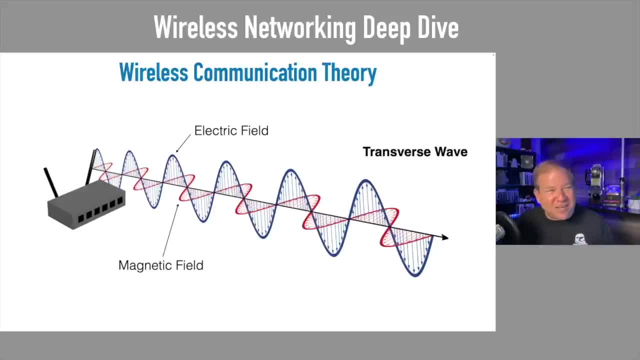 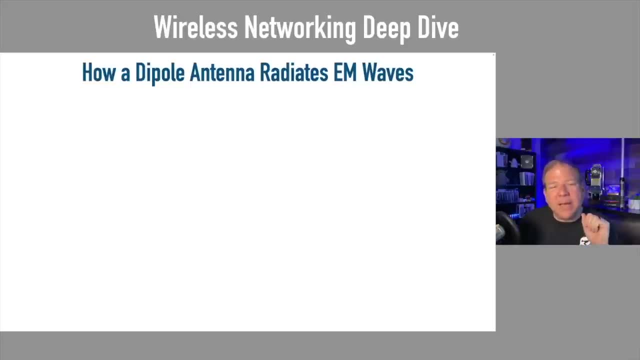 antenna theory was one of the most complicated things I studied. It got super, super mathematical. But I want to give you just a taste of what that's like. Let's talk about a simple antenna, like a dipole antenna. We'll talk about antenna types today. You need to know that for the 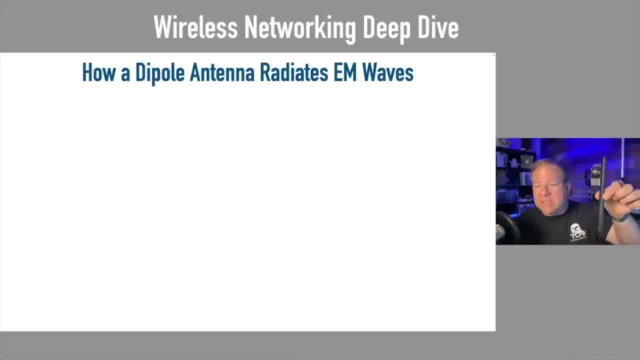 Encore exam, by the way, antenna theory- But this is a dipole antenna. Let's talk about how a dipole antenna works First. let's imagine that I've got some sort of antenna. I've got a dipole antenna. 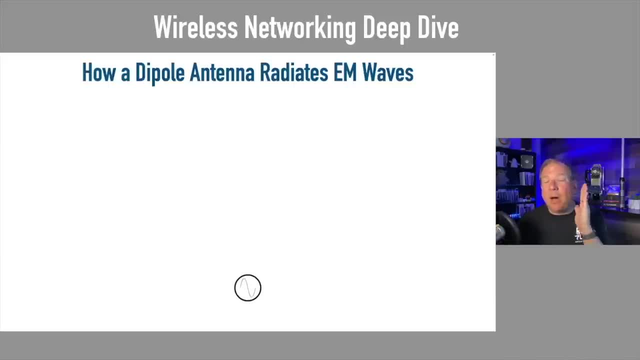 I've got a device that's going to generate positive and negative charges on two pieces of wire. So you see, that's my little device with the little waveform down at the bottom, And we're going to connect to that two pieces of wire And on one piece of a wire we're going to apply. 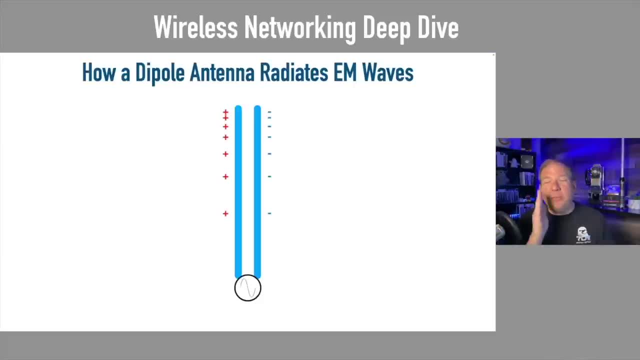 a positive charge. On the other piece of wire. we're going to apply a negative charge And positive charges. they want to go to the negative charge side. So we've got. we've got the charge coming down and then the charge going up- the other side. 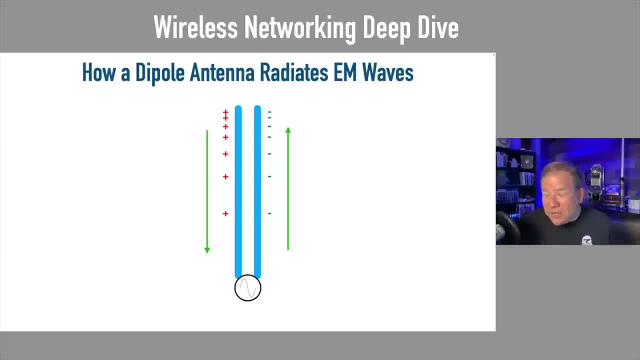 Is this an antenna? No, it's not, But not a good one anyway, because these two wires are side by side, One direction and the other direction. they cancel each other out. So how do we radiate? how do we radiate radio waves from these wires if they're canceling each other out? 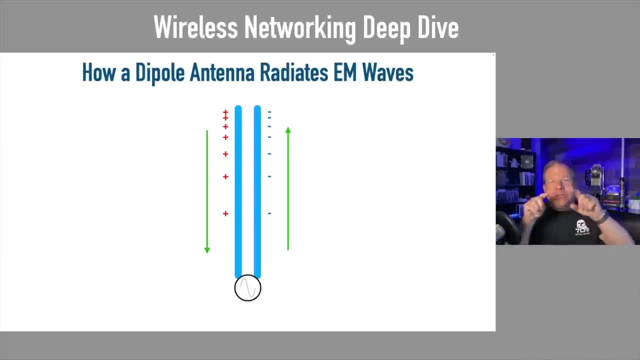 What if we took those two wires going up, we took the very top of the wires and we bent them sideways like this? Let me show you What if I- oh, by the way, yeah, I was going to show you that- that it alternates back and forth. So positive, negative, positive, negative. We're going back. 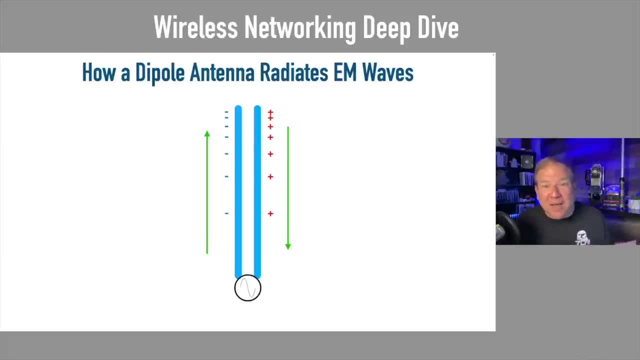 and forth. We're switching the charges, but they cancel each other out, So it's not going to radiate anything. But with the dipole antenna we sort of bend down those wires. So check this out Now, when I apply a positive charge to one side. 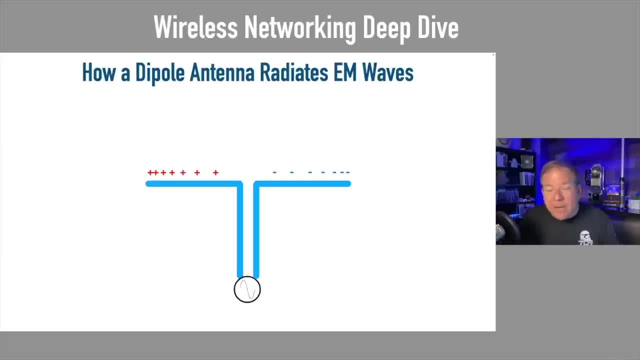 and a negative charge to the other side. notice how the positive flows to the negative. Look at that very top plane. You see how things are bent down. The top plane. it's now all going in one direction. They're not canceling each other out. 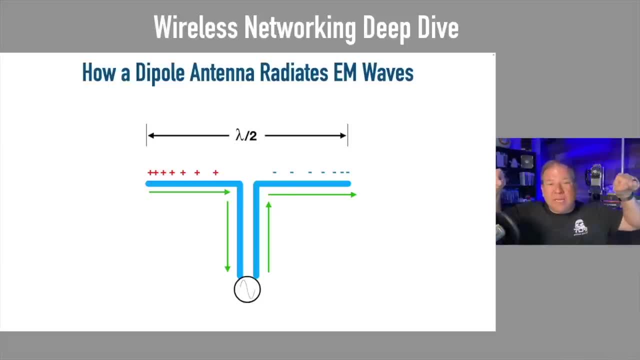 Now the length that we're talking about there, where we bend the wires out, that should be one half of the wavelength. That's one half of the wavelength And we'll talk about the frequency And the wavelength and how that ties in a little bit. But the lambda you might want to put in your 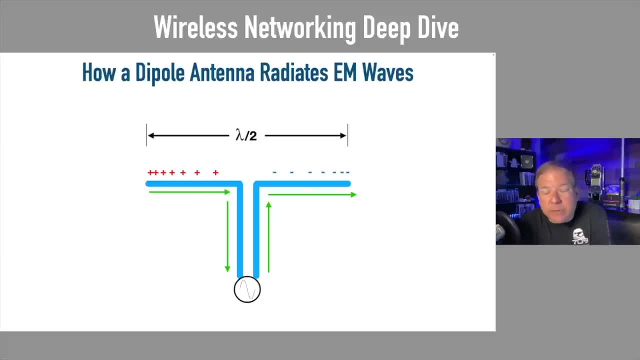 notes. that represents the wavelength typically measured in meters or millimeters, But it's one half of the wavelength And when you do that, that's going to generate half a wavelength. And when you oscillate, when you go back and forth between the positive and the negative charges, 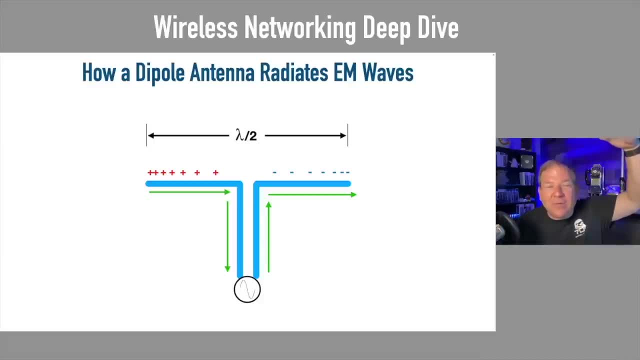 it's going to start radiating out these radio waves. It works in reverse as well. You'll be able to receive those radio waves Now. any questions right now? Go ahead and chat those questions in, if you do, because I know this is a big concept. We're talking about wireless networking all day today. 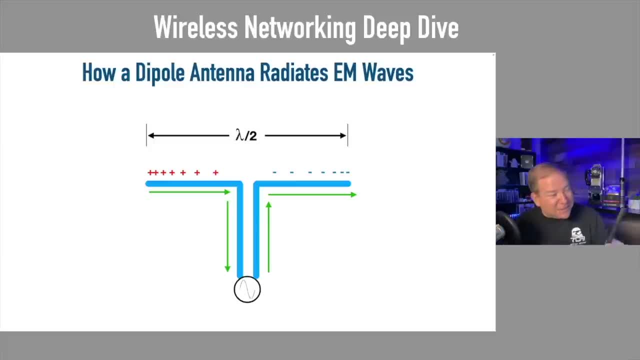 And a fundamental thing to understand is: how does that work? How do I send a radio wave out of an antenna? So if you notice- and I'm not sure you can see it on camera- but when I unscrewed this little dipole antenna, there is a connector in the very middle. 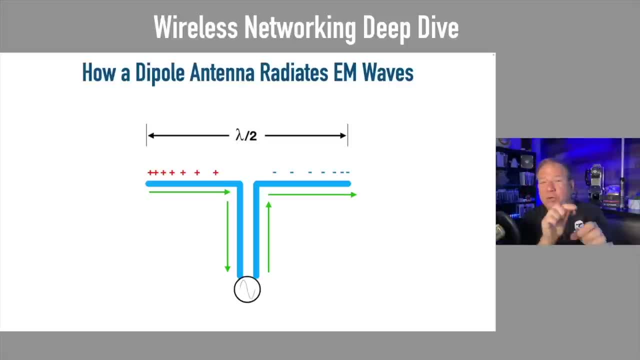 And then there is like a shielding around it. So there are two conductors going up in here And it goes about halfway, And then it breaks apart And one half of the wire goes this, or one wire goes this way, one wire goes this way. So we're actually radiating the signal. 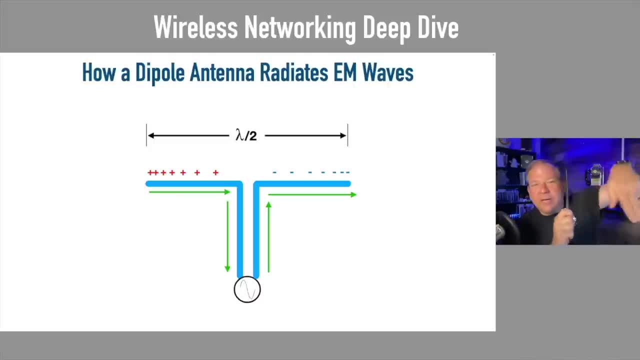 out this way out from the antenna in all directions. We'll talk more about that when we get into the antenna theory. But I needed you to understand how we get these electromagnetic waves off the wire. How do we transmit them out into space? How do we transmit them out into space? 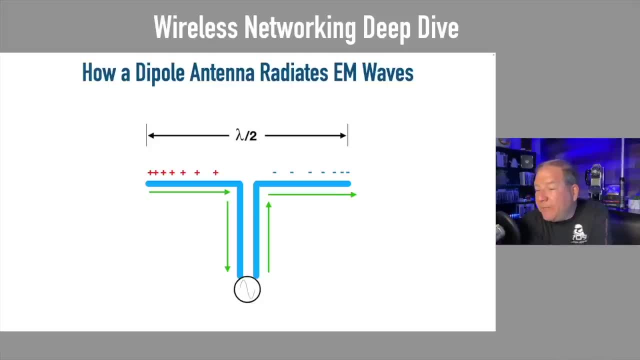 Let's see the propagation of the signal. is the electric field? It's actually both. It's an electromagnetic waveform that's being transmitted out. So it's actually both. Let's see. somebody said I took radio instrumentation in 1981.. This is old hat, Yeah, I realize for some. 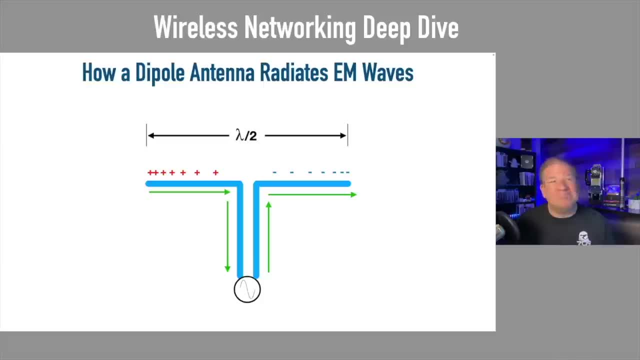 of you. if you have your FCC first class license, you know this like the back of your hand. I want to get everybody on the same sheet of music, though, And so we're going to try to cover some of these things, And we're not going to go deeper than this, because it gets super, super complicated. 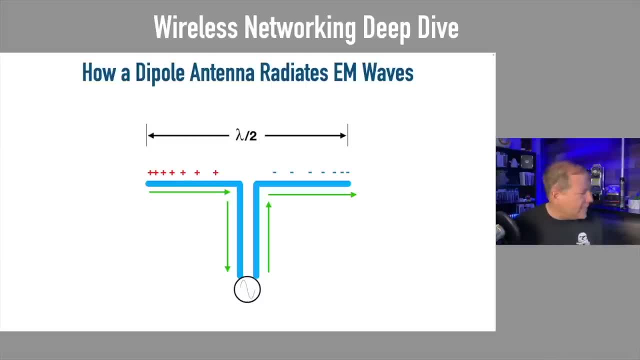 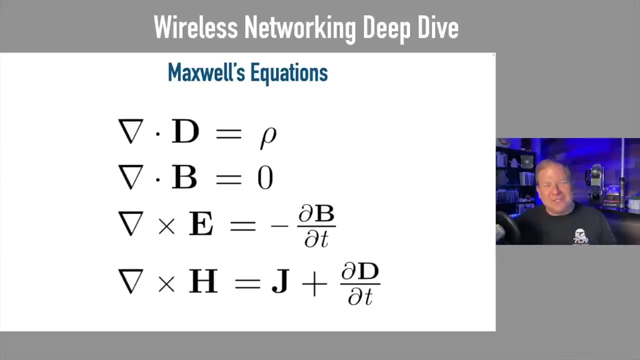 if you get way, way deep into antenna theory. But any other questions? I'm just trying to take a look here. Yeah, Looks like we've got most of those covered now- Awesome. Well, let's take a look at Maxwell's equations for a second. I just wanted to bring this up because electromagnetism and how. 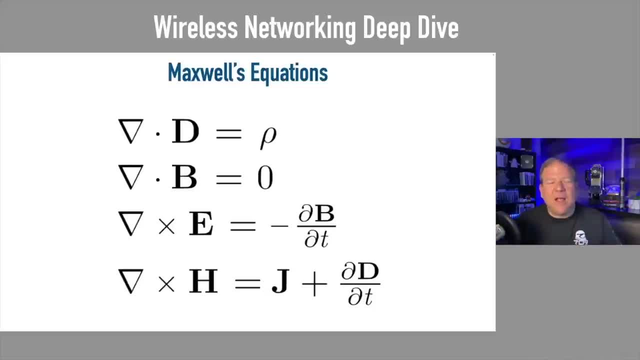 electric fields cause magnetic fields and vice versa. that is all governed by these things called Maxwell's equations, And this is what I studied for two semesters in that: electromagnetic fields and waves theory, all the different things that you see on screen here. which brings me to my favorite joke in all of electrical engineering. 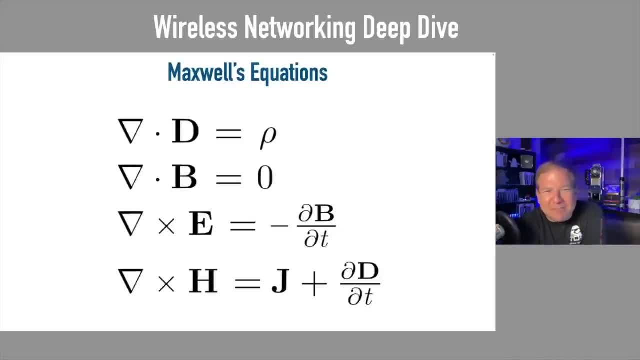 So if you've got some people that are taking advanced physics or you've got some double E friends, they might enjoy. this joke Here goes. There was an electrical engineering doctoral student and he went before the board where he had to go defend his thesis. And you've got this board. 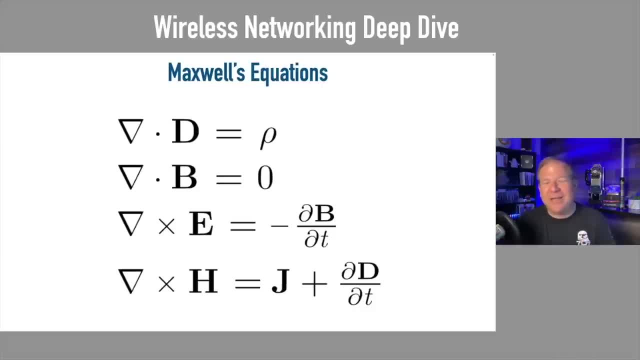 of professors asking questions to make sure he can qualify, And one of the questions they asked him is: can you list for us? can you list for us, Maxwell's equations? So this engineering candidate said, yeah, I got this. And he starts listing off all of these equations. but he made a mistake. 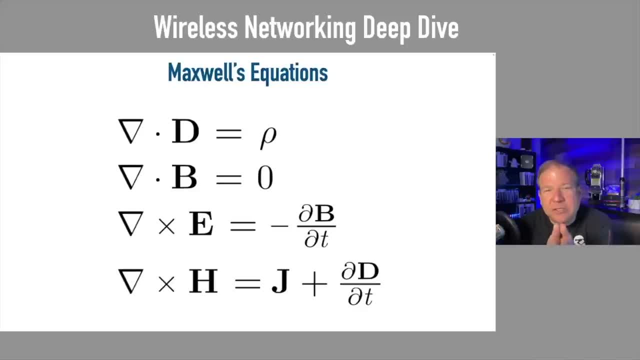 By the way, I should have mentioned these are not just equations for radio waves. These are sometimes called Maxwell's light equations because radio waves and light they're the same thing. We cannot see radio waves with our eyes, but they're all part of the electromagnetic spectrum, For example. 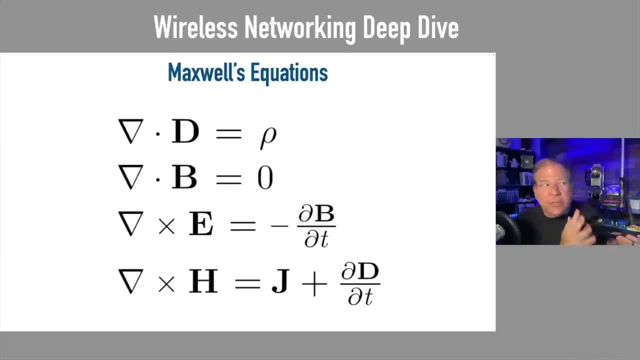 when we talk about our wireless access points, it's going to be using a frequency of something like 2.4 or 5 gigahertz. If we're talking about light like the color red, that's one of the longer wavelengths It has a frequency I think it's about 430 trillion hertz. 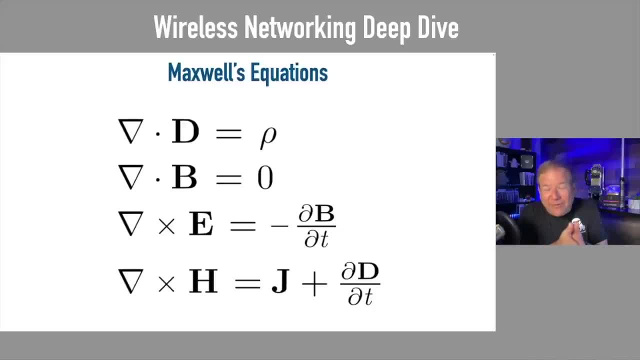 So it's still an electromagnetic wave, but it's just a lot faster. So it's also a light equation. That's his doctoral candidate. to list off Maxwell's equations, He does, but he makes a mistake. He forgets to say the negative sign on that third equation. And one of the professors 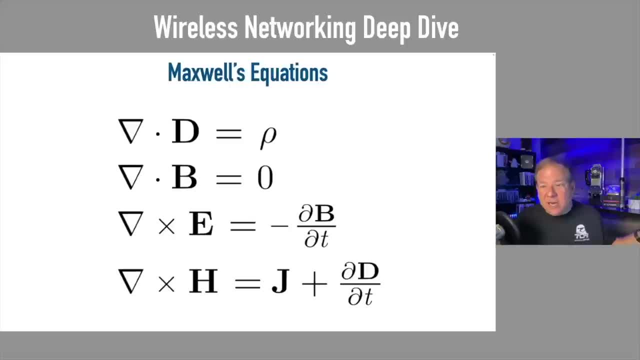 just on, the board goes nuts. It's like how could you be so stupid? You left off the negative sign. What are you thinking You expect us to give you a doctoral degree? And the doctoral candidate is kind of taken aback. He thought that was a bit of an overreaction And he said: yeah, I left off the. 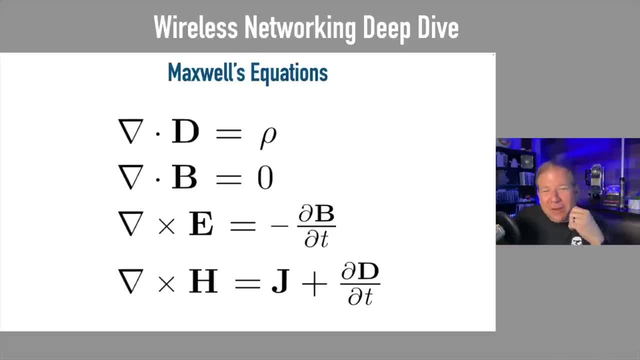 sign: What's the difference? And the professor says: what's the difference? It's the difference between night and day. Get it Light. equations: negative night and day. This is one-way communication. I'm visualizing that everybody's cracking up right now. when I gave the punchline, 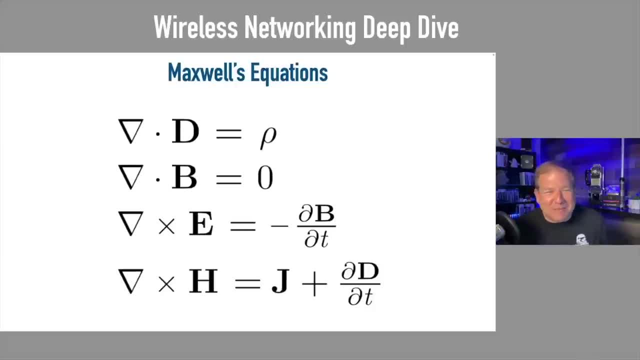 but tell that to your EE friends, your physics friends. They might get a kick out of that one, But that's my favorite joke. That's one of the few things that I actually remember from my degree after going to school. So that's one of the few things that I actually remember from my degree after going to school. 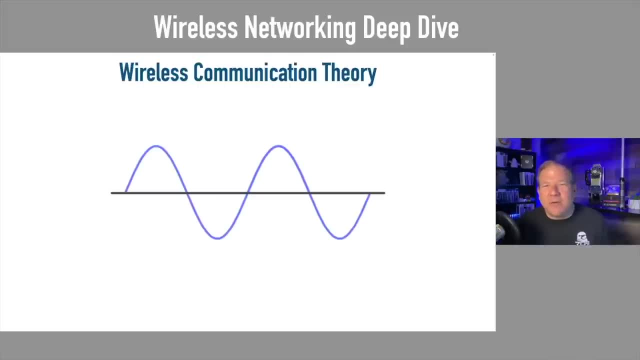 to college, But Maxwell's equations. that's going to govern all these things we're talking about. Now. let's define some terms. We have a waveform that goes up and down, So it goes positive, then it goes back to zero, It goes negative and back up to zero When it makes that complete cycle. 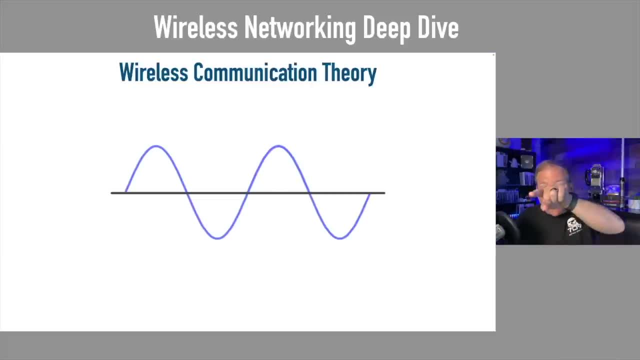 all the way up through the zero and then all the way back up. that's one cycle, And the number of cycles that it makes in a one second period of time is called the frequency. So notice this waveform on screen. We've got a one second period of time. 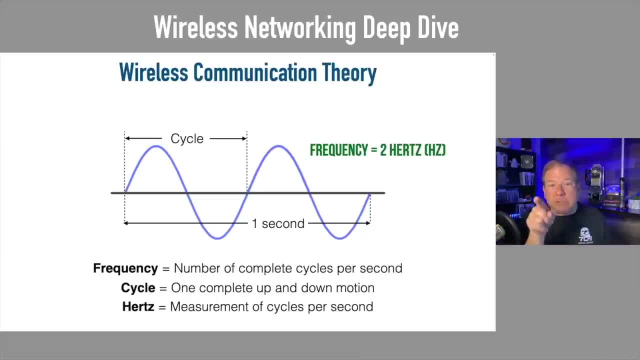 and there have been two complete cycles. We went up and down and then back up. That's one cycle, and then we did it again, So we did two cycles per second. That's a frequency of two cycles per second, which we also call Hertz. Hertz is a unit of measurement of frequency. It's the number. 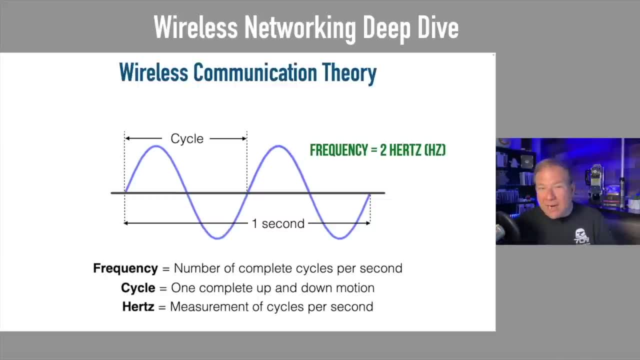 of cycles we make per second, named after Heinrich Hertz that we mentioned earlier, And we really need to understand that as we get into talking about all the different channels and sub-channels and frequencies that are going to be used by our wireless communication devices. 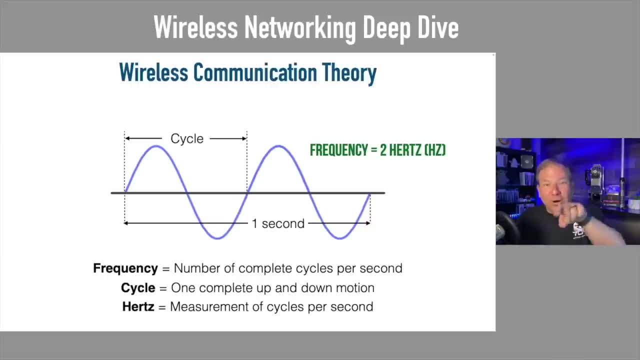 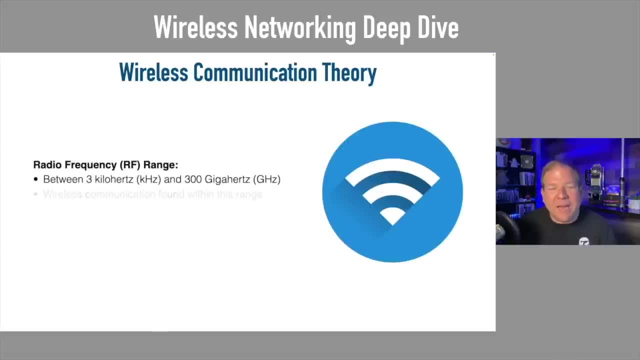 So here we've got a two hertz signal. We're going to be dealing with like gigahertz, billions of hertz when we talk about our wireless communication And specifically, we have two different bands of communication that we're going to be concerned about today. 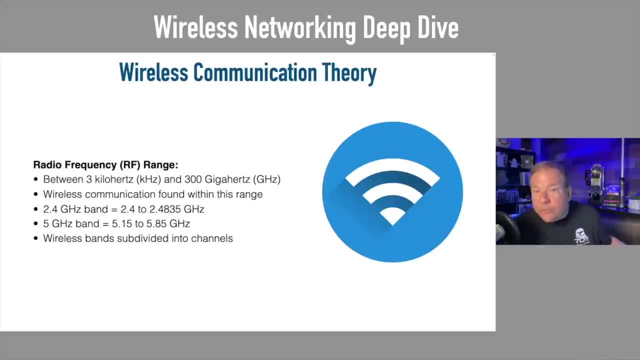 for your notes. Those are the 2.4 gigahertz band and the 5 gigahertz band. Now, a lot of people misvisualize this, so please make sure you get this right When we say this is operating at 2.4 gigahertz. 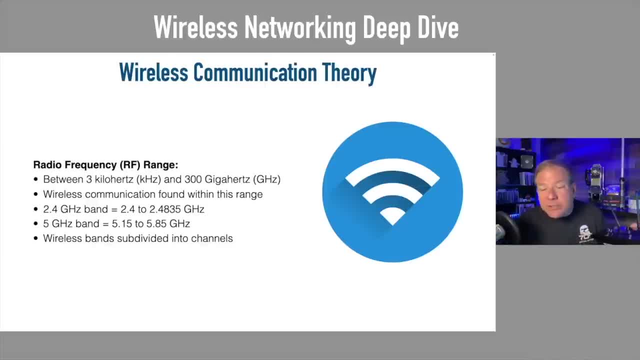 it's operating on a range of frequencies that are close to 2.4 gigahertz. It's actually a range of frequencies. You see it on screen. When we say the 2.4 gigahertz band, we're not talking about. 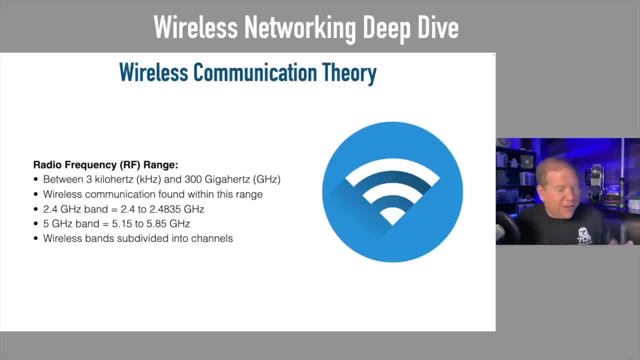 just exactly 2.4 billion cycles per second. We're talking about 2.4 gigahertz, all the way through 2.4835 gigahertz. When we talk about the 5 gigahertz band, we're not talking about exactly. 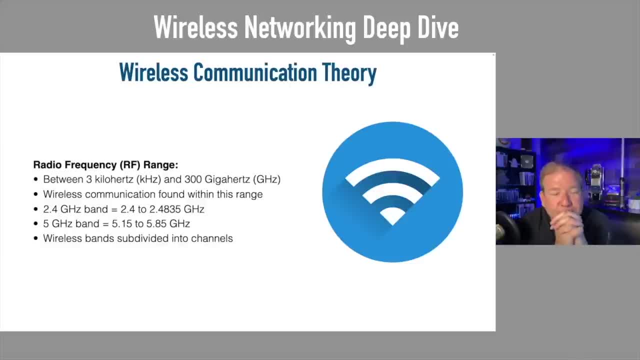 We're not talking about exactly 5 gigahertz. we're talking about a range of frequencies and you see those on screen. And when we say we're using this band of frequencies, if we're sending out bits of data- ones and zeros- through the air today, anyway we're not taking up that entire band. 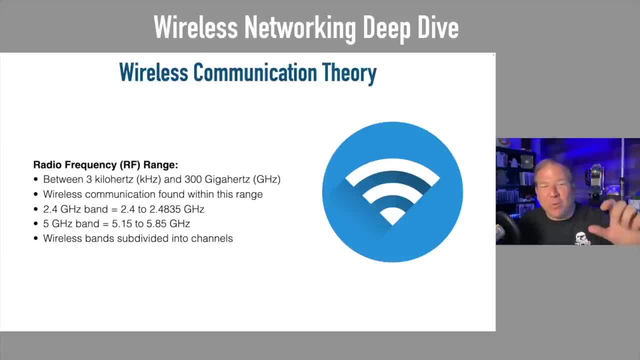 of frequencies to send a binary zero and then a binary one. No, we take that channel that we're using, we're going to divide it up into different channels And then, within each channel, we're going to divide that up into subchannels And we're going to be able to send different communication. 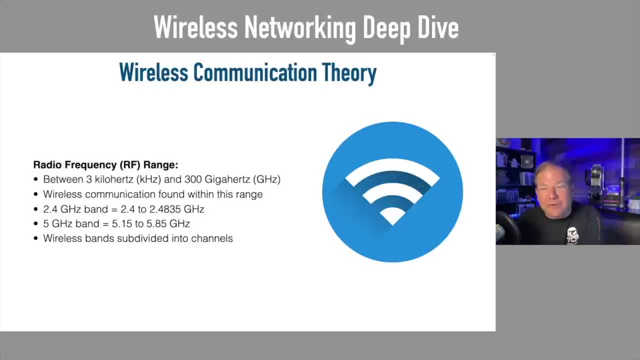 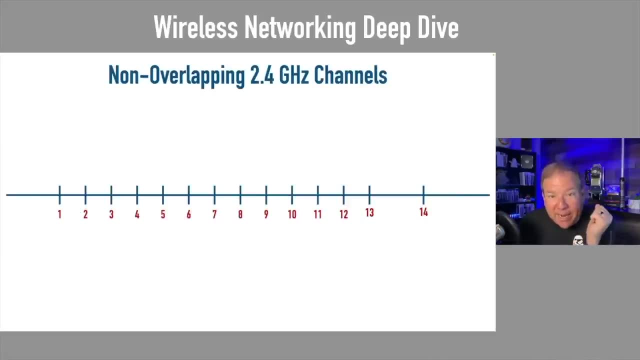 streams on the different subchannels that are part of different channels. I'll give you a visual of that here in just a few moments. First, let's take a look at the 2.4 gig band. We have 14 channels that are defined in the 2.4 gig band of frequencies And we know that we don't want to have 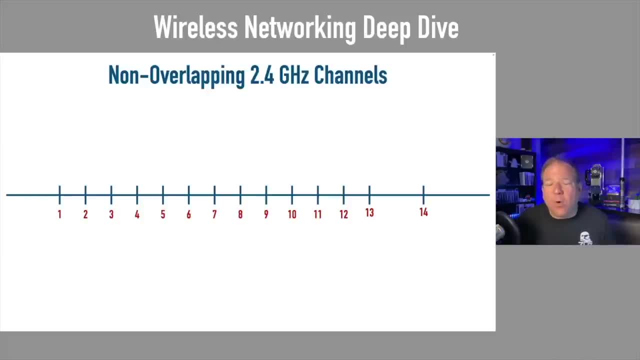 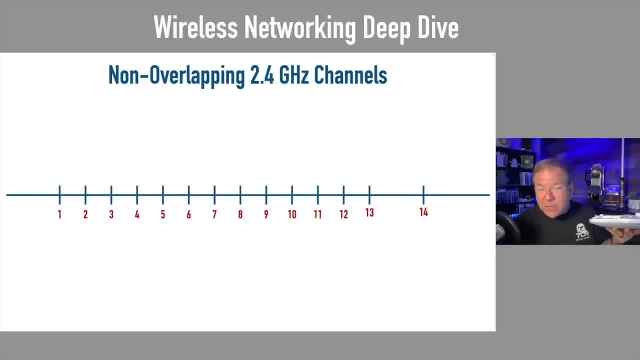 two as well. that's going to be interference And that can cause all kinds of problems with your communication. You're using the same channel, So we know we shouldn't use the same channel. but here's another common point of confusion: A lot of people realize that you should not use. 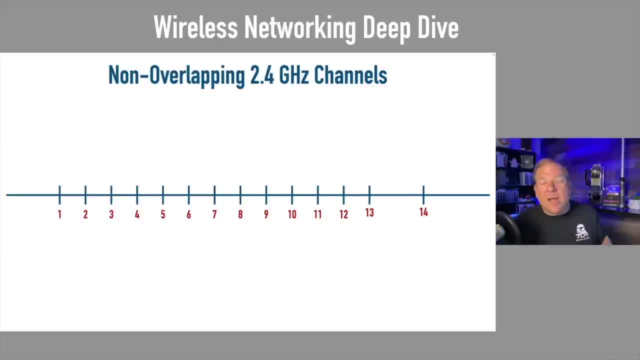 the same channel, but they say, well, I'll just use channel three, My neighbor's using channel two, I'll use channel three. That doesn't overlap- Oh yes, it does- When I say I'm using channel one, for example, or channel six. that's my center frequency. So it's actually sort of like: 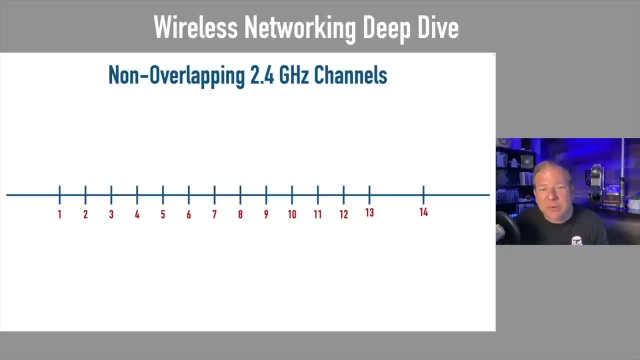 a Gaussian distribution curve. That's my center frequency. Let me, let me show you how to do that. I'm going to show you how to do that. I'm going to show you how to do that. Let me show you. We have five megahertz of bandwidth between each of these. 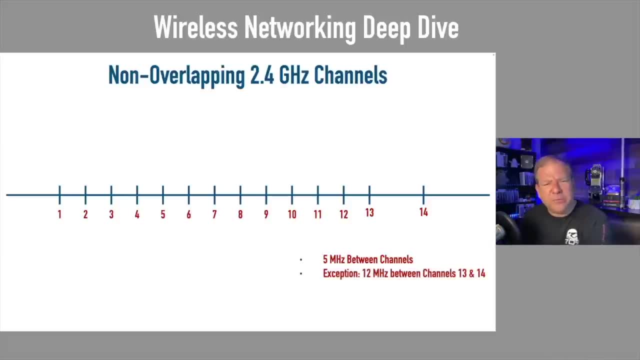 channels. There's one exception: channel 13 to 14.. You see it's kind of spaced out larger. There's 12 megahertz there. You're probably never going to have to deal with channel 14,, by the way. 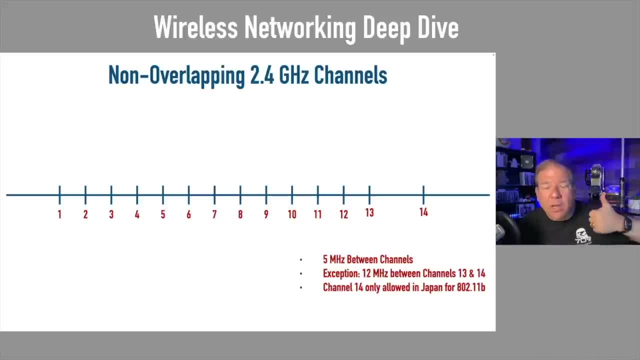 Channel 14 is only going to be used if you meet two criteria. Number one, you're in Japan And number two, you're using the very, very, very old 802.11b standard, which hopefully none of us are using today. So we can largely forget about channel 14 being there, But if I say I'm using 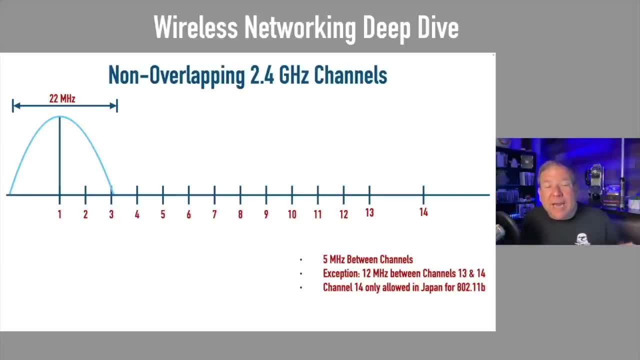 channel one. notice, I'm really using a 22 megahertz range of range of frequencies. The middle one is right on channel one, but I'm I'm extending into channel two and I'm extending a little bit into channel three. So if I tried to put my neighboring access point on channel two, 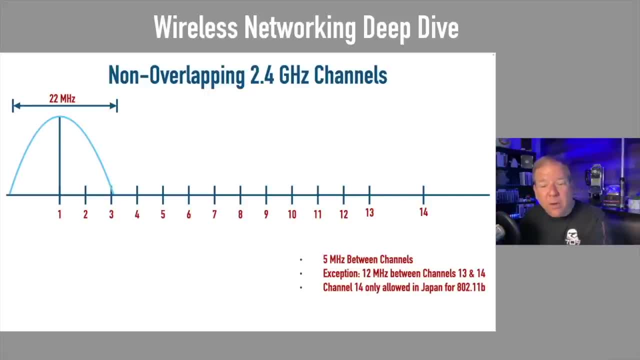 or even on channel three, they're going to be interfering with one another. If I put it on channel four or five, that's going to interfere. So how do we have non-overlapping channels in the 2.4 giga range? Here's the key for your notes. We need to have 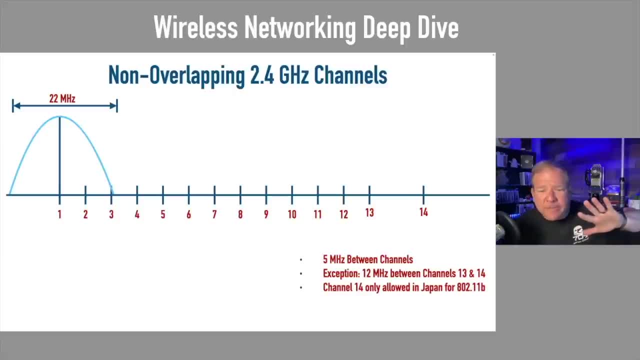 five channels of separation because that that 22 megahertz extends a little bit beyond four channels. Remember, channels are separated with five megahertz. So if we're we have, we have 22 megahertz. that's going to extend a little bit beyond four channels, So we need to 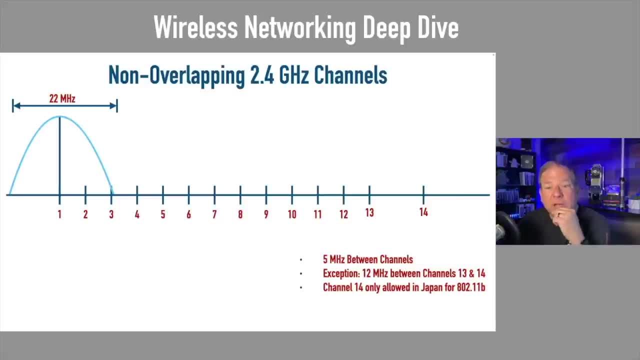 have five channels of separation. So here's the way it's normally done: You go from channel one, add five, and you use channel six, add five, and that's going to give you channel 11.. Now, if you're using .11b and if you're in Japan, yes, you could use channel 14, but 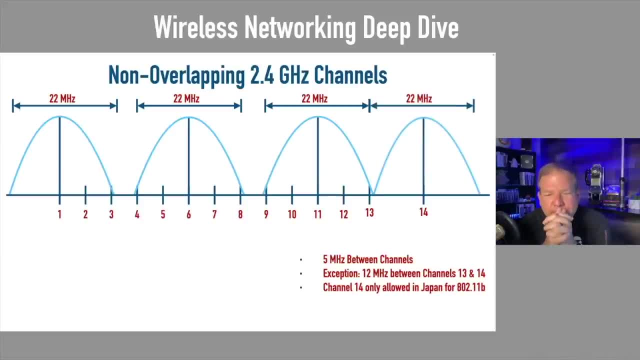 we're probably not going to do that Now. the question is if I'm just going to be using channels one, six and 11, I've got a big network to cover. I need more than three access points. How do I get coverage over this huge area? 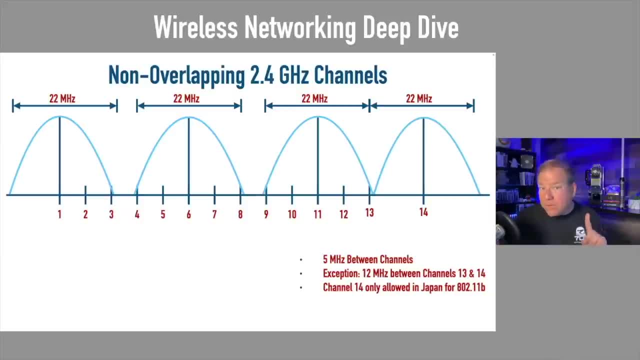 And I've only got three channels that I can use. There's actually a way to do it. What you can do is make sure that you, just when you have an access point, it's got this cell around it, this coverage area. You don't want to be bordered with the same channel. 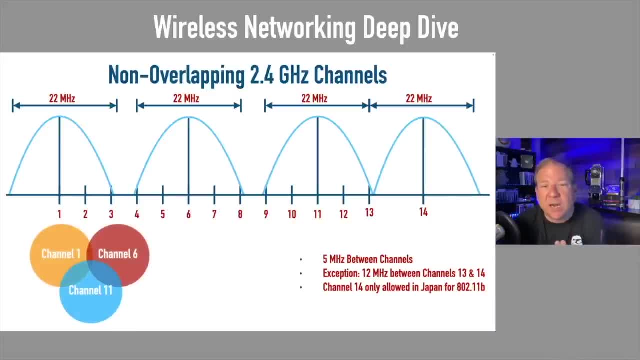 that you're using. So you're going to space out channels one, six and 11, where they'll never be touching another coverage area of their own channel. For your notes, it's called a honeycomb design. Let's start with a honeycomb. Let's start with a honeycomb. Let's start with a honeycomb. 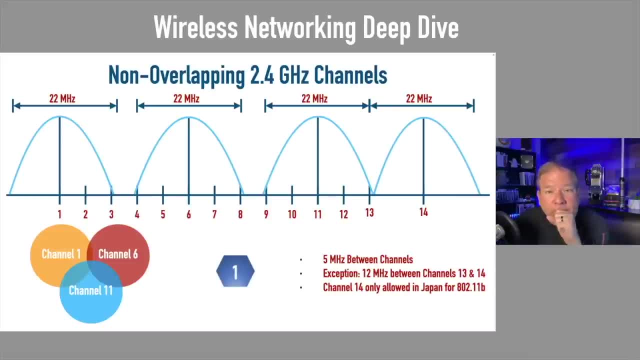 Let's start in the middle with an access point that's using channel one. With channel one, we're going to border that just with channels six and 11.. So I'll put six up top. Now, in that area between one and six, you guessed it, we're going to put an 11 there, So I'm going to put six on top. 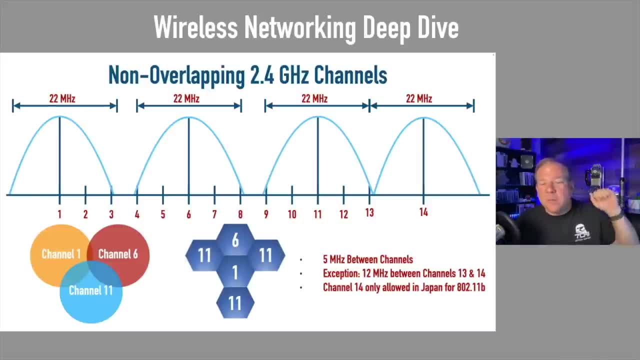 11 below and between one and six. I'll put 11s Between one and 11,. I'll put six and then we can extend it out Between six and 11,. I'll put 11s Between one and 11,. I'll put 11s Between one and. 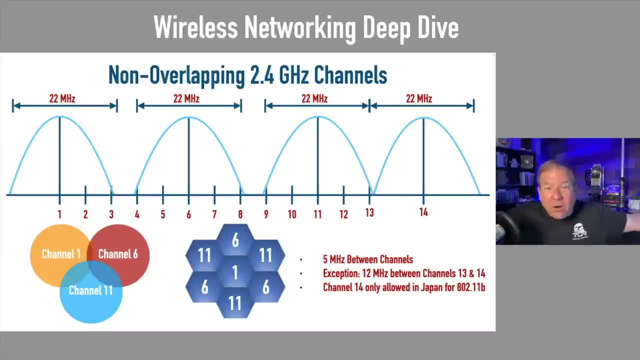 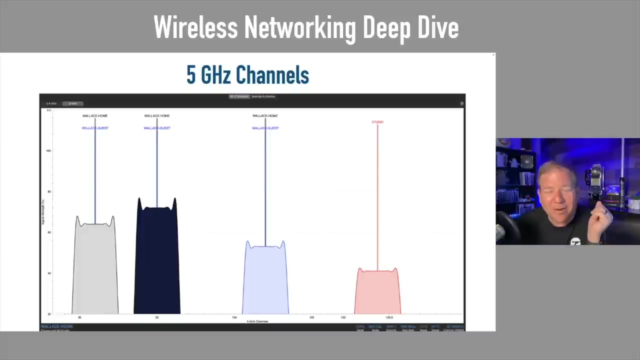 11, I'll put 11s. Between one and 11, I'll put 11s. Christina, The great news is, with five gigahertz we've got a lot more elbow room. We've got a lot more non-overlapping channels that we can use. Now there's been a recent development. 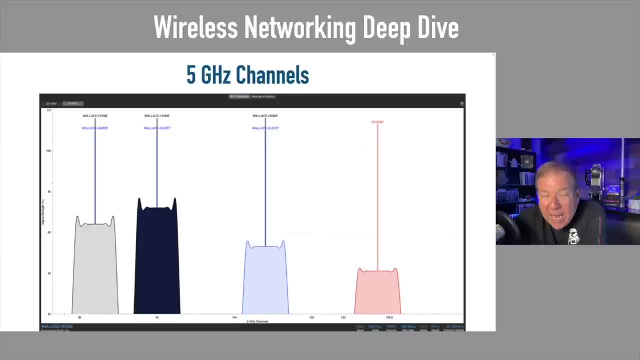 has anybody heard of Wi-Fi 6E? In fact, that's so new you don't even need to know about it for the CCNA or the Encore exam. I'll talk about it a little bit more, but there's actually now the 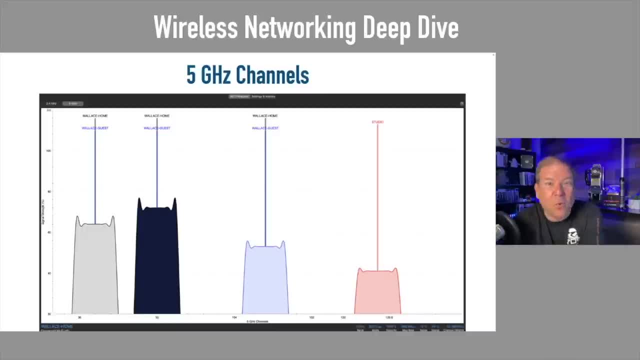 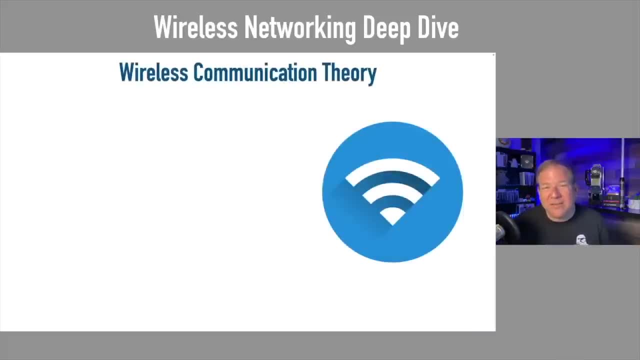 6 gigahertz band. that gives you even more channels, But in general you're not going to have a lot of interference problems with the 5 gigahertz. You're not restricted like you are with the 2.4 gigahertz, And I said that we're going to have this access point and it's going. 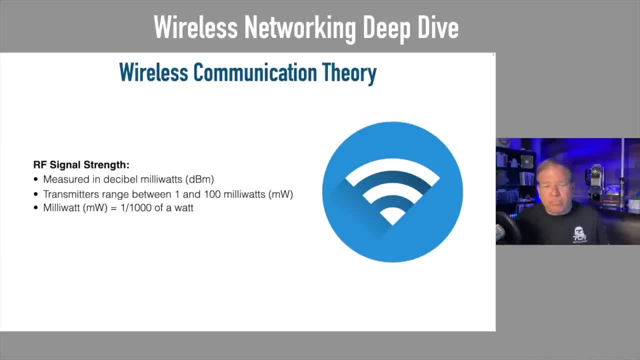 to have a coverage area around it. Let's think about how that coverage or how we measure the signal strength of that coverage area, The signal strength- and you can actually see this on some software and I'll show you an example of that in a few moments. You can see the signal strength. 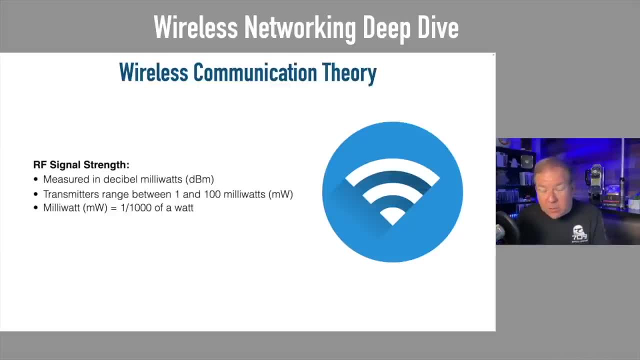 measured in dBm. Now for the Encore exam. that's a term you need to know. That is the measure of signal strength and a dBm is a decibel milliwatt. And if you've ever walked or worked with a logarithmic graph paper in school, where things are, it's not linear, it's the powers of. 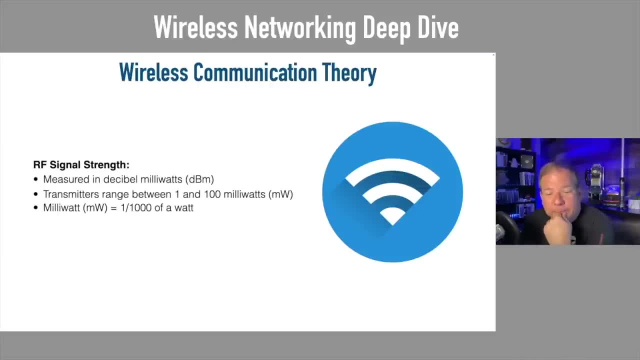 10 going up the y-axis. that's what we're doing here. So when we talk about a milliwatt of power, that's one one-thousandth of a watt, And when we transmit out of one of these antennas, the power. 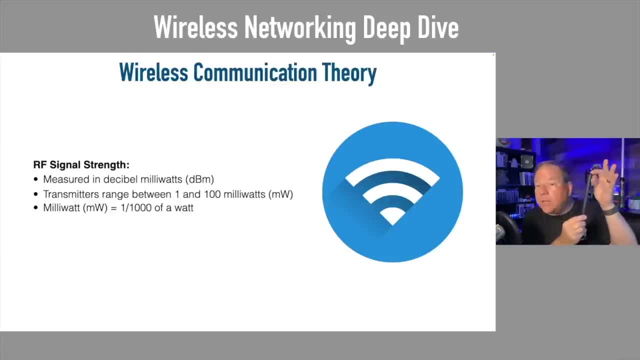 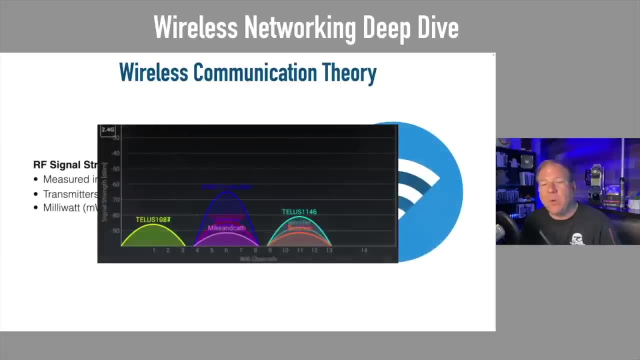 that we're using is probably going to be somewhere between one milliwatt and 100 milliwatts, So maximum we're probably sending out a tenth of a watt And you can have these wireless network analyzers, much like you see on screen, The one I use, by the way, I run on a Mac and the one I use. 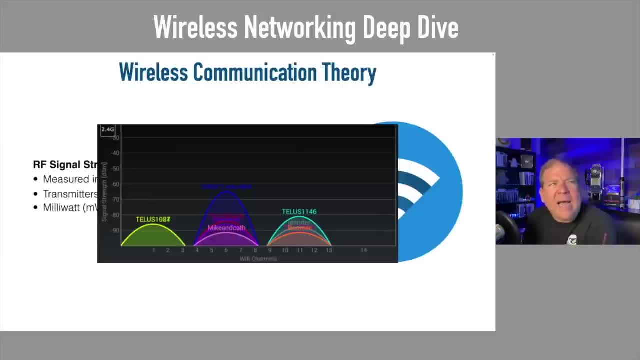 is called iAnalyze. It's called iAnalyze WiFi, So lowercase i, uppercase A iAnalyze WiFi. You can find that in the Mac App Store, So that's the one I use, But it shows you these different networks. 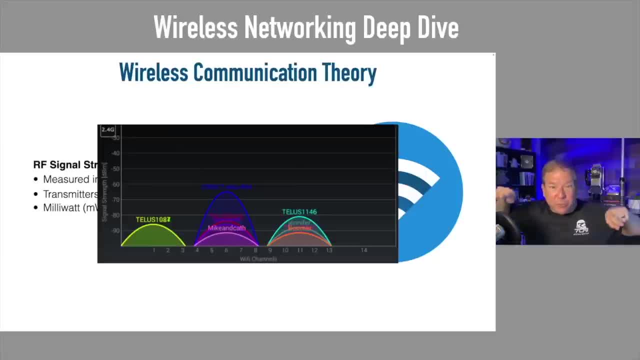 and it shows you what channels are on. Notice that distribution that we talked about, where we're actually expanding a little bit beyond four channels in width. And it shows us if we're on channels 1,, 6, and 11,. we don't have interference, But it also shows us on the y-axis. 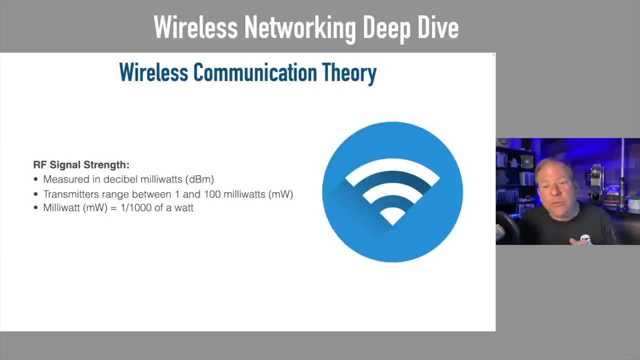 the power. Now, what I need you to be able to do for the real world and for the exam is to be able to understand this relationship between milliwatts of power and dBm, the measurement of power, And here's the way it. 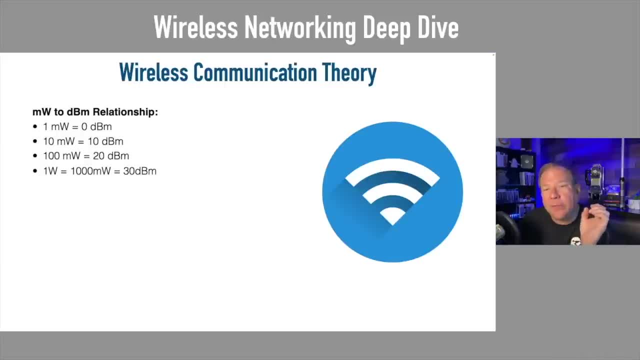 works. If I multiply the wattage by 10, then I'm going to add 10 to my dBm. So follow me: If I take one milliwatt and I multiply it by 10, what happens to my dBm? 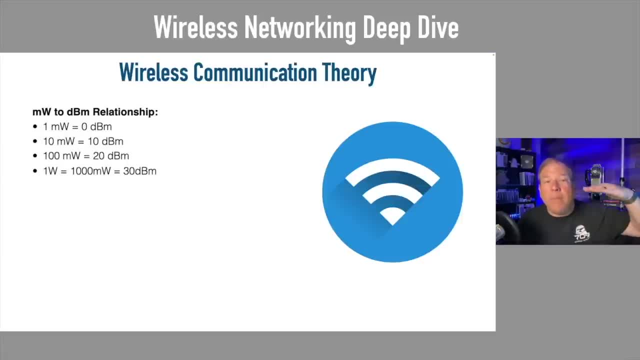 We add 10.. So one milliwatt of power equals zero dBm. If I have 10 milliwatts of power, so I've multiplied my wattage by 10, I just add 10 to my dBm. Let's multiply 10. 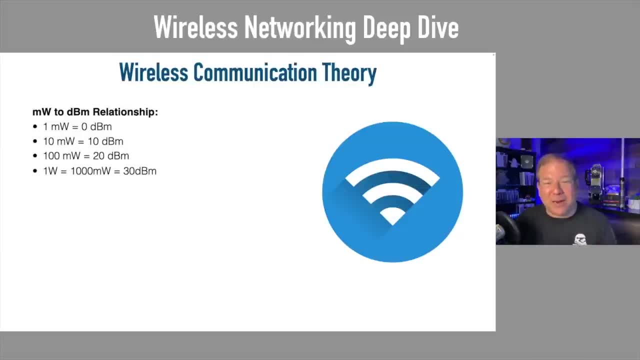 milliwatts of power. Now I have 100 milliwatts of power. What happens to my dBm? Again, I just add 10.. So we're not working with a linear scale, We're working with a large scale, We're working with a 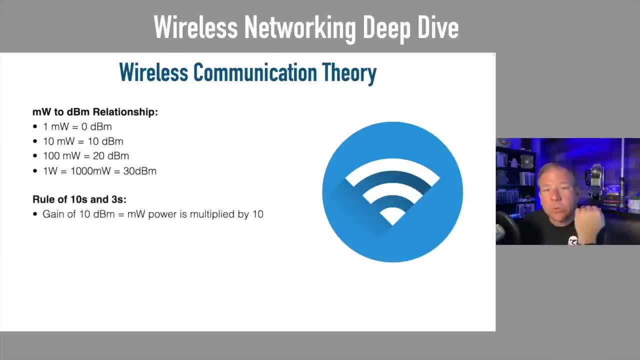 logarithmic scale. Here's an easy way to remember it. It's called the rules, or the rule of tens and threes. If you add 10 dBm, then you just multiplied your wattage by 10. So you add dBm by 10,. 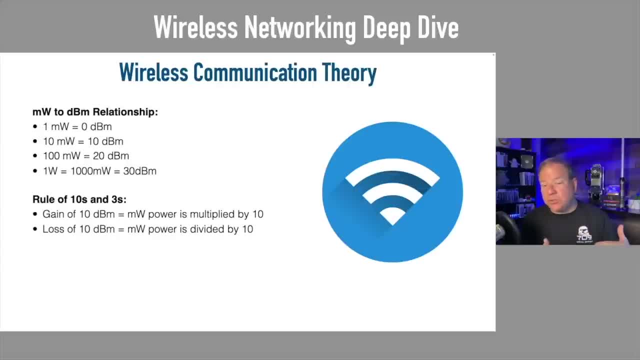 you multiply the wattage by 10, or the reciprocal is true as well: If you lose 10 dBm in signal strength, then you've divided your wattage by 10. Or if you're just concerned about doubling your wattage, if you double your wattage you gain 3 dBm. If you cut your wattage in half, 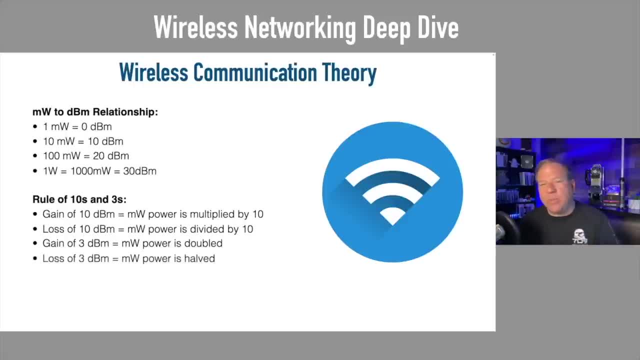 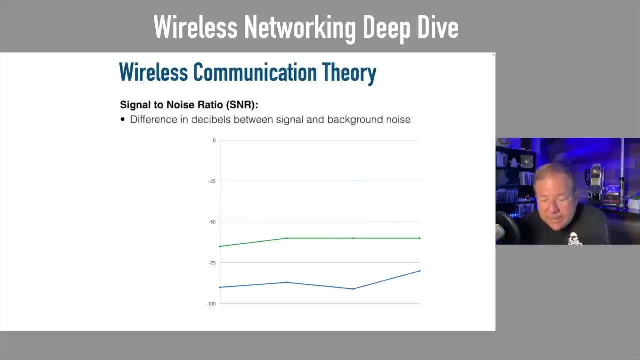 you've lost 3 dBm. So that's just an easy way to remember without having to break out the logarithmic paper. And this is going to show up on that receive signal strength indicator, on that piece of software that I just showed you. Another metric that is key, oh, and I should. 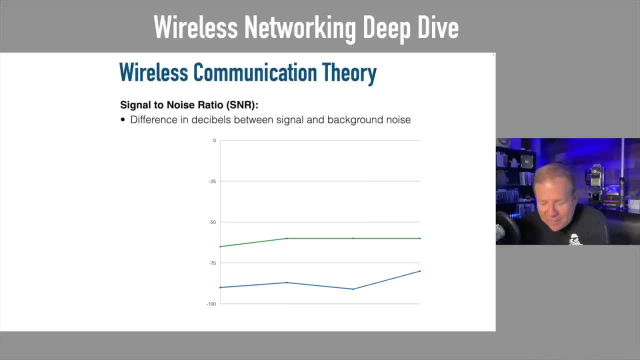 probably mention what's the, What's a good number and what's a bad number. I said that we're going to be measuring these. Well, generally, let's see if I've got my access point here and I've got my phone right next to it. 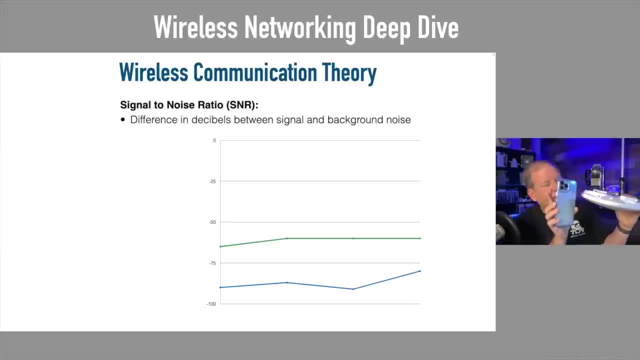 if I'm right next to an access point, typically that's going to be about negative 30 dBm in signal strength. That's typical. So about negative 30 is you're as close as you're going to get. That is a good number, And the further away we get, because we're dealing with negative 30 dBm, the number's 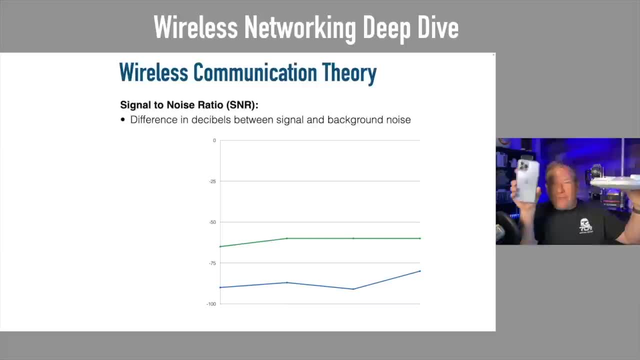 just decreased. So we go negative 30,, negative 30,, negative 40,, negative 50,, negative 60, and so on. If you get down to about negative 90, that's considered to be pretty much unusable at that. 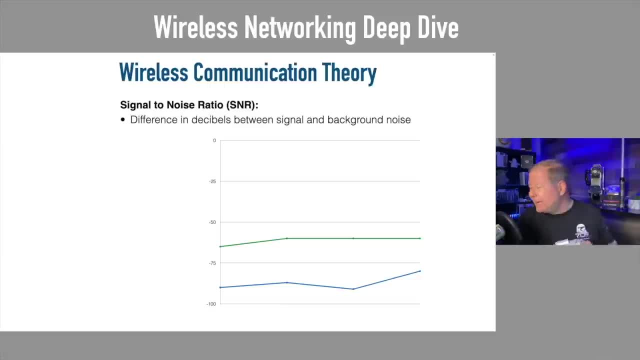 point. So anywhere between negative 30 dBm and negative 90 dBm. as you're looking at that on your software, that's kind of what you're looking for. Another metric you need to know is called the signal-to-noise ratio. Now I think the term 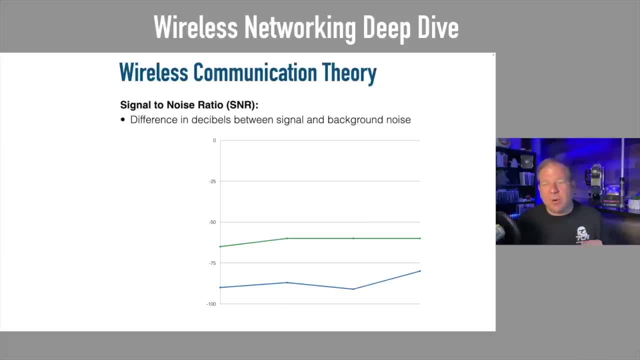 ratio is a little bit tricky here, because a ratio I normally think of it's one number compared to another number. Well, here the ratio is simply the difference in the background radio noise that you have in an environment- Whoops, didn't mean to advance the slide there- The background radio. 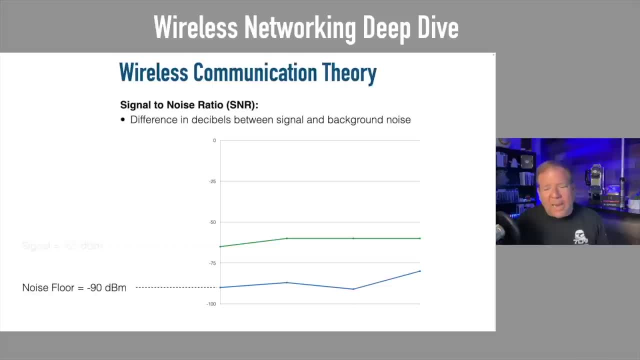 noise you have in an environment and your signal strength. So here I've got a noise floor, Just the background is negative 90 dBm. in this case, My signal strength is negative 65 dBm. So what's my signal-to-noise ratio? I want you to know how to do this. 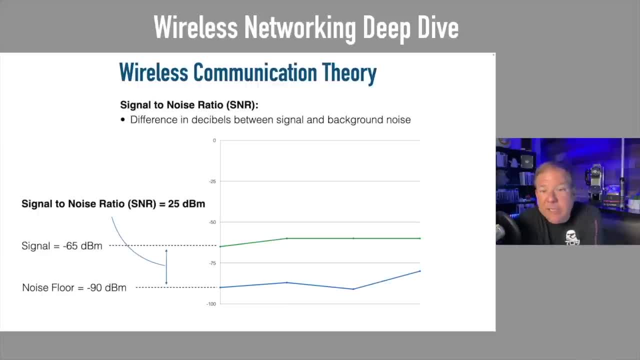 calculation for the Encore exam, by the way, And it's simply the difference. What's the difference between negative 65 and negative 90?? It's 25.. There's a 25 dBm difference. Is that good? Well, generally you'll want greater than a 20 dBm signal-to-noise ratio for just regular data. 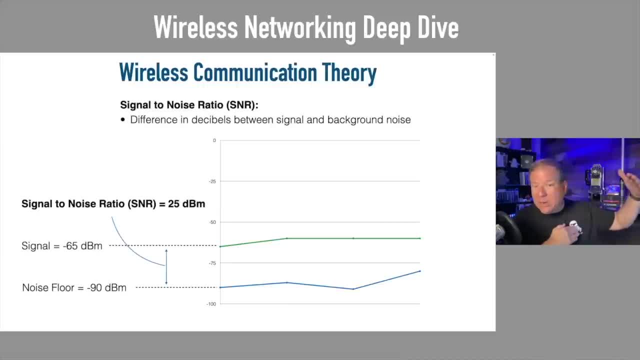 So anything 20 or better, 20 or higher, that's probably going to be good for data. If you're doing voice which is latency sensitive, it's drop sensitive. If you're doing something like voice or maybe video, a little tighter tolerance there for your notes. That's where you want: 25 or higher. 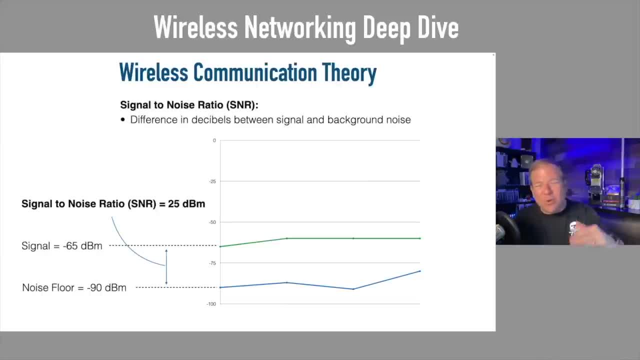 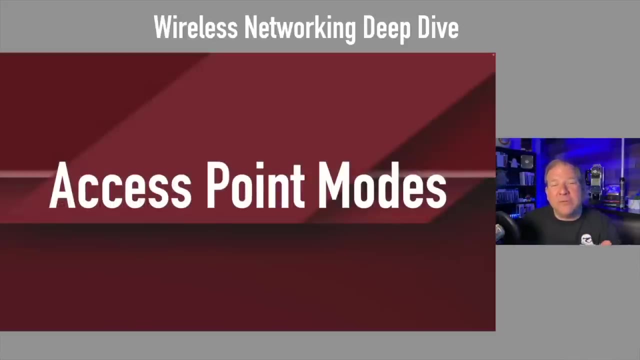 We're minimally meeting a requirement for voice. We've got a difference of 25 dBm. That's okay for voice. It'd be nice if it was 30 difference, but 25, that should be just fine. Next up we want to talk about and, by the way, for those of you joining us live, we are going to 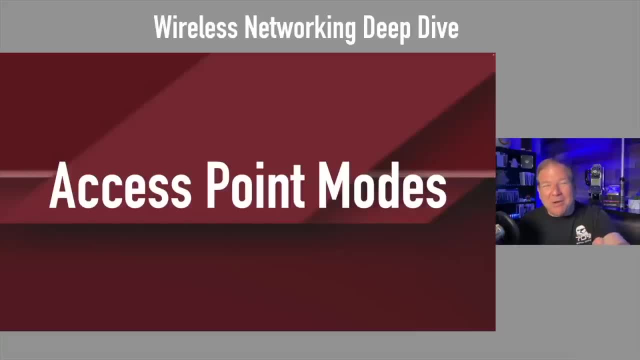 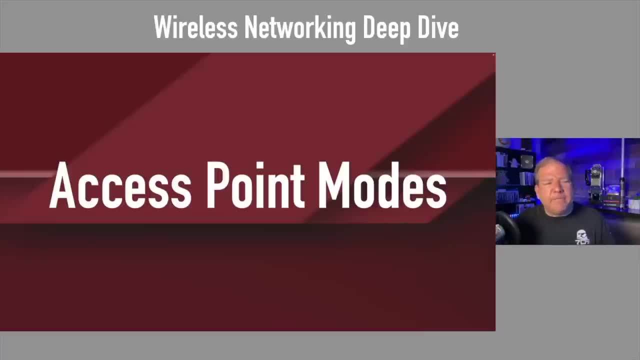 the YouTube replay that we post in a week or so. If you've got questions and you think Kevin's not answering my question, we have. let's see. we have just doing a quick count here. We've got about 700 people joining us right now. It's just not realistic for me to try to take 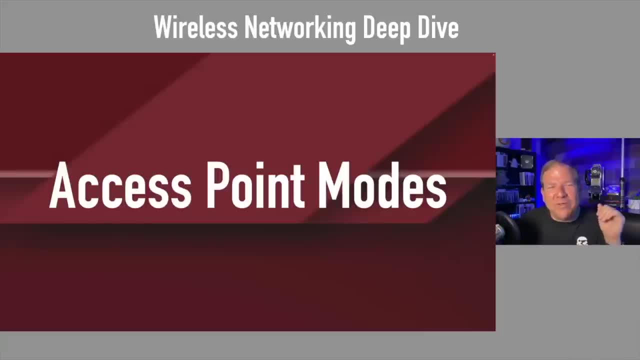 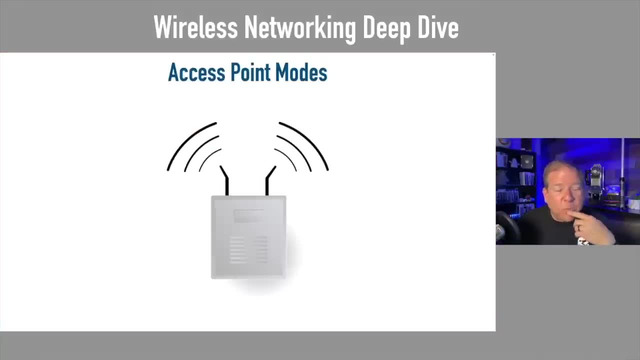 questions as they come in For you joining us live. we've got some dedicated Q&A time. Next up, we'll talk about access point modes. We've already talked. we introduced this at the beginning. We said the one mode that we could operate in is an autonomous access point. This is what you might. 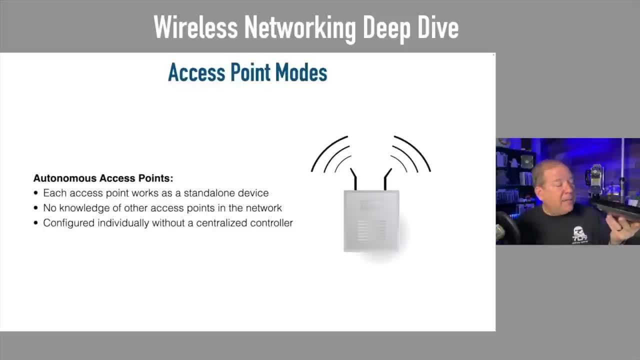 have in a home or a small business, And even though we typically call this a wireless router, you could use this as an access point. Here's what I mean You've got. you've got your port on the back that connects to the internet, and then you've got the ports- ports that connect out. 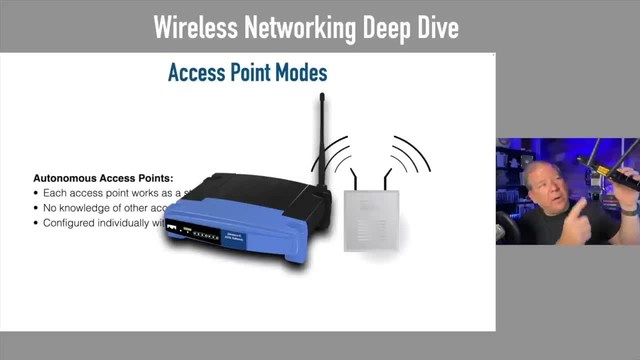 to the rest of your wired network. What you can do is with one you can connect into the internet, into your cable modem, and then you go into your, take one of these ports and go into your switch. Then you take another one of these in a different area of the building. 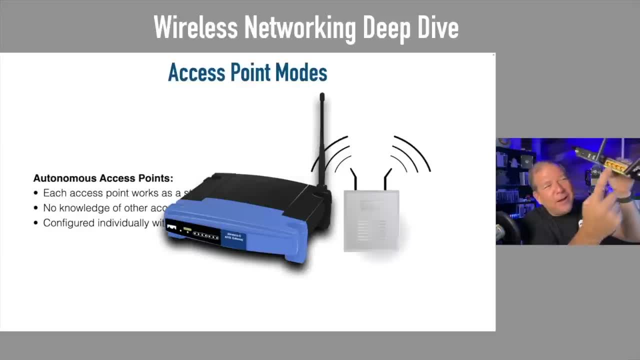 You don't mess with the internet port here. You're not going to use it as a router. You just go from a switch port back to that centralized switch. You put another one in the building somewhere else, giving you nice coverage area. Again, you don't mess with the. 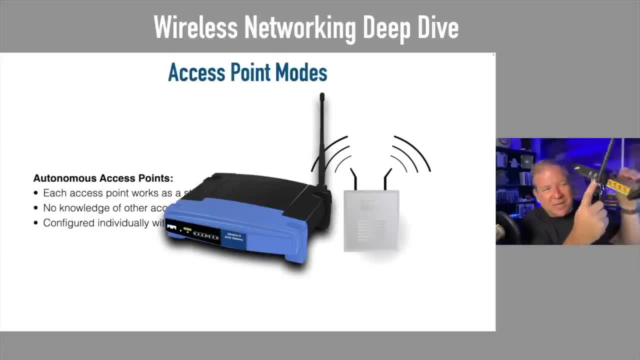 internet port. You're using this just in an access point capacity and you connect this to a switch. If you get all the configuration to match, it's going to be a very good thing, because you're going to be able to run your network. 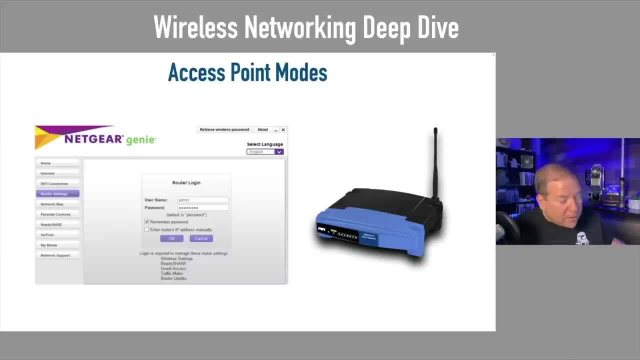 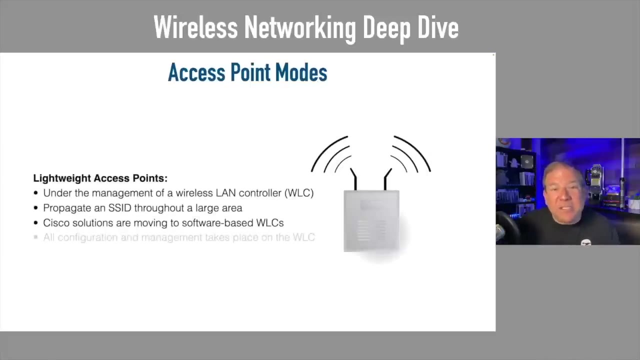 authentically, And by that I mean you set up the same uh, the same SSID, the same wireless, the same wireless network name, the same password. Yeah, You can take your device and you can roam from location to location to location And it's, it's seamless. but that doesn't scale well for the 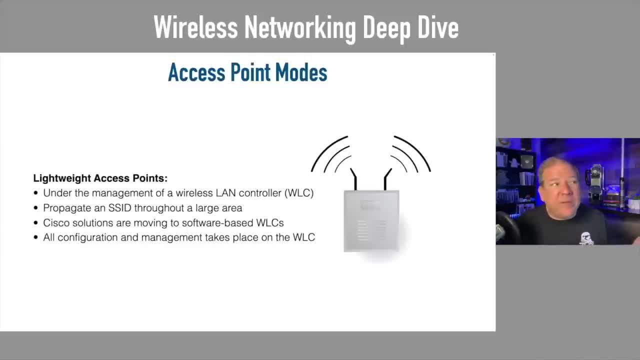 enterprise, For the enterprise we said we're going to start. By the way, the cutoff is about four. I would not want to have more than four. I would not want to have more than four. I would not want to have more than four. 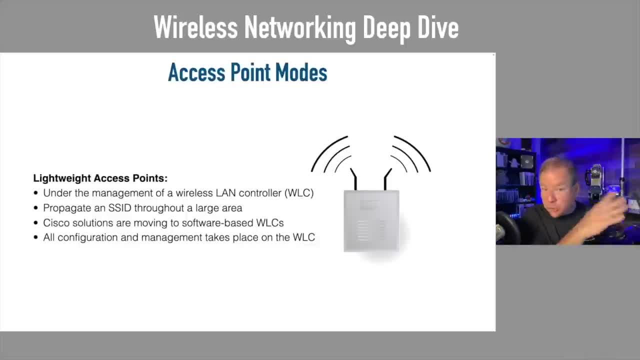 four autonomous access points serving an area. if it got more than that, that's where it starts to make sense to have this lightweight solution. With the lightweight solution, that's where we don't do configuration on the access point itself. We do the configuration on a wireless LAN. 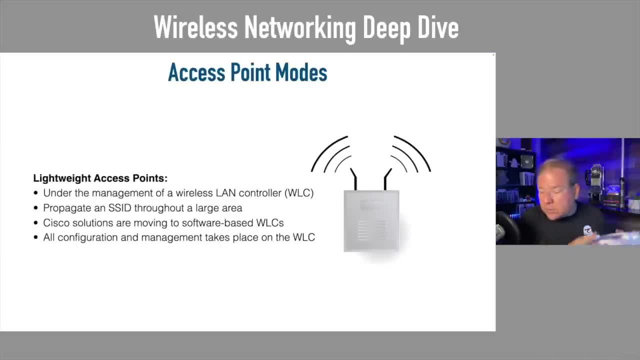 controller and we push that configuration out to all of the access points And we're going to be using that protocol called CAPWAP C-A-P-W-A-P- Control and Provisioning of Wireless Access Points. That's going to be the language of love that we speak between our access. 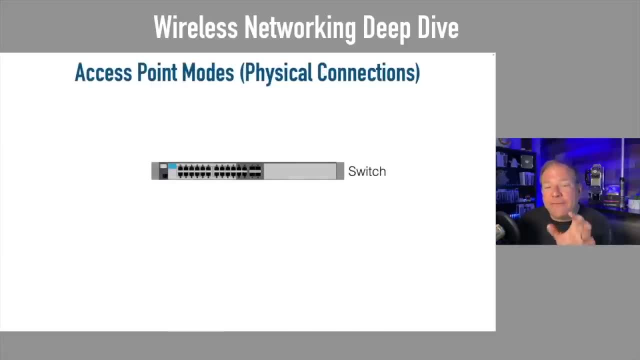 points and our wireless LAN controller. And physically, I want you to notice a potential bottleneck here and what we can do about it. Physically, you've got these access points scattered throughout your enterprise and they're going to connect back to an Ethernet switch. 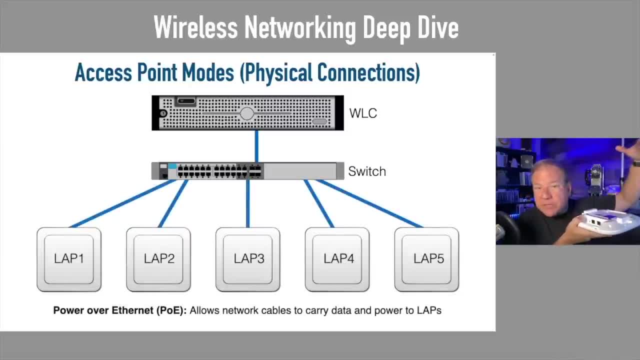 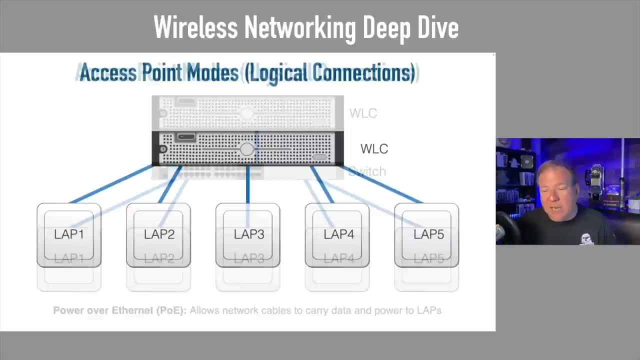 And that Ethernet switch is going to connect out to your WLC, your wireless LAN controller. Now, this is the way it's connected physically. Now let me just- I'm going to advance the slide, then I'm going to come. 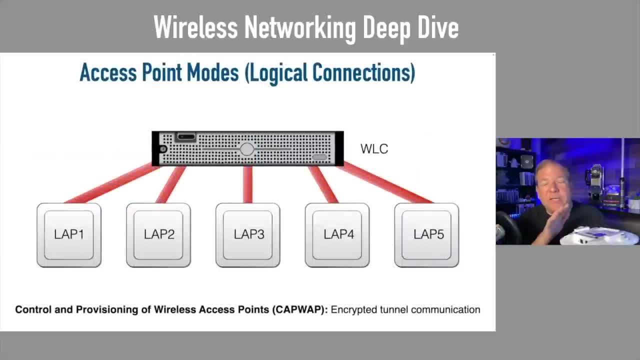 back. Logically, you've got these CAPWAP tunnels. didn't mean to advance that much. Logically, you've got these CAPWAP tunnels going from your access point to your wireless LAN controller because, remember I said, most of the time there are exceptions, but most of the time 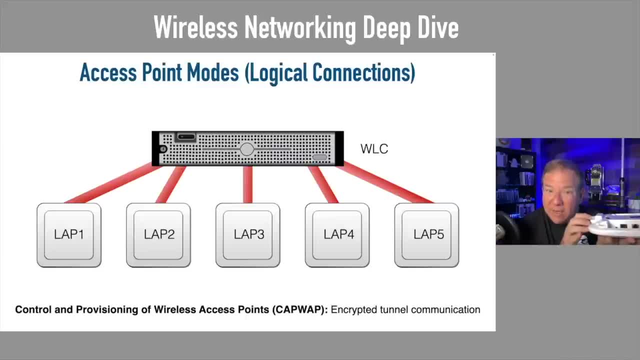 it's not just your control traffic, it's also your data that's going to be going from your access point to your wireless LAN controller, back out to the destination access point. So let's go back to our physical topology for a second. Do you see a problem with this? 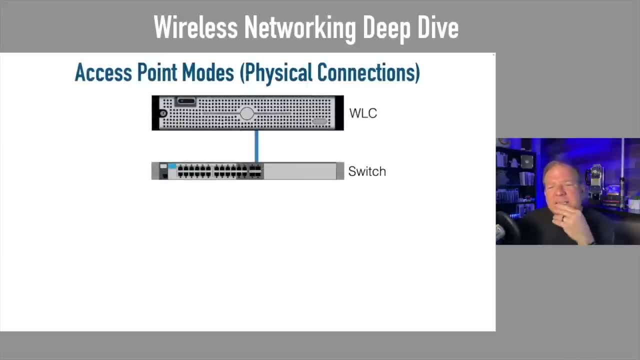 If I'm sending all the data to my wireless LAN controller from all these, maybe I've got dozens, maybe I've got hundreds, maybe I'm like Ken and I've got thousands of access points. Do you see a bottleneck here? What about that connection between the switch and the wireless LAN controller? 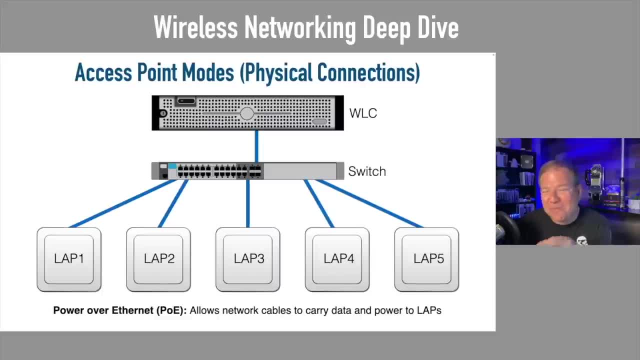 That seems problematic, doesn't it? I think so. So what you'll normally be able to do with your Cisco wireless LAN controllers? depending on which model you buy, you'll be able to have multiple connections. Somebody tell me in the chats what do we call it? 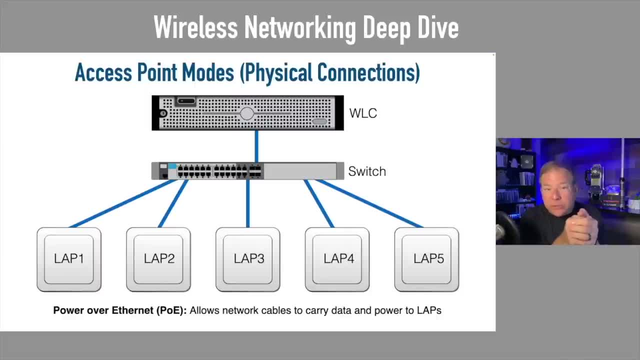 when I have multiple physical connections between two switches and I logically bundle them together So it looks like one logical connection, even though it's multiple physical connections. What do we call that? Go ahead and chat that in. Yeah, we might call it an ether channel. 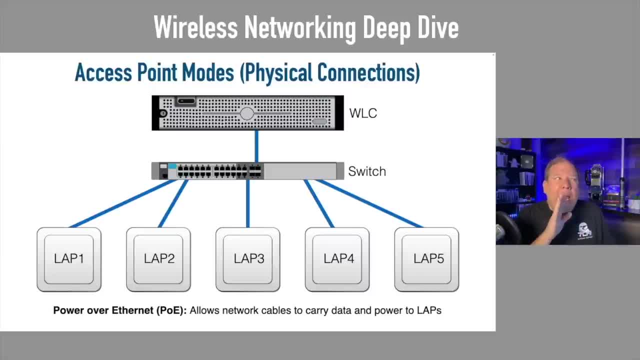 An ether channel And when you learn about ether channels, which is something if you- I don't know if you've taken your the CCNA training that we do or not- we've actually got a CCNA course coming up week after next. I'll tell you more about that later. 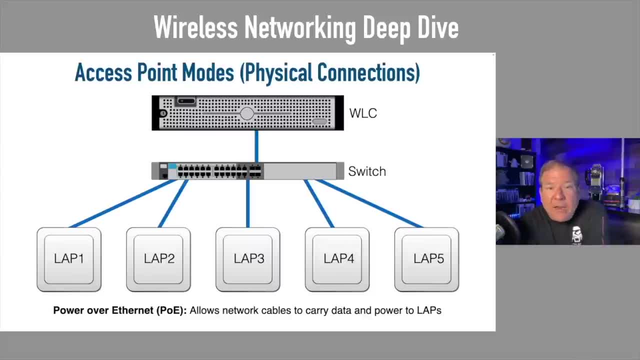 But we talk about ether channels and there are protocols that you can use to set up an ether channel connection between switches And in this case you're not going to be using any of those protocols. In the CCNA course we talk about protocols called PAGP- Port Aggregation. 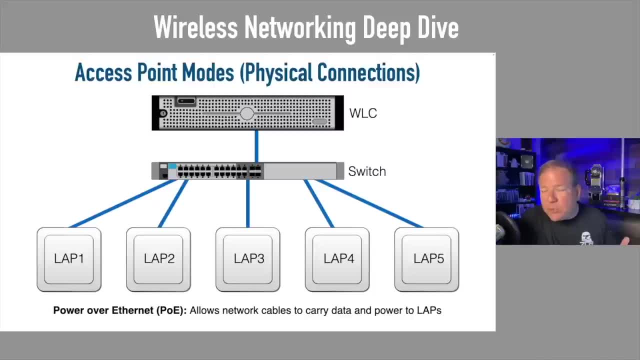 Protocol. We talk about LACP, the Link Aggregation Control Protocol. Our wireless access points don't speak those languages. Our wireless access points simply have basically a switch, Turn it on or turn it off. You can turn on Link Aggregation. It's not going to run any of 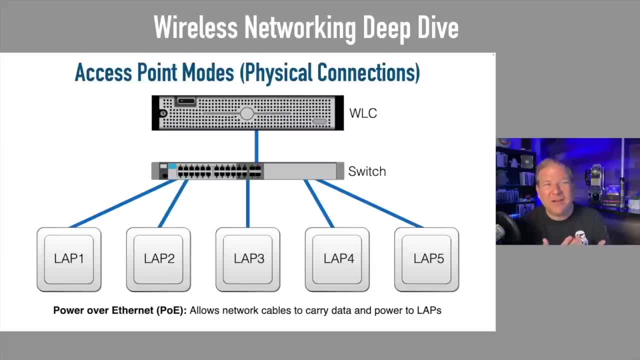 those fancy protocols that negotiate an ether channel. You just say, yeah, I want to create. it's called LAG, Link Aggregation. No protocols, just turn it on. I'm going to have multiple connections going from my wireless and controller down to my switch And again, sometimes you might. 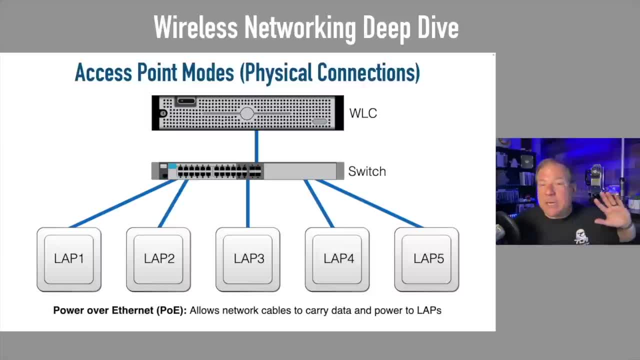 see only two ports on your wireless and controller. Sometimes you might see four, You might see eight. It depends on what model of wireless and controller you buy. but you could have eight gig ports in one logical connection going down to your switch, because that is. 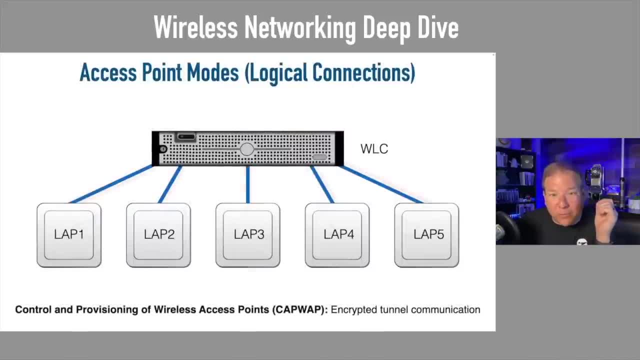 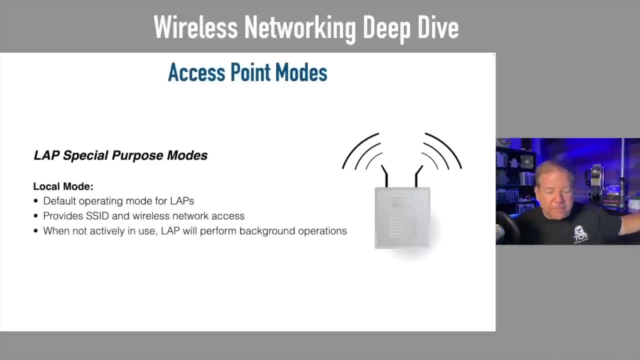 definitely a potential bottleneck and we want to avoid that. Again, that doesn't happen all the time. Remember we talked about FlexConnect earlier. I also want you to know that, in a large enterprise environment, this is not something what I'm about to describe. it's not something. 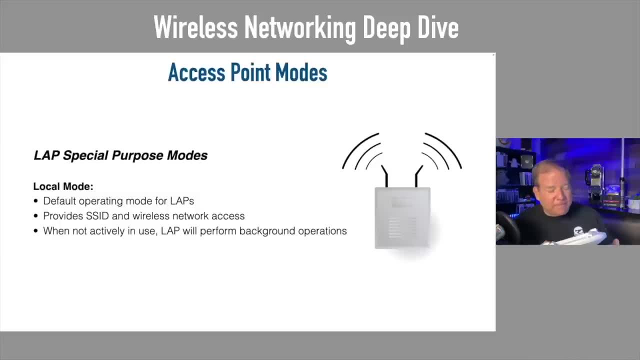 home or small business probably, But in an enterprise you could have, you probably do have hundreds, or Ken has thousands- of these access points. You could run them in different modes. The default mode that I normally think of is just called local mode. It's being a basic. 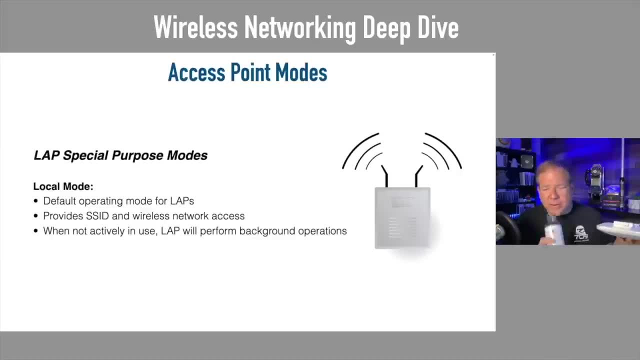 access point And what it's doing. it's handling user data, It's advertising the local, it's advertising your wireless network. Now, when it's not busy doing those types of things, it can do some background operations, One of the cool things that the Cisco wireless solution does. 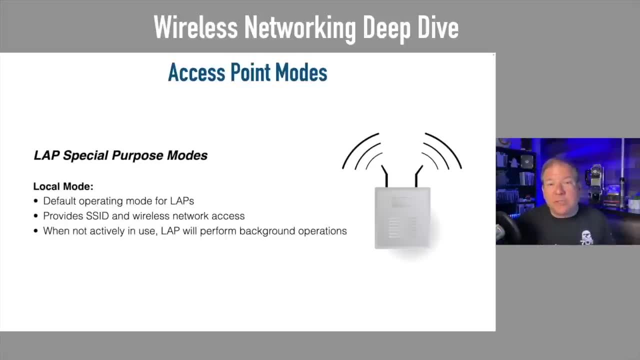 is it will look for for security purposes. it will look for rogue access points. It'll try to make sure somebody hasn't brought in their own access point and they're trying to do something mischievous. But it'll do that if it's got time to do it. But that's just called local mode. That's what I normally. 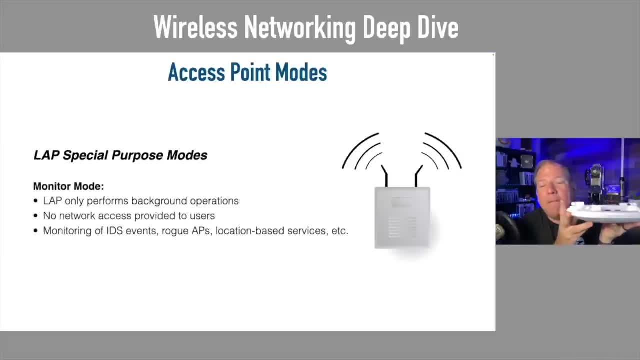 think of, But you could have one dedicated to be a monitor. Now, if it's in monitor mode, it's not going to be handling user data, It's going to be doing those background tasks. It's going to be searching, scouring for rogue APs that somebody put in It might be used to do. 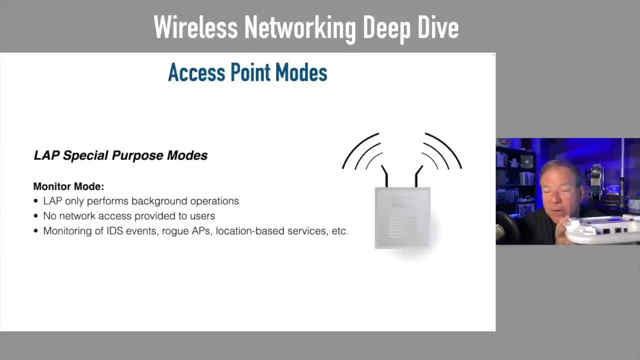 triangulation. It might be used to do, you know, like you know, like you know, like you know, the location for the location-based tracking we talked about earlier. It might be monitoring, It might be working with a wireless IDS or IPS intrusion prevention system sensor to to to. 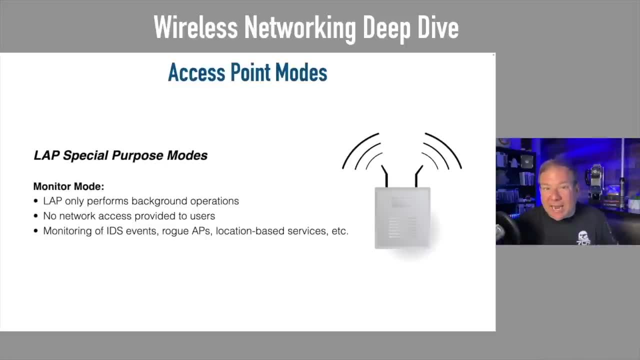 send copies to that IPS sensor to scan for malicious traffic coming in, So we could be dedicated to just monitor what's going on, not really handling the traffic. Now the next one- we've already talked about this- is where I've got that remote office over a WAN connection. 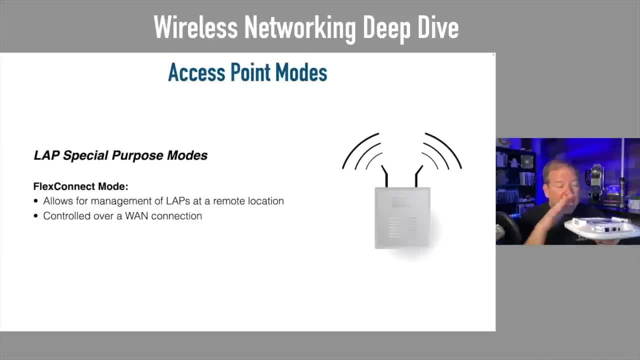 and I'm using a remote office over a WAN connection And I'm using a remote office over a flex connect. That's where I still hear me on this. I still send control traffic over that CAPWAP connection back up to the headquarters over the WAN connection. But if I'm going from 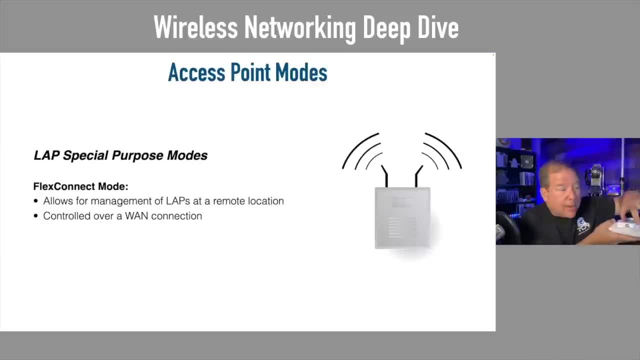 one access point to another access point at this remote site. there's no need to send the data all the way back to the headquarters and then all the way back. No, I could run in flex connect local switched mode and just go from one access point to the other access point within my remote. 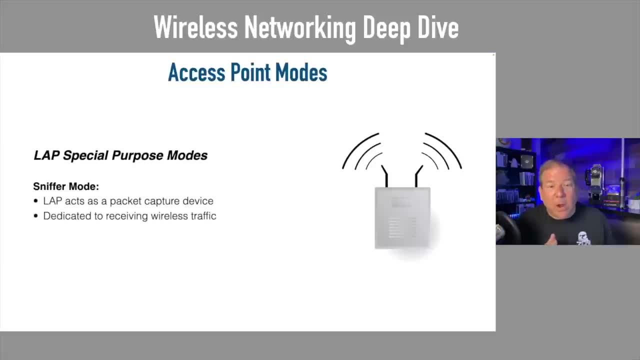 location. So we might be set up to run in that mode. We could run in sniffer mode. This is used to analyze traffic, maybe for troubleshooting purposes, maybe for security purposes. but we could have one of these dedicated to just capture and then maybe send that traffic. 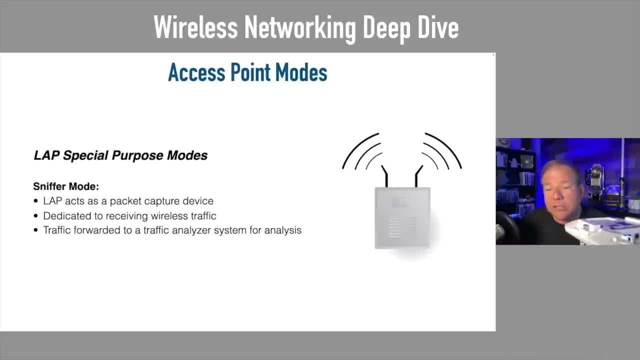 to something like a Wireshark to do a traffic analysis with. We could have one. I said that we might have a couple of these modes. might be looking for rogue access points in the background. If you really think that's a big concern, you could have an access point And that is its. 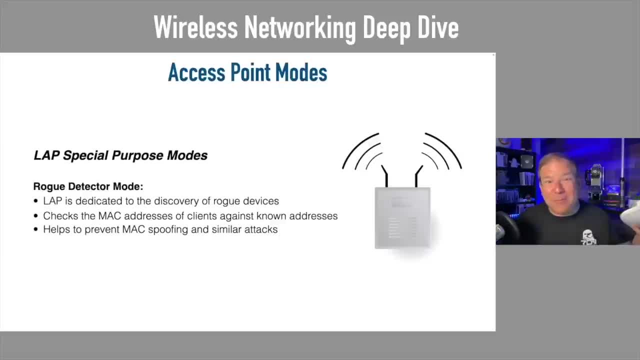 purpose in life. It is looking for those rogue access points And that's pretty much all it's doing, And you're going to be able to much more efficiently catch any rogue access points that somebody adds Now in bridge mode. this is where you might have a couple of mesh networks. We 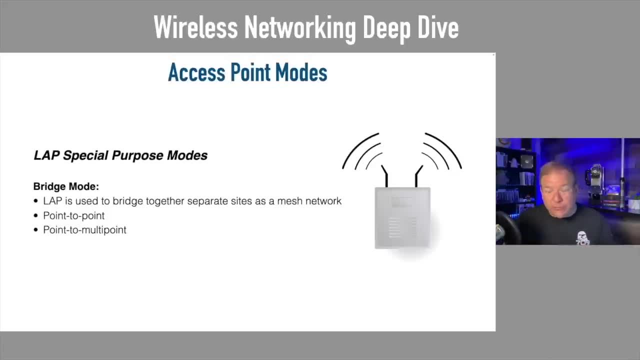 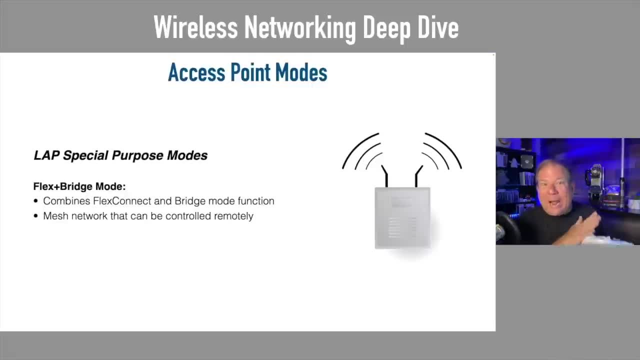 them. you can have one that is acting in flex connect mode and in bridge mode, maybe for a remote site, And finally there's one called S E connect mode. Cisco has this piece of software called spectrum expert And it's going to do an analysis of the radio frequency spectrum. 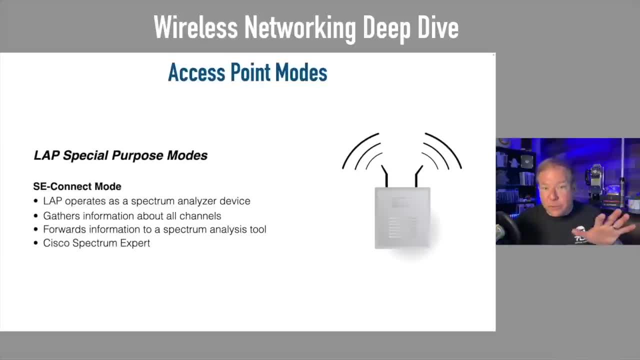 it's going to see which frequencies are busy, which are best used for maybe a specific channel. if you let it auto select the channel and it's going to, you could have a an access point, And that's its purpose. It's scanning the radio frequency spectrum And 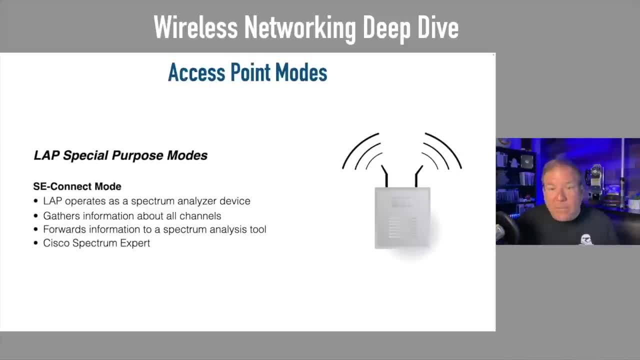 it's noticing what's happening Now in in my home. just to give an example, I'm doing lightweight access points in my home and I have seven of them. We built a home about three years ago and we've got. we've got two, two stories. 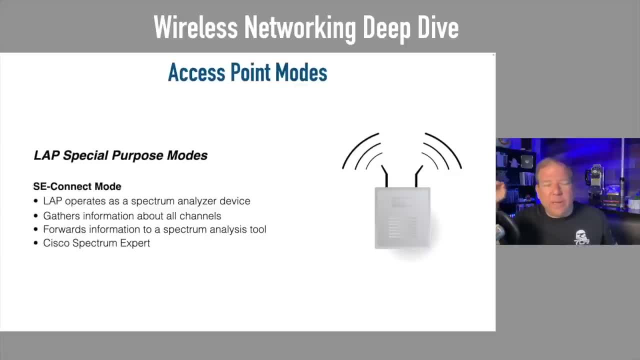 and we've got an area out in the back, a pool area, where we want to have wireless coverage as well. So I've got seven different access points And sometimes I'll get an alert because we live nearby and an army base where they store chemical weapons And, yeah, that makes me a little bit. 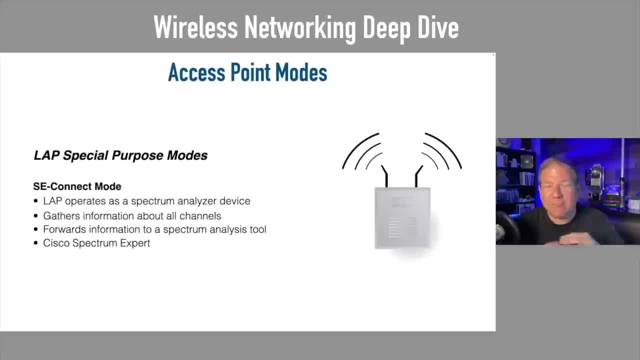 nervous sometimes, But I get. I get these alerts that radar has been detected on certain channels of my wireless access points And when that happens, okay, what's? it can automatically select a different channel to use it, but it will notice the radar. That's the kind of thing that Cisco's 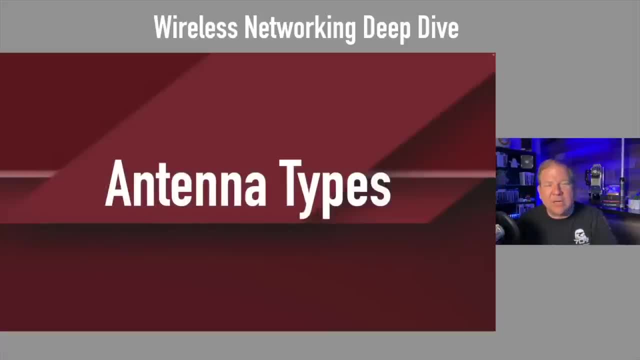 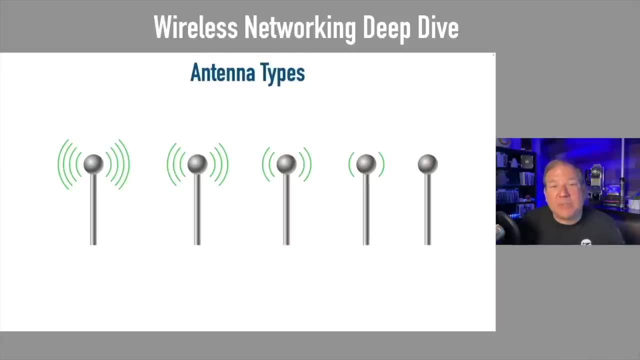 spectrum expert would use. Now, before we take our first Q&A break, let's talk antenna types And then we'll. we'll take that first break that I was telling you about, And we got into antenna types a little bit earlier. I gave you the example of a of a dipole antenna. We talked a little bit about how. 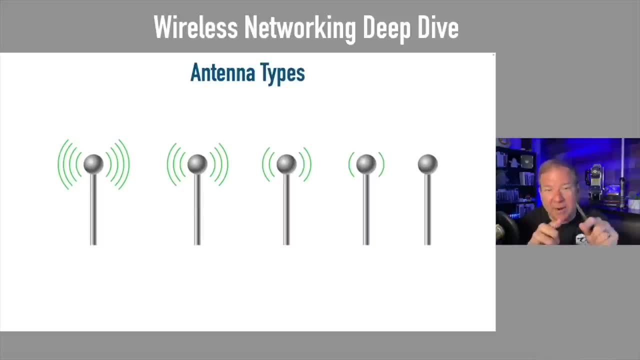 that worked. Remember how we applied charges on two wires, kind of bent the wires down, So across one plane, which is like up and down, here we're be able to radiate out. Well, we have some antennas like this that go out in all. 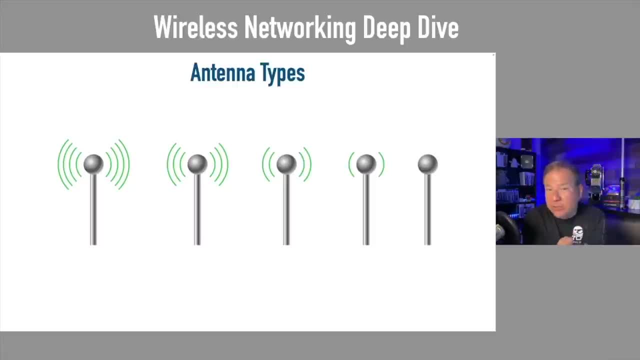 directions. some antennas- we might want them to be focused- And for the encore exam specifically, you need to be able to look at what are called plot graphs, graphs that show you coverage areas of antennas. I want you to be able to look at a plot graph and say, Oh, that's a dipole antenna or that's. 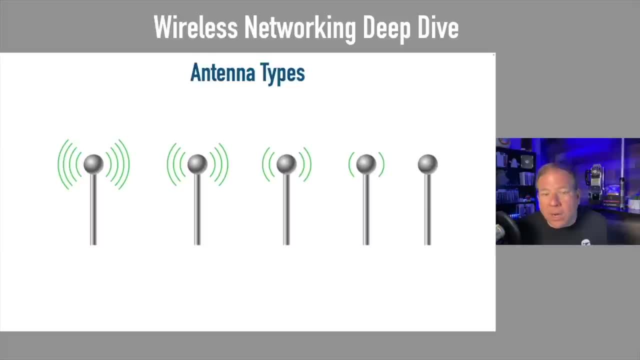 a patch antenna or that's a Yagi or antenna, And I'm going to give you examples of that. So when we're looking at the radio frequency coverage area of an antenna, it's not enough just to have your traditional x- y axis. we need to go, we need to go three dimensional here. So we need an x and a y. 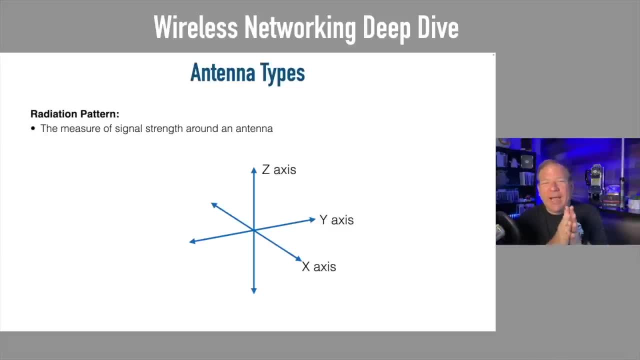 and a z axis. So we're going into the third dimension And we're trying to represent this on a flat screen. So we're trying to visualize something that's 3D on a flat screen. So here's the way we do it. 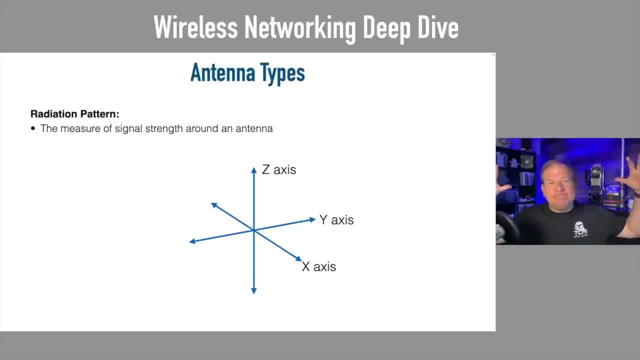 Imagine that we had this big think of a big beach ball Like this and we're going to cut it in half. Okay, pretend it doesn't pop. when we cut it in half, We get this big beach ball. we're going to slice it. 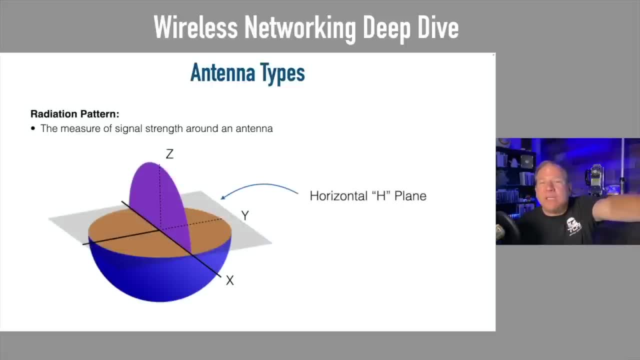 When we slice that big beach ball horizontally it might look something like this: That beach ball represents the coverage area of an access point. So we've got our access point right in the very center of that beach ball And we're saying: let's look at the radio frequency strength this far out on the surface of the beach ball. 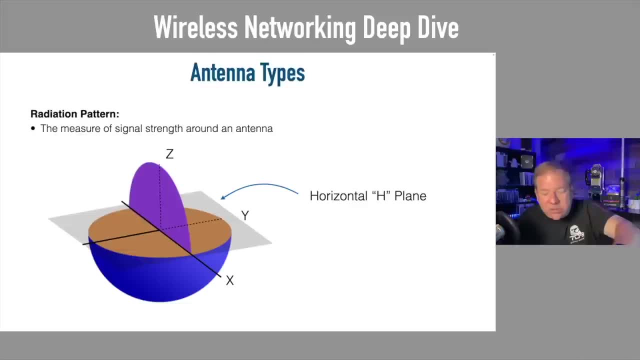 And if we cut that in half horizontally, in other words, and we're looking down on the top of that access point, we want to be able to graph what the coverage area is. Now to make this 3D, we want to take that beach ball again. 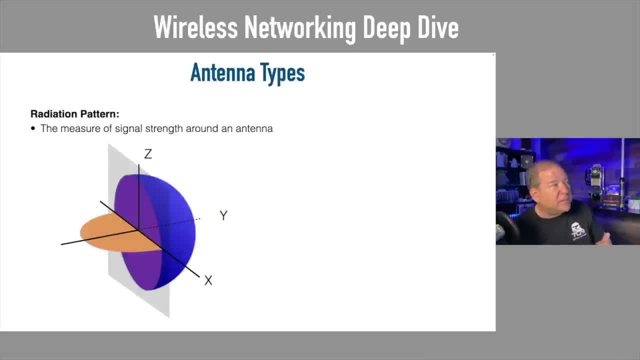 And this time we're going to, We're going to cut it vertically and we're going to say: okay, looking at this vertically, what does the coverage area, what does the radio coverage area look like? And this is called the elevation plane. 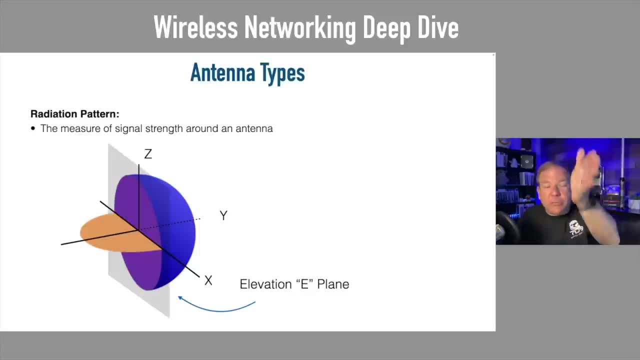 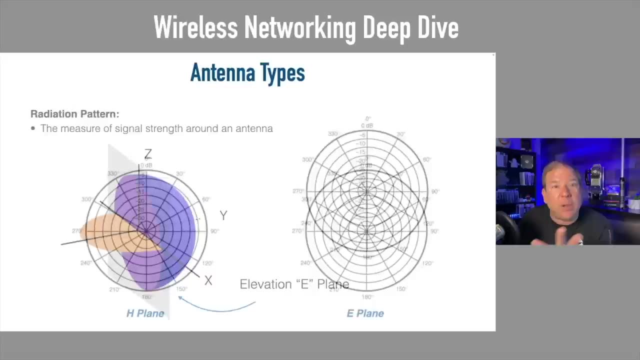 So we've got the horizontal plane flat and the elevation plane top to bottom. Now let me give you some examples. We're going to use this 360 degree plot graph to visualize this, And the first one we'll consider is: and for your notes, 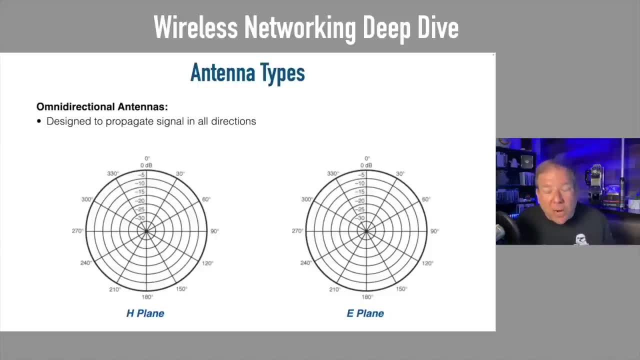 it's an omnidirectional antenna. Omnidirectional implies that we would like- it's not always perfect, but we would like- to have coverage area or coverage approximately equal in all directions. So it's not just going straight, It's not just going up and down. 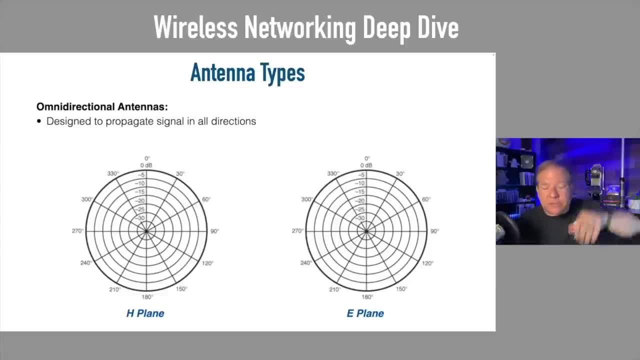 It's like that beach ball: We want it to go out equally in about all directions. Now, this dipole antenna that we talked about earlier, that is considered to be an omnidirectional. It's considered to be an omnidirectional antenna. 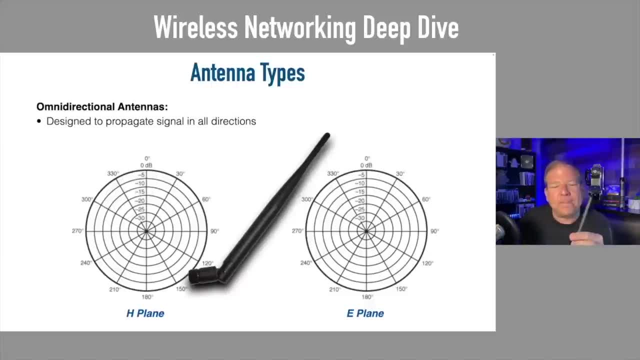 That's what I'm showing you here on the screen Now. I kind of described how this worked before I said we had these two connectors or two conductors. It kind of goes in the middle: One wire goes this way, One wire goes this way. 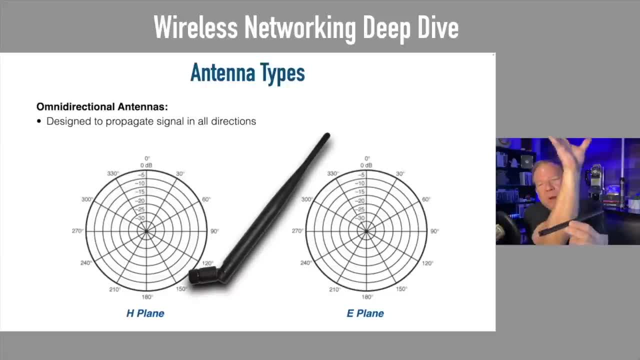 So we've got the same charge going across this way and it's going to radiate out these signals And it's going to do that all the way around this antenna. Well, it's kind of going the same in all directions, but it's not perfect. 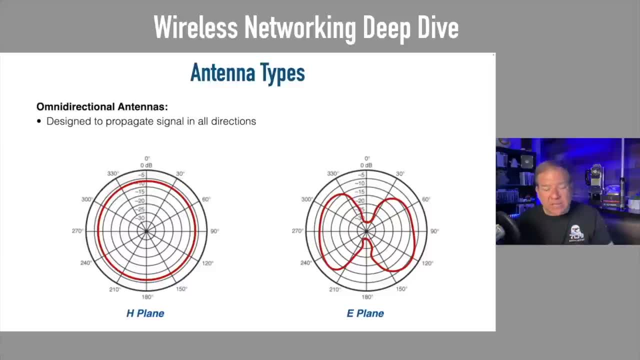 Now, if I looked at the H-plane- in other words, I'm looking down. let me hold it like this: You're looking down on the antenna and you're looking at the coverage area That's the H-plane graph. Notice it's a perfect circle. 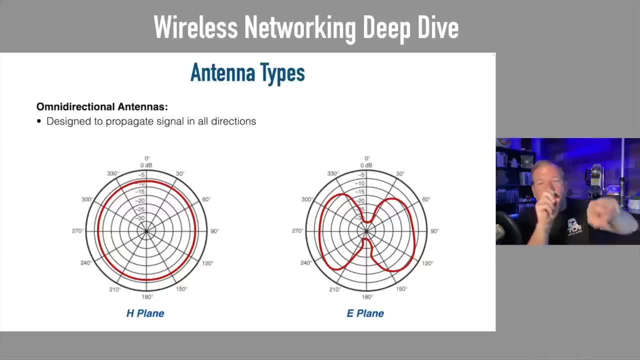 because we're radiating out the same signal strength all the way around. this. It's going out this way: Now, if I hold it vertically like this, that's the E-plane. Now, it's not perfect If you're looking at it like this. 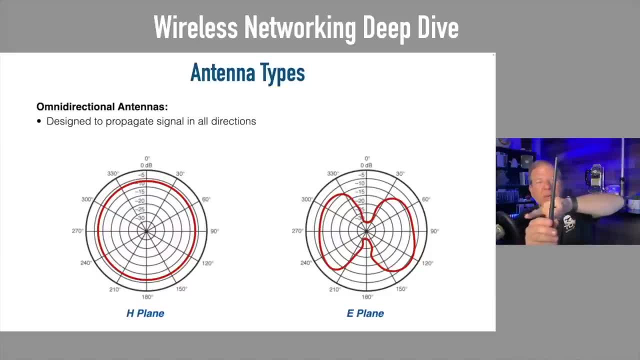 yeah, we do radiate. We do radiate out pretty much equal directions on all sides. But notice, at the top and the bottom we're not really radiating out much, if anything, there. So we've got a couple of null points at the top and the bottom. 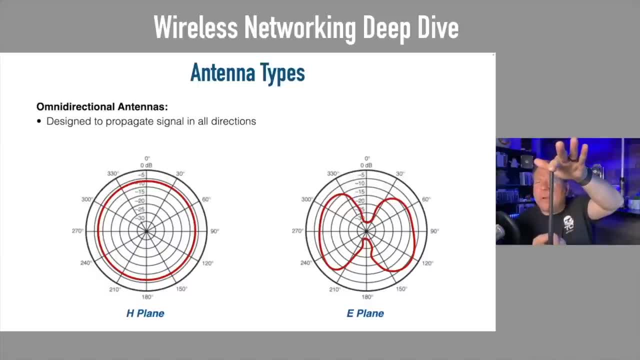 So it's not perfect, But in general we still call this omnidirectional because it's going in all directions and it's just kind of failing a little bit, going straight up and straight down. It's almost like a donut-shaped coverage. 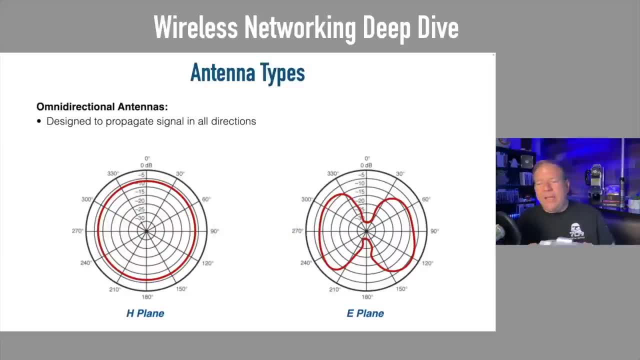 if you think of it like that. Now, here we have an access point that has multiple internal antennas And, by the way, you can have antennas that are perfectly flat. Not everything works like the dipole. I wanted to give you one thing as an example. 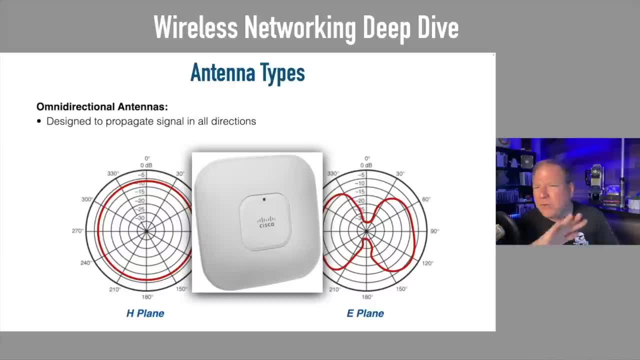 to help you visualize how it works. It all deals with moving charges around, but some of them can be flat and curved and they're not all dipole. So here I've got a series of antennas, and this does give me very much of a 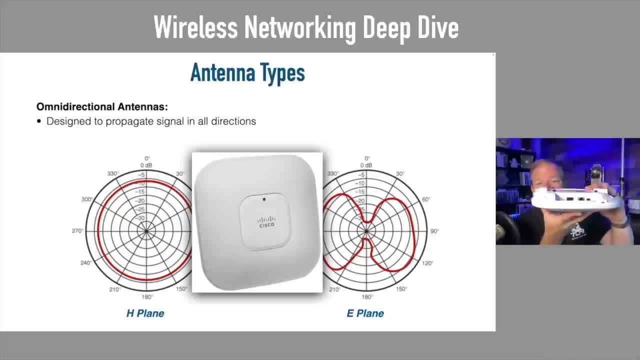 spherical coverage area. So you mount this, it's going to give you almost approximately same signal strength going up and down and left and right and all the way around, So we would also consider this to be an omnidirectional antenna. Now some antennas. 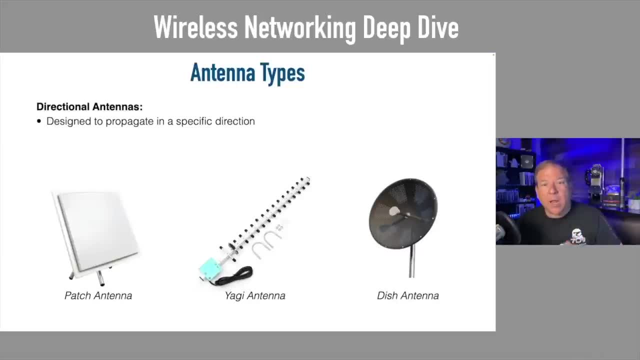 we want to go in a fairly specific direction, because it's a trade-off, isn't it? I mean, I've got a finite amount of power that I can use to radiate out my signals, and I could choose to divide it up equally. 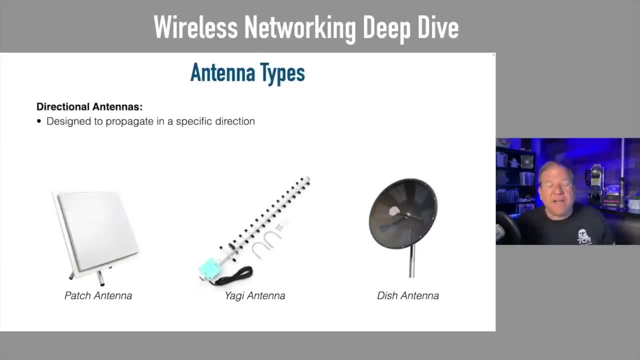 and try to send equal power in all directions. But if I needed to get from this building to that building over there, I don't want to go in the other direction. I want to focus my energy going to that other building. So that's what a directional antenna can do for us. 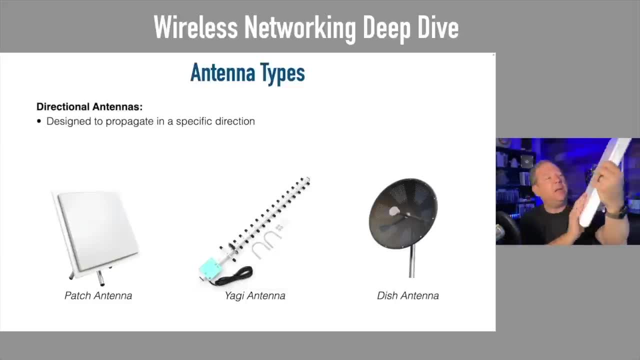 Now, one type is called a patch antenna, And here's an example. here's an example of a patch antenna. This is the kind that I mentioned that we had a pool area behind my home. This is what I mounted as an outdoor patch antenna. 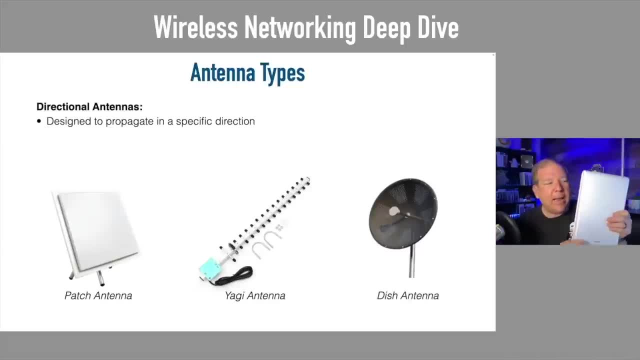 because I want to cover the whole pool deck And I don't really need any coming back into the house. It's mounted on the side of a brick wall. I'm not trying to come back. I'm not trying to come back this way. 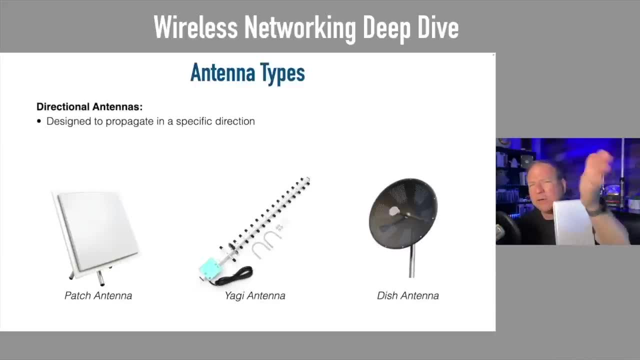 I want it all to go kind of not a straight line, not like a laser focus line, but just kind of in general, kind of that way. And that's what a patch antenna does. It goes generally most power in one direction. 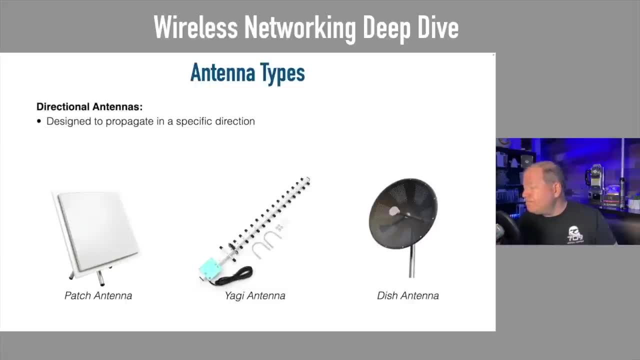 Now a Yagi antenna. that's much more directional. So if you're trying to go between a couple of nearby buildings, perhaps- yeah- you might want to use a Yagi antenna. That's very directional. or down a long hallway, That might be a good use for a Yagi antenna. 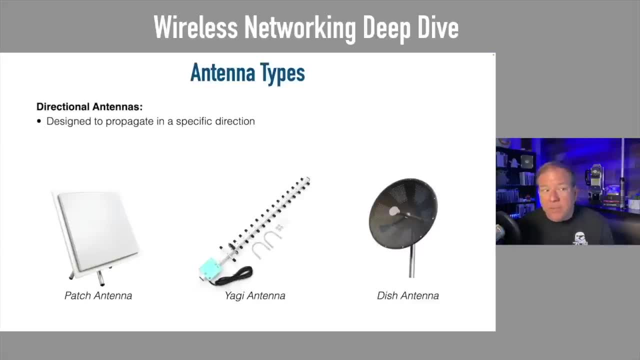 A dish antenna or parabolic antenna that's going to give you a further distance than you typically get with a Yagi, Because if you remember from a math class and your conic sections, you've got a parabola and you've got this foci. 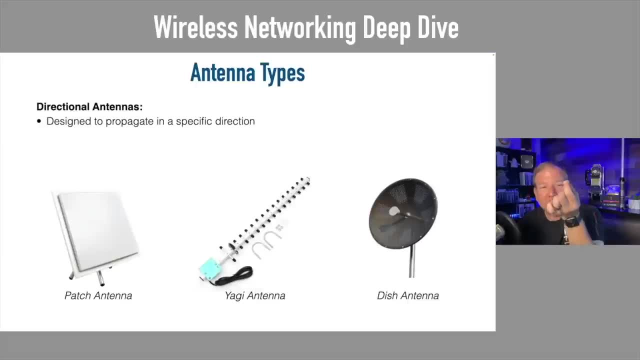 Well, the, the pickup, if you will, is located at the foci of this parabola And it's going to be able to focus your energy coming in and coming out. And yeah, if you've got line of sight. 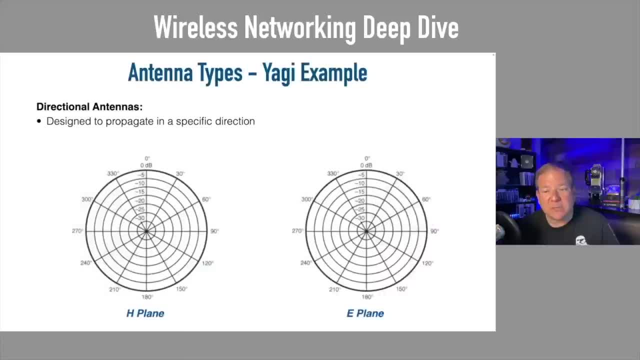 you can go for miles with these dish antennas sometimes. Now I want you to be able to recognize the plot graphs. You might need to know this for the encore exam If you're looking at a Yagi antenna. nope, I advanced too soon. 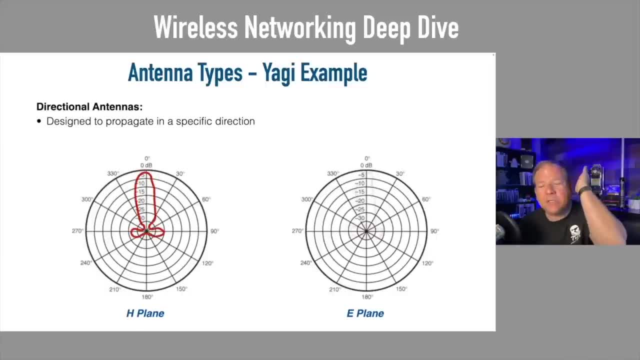 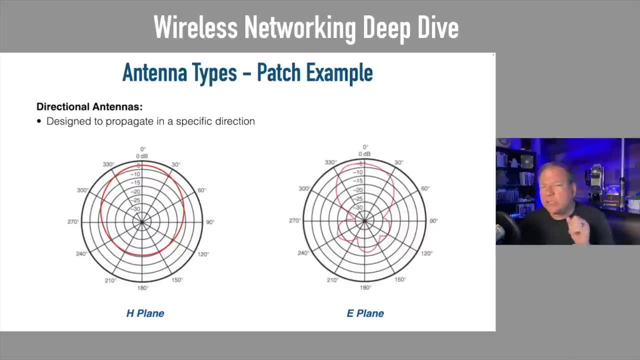 A Yagi antenna. it's going to be. it's going to be very, very directional, like you see here, Like going down a hallway: The patch antenna. I said it wasn't super directional but it's going. let me. 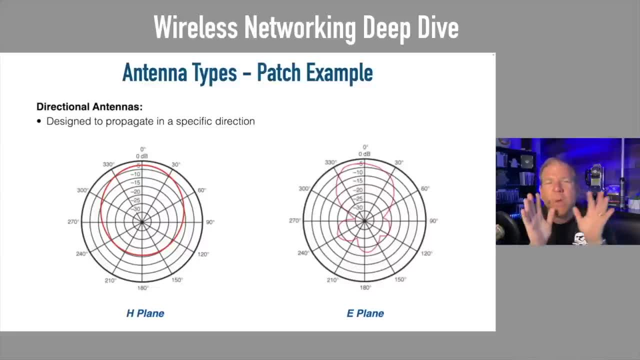 I didn't mean to advance there. It's not super directional, but most of the energy is focused in one general direction. So that's what we see here. This is the the plot graph of a patch antenna. So just to sum up what we said about antenna theory. 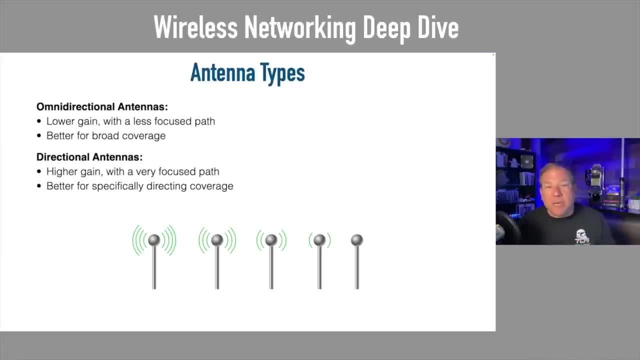 we've got two main types that I want you to know for exam purposes: Omni-directional: they want to, in general, go in equal directions, equal strength in all directions. It's not perfect. I mean, our dipole isn't going to give us great coverage. 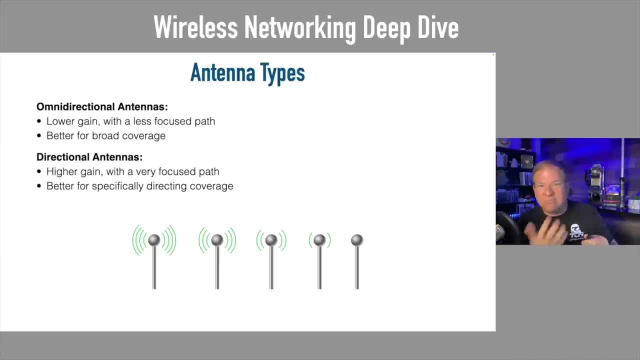 going straight up or straight down, because we're just not. there's no plane of charge that radiates out in that direction, but it does a pretty good job in all the other directions. A directional antenna: that's where we want to take our signal strength and focus it. 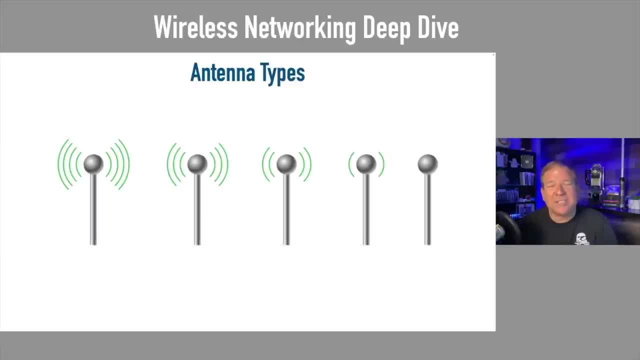 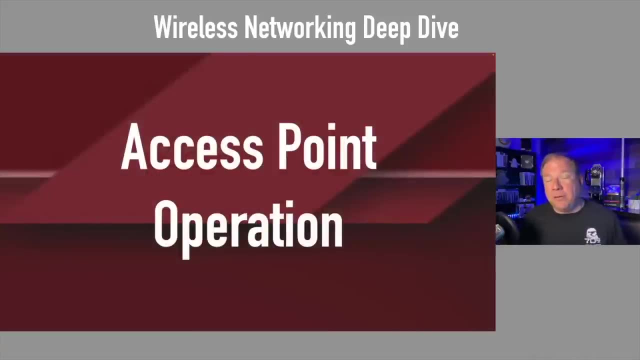 in a general direction. So that's a look at antenna types And welcome back for the break, everybody. Hope you're rested and ready to go for the next session or the next section in today's class- And we're kind of Star Wars themed today- 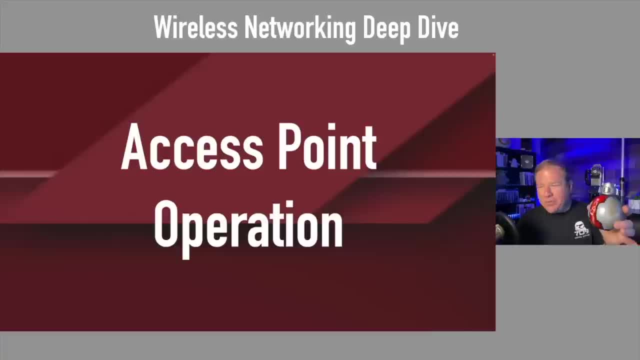 if you haven't noticed, So I thought I would quench my thirst with a thermal detonator of Diet Coke. If you've ever been to Galaxy's Edge down at Walt Disney World or in Disneyland, you can find it on your favorite app. 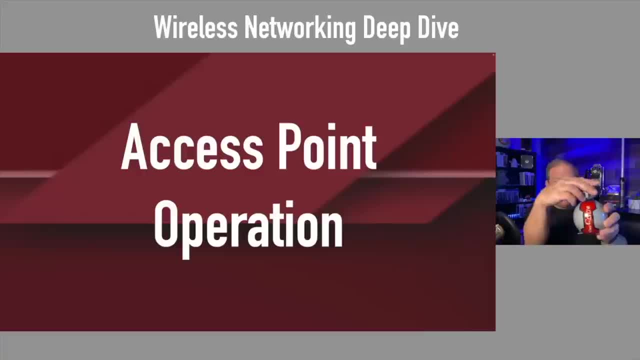 When you buy Coke or Diet Coke, they put them in these little thermal detonator containers, which I absolutely love. But hope you enjoyed your break And thanks to everybody that took advantage of our webinar only discount offers. All right, let's get going with some access point operation. 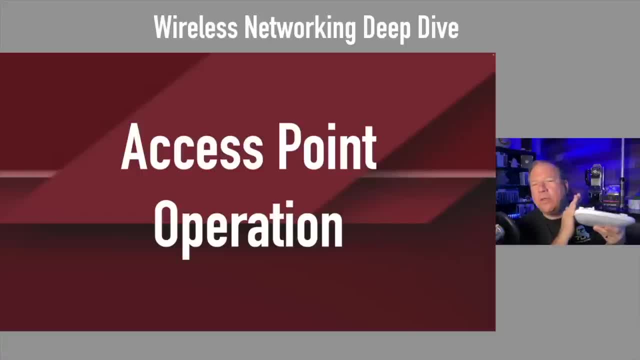 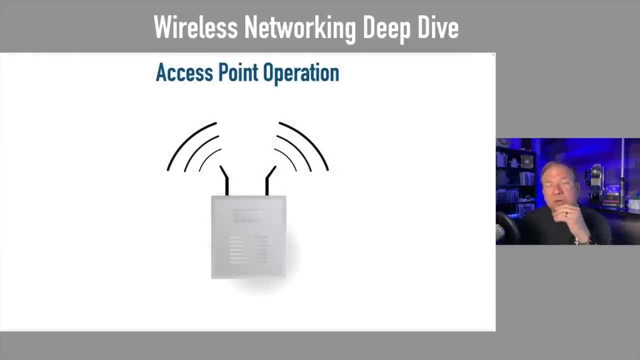 Let's go through the process of what happens when we power. one of these access points on What happens between the time we apply power and it starts doing its thing And doing service. So let's get into the step-by-step process, And this is specifically relevant to the Encore exam. 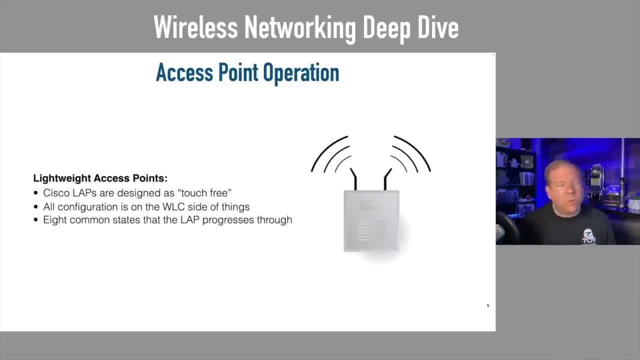 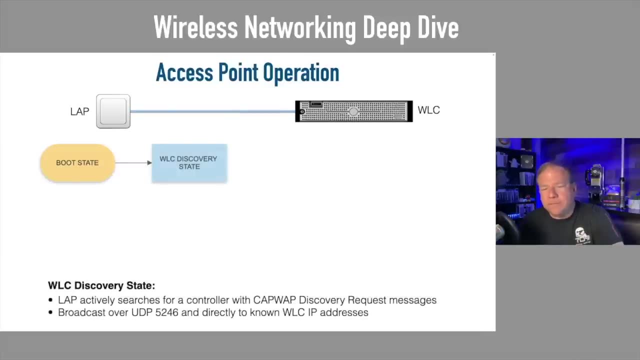 First we know that. make sure we're on the correct. there we go. I needed. I wanted to advance to that slide. Let me back up just a little bit. There's the slide I wanted to be on For our lightweight access point operation. 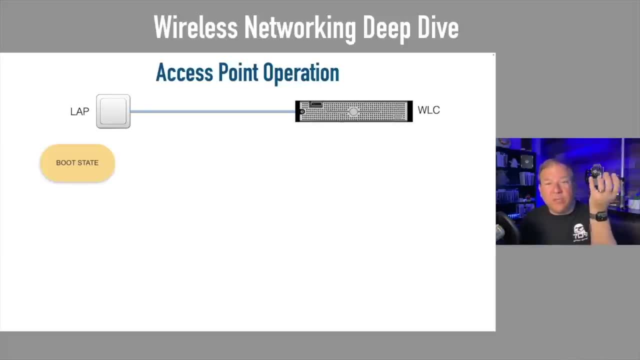 the first thing that happens is our access point boots up, So we apply power to it And here it's got an internal kind of a miniature version of Cisco IOS or it's operating system that it's gonna boot from And it's gonna get an address, maybe from a DHCP server. 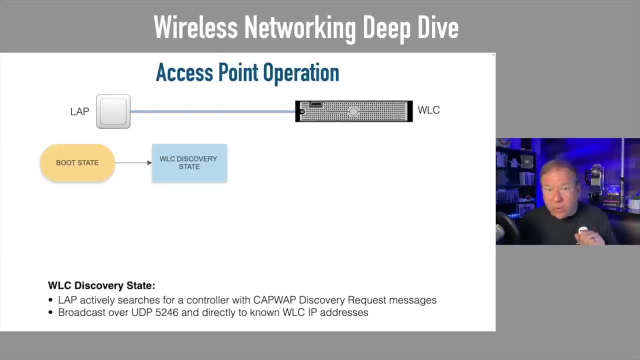 And it tries to locate it's wireless LAN controller. You have to locate it's wireless LAN controller. It's gonna go through a few different steps And we're gonna go through those steps together in a few moments, But it's gonna try to destroy it. 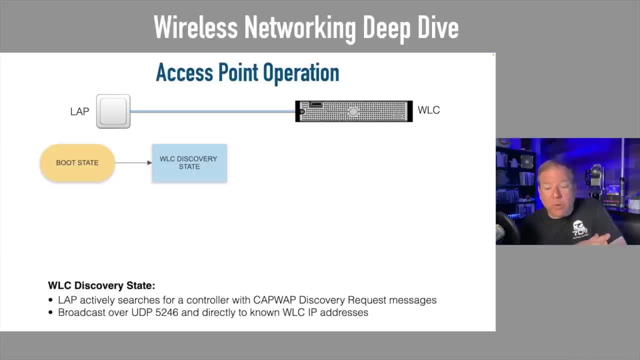 to discover, unless it's already been pre-programmed with one. it's going to try to discover a wireless LAN controller And after it does that CAPWAP secured tunnel that we talked about, that tunnel is established And over that single secured tunnel we're going to be able to send. 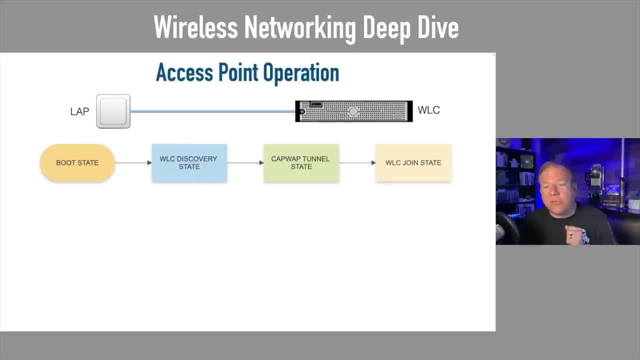 data and control traffic to the wireless LAN controller. And then we say: I would like to join you, I would like to be associated with you, Mr and Mrs Wireless LAN Controller, And assuming that happens, the wireless LAN controller says: let me check what version of firmware are you? 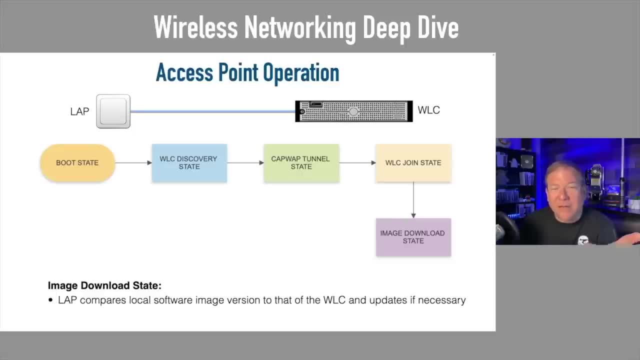 running on your access point And the access point says, oh, I'm running version X, And the wireless LAN controller might say, awesome, that's the current version, let's rock and roll. Or it might say, oh, you're a little bit out of date. And if the access point is out of date, then the wireless 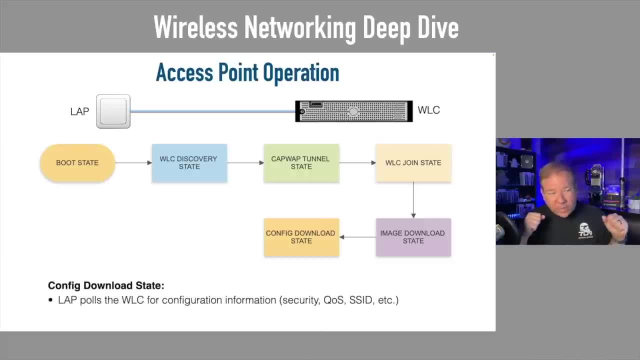 LAN controller is going to update it with the current version. It's going to have to reboot, But assume we're up to the current version now. the configuration for the access point is going to be downloaded from the wireless LAN controller. That is the big advantage of doing this lightweight approach. 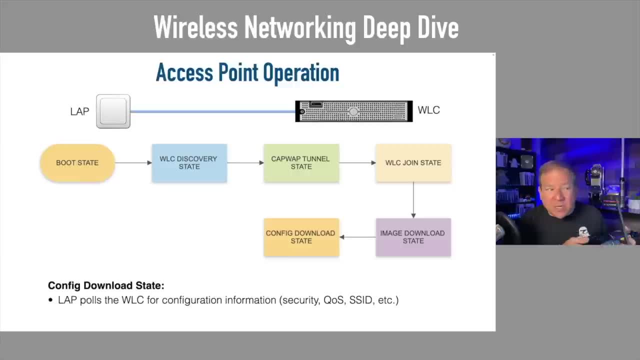 because, remember, we said with our autonomous access points we had to go configure everyone individually. Now we've got this single point of configuration on our wireless access point or, excuse me, on our wireless LAN controller, and it just gets pushed out to. 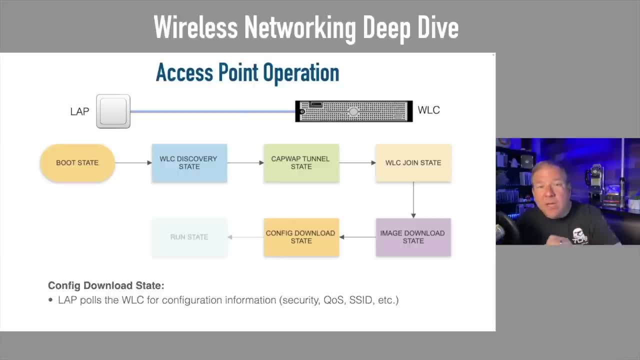 everybody. So now we're pushing out the configuration to this access point And now we're up and running. We're in our steady state. Now you can go in and administratively say you want to do a reset, and it goes through the process again. But that's how an access point goes from being. 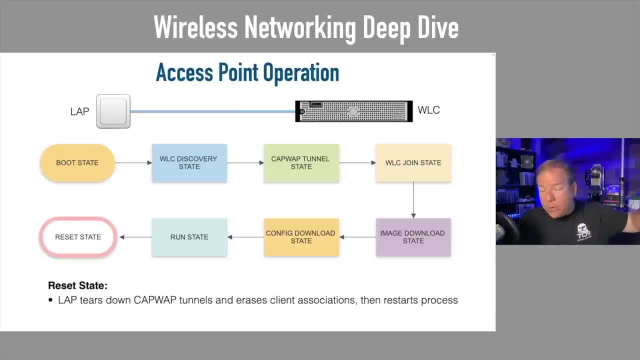 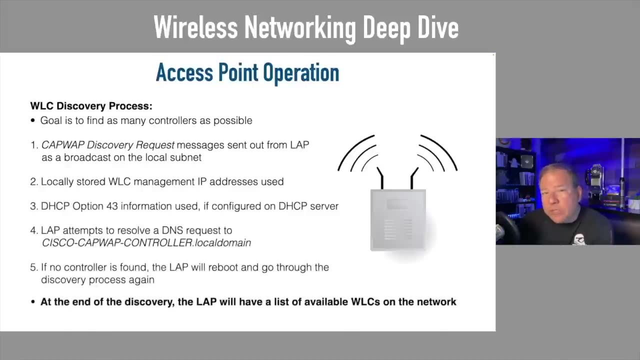 plugged in and getting power, probably using power over ethernet to the point where it is up and running. Now let's revisit something I said it's going to do when it boots up. it's going to try to discover- and, by the way, this is an 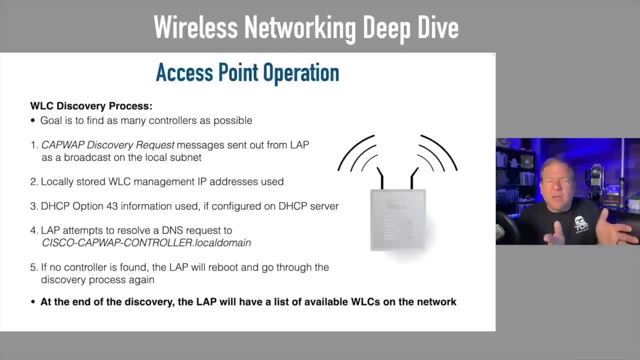 Encore topic. I'll try to point out some of the topics that apply to CCNA versus topics that apply to Encore. but this is an Encore topic. How does it go about trying to discover its wireless LAN controller? Well, one thing it'll do: it can send out a broadcast, And we know that a broadcast. 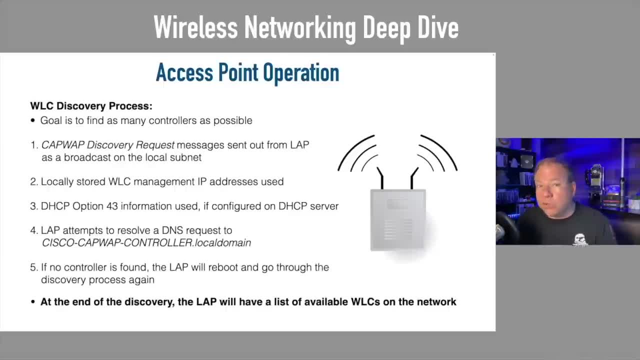 is only going to be seen on a local subnet. It's not going to go through a router. It's only going to go within its broadcast domain, which is a subnet or a VLAN. And if there's a wireless LAN controller on its local subnet, it can respond and say: 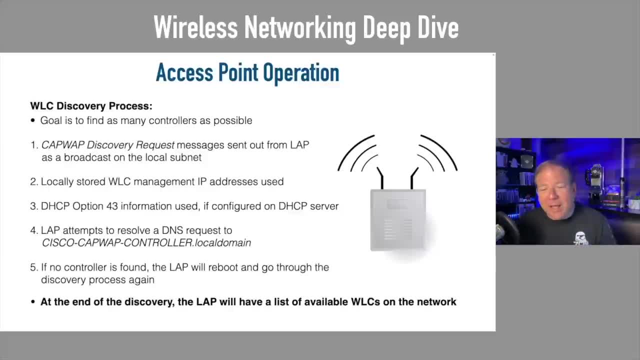 yeah, I'm a wireless LAN controller. Feel free to register with me Something else it can do. it's going to send out a direct request to join a controller if we have pre-programmed the access point with the wireless LAN controller's IP address. 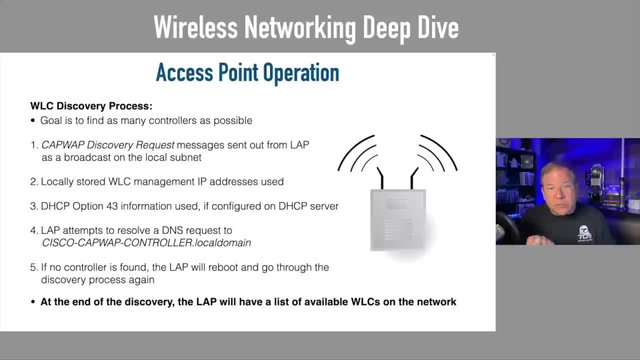 Now I've done that. Before you can actually go in with a console cable, You can go in and configure the access point directly. It kind of defeats the purpose, though, of having a lightweight access point, So, even though I have done it, I wouldn't recommend doing it, But you could if you're having trouble. 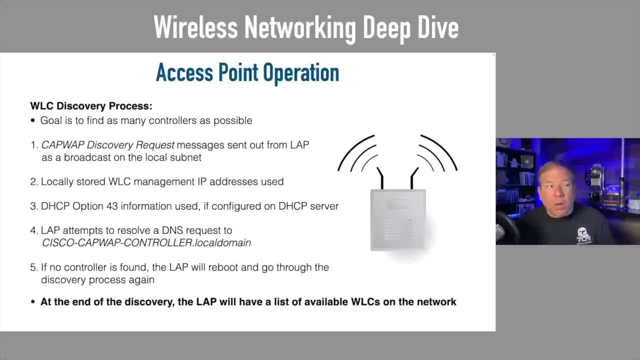 yeah, you can say: go to this IP address. Or when we went out and got our IP address information, initially from DHCP. a DHCP server says things like: here's your IP address. Here's your subnet mask. Here's your default IP address. Here's your IP address. Here's your default IP address. Here's your. 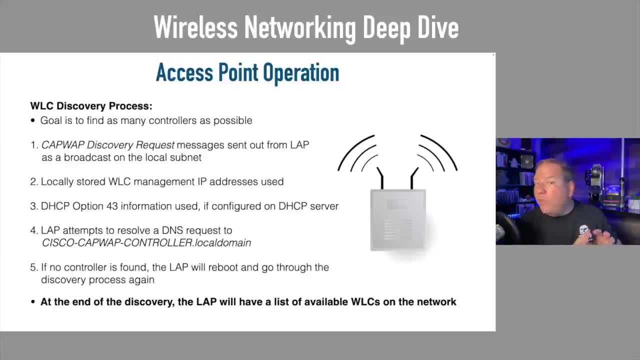 default gateway. Here's your DNS server, And we could have all of these different DHCP options that we provide. One of those options could be a special option called Option 43, which says here's the IP address of your wireless LAN controller. Or if none of that works, there is a. 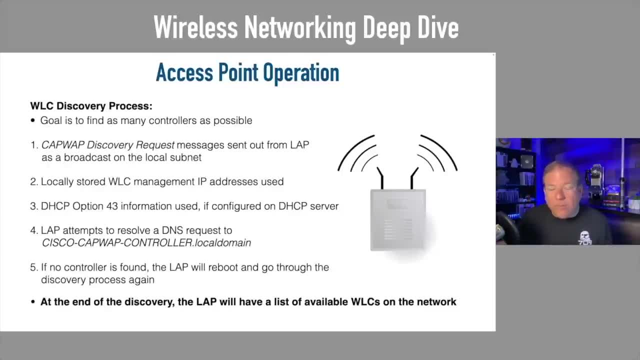 well known fully qualified domain name that wireless LAN controllers should be responding to, If we can configure this in our DNS and it's ciscocapwapcontrollerlocaldomain. So if we've configured that in our DNS server, then, yeah, we can make a request to the DNS server and it's. 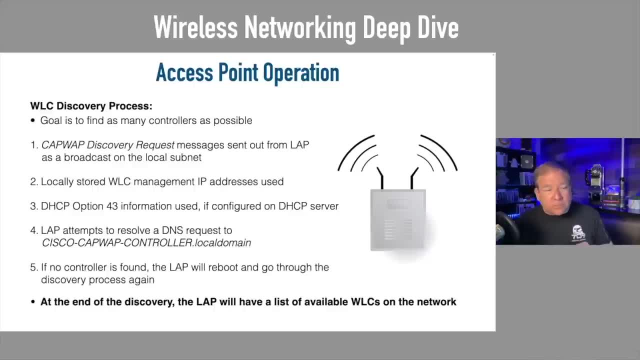 going to say: oh yeah, here's the IP address. So now, oh, by the way, what if none of that works? If it doesn't work, it reboots and it just gets in a stuck state. In my experience, if none of 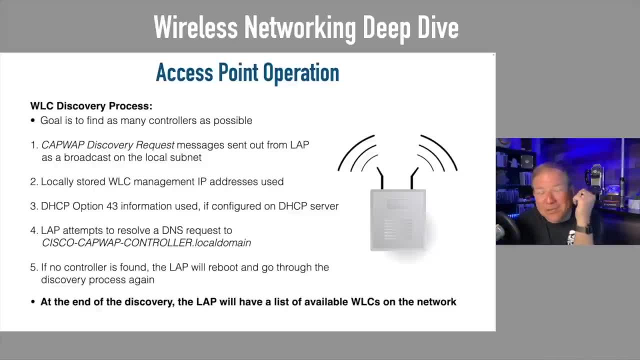 that works and it tries again. it never works until you go try to figure out what's going on. So it's always pretty disheartening to me if it reboots. But let's say that we found several controllers. I mean we tried that lots of different ways. Maybe there's multiple. 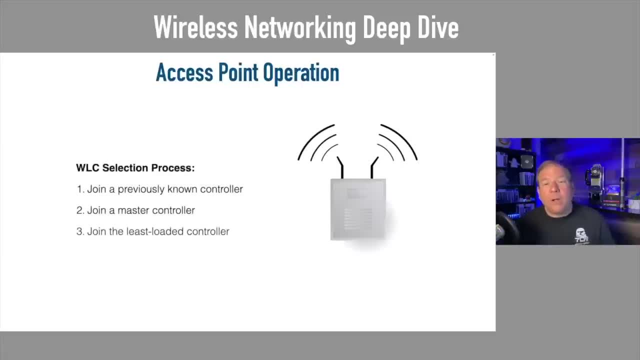 controllers out there. Which one do we use? Well, if we had already belonged or we'd already been associated and we had joined a controller previously, before we rebooted, we'll go back. I mean, that's our buddy. We've been there before, So we'll re-register with that. 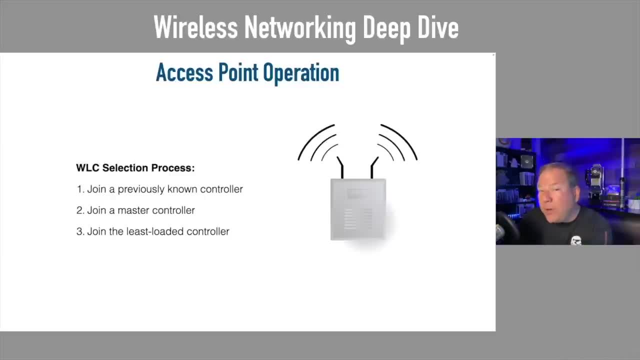 that we were just registered with a moment ago. Now, if we'd not previously been registered with a controller, or if that controller is no longer available, we can designate. if we have multiple controllers, we can designate one of those controllers as the master controller and we'll register with that. Or let's say that we've got. 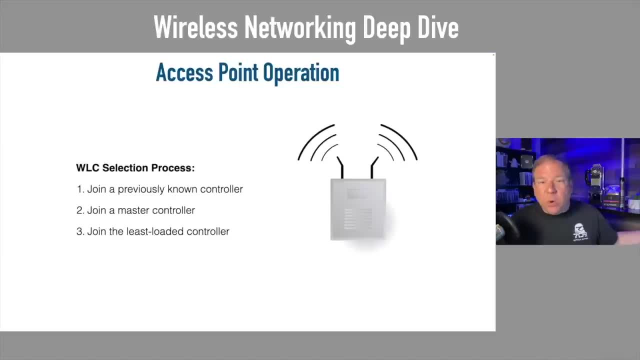 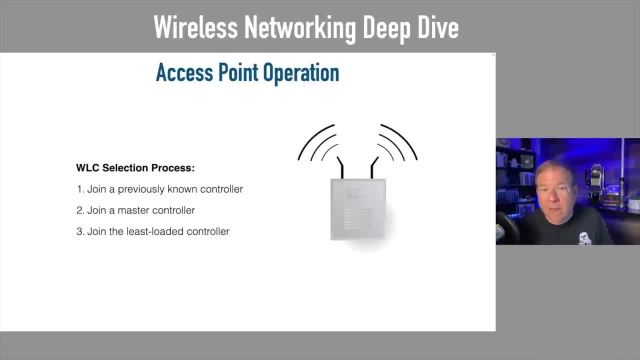 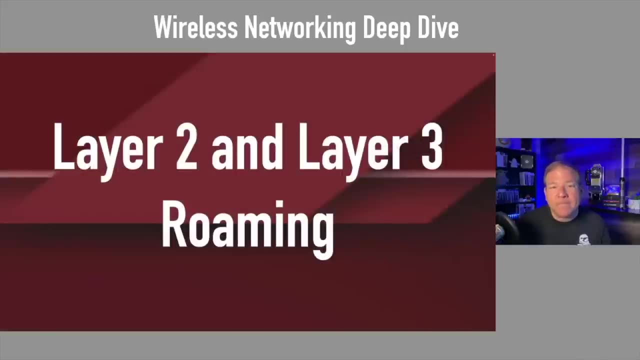 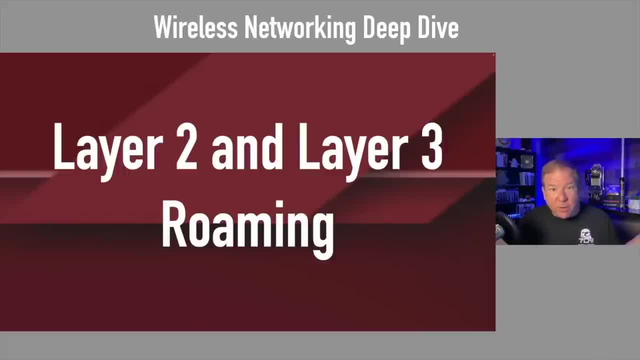 multiple controllers, which we might in a very large enterprise environment. I mean, we're going to have multiple access points. Maybe we want to have multiple controllers to control those multiple access points. What if I'm kind of roaming around the building? I've got my laptop, I've got my 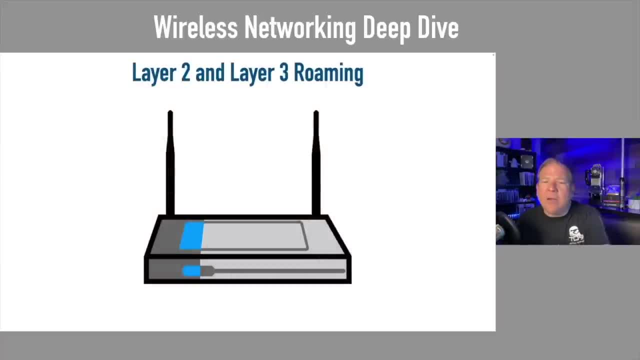 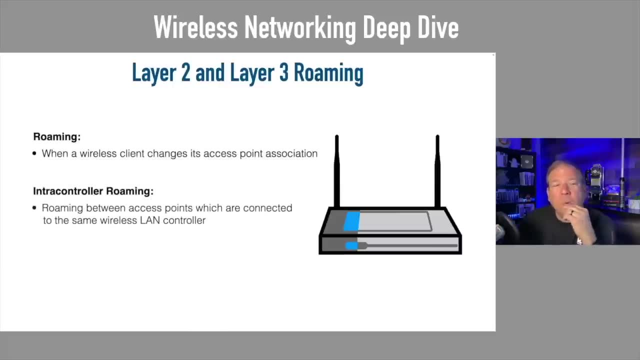 wireless phone. How do I roam from one device or one access point to another? We've got some options. We could do what is called intra-controller roaming. That's where I go from one access point to another access point, but those access points they're both controlled by the same controller. 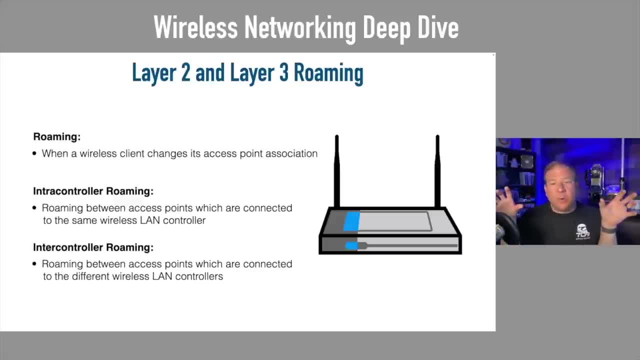 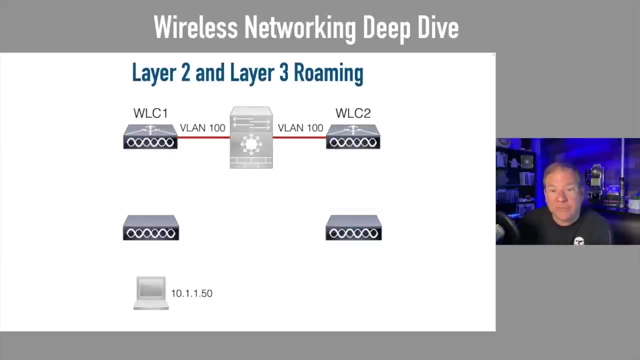 Perhaps I go from an access point to another access point, but they're controlled by their own Different controllers. Will that work? Yeah, it sure can. Let's check it out Here. I'm doing roaming from the access point on the left to the access point on the right And notice they're. 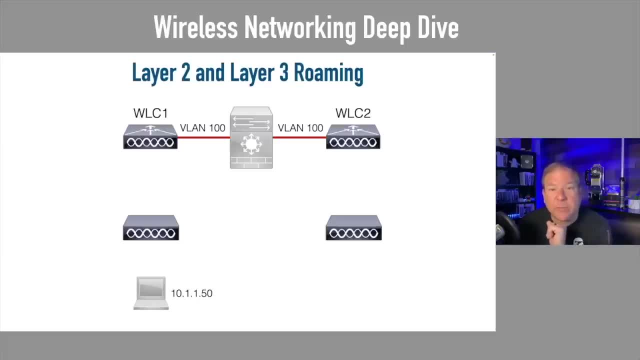 each controlled with different wireless controllers. I've got WLC1 on the left, WLC2 on the right. Now, in this case, we're all part of the same big happy VLAN. We're all part of the 10.1.1.0.. 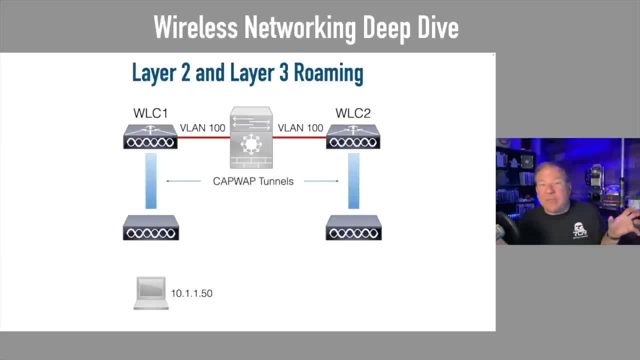 Slice 24 network And these access points. they've got those CapWeb tunnels going up to their controllers. And if I'm just roaming around and I roam over to that access point on the right, do I get to keep my IP address? Yeah, I sure do. In fact I'm still part of the same VLAN. I'm. 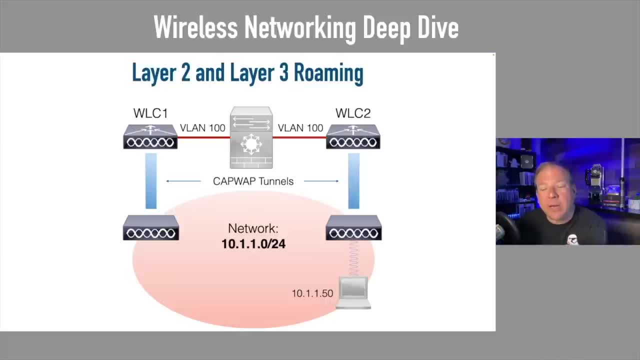 still part of VLAN 100.. I just happen to be talking to another access point, But it's on the same VLAN and I am, So no worries, It's the same SSID, So it's totally transparent to me. It gets a little. 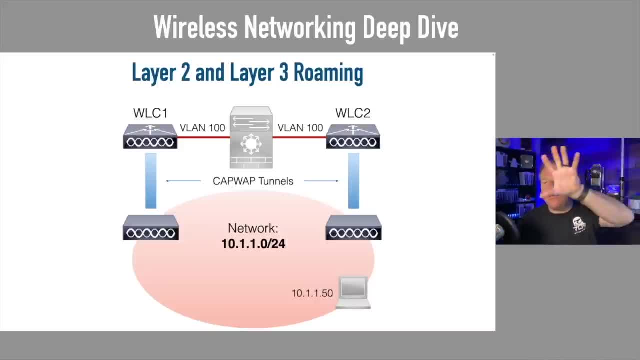 bit more tricky if I go from one controller to another controller and they're in different VLANs. Check this out Here. I've got a VLAN on VLAN 100 on the left which has the address space of 10.1.1.0., Slice 24.. I've got the controller on the right which is 20.1.1.0., Slice 24.. That's. 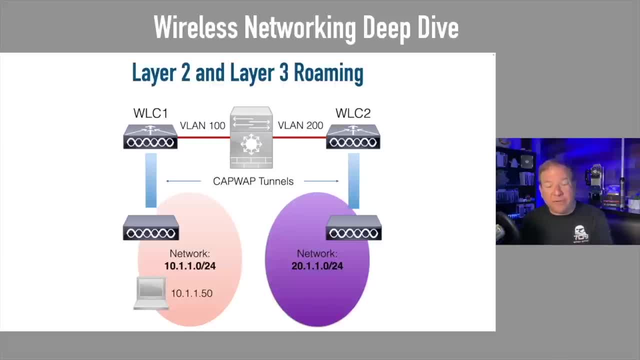 20.1.1.0.. What if my IP address of 10.1.1.50 assigned to my laptop or PC? what happens to it as I roam from one access point over to this other access point in a different VLAN? Do I have to get? 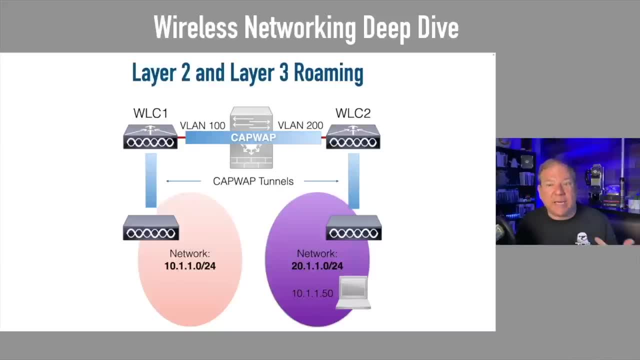 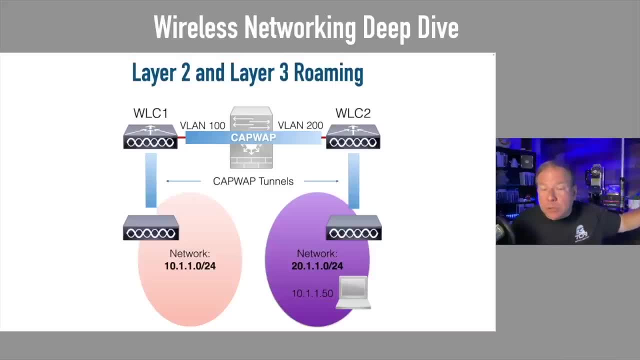 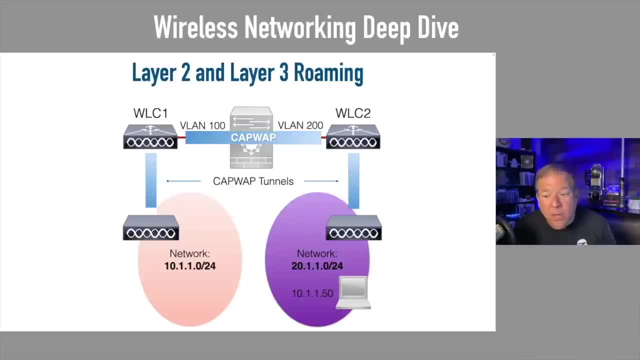 different VLANs. they can have a cap-wap tunnel between them as well. So I can go through this foreign wireless LAN controller over to my original wireless LAN controller, My original wireless LAN controller. I'm anchored to that. It's called my anchor controller. I just have to. 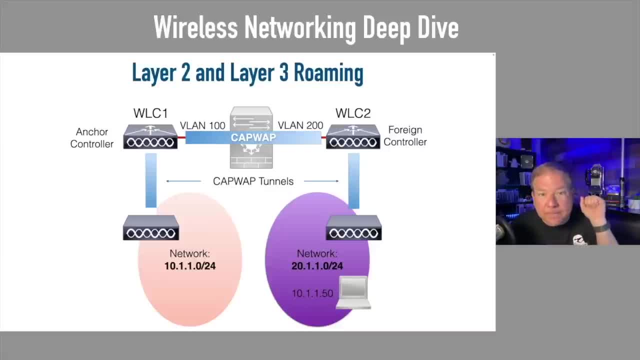 happen to be going through my foreign controller to get there And there's the cap-wap tunnel, so my data still flows over to my anchor, to my original wireless LAN controller. So still, the bottom line is, even though I'm roaming between VLANs, this is transparent to the end. 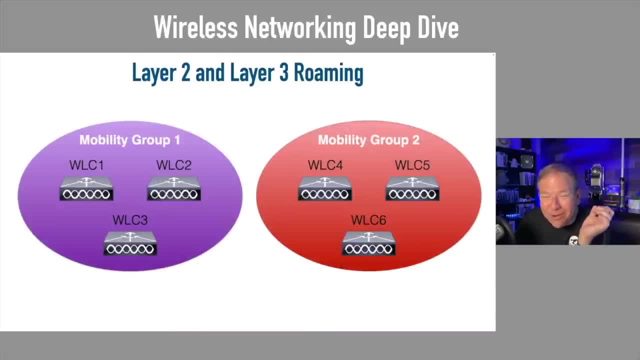 user. If I've got a very large network, though, and I've got lots and lots of wireless LAN controllers, there is a time- and I want you to know this, it might be good for your notes- there is a time where I am going to have to get a new IP address and my connections are going to be reset. 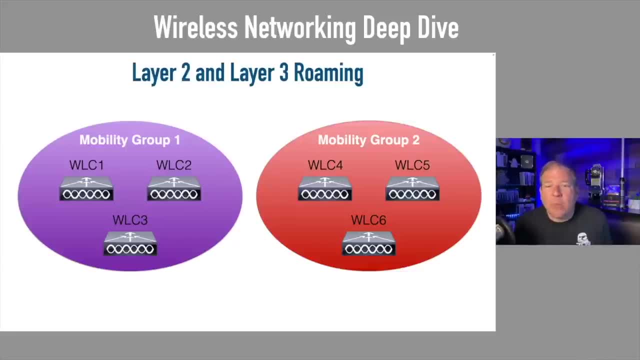 and I might have to re-authenticate. I used the term mobility group earlier. A mobility group is a group of access points that know about one another. So here I've got mobility group one, mobility group two. So within a mobility group, that's. 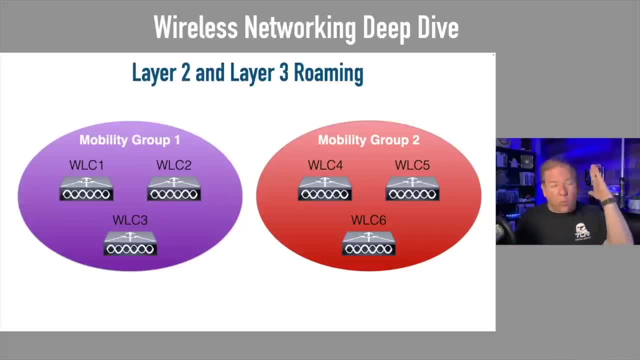 what we've been doing up till now Within a mobility group. I can go from one to the other to the other, And I can go from one to the other to the other, And I can go from one to the other to the other, And I can still be anchored to my original controller. We call it the. 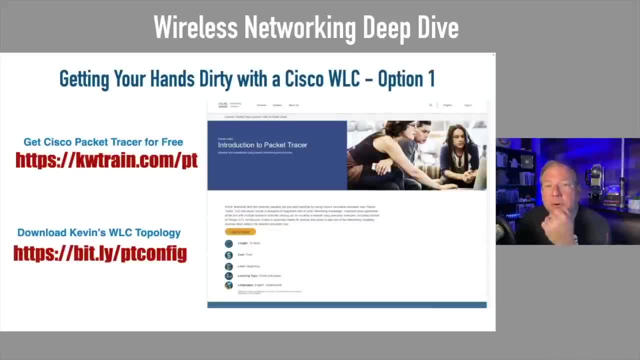 anchor controller. But if I move between mobility groups, game over, I've got to get another IP address, I've got to basically reset my connections, I've got to re-authenticate. But in larger environments or for security purposes, that's what you might find in an 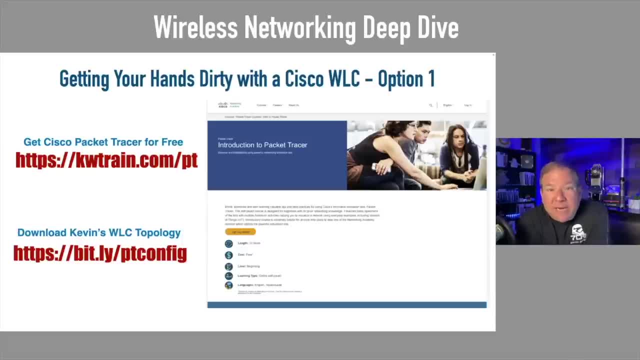 enterprise. Now one of the questions you might have- in fact, I've already had this question come in- is: how do I get to my IP address? How do I get to my IP address? How do I get hands-on experience, Kevin? How do I practice on this? I don't have a wireless LAN controller. 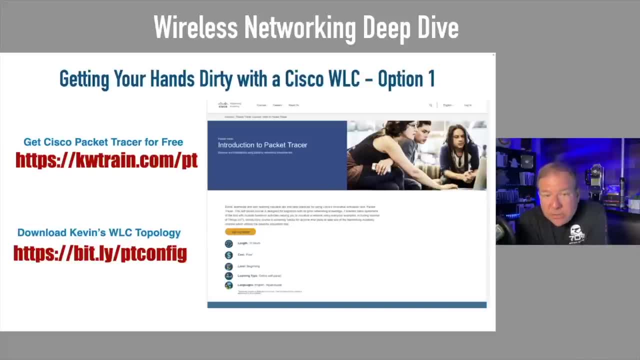 Well, I've got a few options for you. I've got three solutions. Let's go through them one at a time. The first solution, I think, is perfect. if you're a CCNA candidate, On the CCNA exam blueprint, it tells you very clearly what you need to be able to do. I think I might have 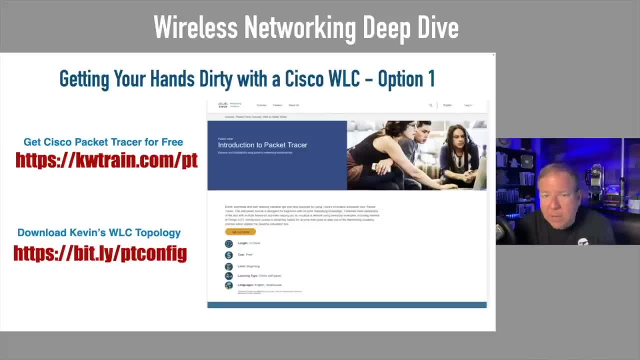 mentioned it earlier. It says you need to be able to create a wireless LAN, configure security for pre-shared keys. Yep, you've got to do pre-shared keys. You have to use AES encryption, You have to use WPA2.. I'm actually going to do that for you today. I want to show you how to do. 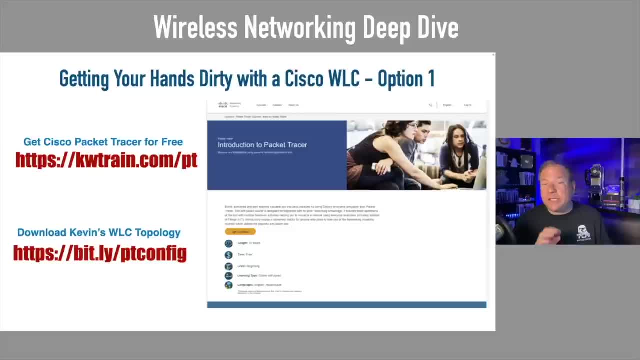 it. How can you do that? Well, Cisco gives you for free this piece of software. It's a simulator called Cisco Packet Tracer And beginning in- I don't remember if it was version 7.2 or 7.3,. 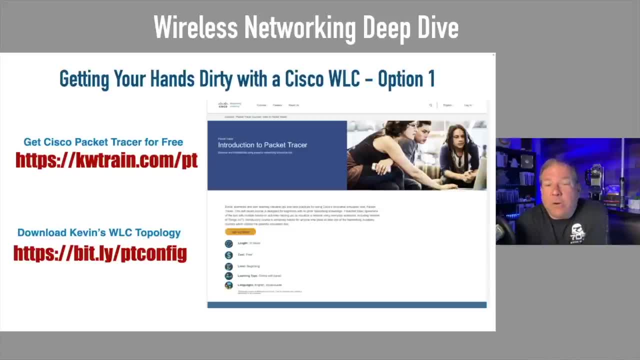 I think it was 7.3.. Um, they started offering wireless LAN controllers And you can. I just gave you a shortcut so you didn't have to try to find it on the web. You can go to kwtraincom slash pt. That will redirect you. 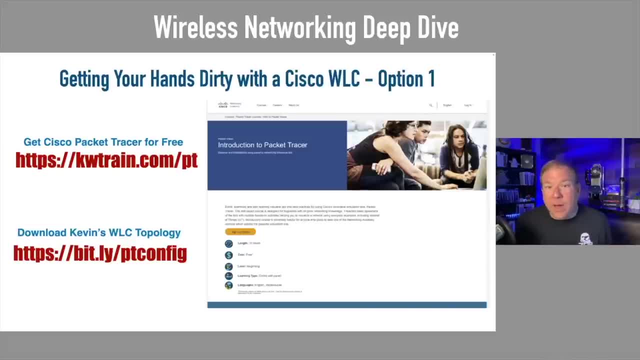 to Cisco's website where you can get your free copy of Cisco Packet Tracer. Excuse me, You can get your free copy of Cisco Packet Tracer Now. to do that, you're actually- you're actually registering for a class. You're registering for a class with the Cisco Networking Academy called. 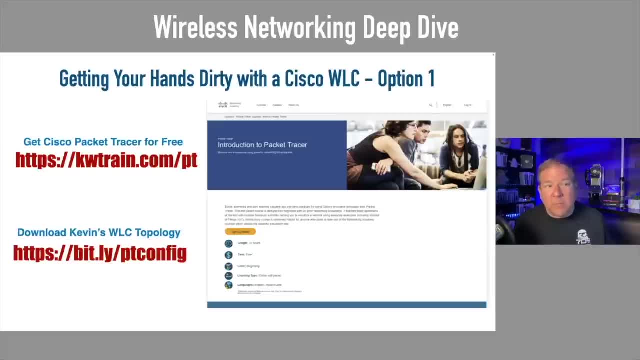 Cisco Packet Tracer. It's free, But once you get registered you can then download a copy for free of Cisco Packet Tracer. Once you get your copy of Cisco Packet Tracer, you can just start creating all kinds of topologies. It is an amazing piece of software. Cisco is so generous to give us that. 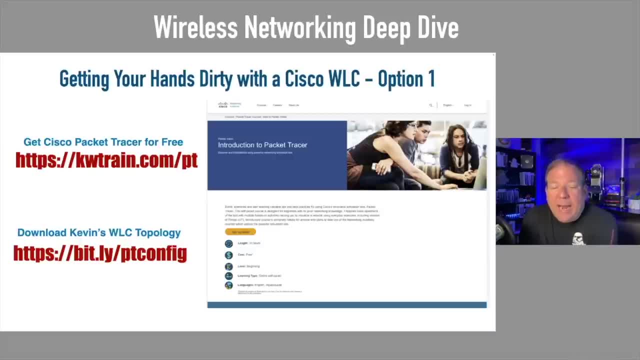 very robust free piece of software And to work with wireless networks. I want to give you a head, a pkt file that has a fully functional wireless network in it. I'll show it to you in a second, But if you want to download that, that free pkt file that you can then upload, you can import. 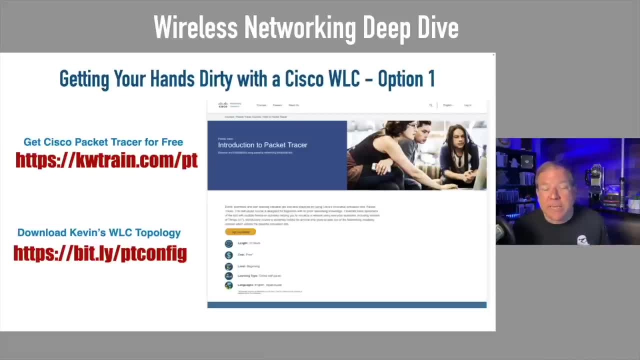 into your copy of Cisco Packet Tracer. go to bitly b-i-t dot l-y slash p-t config, b-i-t dot l-y slash p-t config, And that'll download a pkt file. And let me show you what. 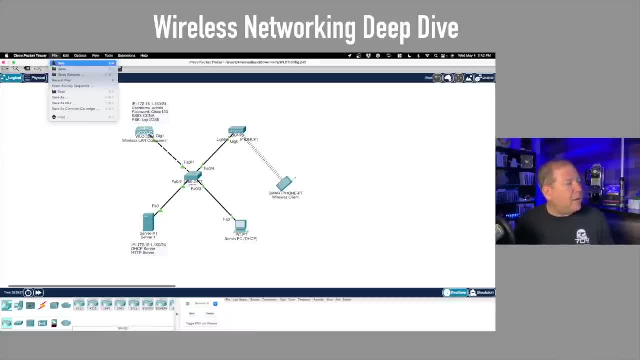 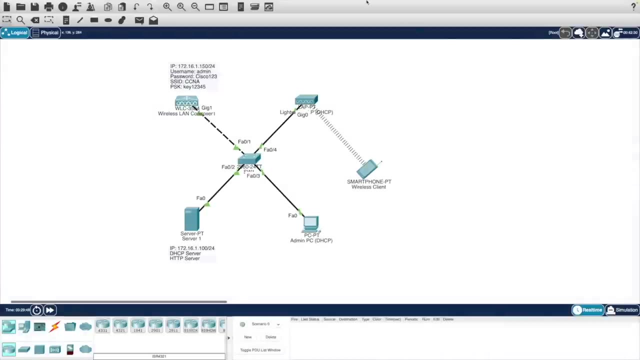 I've got here. You're just going to go under file and you're going to say open. In fact, let me, let me, let me take my face off the screen here so you can see this a little bit better There. that's a little bit larger for you. You're going to go under 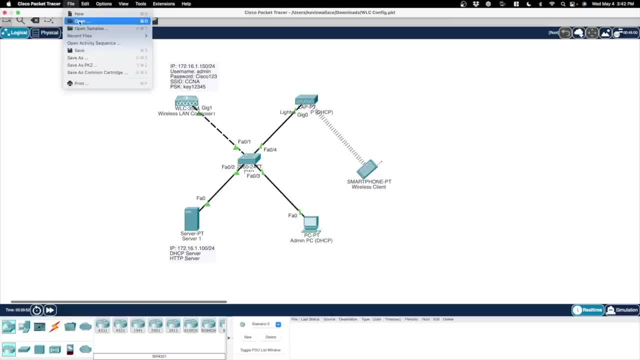 file. You'll say open and you'll open that pkt file that you've downloaded And notice what I've got here. I've got a switch. I've got a wireless LAN controller. Here are the credentials for it. I've got a smartphone. That's going to be my wireless. 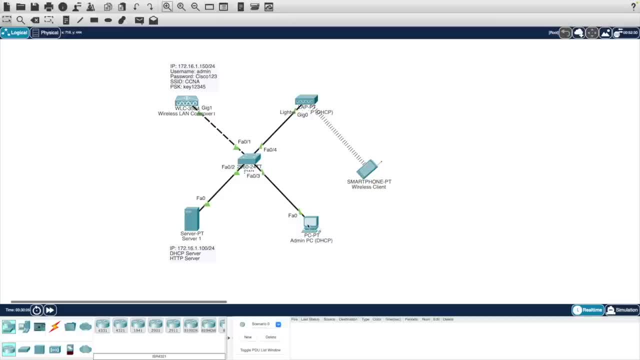 client. I've got a PC. I can use the browser on this PC to do administration on this wireless LAN controller. In fact, let's do. let me just show you how easy this is. I'm going to open up, I'm going to click this PC and that opens up a separate pane And I'm going to go to the desktop. 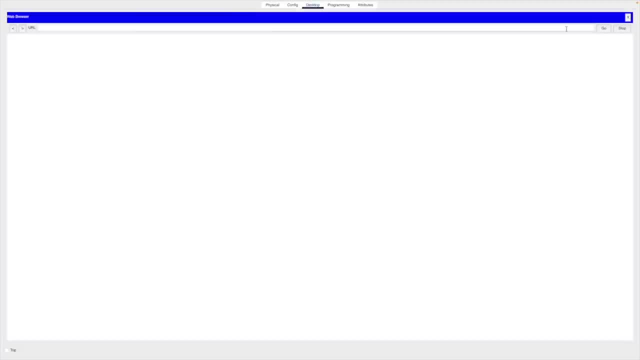 of the PC. I'm going to open up a web browser and I'm going to go to https, colon slash, slash, 172.16. .1.150.. And then I get to log into this wireless LAN controller. You see, here's the IP address. 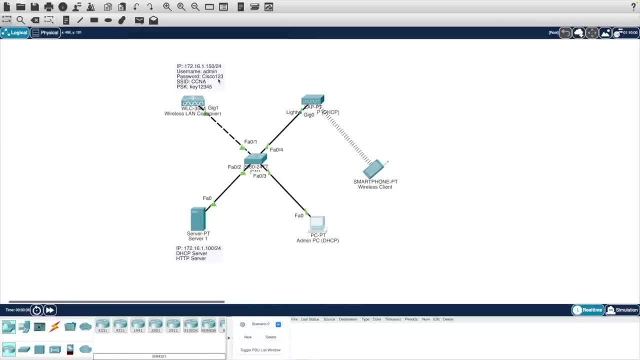 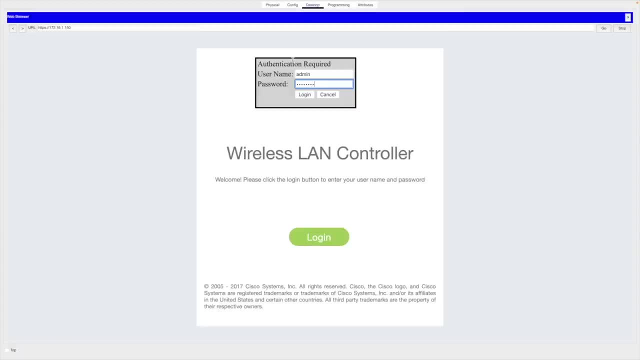 So that's how I knew that The username is admin, The password is Cisco123, capital C. So let me log in. Let's say admin, Cisco123.. Oh, I must've mistyped something. Let me try again. Oh yeah, I hit caps lock. 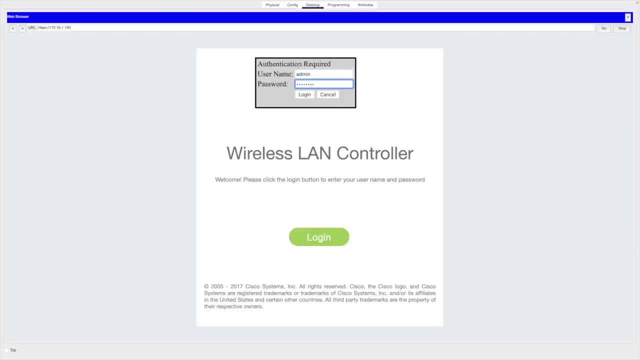 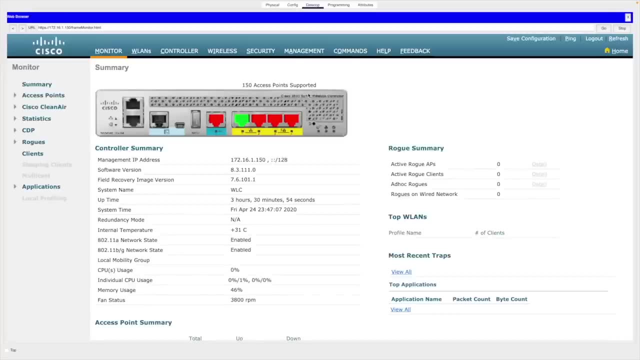 Admin, Cisco123.. And look at this. This is in a simulator that you can get for free And this looks like a we're on a wireless LAN controller right now. folks, This is pretty cool. Now, admittedly, this is a simulator. It's not going to do everything that a real live. 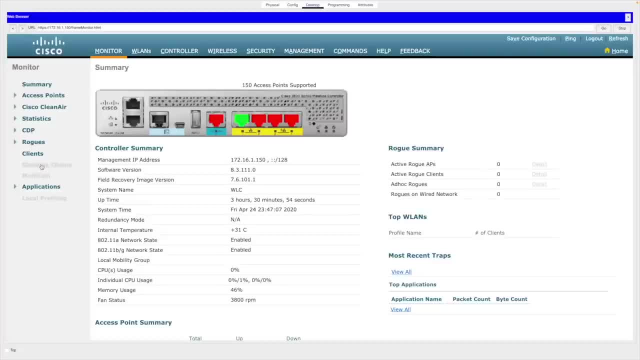 wireless LAN controller would do- Like some things are great at, you're not going to be able to do, but you can do everything that you're told that you need to do for Cisco's CCNA exam. In fact, I'll come back here later when we 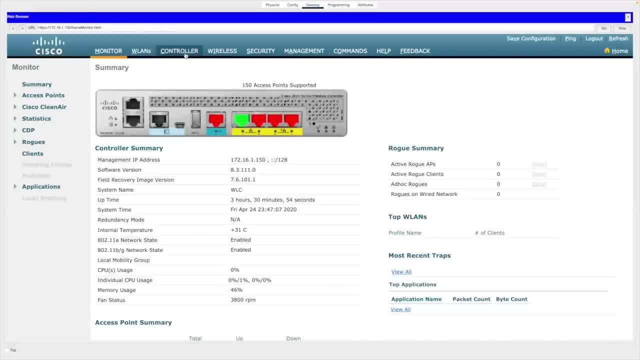 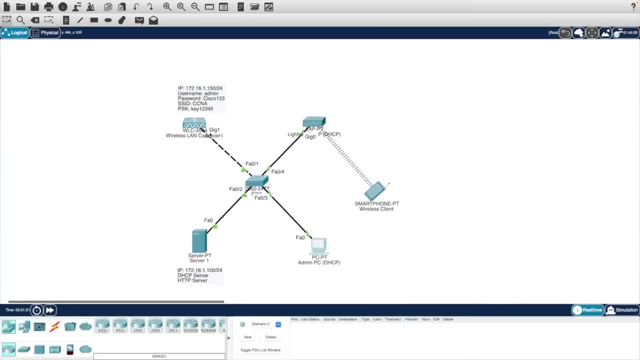 talk about security and I'll show you exactly what you have to do. But how cool is that You get to? you get to get this free access to the simulated wireless LAN controller. That's one option And that's my recommended option If you're going to be going after your. 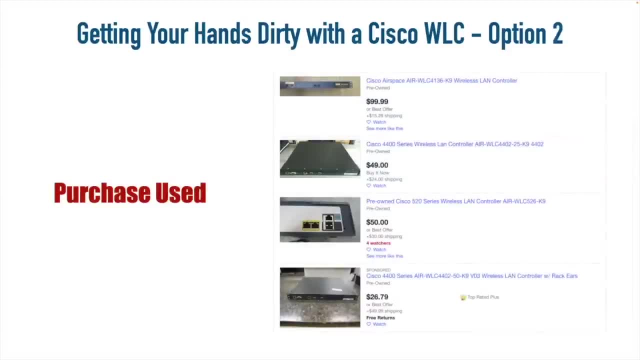 CCNA. A second option is you can go on to eBay or somewhere and you can buy a U-Buy. I've done that as well. You can get it for probably well under a hundred dollars. I've done that. I've used it in class. It works. I've not had as great a luck with this. 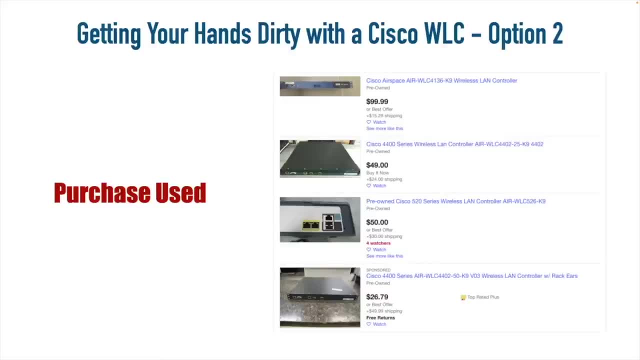 because what you buy on eBay, you're probably not going to have the smart net maintenance contracts, You're not going to be able to update the firmware on it And it's probably going to be lacking some features because it's probably old. When I, when I got mine, they had 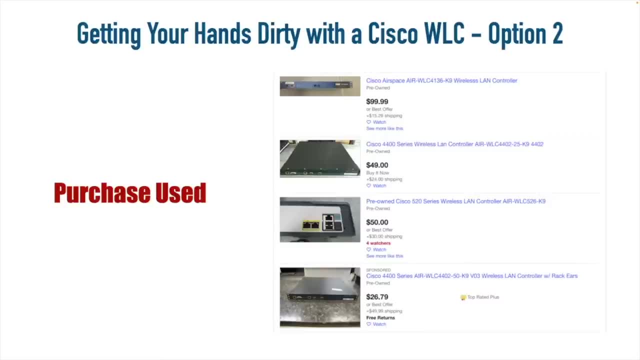 neglected to include, like RAM or something really critical. I had to get that And then the, the, the, the license, the digital certificate expired on me. It was kind of a pain. I just wanted to let you know that's an option If you want to get your hands on. 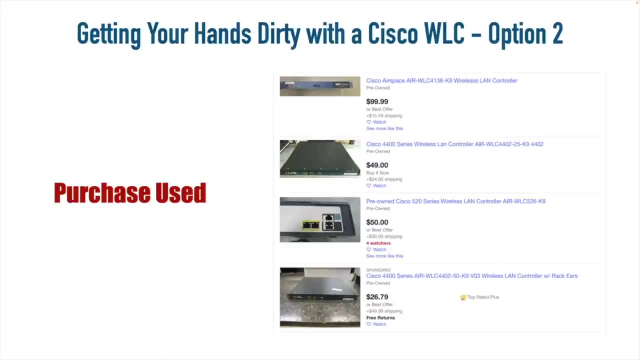 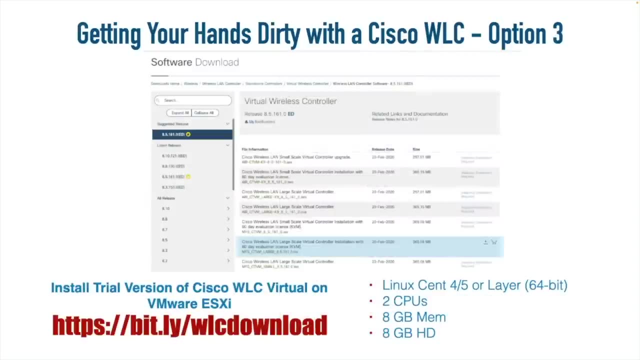 some physical gear. I really don't recommend that, but it is an option for those of you going after your Encore exam and you need to do more than you can do with the the packet tracer version. You can get a fully functional virtualized wireless SYNC controller from Cisco for free. 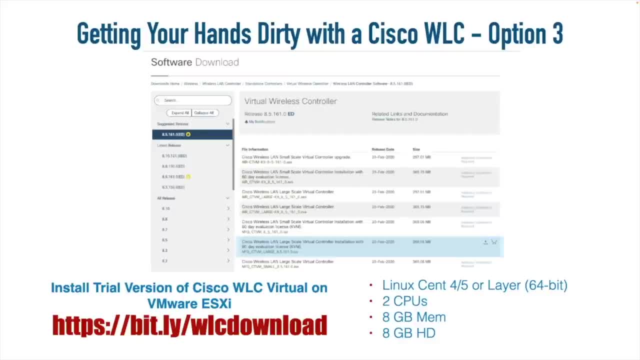 We're not stealing here. They give it to you for free. You can get a free Cisco account- unless you're you probably already have one If you're going after your Encore exam. but you can log in and I created a shortcut link for you. You go to bitly. B-I-T, dot, L-Y, slash W-L-C. 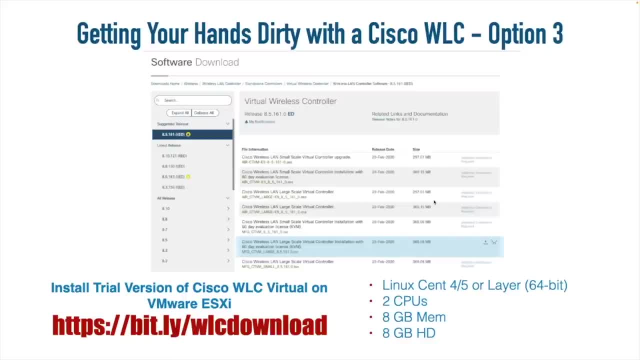 download and you'll go to this screen And this is the download screen for their wireless SYNC controller software. Now you'll you'll have to log in And once you log in, most things are going to say additional entitlement required, meaning they're not giving it away for free. You got to, you got to buy it. 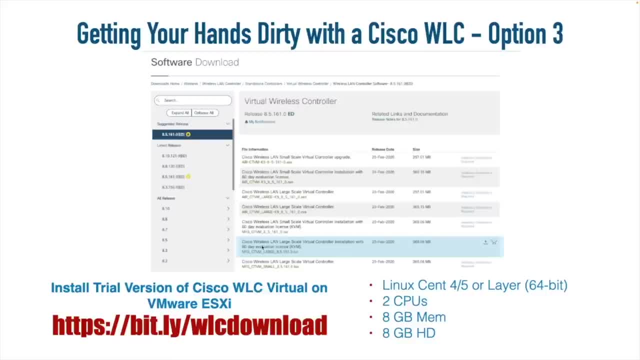 but they give you a trial version, a 60 day evaluation, for free, And that's the only one that's going to be downloadable. but it is a large scale virtual controller installation with a 60 day evaluation license And you can run this in a virtual machine. Now, personal experience, this has been a little bit. 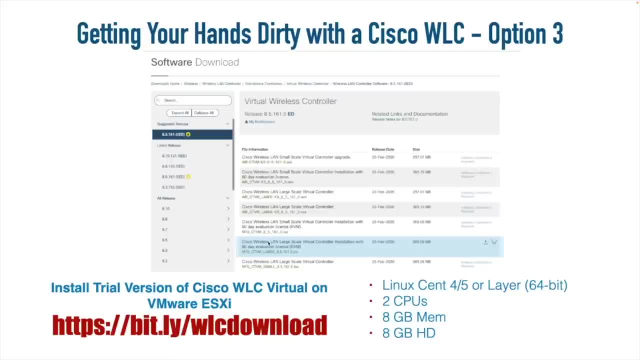 finicky for me. Sometimes I get it to work, Sometimes I don't get it to work, but I made some notes when I did get it to work. but I'm running this right now on VMware ESXi And I set it up. You, if you want to take a screenshot, I set it up for 64 bit. 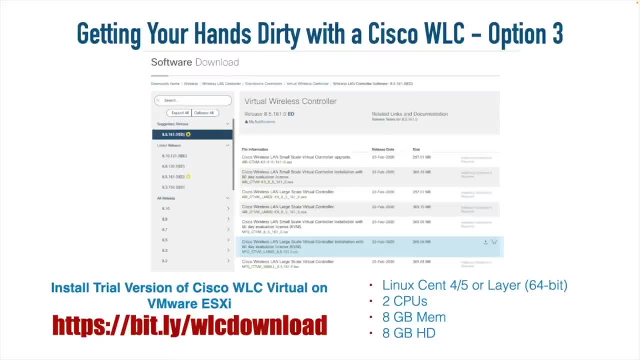 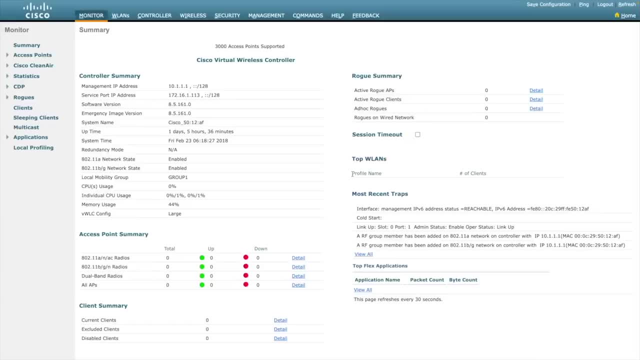 SYNC OS with two CPUs, three gig of memory, three gig of hard drive, And I'll show it to you Here it is. This right here is a fully functioning 60 day evaluation, So don't use it in the real world. 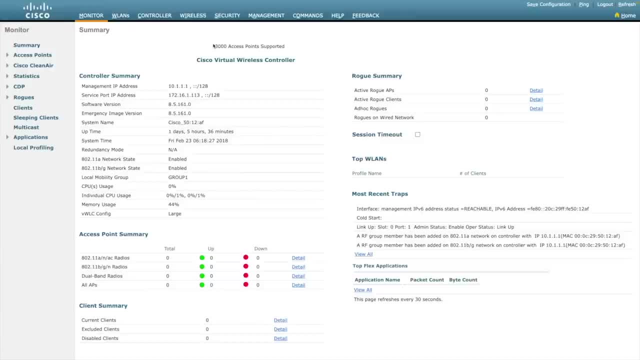 but this is a fully functional wireless SYNC controller. It supports 300 access or, excuse me, 3000 access points. I'm going to be doing some demos later today inside of this environment, So again, let me give you those URLs one more time. Let me back it up. 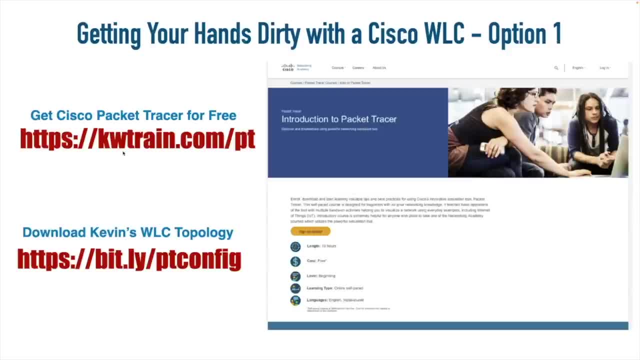 If you want to get packet tracer for free from Cisco as a shortcut, you can go to kwtraincom slash PTcom. And you can get a packet tracer for free from Cisco as a shortcut. You can go to kwtraincom slash PTcom. You might want to take a screenshot of this If you want to get my PKT. 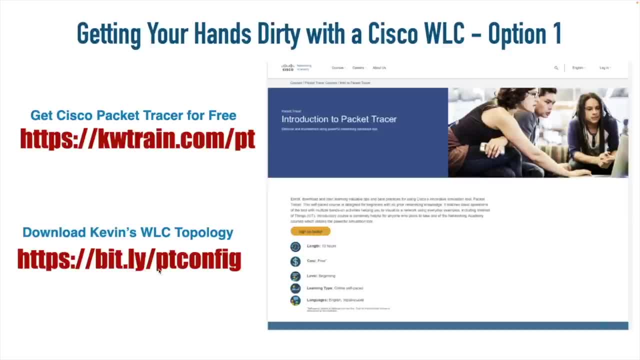 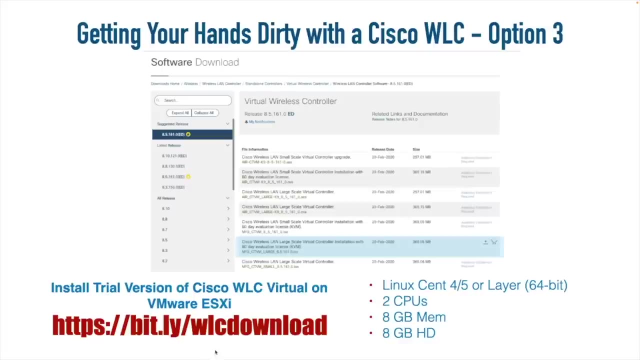 file you can go to bitly bitly slash PT config. Give you a second to screen cap that. Again, you could buy one used. I haven't had great luck with that. For Encore students I recommend going to bitly bitly slash WLC download. 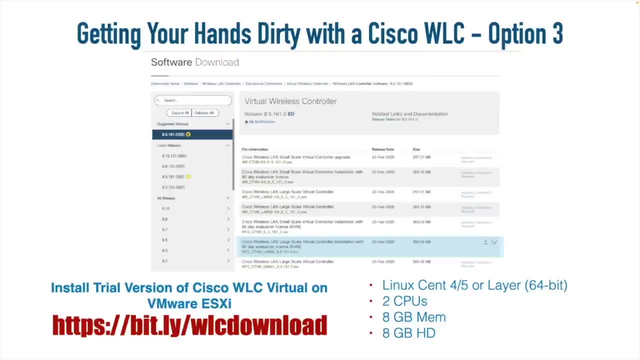 Log in with your Cisco credentials and you can get a packet tracer for free from Cisco as a shortcut. You can get a packet tracer for free from Cisco as a shortcut. You can download that fully functional 60-day evaluation license, run it in a virtual machine. It is amazing. It is full featured. 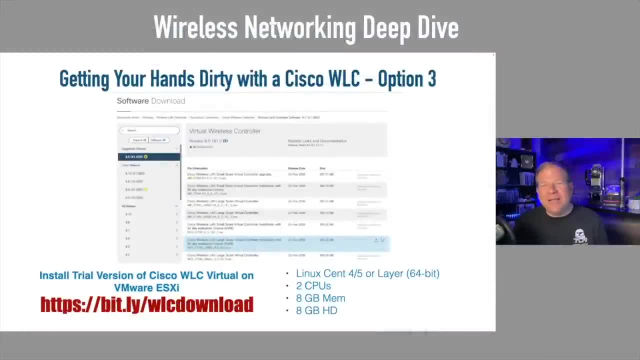 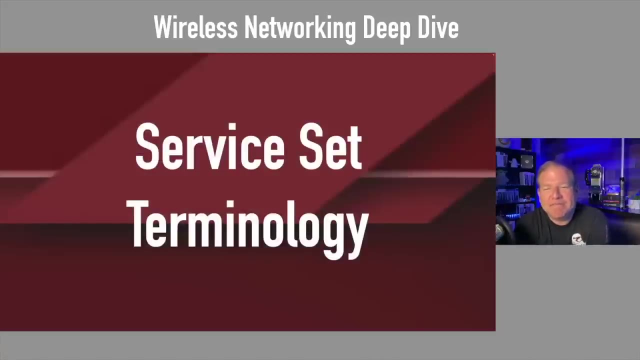 All right. Hopefully that will be helpful for many of you, getting some hands-on experience, And I'll actually be going out and when we do some demos later today I'll be doing demos in both the packet tracer and the virtualized WLC environment. But now for your notes. 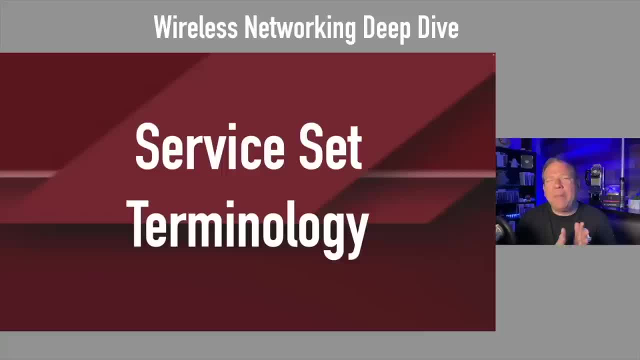 it's time for a few more definitions When we talk about the name of a wireless network. for example, on my phone, if I pull up my wireless settings and it shows me all the networks that are available to me, those network names are SSIDs, service set identifiers. But there are some other. 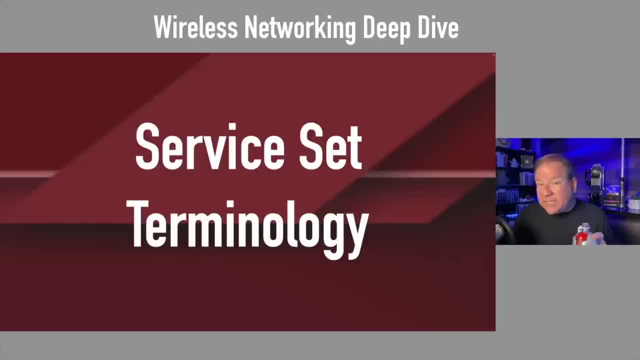 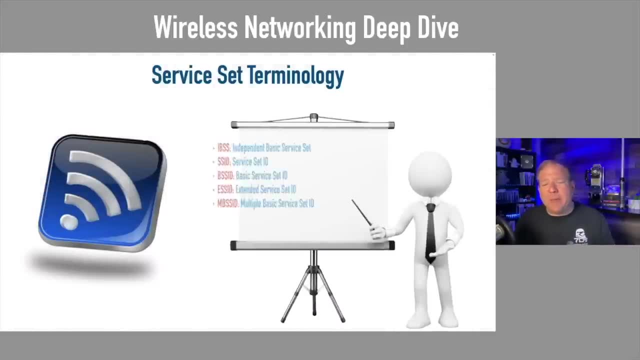 service set terms that I would want you to know for your CCNA exam. Here they are, and then we'll talk about them one at a time. But we want you to know about independent basic service set service set ID. I won't read them all. 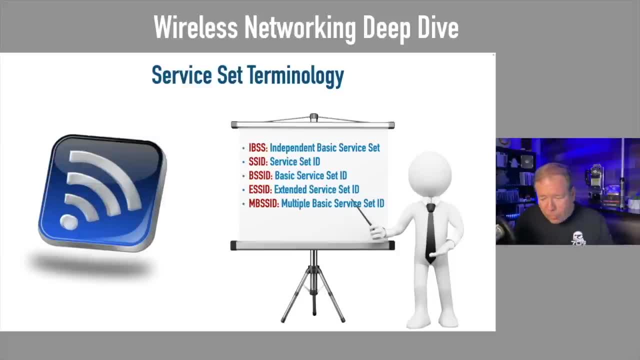 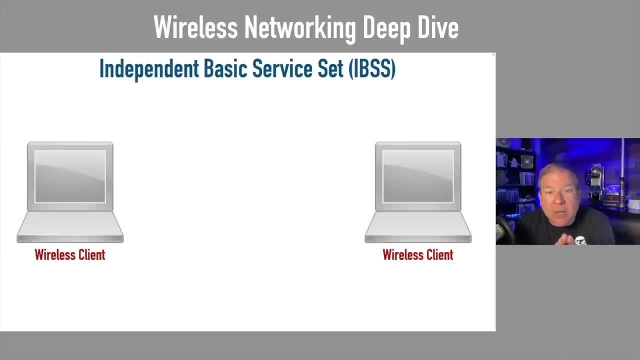 These are the ones that we're about to talk about. All right, Let's get into it. The first one is what we talked about earlier. We talked about an ad hoc network where I've got these two phones and they're just talking directly to each other. 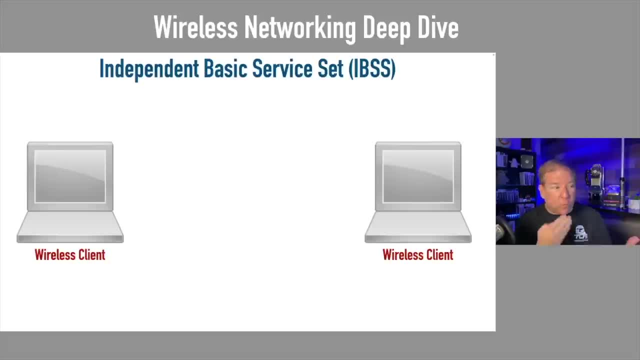 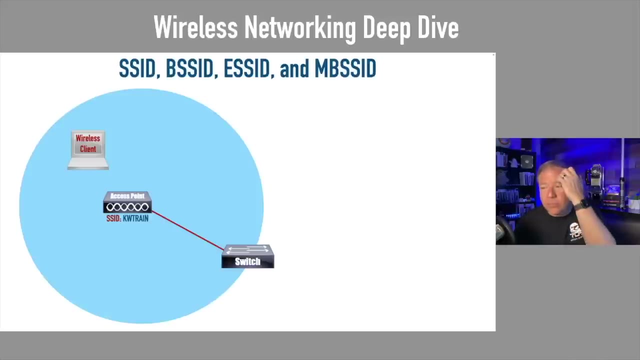 There's no infrastructure, There's no access point, They're just going from one device to the other device. That is called an independent basic service set, No infrastructure. So it's an IBSS independent basic service set. And oh, somebody's saying you can get free ESXi host-only license if you register on VMware. 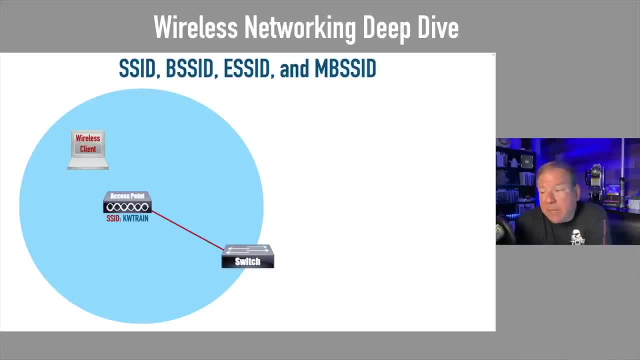 Yeah, In fact, ESXi, you don't get support. Shane's talking about getting a free copy. They don't give you support for a free copy, but they give you a licensed copy. No kidding, In fact I've got a YouTube video, If you want to just search for on YouTube. 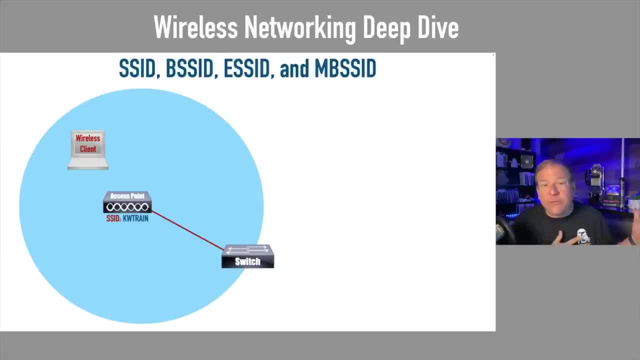 search for Kevin Wallace ESXi. I've got a full video showing you how to go out and get a free, licensed copy from VMware. Again, there are some limitations- They don't give you support, but it's free and you can get the 60-day eval for free. So yeah, if you've got the machine to. 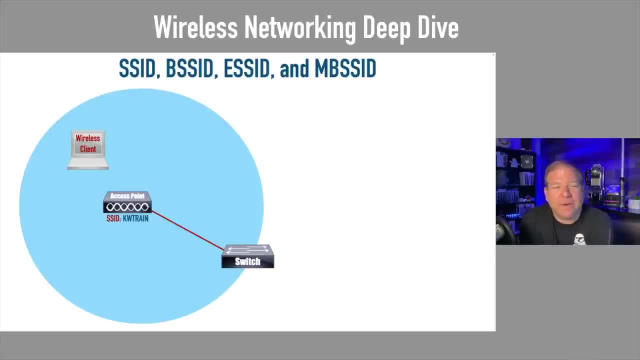 run it on. yeah, that's pretty amazing. But back to our story here. When I say that I'm advertising network name, that's the SSID. So let's say that I've got an SSID of KW Train, That's my network. 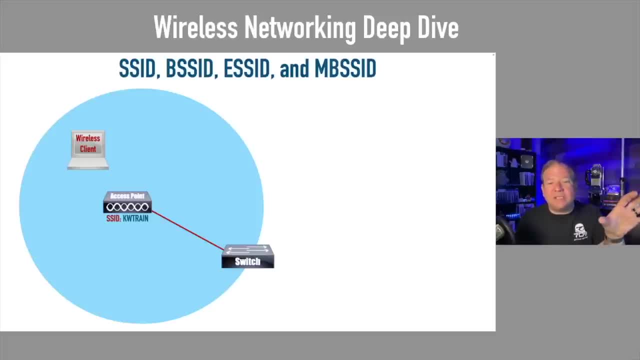 that I'm joining And I'm this wireless client and I'm connected to this access point, But then I decide to roam. My SSID that I'm connected to is KW Train, But now I need to roam over to this other area, to this other access point, But it's also advertising KW Train as the SSID. Well, 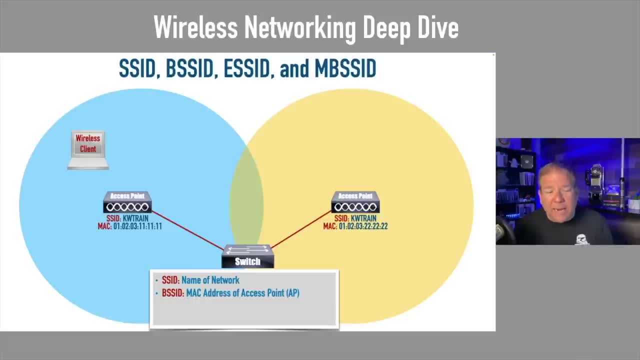 when I do that. when I do that, I'm staying on the same SSID, but how, in the background, am I talking to a different access point? How do I know which access point I'm talking to? Because each access point has a. 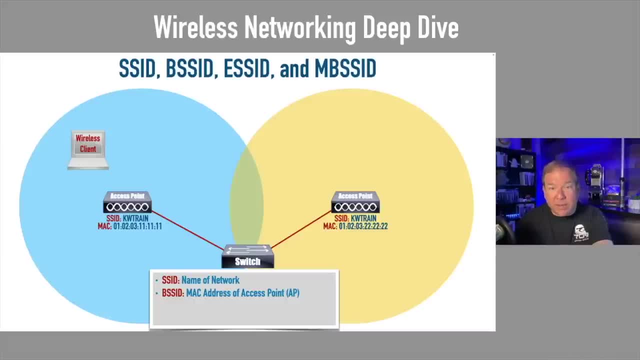 different MAC address, just like your computer has a unique MAC media access control address. When I move over there, I'm talking to the same network of the same SSID, but I'm talking to a different MAC address. That MAC address is called the BSSID, the Basic Service Set Identifier. So 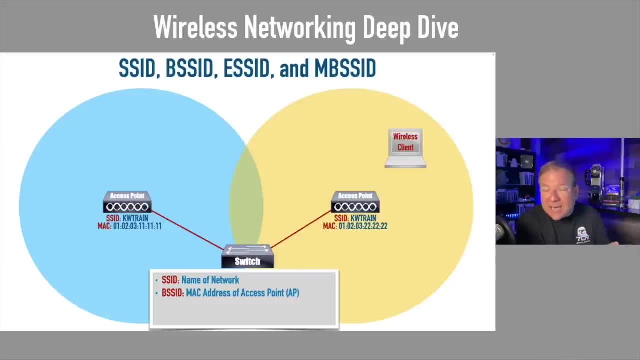 for your notes. I want you to know that the BSSID, that's the MAC address of an access point. I also want you to know the term, even though I rarely, if ever, use it. In fact, the only time I 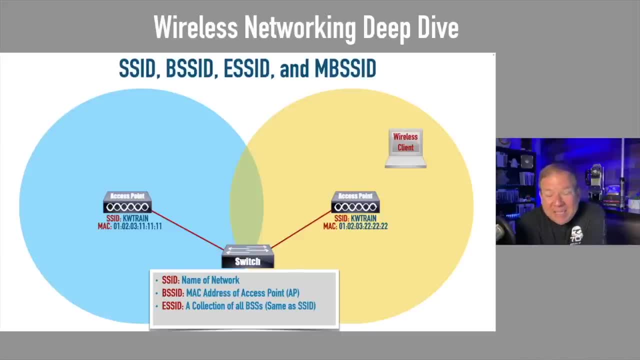 use. this is when I'm teaching. it is an ESSID. Honestly, I wish this term didn't exist. It stands for the Extended Service Set Identifier and it is a collection. It says this includes all of the access points, all of the BSSIDs that are advertising the same network, that are advertising the same SSID. 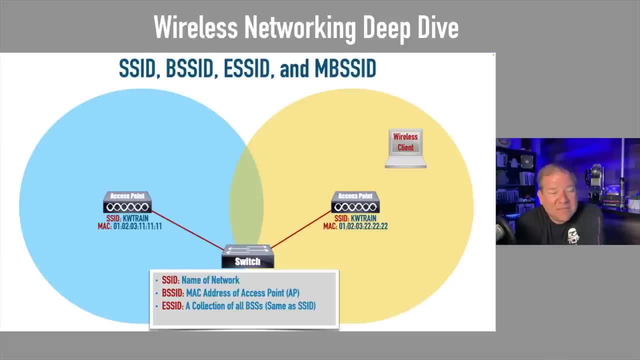 So what is the ESSID of this network, KWTrain? It's the same thing as your SSID. We don't need two different acronyms to talk about the same thing. So in the real world, I never use the term ESSID because it is the same thing. 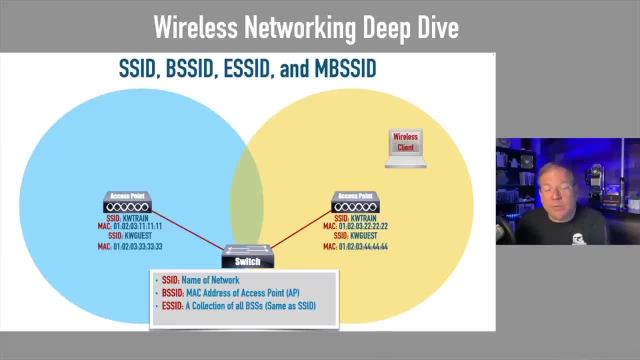 It's just an SSID. There is one other term I want you to know, though, and that's, if I have more than one SSID, that I'm advertising from an access point. So maybe this access point is not just advertising the KWTrain wireless network. I've got a KWGuest network as well. 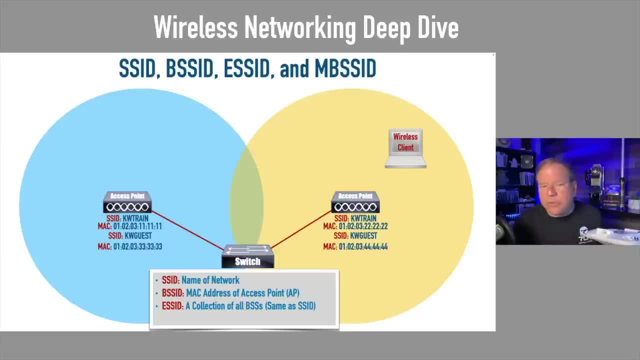 that might be limited in terms of security and bandwidth usage, but I'm advertising both of these networks. How does that work? Well, each SSID has its own MAC address. So each SSID that I'm advertising, they each have their own BSSID, They have their own MAC address. But if I have an access point, 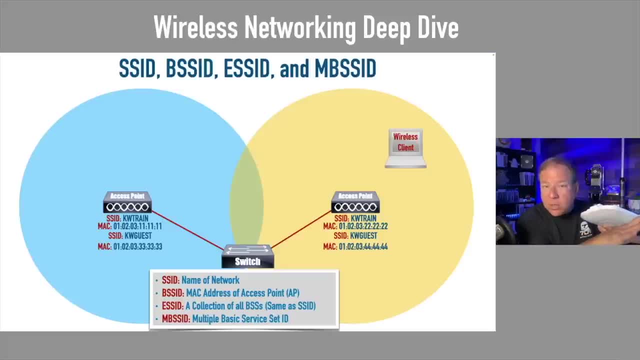 that is advertising more than one wireless network. that's called an MBSSID- multiple basic service set ID, because I've got more than one MAC address. So I've got multiple BSSIDs because that's the MAC address. So those are just some terms that I need you to know for. 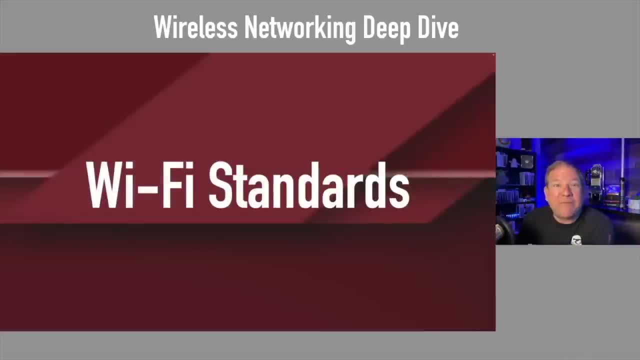 the CCNA exam. And next up we're going to talk about one of my favorite topics today and that is some of the different wireless standards that are out there. When I first was exposed to wireless networking, it was back- wow, I don't even know- probably back in around 90,, I don't know late. 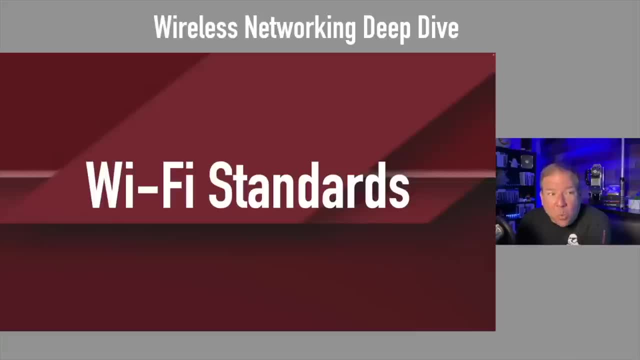 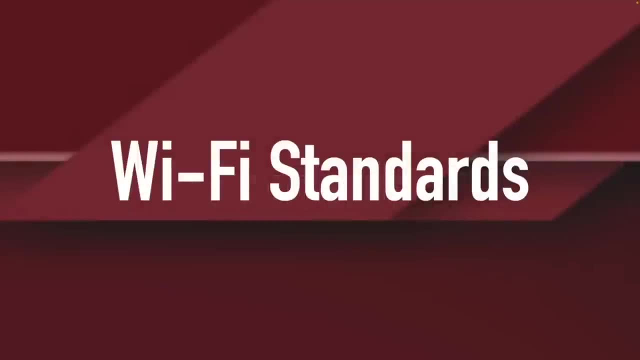 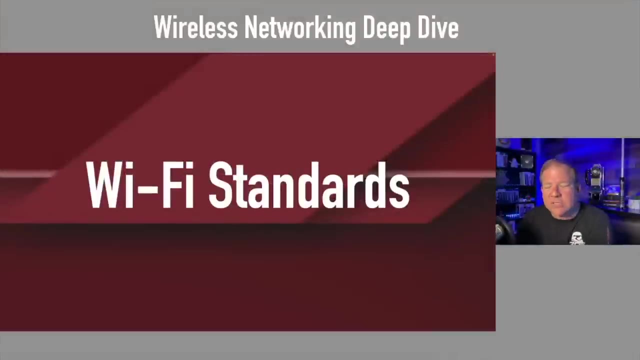 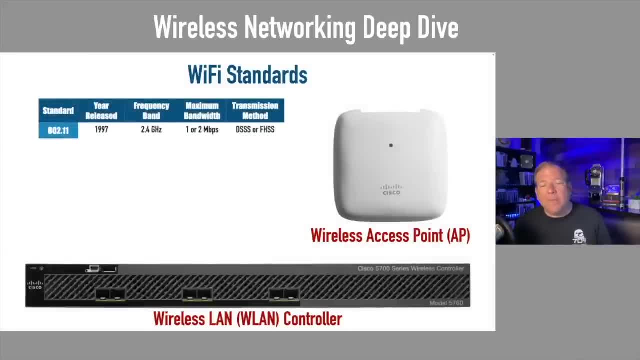 of the different wireless standards and how they have evolved over time. But back in 1997, that's about the time I first came in contact with this- Yeah, it only. it was .11, and it only ran at like one or two megabits per second. I remember going into. we went into a library at a university. 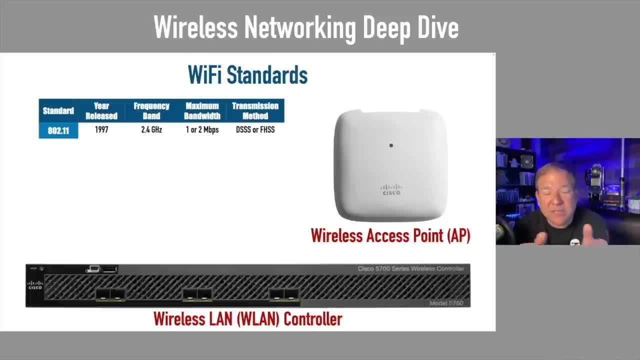 and we were discussing giving wireless coverage throughout the library. where students could like it was at a university library. They could rent a laptop and then go somewhere and they would have access. But I remember being disappointed that it was only running at like one or two meg. 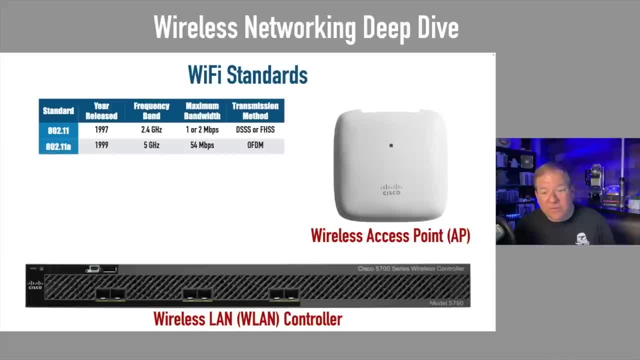 And yeah, not great. It evolved to .11a and .11b in 1999.. Notice: .11b used 2.4 gig, .11a used 5 gigahertz band .11b was a lot more popular, If you remember back in the day. 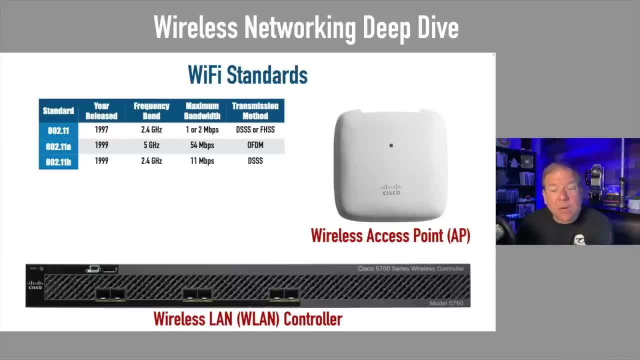 it wasn't as much throughput. .11b only gave us 11 megabits per second. .11a gave us 54 meg. That sounded pretty good. Now notice some of the transmission methods. here We're going to be talking about those. And we have DSSS, that's direct sequence spread spectrum. 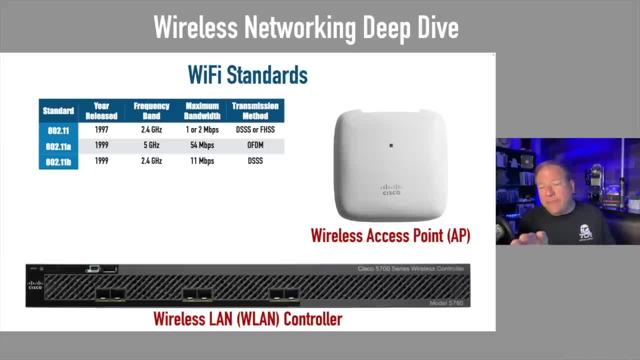 I'm going to describe that one to you in a few moments. And then we have frequency hopping, spread spectrum. The basic difference between those is: direct sequence is I'm using different carrier frequencies but they're in a direct sequence with one another. Frequency hopping is I'm going. 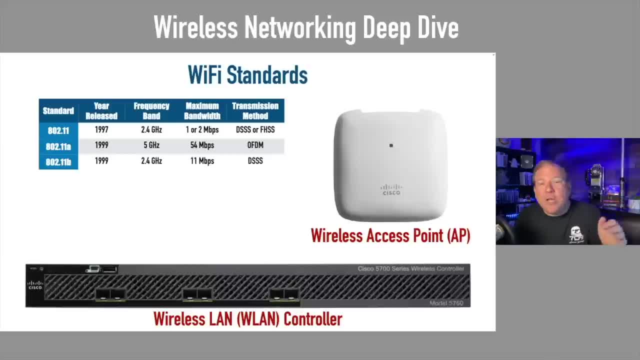 to jump from this carrier frequency to this one and back to this one and this one. You're not going to be able to predict it. Only the sender and receiver knows which frequency we're going to be using next. So it adds a layer of security. That's the difference between direct sequence and 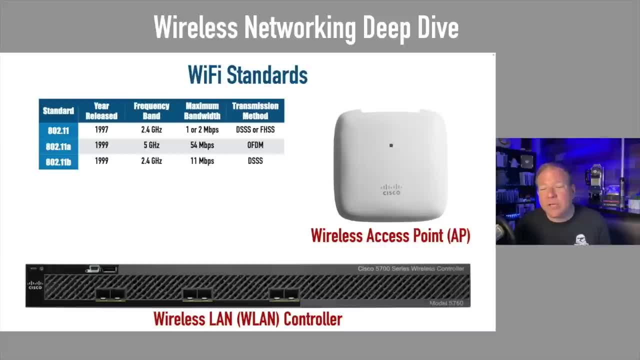 frequency hopping spread spectrum. We also have OFDM, Orthogonal Frequency Division Multiplexing. We'll talk about that. And then .11g. I remember being really excited when that one came out because it used 2.4 gig, which I was familiar with. 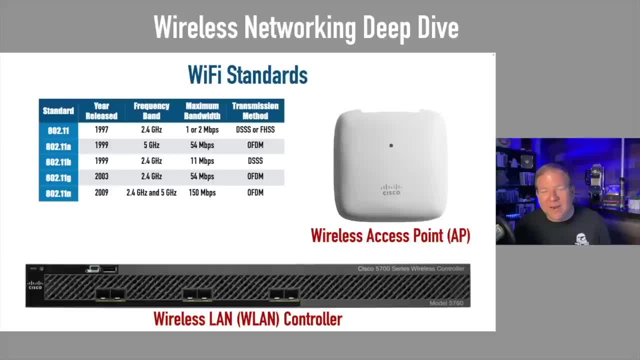 54 meg, Nice, nice. Then .11n came out. It could run both 2.4 or 5 gig and it gave us a whopping 115 megabits per second And it used orthogonal frequency, division multiplexing, And I thought. 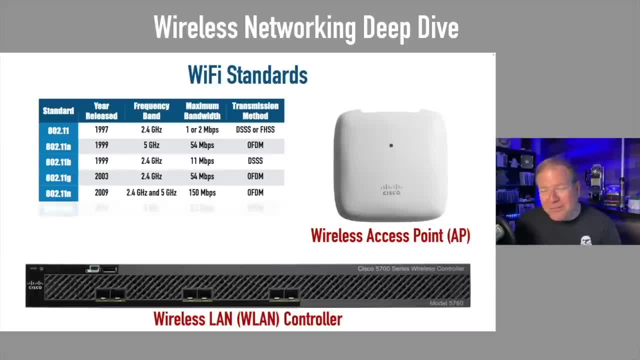 at the time I have no idea what that means, But it did, So we're going to talk about that. That means you're going to know here in just a few minutes, though, if you don't already: .11ac came out in 2014,. running at 5 gig. running at the 5 gigahertz band: 3.5 gig. 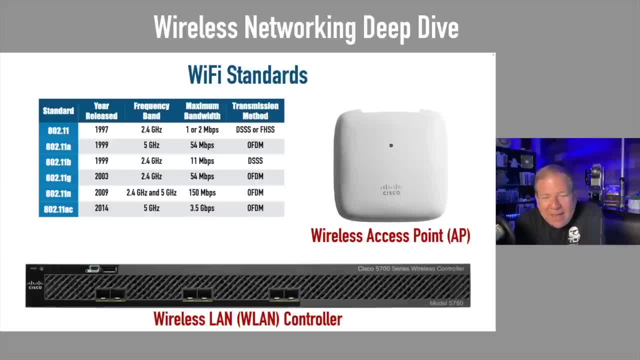 theoretical throughput. Wow, Yeah, It's at that point where your access points start to be, or rather your gig switches start to be your bottleneck. at that point, And then, more recently, just in 2019, .11ax, also known as Wi-Fi 6, came out. Again, theoretical throughput, I've 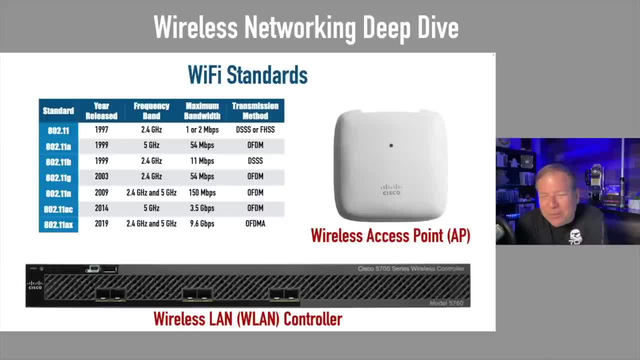 personally never approached a 9.6 gig, but theoretical. if you include all the different flows coming in at one time, it adds up to, theoretically, 9.6 gig of throughput. That's wild. The transmission method is different than anybody else. It's not OFDM, It's not orthogonal. 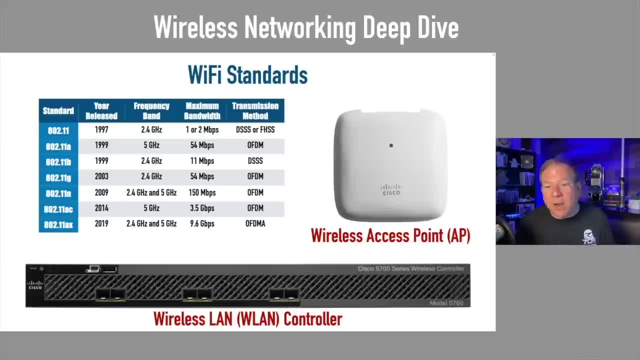 frequency division multiplex. It's OFDMA orthogonal frequency division, multiple access. You're going to learn, if you don't already know, what that means in just a few minutes. Now we're not going to get into Wi-Fi 6E very much because it's not on the exams. It's a much more recent development. just 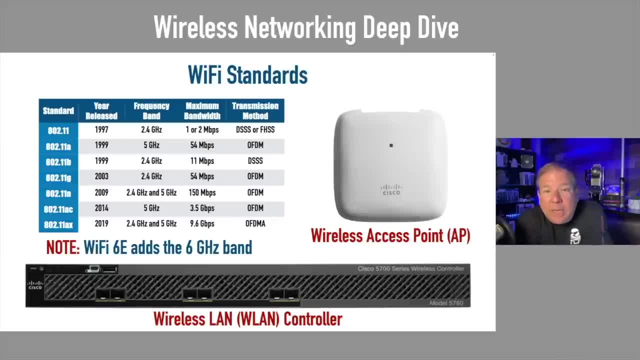 in the last few months. But basically what it does? it opened up a band that we were not allowed, or the companies were not allowed, to use prior to this, the 6 gig band, And when we talk about channel widths a little bit later, we can have seven additional non-overlapping. 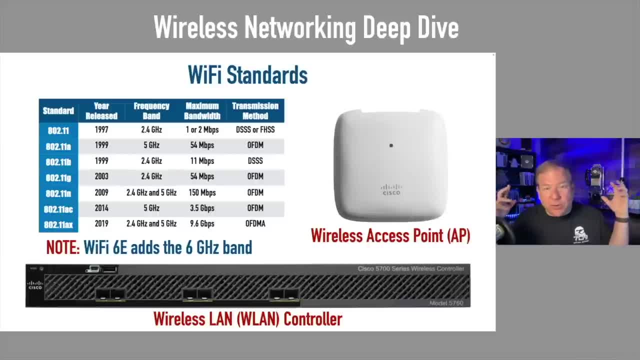 channels and those channel widths are huge. They're 160 megahertz. more on that later. But yeah, Wi-Fi 6E, it's just going to be an add-on to Wi-Fi 6 to give us even more channels if we 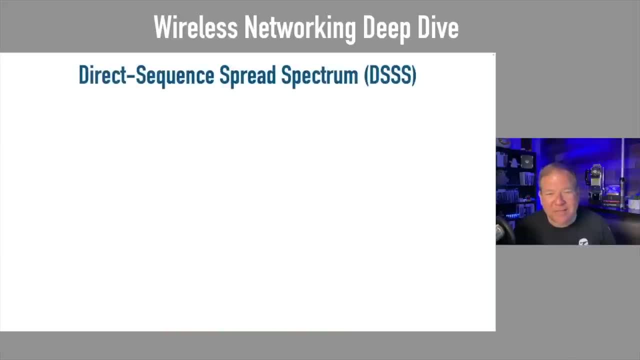 need those, But not on the exam, so we're not really going to focus on that one. Now let's go back in time to .11b and talk about direct sequence. So we're going to talk about direct sequence, spread spectrum or DSSS. The idea is we can send 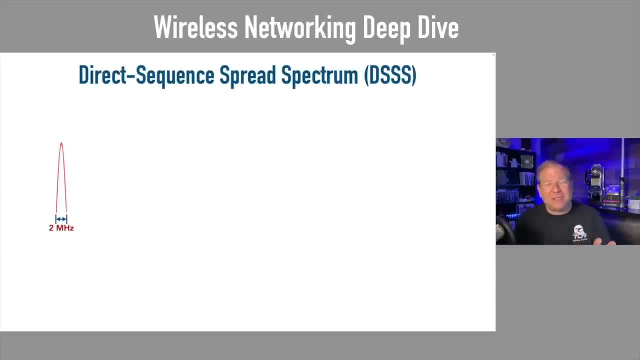 one. please follow me on this. This is going to be a lot of information. I'm going to try to take it slow. I might repeat a few things so you get it. Please take some notes on this. This is key stuff to understand, to really understand how wireless works. It's one of the most important. 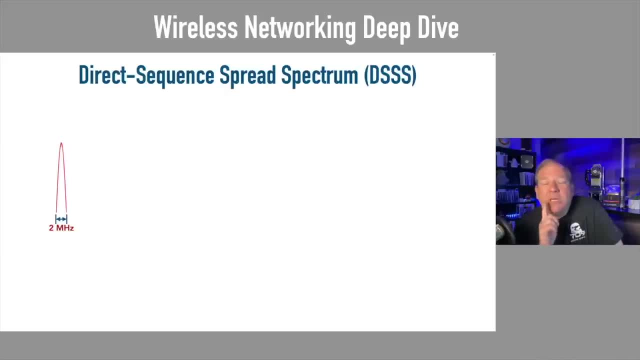 topics we'll get on today, But you can send one bit of data using two megahertz of a frequency range. That's a lot of data. So you can send one bit of data using two megahertz of a frequency range. It's not much, two megahertz. Remember earlier, somebody type it in When we talked. 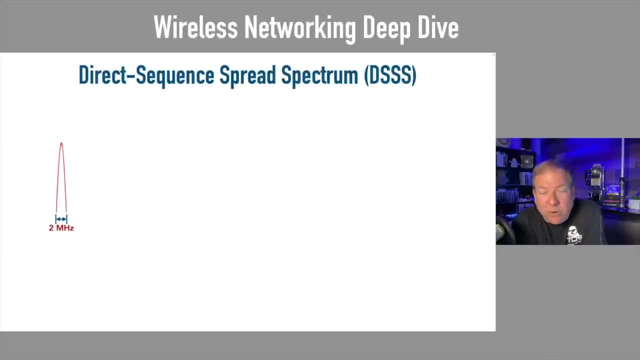 about those 2.4 gig channels. I said we should use channels 1,, 6, and 11.. Who remembers Chat it in if you would? What range of frequencies did that? or I should say what was the channel width. 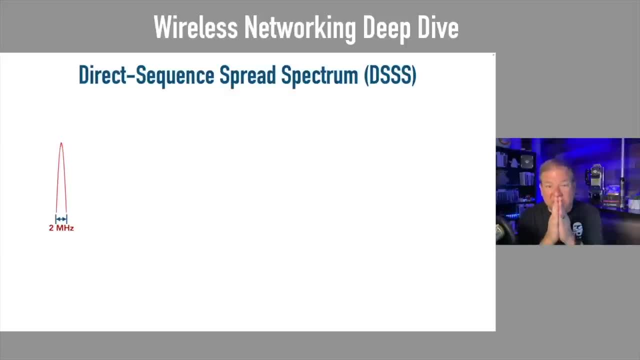 of channel 6?? We said channel 6 was the center frequency but it extended a little bit. What was the channel width of channel 6, or channel 1, or channel 11?? Do you remember? Go ahead and chat that. 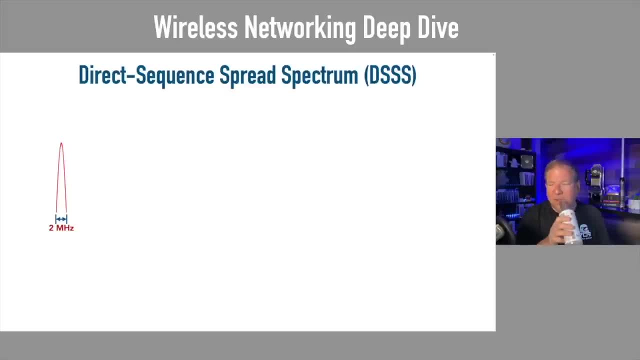 in. Somebody says: what is the max throughput I've seen in Wi-Fi 6?? I'm trying to remember. Last time I used Wi-Fi 6 was about two or three months- I honestly don't remember, but I remember I was disappointed 22, yeah. Somebody says their tagline is: 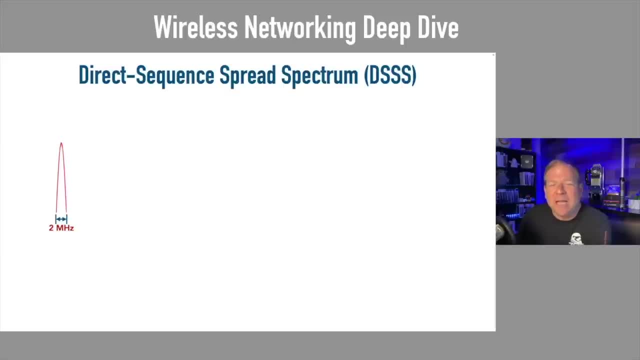 I may roam, but yeah, it's saying 22 megahertz. Danny says 22 megahertz. Yeah, it's 22 megahertz. If I've got a two megahertz sub-channel, we'll call it. how many of those two megahertz little sub-channels can I have? 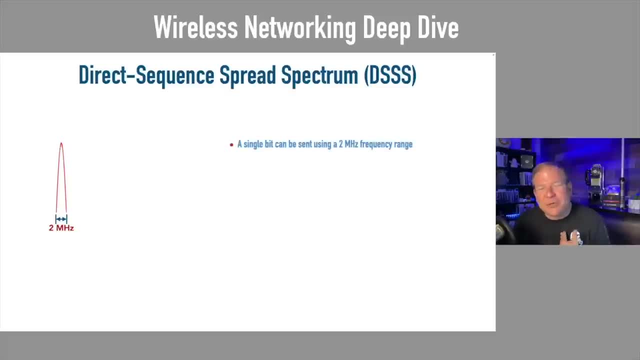 that can represent bits of data. Well, if I've got 22 megahertz to play with, that sounds like 11 bits of data that I can send, but back in .11b. this is going to blow your mind- Back in .11b. 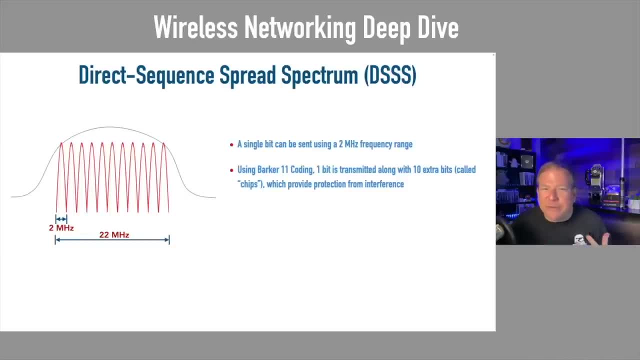 there was such a concern about interference and data corruption that, even though we could send 11 bits of data, we sent one bit of data and then 10 bits called chips. That was meant for error detection and correction. So this is called Barker 11 encoding. We've got eight bits or 11 bits. 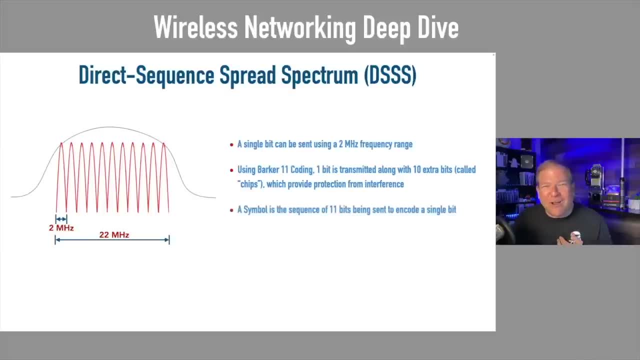 being sent, but only one was data. The rest were for error detection and correction. So that's not super efficient, is it? Maybe that's why we only got 11 megabits per second of throughput with that, but that's what we used for years with .11b. Let's go forward in time a little bit to FDM. 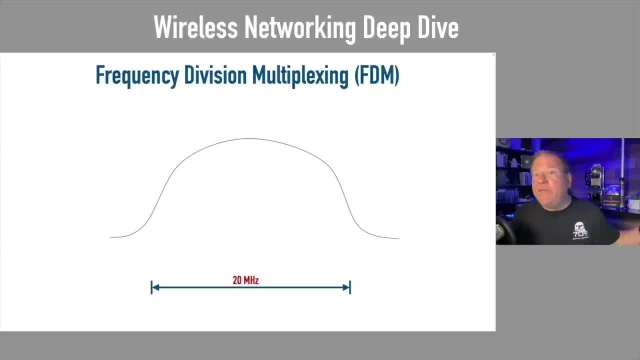 frequency division multiplexing Here. we don't even bother saying: yeah, I know it's a 22 megahertz channel width, but it's not. We don't even bother saying, yeah, I know, it's a 22 megahertz channel. 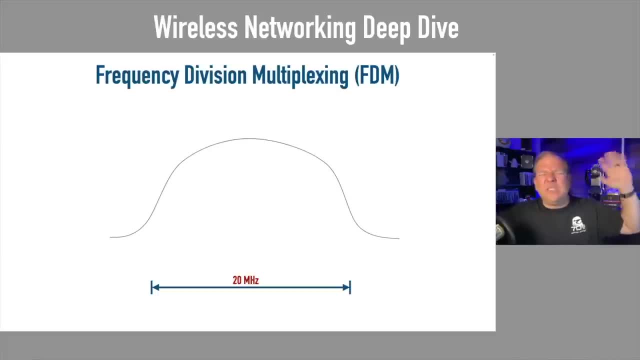 width. but it's not. We don't even bother saying: yeah, I know it's a 22 megahertz channel width. I mean it's kind of low on those end points. Let's just use 20.. Let's round down to 20.. 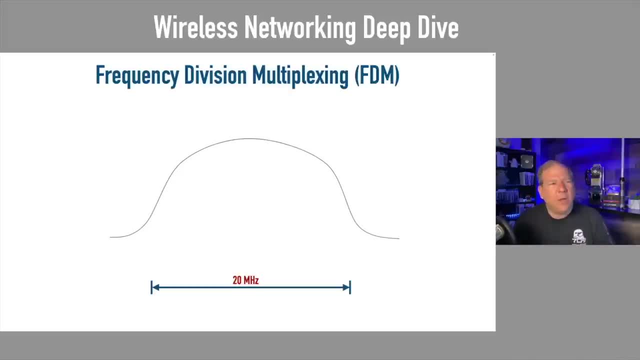 So now, if I'm using a 20 megahertz channel width, how many of those little two megahertz subchannels do I have? 10.. So I could send 10 different bits, And here we're not really concerned with all the. 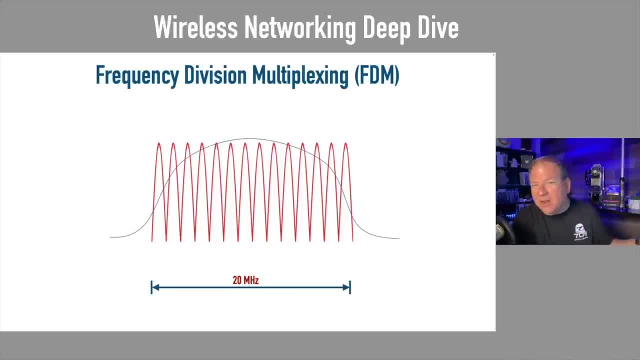 error correction and detection. I, mean times, have changed The silicon's much better. We want to send maybe 10 separate conversations. We don't want to send 10 separate conversations, We want to one on each of these subchannels. The challenge is those subchannels they could interfere with. 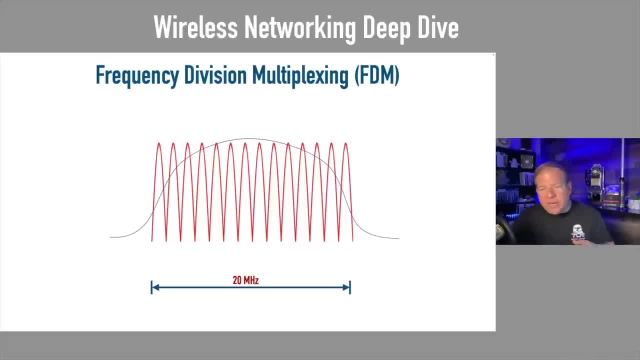 one another a little bit Now. I know, looking at the screen it's like you've got two megahertz. two megahertz, They don't overlap, They're next to each other. but they don't overlap. But come on, I mean they're right next to each other. There's going to be some. 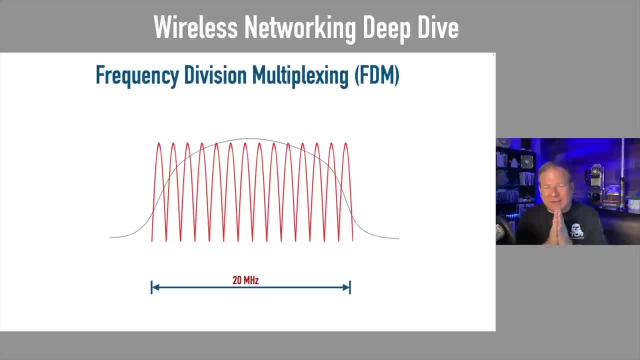 interference if we just stick them all side by side like that. That's where orthogonal frequency division multiplexing comes in. So many people miss this concept. I mentioned earlier that orthogonal means at right angles to at 90 degree angles. I said if my arm is like this and my other arm is like, 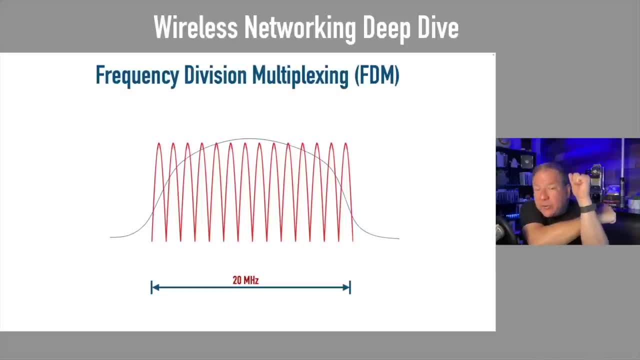 this. my arms are orthogonal. They're at 90 degree angles to each other. Now a lot of people misinterpret this. They say: oh well, one subchannel is going up, like the E field, and the other one's going back and forth, like the M field. That's a good theory. 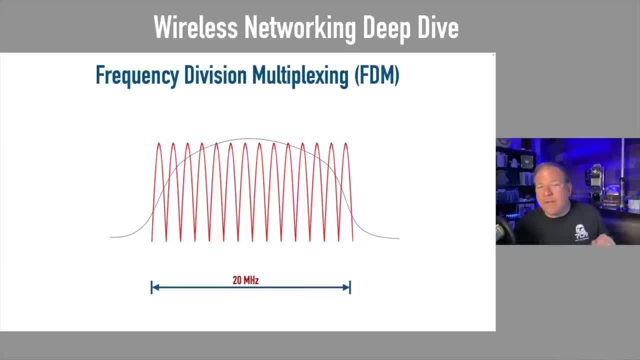 but that's not what it means. They're not physically at 90 degrees. Do you remember trigonometry in high school or college? Somebody tell me. Well, we talked about it earlier. I showed you a sine wave. We said that was one cycle. Somebody chatted: in How many degrees? 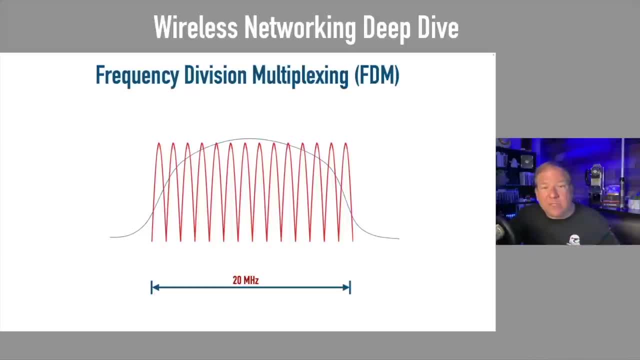 do we have in a full wavelength of a sine wave? How many degrees do we have in a full wavelength of a sine wave? How many degrees We go up, we go back to zero, we go down, we come back up to zero. 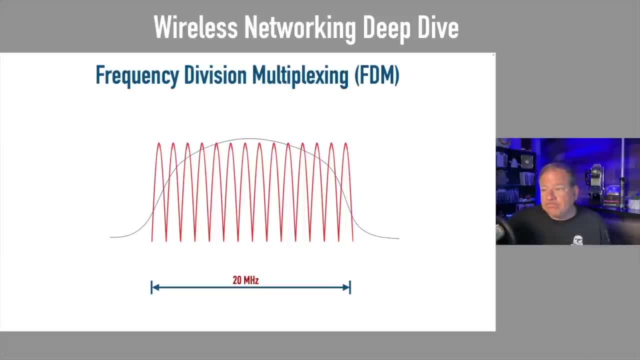 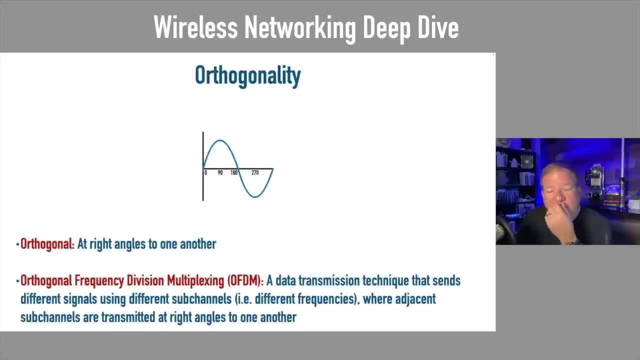 How many degrees is that? Yeah, it's just like a circle, It's 360 degrees. So in trigonometry we learned that this sine wave, like you see on screen, that represents 360 degrees. When we reach that first peak, that's 90 degrees. When we come back, 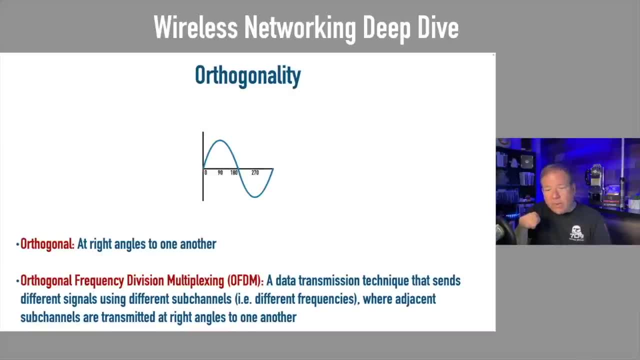 to zero, that's 180.. When we come down to the bottom, that's 270.. We come back up to zero, that's 360 degrees. That's a sine wave. Do you remember what a cosine wave is? A cosine wave looks like this, this red line on screen. 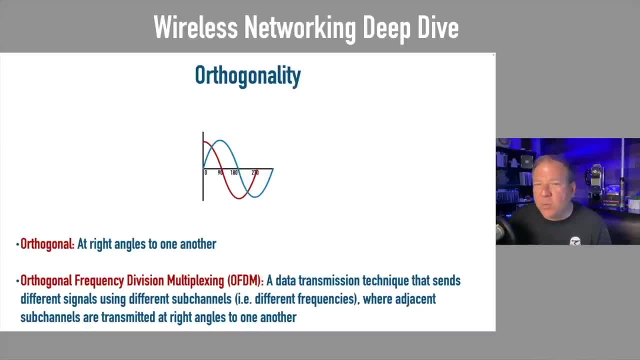 Follow me here. The difference between a sine wave and a cosine wave is they're phase shifted 90 degrees. You see where I'm going with this. This sine wave and this cosine wave, they're 90 degrees apart from each other. They're not physically one up and one sideways. 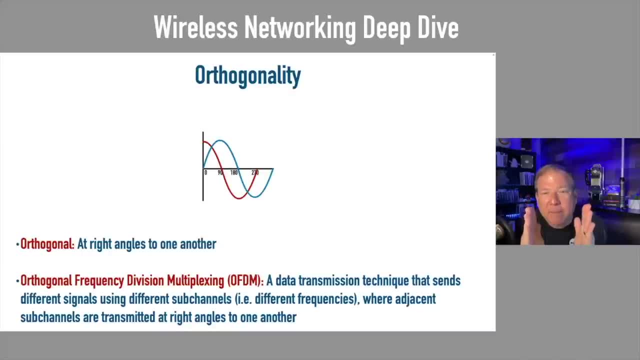 but they're phase shifted 90 degrees. That means they are orthogonal to one another. Why do we care? Notice the graph: When we're at zero degrees, we're at peak power of the sine wave, Or, excuse me, the cosine wave which is red. Where's the sine wave Zero? So when we're sending, 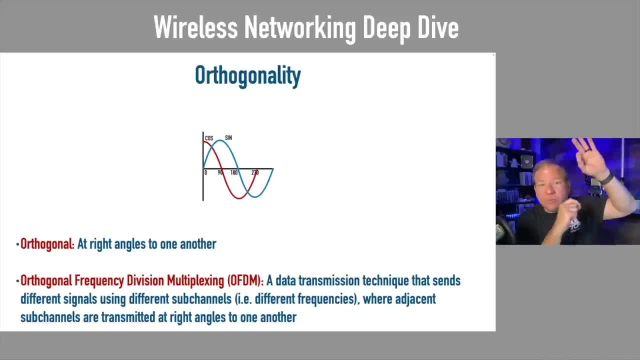 peak power for one wave, there's going to be zero interference from the other way because its power is zero. When I'm at peak power for the sine wave at 90 degrees, what's the power of the cosine wave? Zero. You see, when one wave is peaking, the other is at zero. That gets rid of the interference. 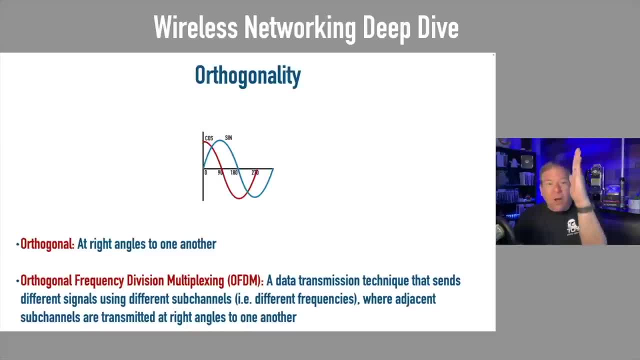 friends. That's why we say they're orthogonal. They're not up and sideways, they're shifted 90 degrees. That is the magic of orthogonal frequency division multiplexing. So now we can have two megahertz, two megahertz, two megahertz each sending ones and zeros. 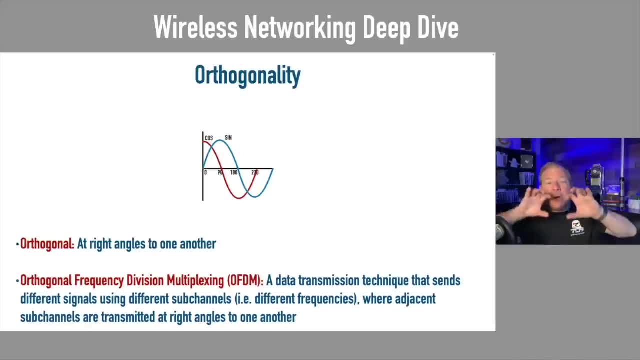 ones and zeros, and they're not going to interfere with one another because of the phase shift. So that's going to get us much higher throughput than 11 megabits per second that we had with direct sequence spread spectrum. Let's take it a step further. 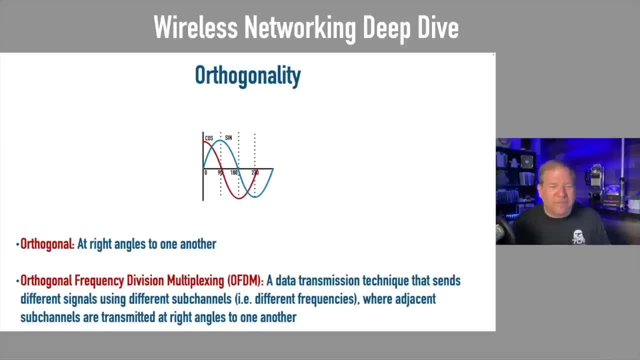 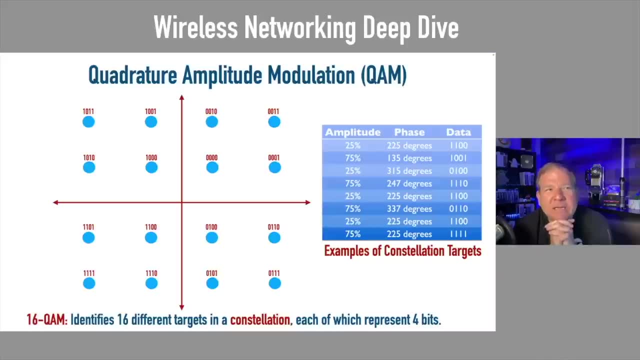 This is where it gets really cool. Let's talk about QAM- quadrature amplitude modulation. As a metaphor, you might've seen I posted this yesterday, I think, or the day before. I posted a picture of a dartboard and I said quadrature amplitude modulation, or QAM. 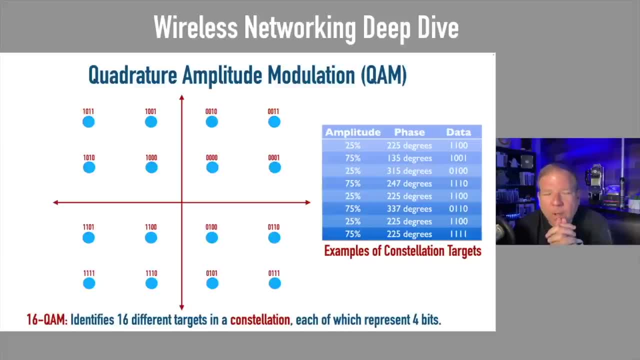 that's a lot like throwing darts at a dartboard, Because I've got this two megahertz channel width And I said it could send a single binary, one or a zero. Okay, What if? what if I could take that two megahertz channel width and, instead of sending 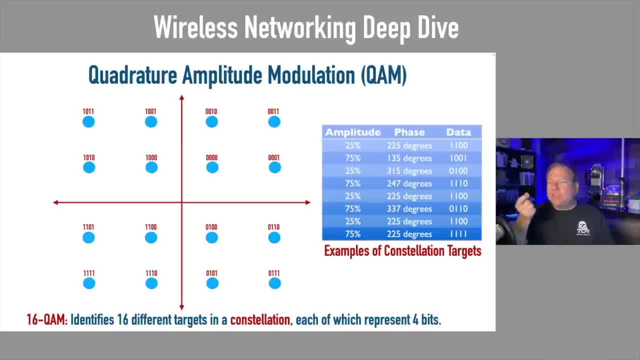 a single one or a zero? what if I, just like I, was throwing a dart at a dartboard? what if I could use that two megahertz wave and pinpoint one of these dots on screen? If I pinpointed that dot up in the upper, if I threw my dart and hit that dot in, 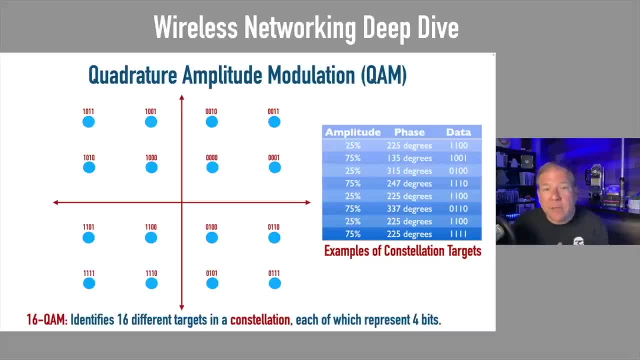 the upper left-hand corner. instead of representing one bit, it would represent four bits. If I could hit that dot in the upper or, excuse me, upper left-hand corner, that would be a one zero one one. So instead of sending one bit, I just sent, I just transmitted four bits. 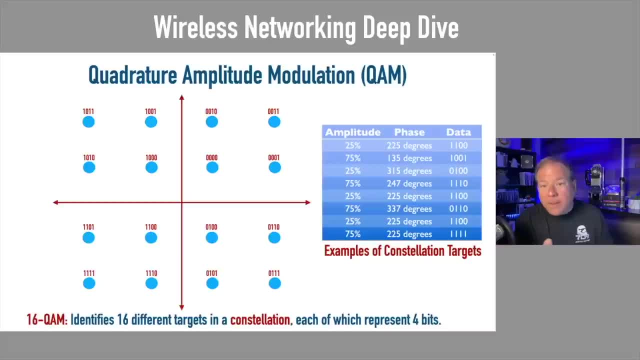 Now here. just to keep it simple, this is called 16 QAM because I just didn't want to draw like a thousand dots on screen. It's going to be a lot easier to see like this. But the question is: how many binary bits does it take to represent 16 values? Four, two raised to the power of four is 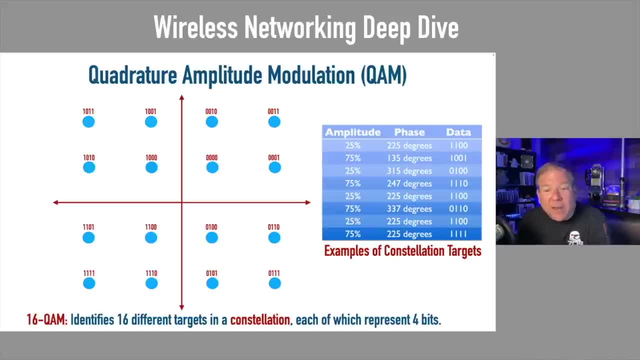 16.. So I've got 16 dots on screen and they each represent a different four bit pattern. So if I hit this dot, it means these four bits. If I hit the southern dot, it means these four binary values. The question is, I've got two megahertz. How do I, how do I, throw a dart and hit one of? 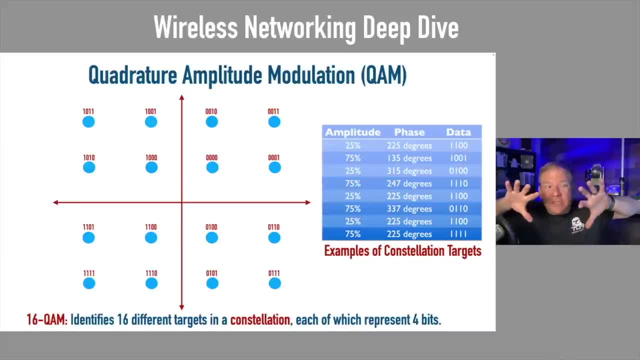 these dots And, by the way, this, this series of dots. we start to get more and more and more dots the more data we're carrying And it turns into what looks a lot like a star field. In fact, it's actually called a constellation. The question is: how do I hit a dot? 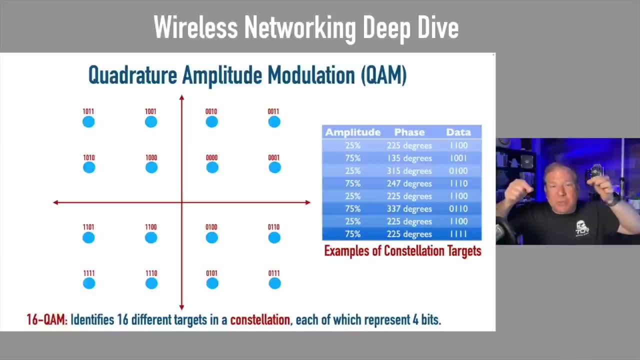 Well, there are a couple of things that I can, that I can adjust with my waveform. I can. I can pump up the volume or I can turn down the volume. I'm adjusting the amplitude. In other words, I can also- just like we talked about phase shifting- I can shift its phase, a certain 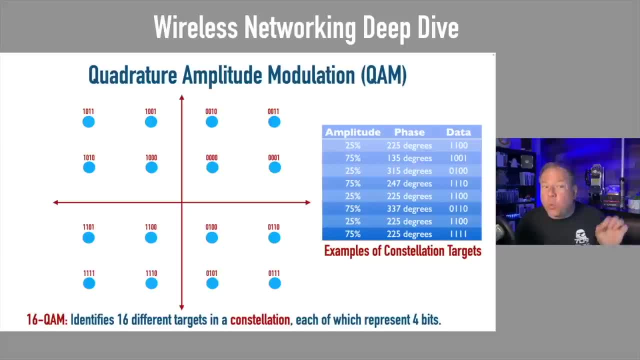 amount. So check this out. Let's say that I sent a waveform and I decreased the volume to 25% and I phase shifted it 225 degrees. When I do that- and this is just a partial table- When I do that, I hit one of those dots. 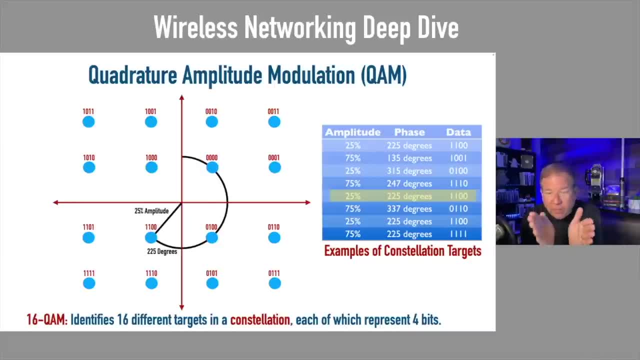 So with my two megahertz wavelength or bandwidth, I just represented four bits. I represented one, one, zero, zero. because I adjusted my amplitude, I adjusted my phase, bam, I hit a dot and it represented four bits. That's the magic of quadrature amplitude modulation. Now those of 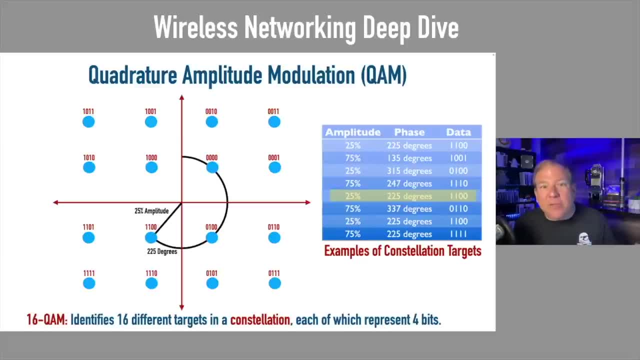 you that have really gotten into this instead of this. yes, I admit there's a lot of math behind the scenes. We don't need to know that. For those of you that are curious, here's what's going on In the background. I'll try to make this super simple. There's actually two waves that get. 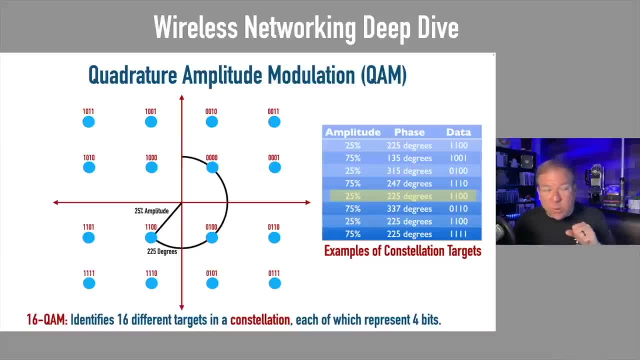 combined. There's the um, there's the in phase wave, That's like the baseline. Uh, I'm telling you way more than you need for the exam. but I've taught this class before and I get some people invariably that are really into all this stuff and they try to correct me and say: well, actually, 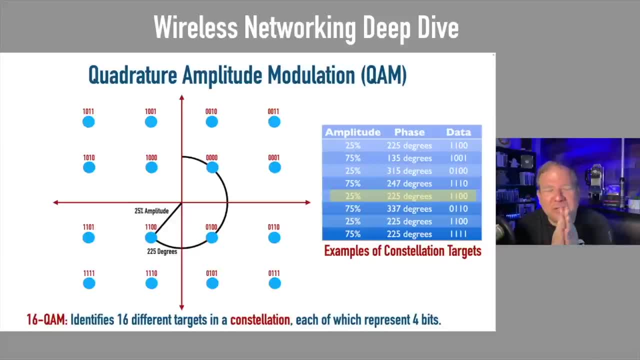 there's a Q wave and there's an I wave. Okay, Here's the simplified version of that. There's a reference wave called the I wave or the in phase wave, because if I'm sending a wave, I'm sending something at a different volume and a different phase. I got to have something to. 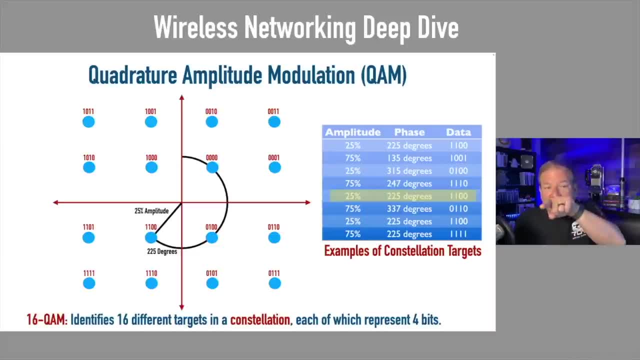 compare it to. So I've got the I wave, the in phase wave, and then I've got the Q wave, the quadrature wave, that is, phase shifted, with the amplitude changed, And by comparing those two, that's how I'm hitting the dot. Now, when you superimpose those two waves on top of each other, 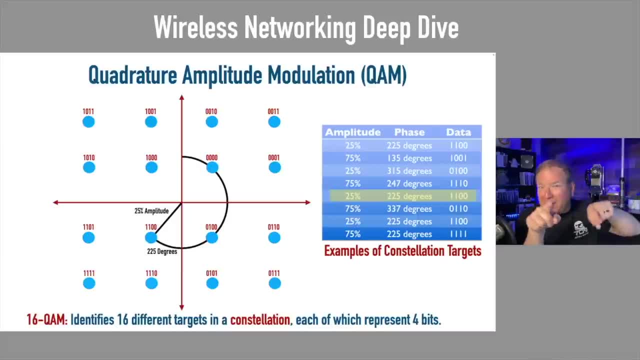 the I wave and the Q wave. you get kind of a funky looking wave, but you can still do that in this two megahertz bandwidth. Now how do you separate those out to know what the phase and the amplitude is Super mathematical? here It uses something called an FFT, a fast Fourier transform. 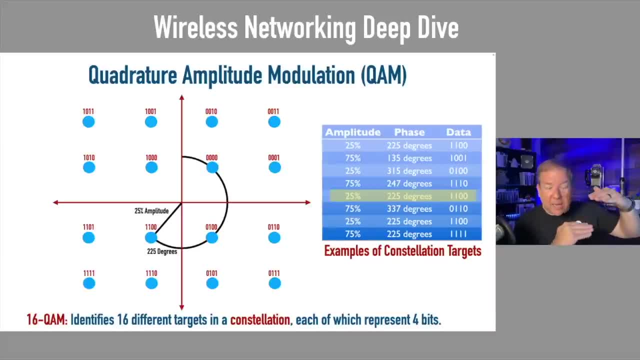 A fast Fourier transform is able to take a composite waveform and extract the individual waveforms that made up the composite waveform, And by doing fast Fourier transforms you're able to determine: oh, it was phase shifted this much And the amplitude was decreased by this much. Let's look it up at the table. Oh, that's 1, 1, 0, 0. 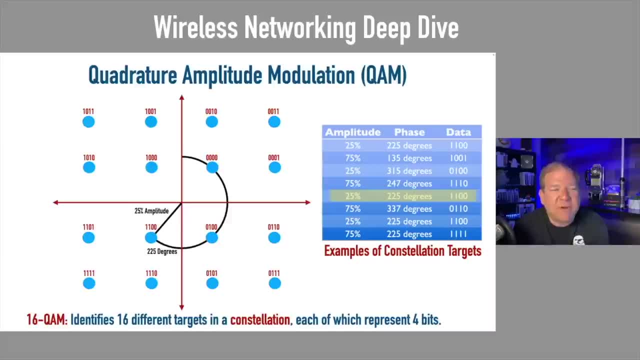 Again, more than you need to know for the exam, but I wanted you to have an appreciation for how that works, because it took me a long time to figure that one out, folks, So I wanted to simplify it as much as I could for you, But that's one way that we're getting these insane. 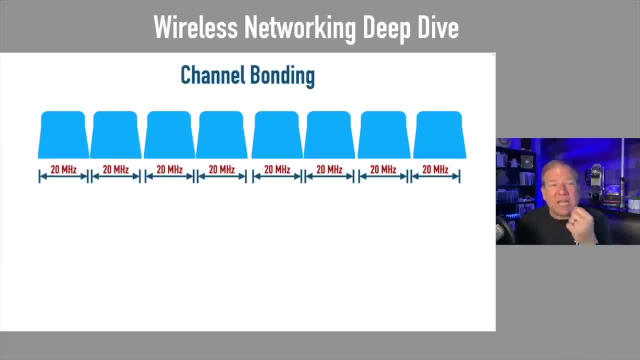 throughputs these days. Something else that will allow us to have more channels to be transmitting at the same time is, instead of taking just these 20 megahertz, we're going to take the 20 megahertz channels and dividing them into 10 subchannels. What if I took a couple of these 20? 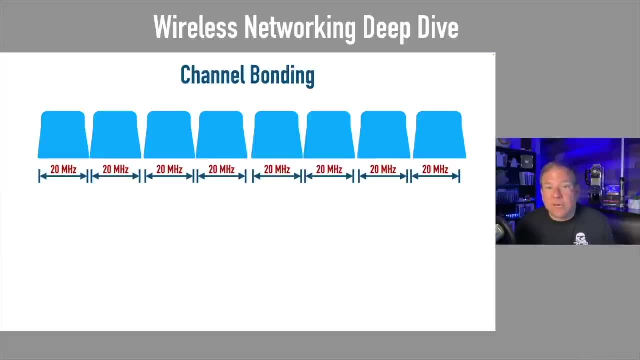 megahertz channels and I bonded them together. That's going to give me a 40 megahertz channel. That's going to allow me to send even more data at one time. What if I took four 20 megahertz channels? That's going to give me an 80 megahertz channel. I could even with some standards today. 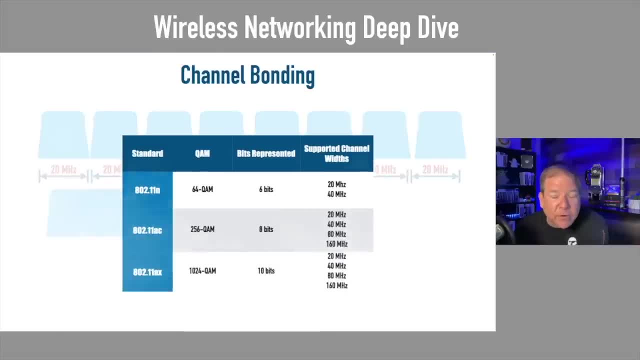 I could bond eight of these channels together to get a whopping 160 megahertz channel. Now here's a reference for you. We talked about QAM. I showed you QAM 16.. I said, if I had 16 dots in my constellation. 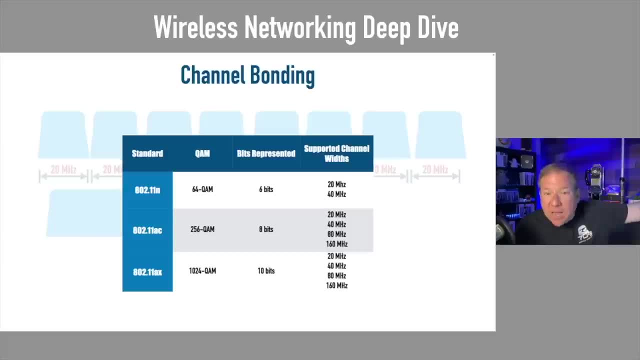 I could represent four bits. Well, back in 2009, 802.11n, it used 64 QAM. How many bits represent 64 different dots? Six bits, So you hit one dot. This is 13 years ago. we could do this. 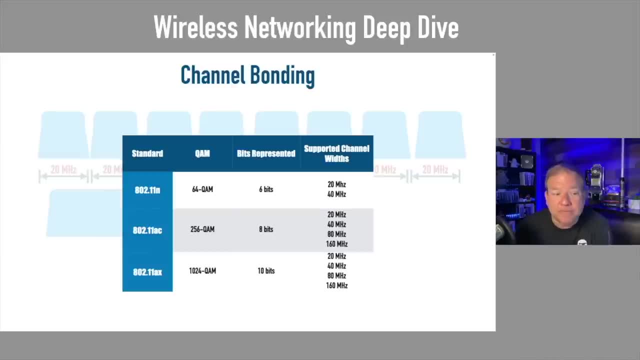 You hit one dot. that one dot would represent six bits. As the silicon, the manufacturing got more and more. I guess manufactured to higher tolerances would be the way to say that We could be more and more accurate. And then we came out with .11ac That used 256 QAM. 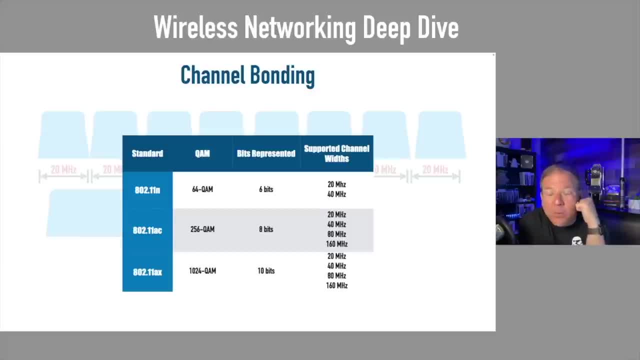 where you hit one dot, that would represent not one bit, it would represent eight bits. And now with .11ax or Wi-Fi, 6, 1024 dots. That's right, You hit one dot and you just represented 10 bits. That's amazing. And you can have 160 megahertz channels, which means you can. 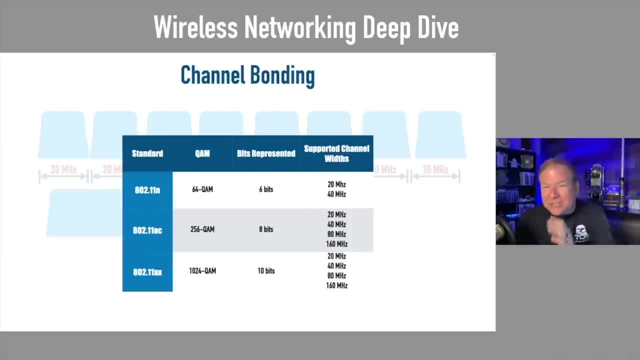 have 80 different communications channels going on there. This is how we're getting such incredible speeds. Now, just as a side note, don't need to know this for the exam, but I wanted to keep you up to date with what's going on in the real world. Recently, Wi-Fi 6E was introduced, which allows us 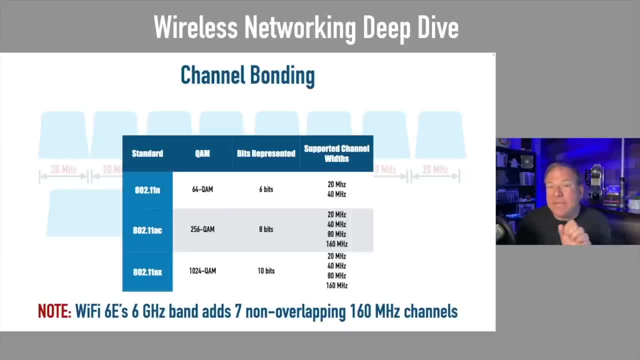 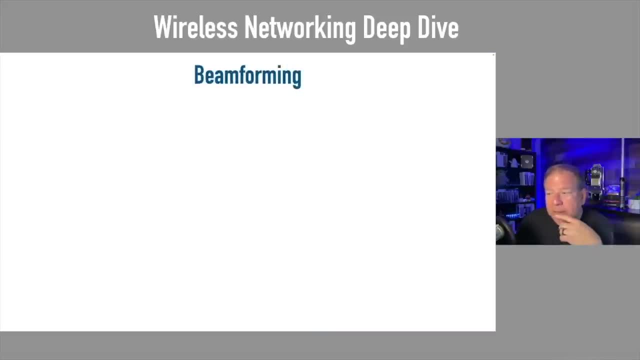 to use the six gigahertz band. That's going to give us seven additional non-overlapping 160 megahertz channels. Something else we can do to improve communication is to focus the transmission towards our device, So I've got my access point in my phone. I know we talked about 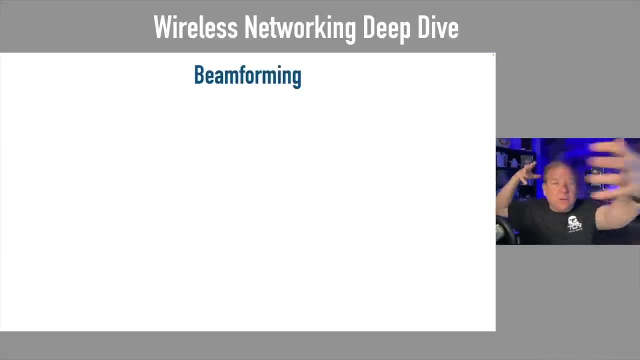 omnidirectional antennas and we said strength could go out equally in all directions. But if I'm talking to this phone, I'm going to be able to focus the transmission towards my device. I want to focus my energy just going to that phone. I don't want it to go out equally in all. 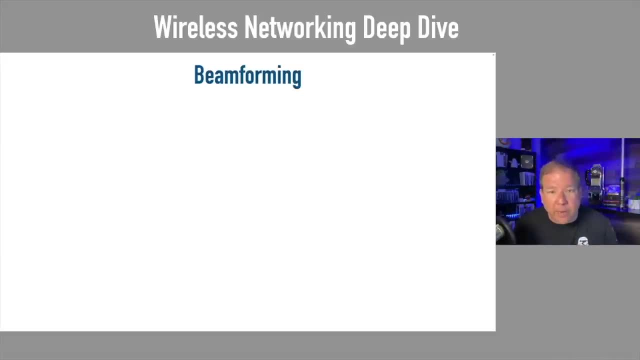 directions. How do I do that? We can do something called beamforming. With beamforming we can use constructive and destructive interference. Now think about this: If I've got a waveform and I've got an identical waveform and I superimpose those two waveforms on top of one, 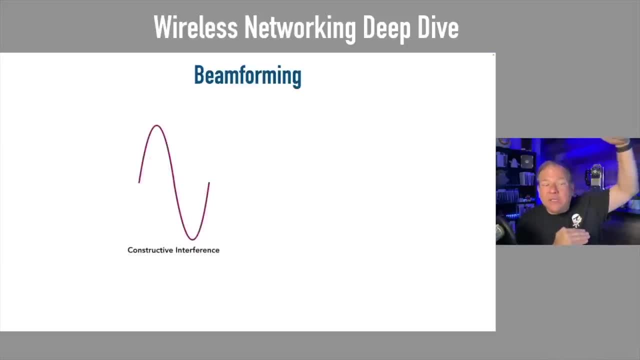 another. the result is they add up Suddenly. that's constructive interference. My amplitude is now twice what it was before. It works in the opposite direction as well. For example, here I've got my Apple iPods Pro. I put those in. They do noise cancellation. 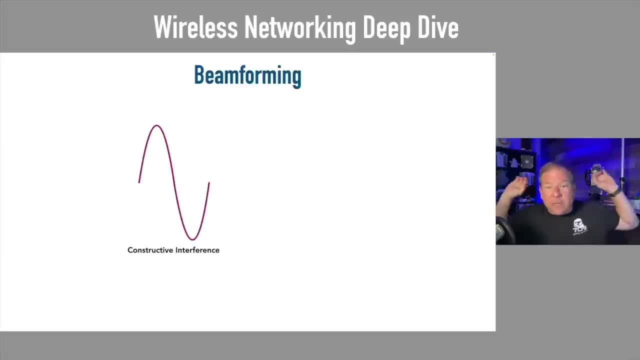 You know how they do noise cancellation. They have microphones that listen to the background noise- Like I'm going to get on a plane tomorrow and go to Disney World and I'm going to be wearing those guys- because those planes can be pretty loud- And it's going to listen to the 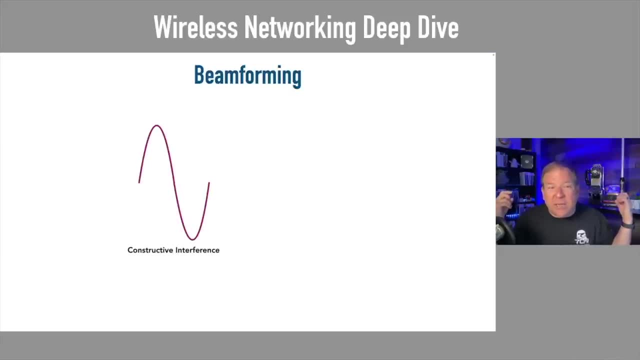 engine noise in the background and it's going to cancel most of it out by playing that engine noise, but it's going to phase shift that engine noise 180 degrees. So if you have two waveforms, one like this and you phase shift one 180 degrees, in other words it's the inverse image. 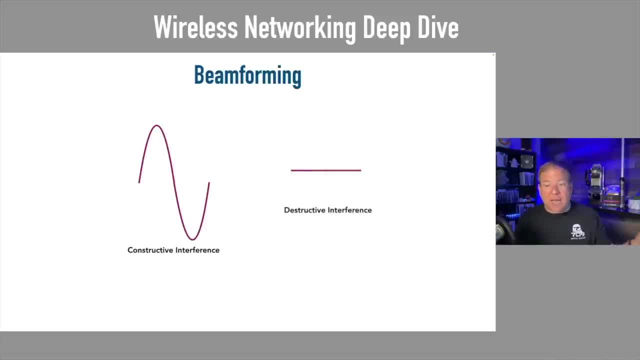 of it. you add those two up, it gives you approximately silence. That's destructive interference. That's how beamforming works. Beamforming works by using constructive interference to focus, and we do this with multiple antennas so it doesn't work on the really old access points that don't have multiple antennas. 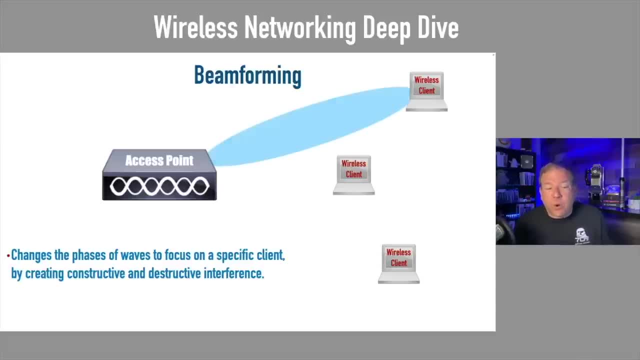 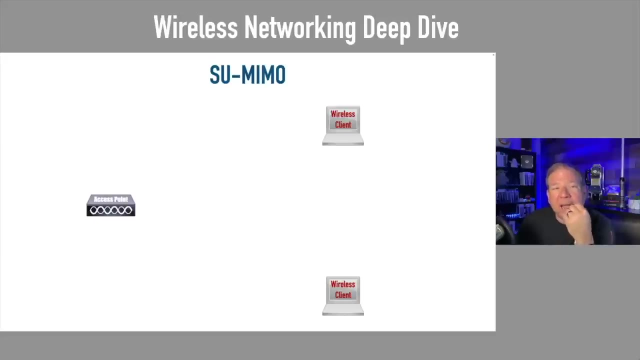 I think it was introduced in .11n, but you can focus your signal strength to this client, to this client, to this other client, without sending energy in the wrong direction. So that's going to give you better connectivity. Something else we can do is have more than one transmission. 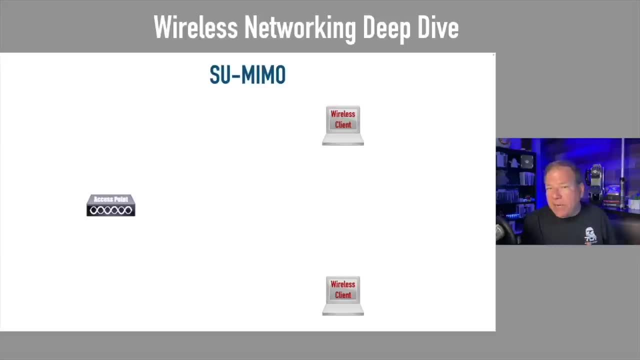 going out at one time. Now let's go back to .11n 2009.. That used something called single user or SU, multi-input, multiple output. We typically pronounce that MIMO or some people pronounce it MIMO. So MIMO or MIMO, whichever you prefer. I typically say MIMO, But single user MIMO. 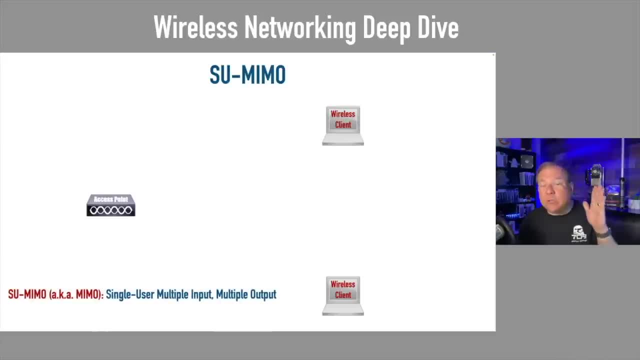 means that the access point can talk to one user at a time. So if I need to talk to these two clients, I have to take turns. I have one transmission path. It's called a spatial stream. I can send one spatial stream to this wireless client. and now, if I want, 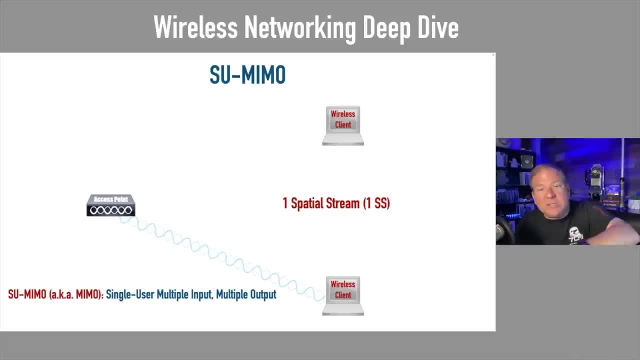 to talk to the other client. I have to then take turns and talk to it, but I'm doing it one at a time. That improved in .11ac That introduced multi-user multiple input, multiple output, also known as MIMO. 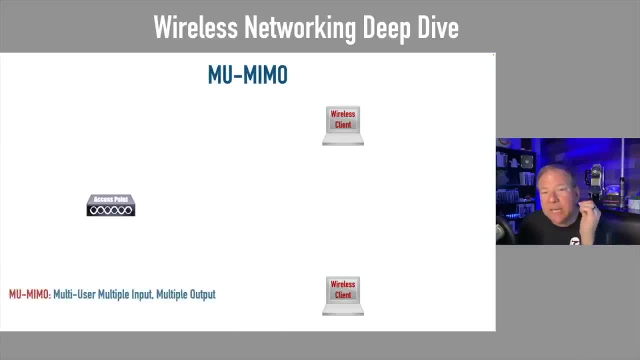 With MIMO we can send simultaneously. if I've got four antennas, I can send four transmissions out to four clients simultaneously. That's going to make it a lot more efficient. That's going to make my network a lot more scalable. Now here, I didn't want to use 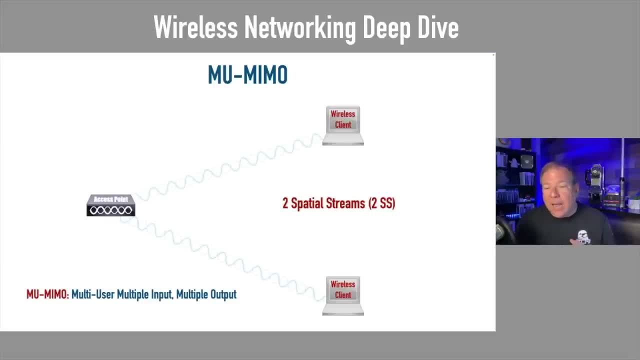 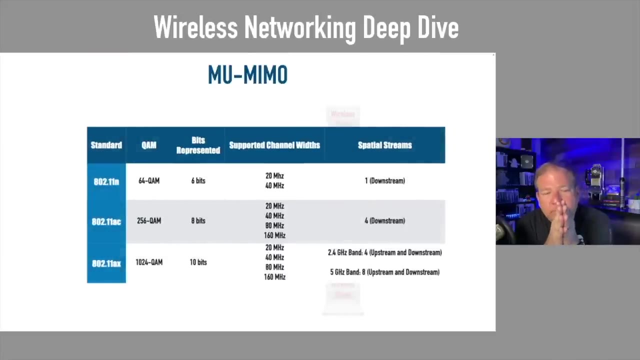 the space to draw four different clients, but this would work with four. I'm sending out two spatial streams to two different clients at the same time. That's going to give me more throughput as well. but with .11ac we could send four downstream spatial streams. but here was the caveat: We can only receive. 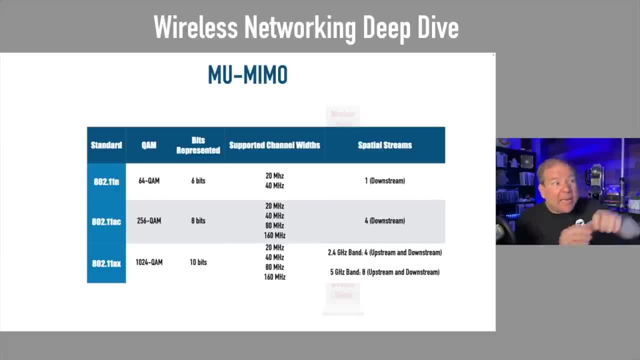 one at any one time. Yeah, I could talk to four devices at one time, but if people are trying to talk to me, it's still like the old Ethernet hub: Only one person can talk to you at one time. So I only had one upstream spatial stream. That improved dramatically with Wi-Fi 6.11ax. 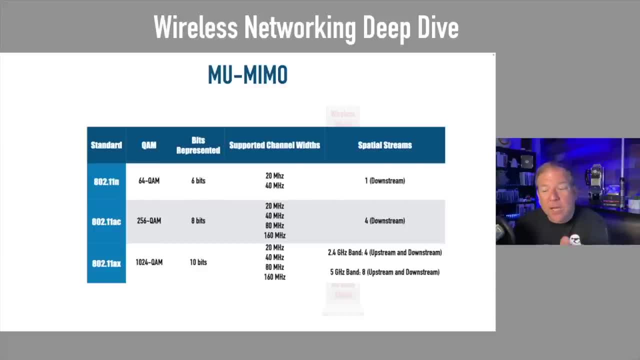 Here with the 2.4 gigahertz band, you can have not only four downstream spatial streams at the same time, you can have four upstream. You can be receiving from four different clients at the same time on the 2.4 gig band. 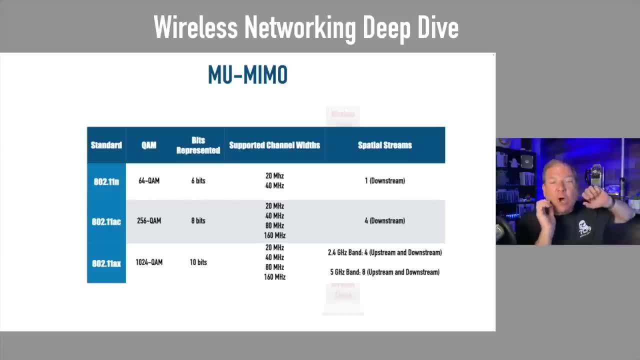 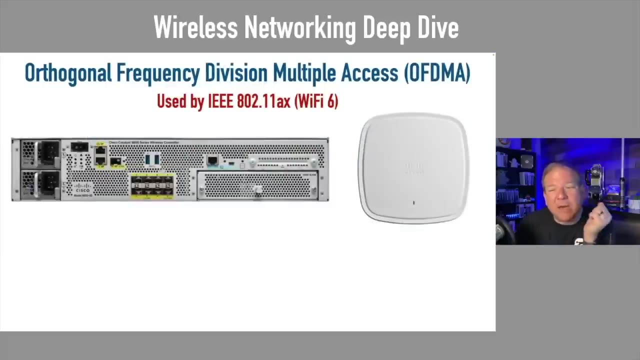 Using the 5 gig band, you can be talking to and listening to eight clients at the same time. That's pretty amazing, So that's going to give us even more throughput. That's how we're getting close to 10 gigabits per second with .11ax, also known as Wi-Fi 6.. A couple of other things I want. 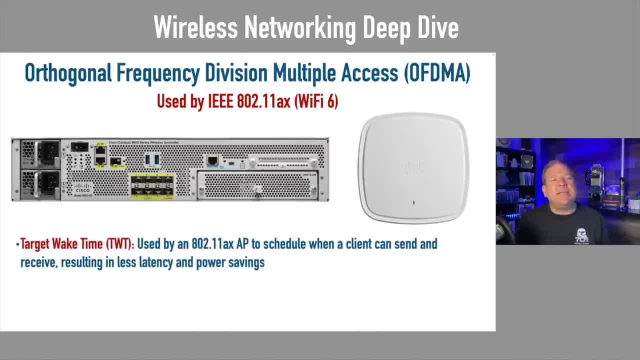 you to know about Wi-Fi 6.. One of the reasons that I would say it's more scalable than previous versions is when I used to teach wireless networking prior to .11ax, I would compare an access point. In fact, this is a .11ac, This is even ax. I would compare this to an Ethernet hub. 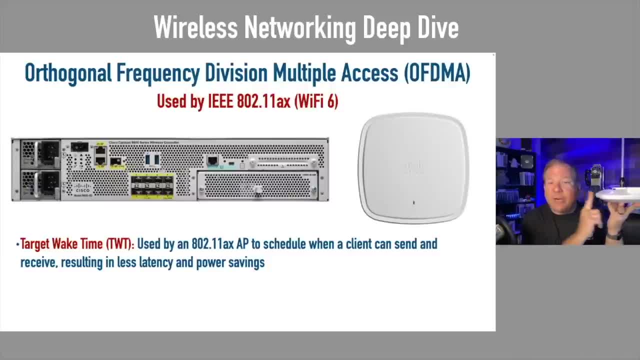 because with an Ethernet hub, you can be transmitting or receiving at any one time, but you cannot do both at the same time. Well, I shouldn't say that. With an Ethernet hub I can only be talking to one device at one time, So we use something called CSMACA. 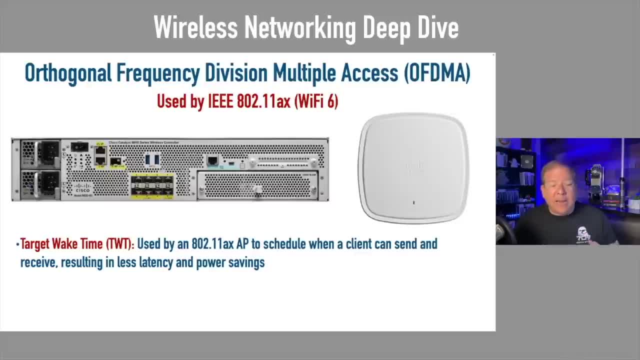 Carrier Sense Multiple Access with Collision Avoidance. And before a client could talk on the network, just like on an Ethernet hub, we had to listen to see if anybody else was talking. Is the coast clear? If somebody else is talking, I'm going to have to set a random backoff time. 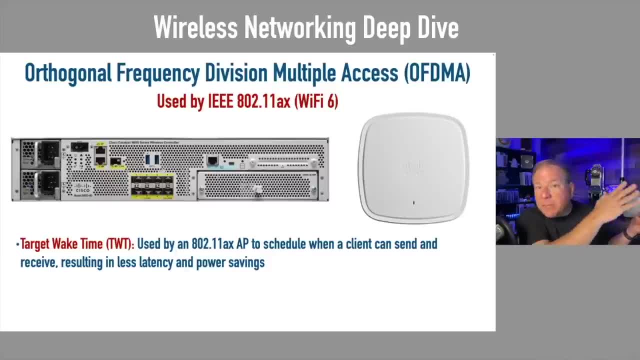 and I'll have to try again later because I cannot talk if somebody else is talking. But here it's a lot more determined. Here's what I mean: When access points connect out to their clients, they give each client a time slot and they say: when it's your turn, when I get to this time slot? 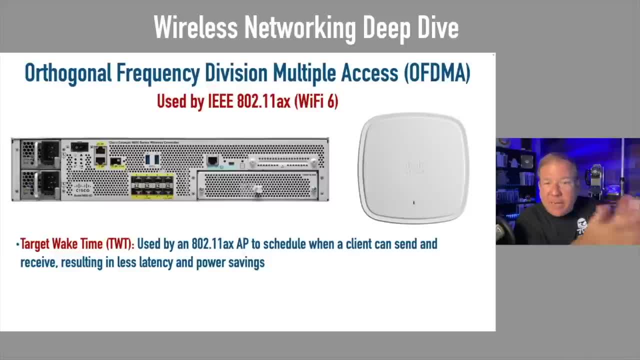 we're going to be able to talk. Don't try to send me anything if it's not your time slot. I'm not listening. Wait till it's your turn, then we'll talk. It goes to the next time slot. It talks. 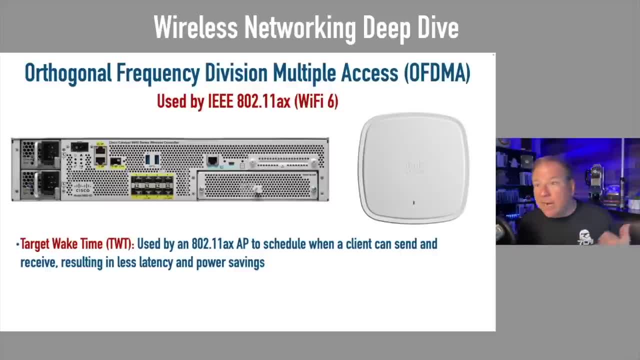 to another client, It goes to another client, It goes to another client, It goes to another client. So there's not this contention of can I talk now? Can I talk now? No, everybody's going to take turns, Kind of like the old. I hate to use token ring as an example, but it's kind of like. 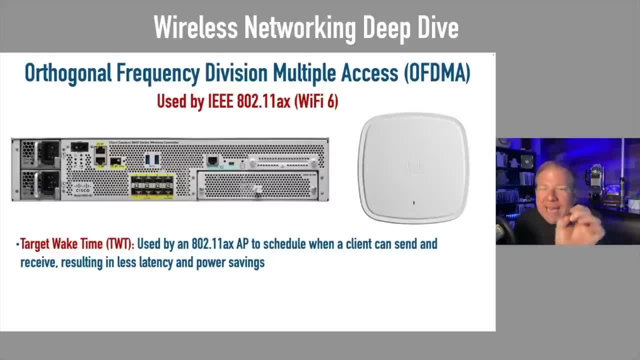 the old token ring network, if you remember that. But by taking turns. that gives us two huge advantages. Number one: by taking turns I don't have to just keep trying to transmit. oh, it didn't work. Somebody's talking. I got to wait. Got to wait. Oh, there's a collision. I got to. 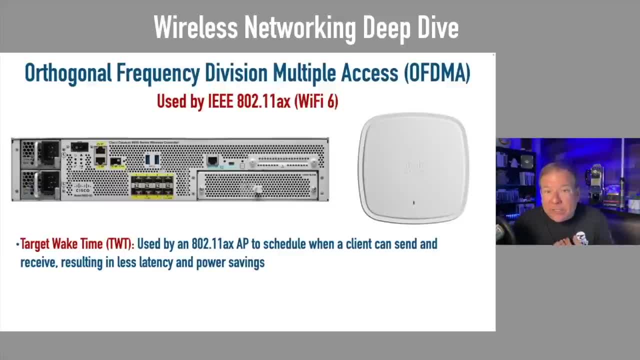 try again. No, I get deterministic transmission. I know when I can talk. Nobody else is going, it's my turn I can talk then. Another advantage I get is I know when it's not my turn to talk. I don't need to be using all this power to power up my radio. I'm going to chill, I'm just going. 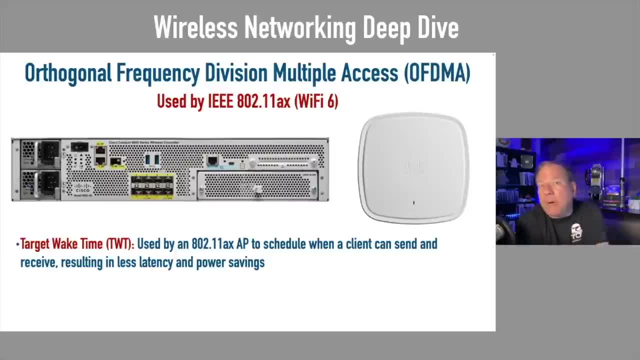 to power down my radio a little. I want to go into a low power mode Now. admittedly, that low power mode might only be for just a few microseconds, but over time it adds up. You're in low power mode most of the time. 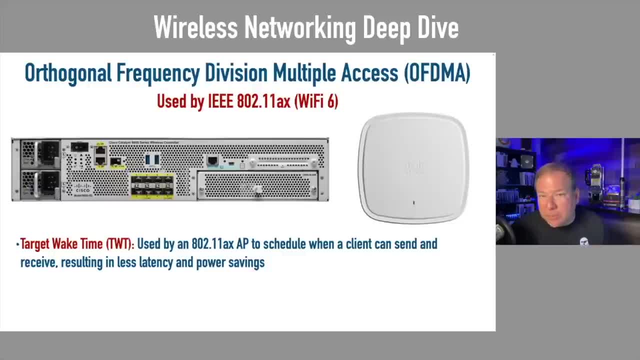 That's going to dramatically reduce the power consumption of your wireless card. So deterministic throughput, low power consumption, those are two big advantages of Wi-Fi 6, and that's called the target wait time. And also we talked about like in an apartment building. 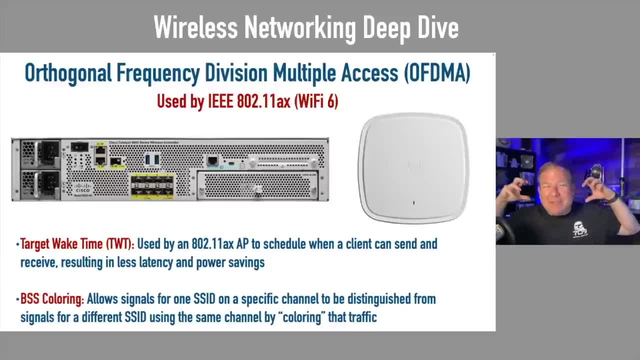 if you've got neighbors and they're trying to use the same channel. well, now there's something called BSS coloring, or basic service set coloring, where you can determine that if I'm trying to talk to my SSID using channel 6 and my neighbor's 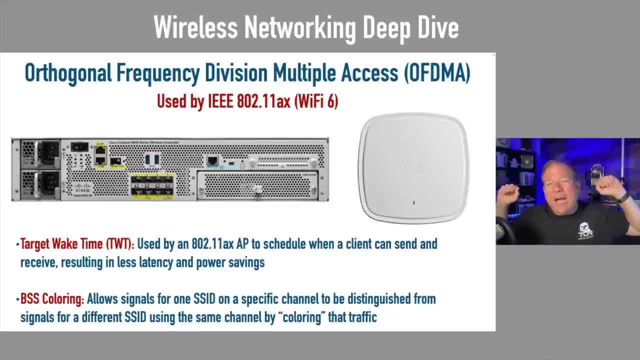 trying to talk to their SSID using channel 6 as well. they're not going to interfere with me because I'm not just considering my channel, I'm considering my SSID. It's kind of like labeling traffic on a VLAN. So that is another big advantage. So here's kind of a summary screen that we saw. 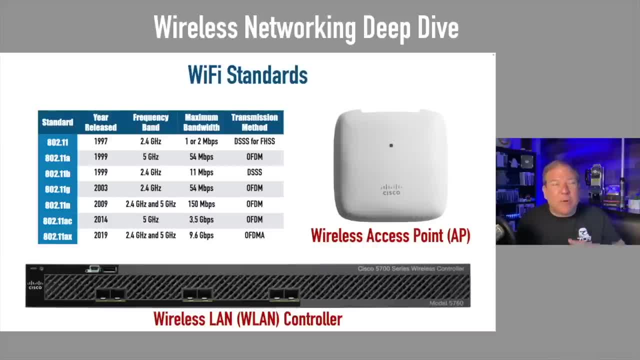 earlier Of the speeds and feeds of these different standards, how we've gone from a measly one megabit per second back in 1997, when I started working with this stuff, to today where we're approaching at 10 gigabits per second thanks to all those cool technologies. 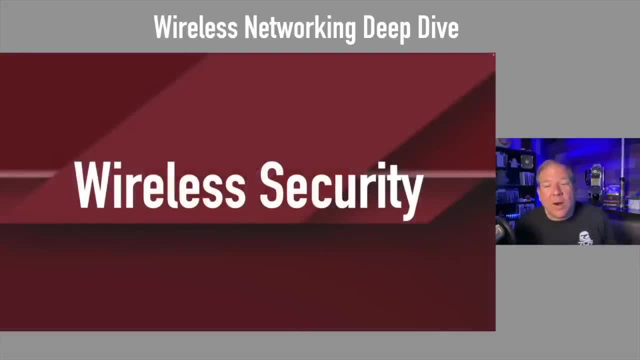 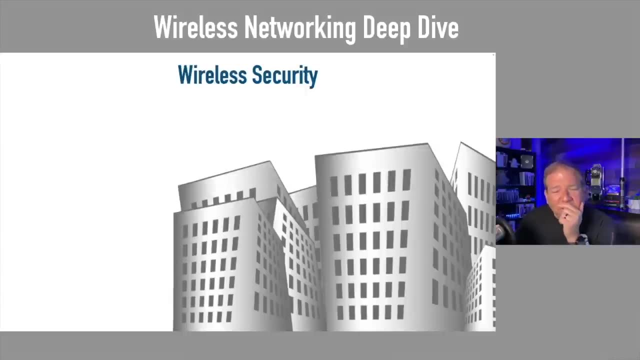 that we just talked about. Next up, we're going to be talking about wireless security, and this is a big concern. I mean, security is such a big concern today. And I would ask you this question: would you ever consider putting an ethernet port in the parking lot of your company's or on the wall of your company's? 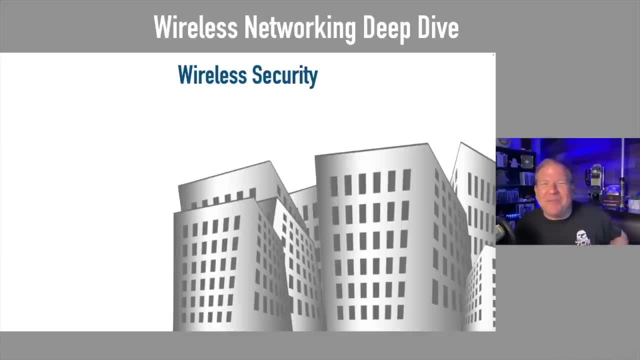 building and somebody could just drive up in their parking lot and plug into your ethernet port and get on your network. That would not be very secure, but that's essentially what a lot of people are doing when they that's what a lot of people are doing when they have wireless coverage. 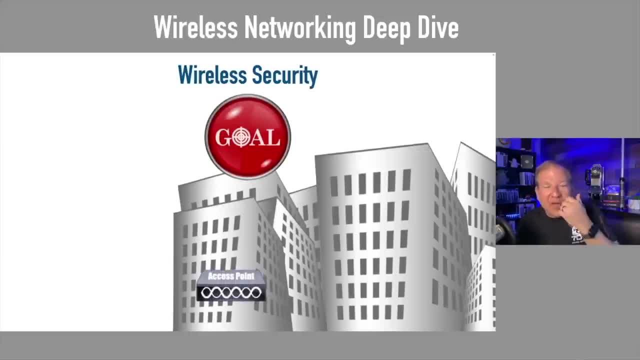 extending outside of their building. They might have a wireless access point and the coverage area extends, maybe out in the parking lot, and if it's not properly secured, somebody could come along and they could get on that network. How do we prevent that? Well, one thing is we could. 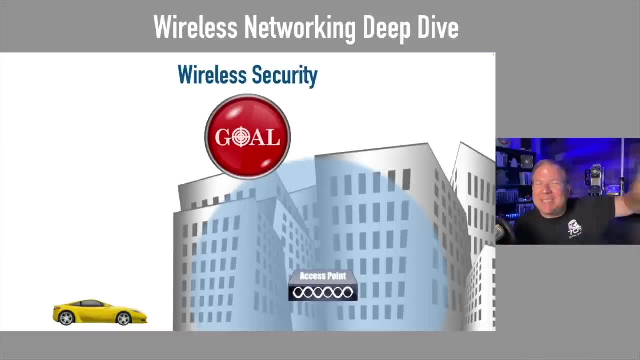 we could move that access point somewhere else where it's not going to be extending out into public areas, or we could adjust the signal strength, the power of the radio so it's not going to go further than it needs to go. But the two main goals we have with wireless security are: 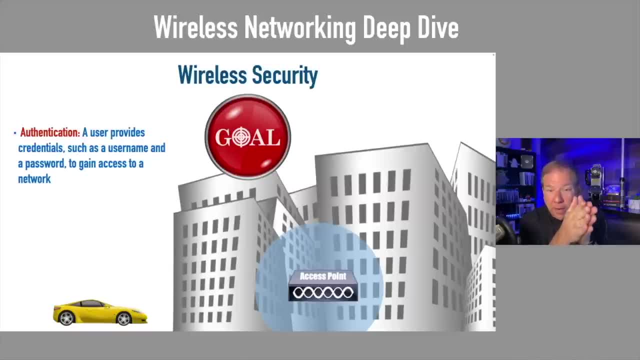 number one: authentication. Number two: authentication. Number three: authentication. We want to make sure people that get on the network are allowed to get on the network. We need them to authenticate themselves and we want to encrypt the traffic Because if we have some 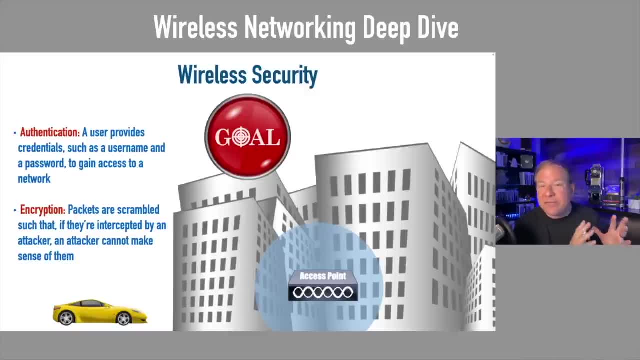 malicious user that's sniffing traffic out of the air. if they do intercept our packets, we don't want them to be able to make any sense of those packets because they're all scrambled up, they've been encrypted And we're going to be talking about in this section different ways. 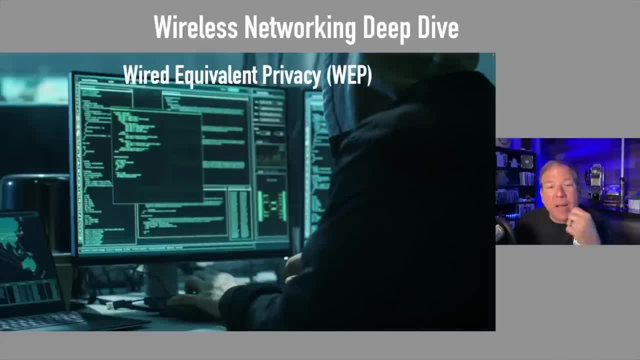 of doing authentication and encryption And we're going to be talking about in this section, different ways of doing authentication and encryption And we're going to start back with the original way of doing encryption, which was not very good. This was present back in the 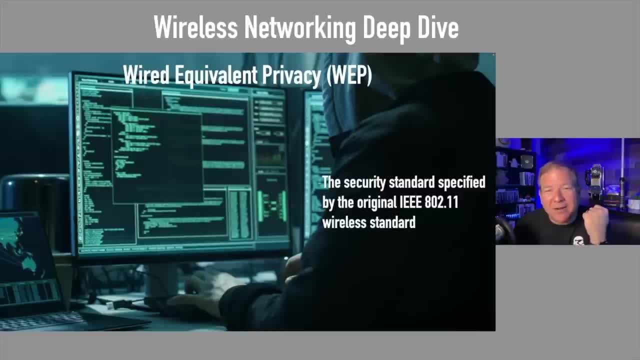 original .11 series or .11 wireless standard when we were running at like one and two megabits per second. It was called WEP- Wired Equivalent Privacy. The implication in the name is: the implication is it's equivalent to being as private as you would be on a wired network. 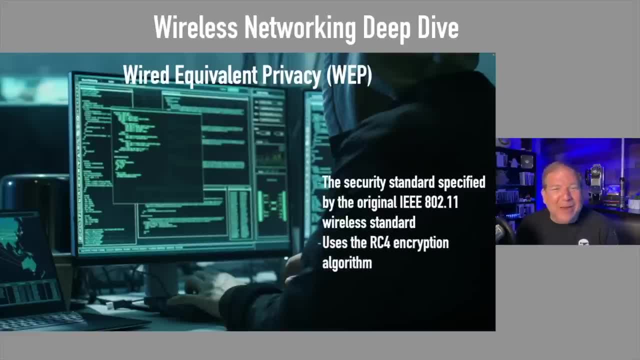 It's not even remotely close to the truth. It is very, very crackable. It is trivial to crack. If you're in an environment with an average amount of traffic, you can run an application on your laptop. You could sniff traffic for about eight minutes max and you'll have a 75% chance of being 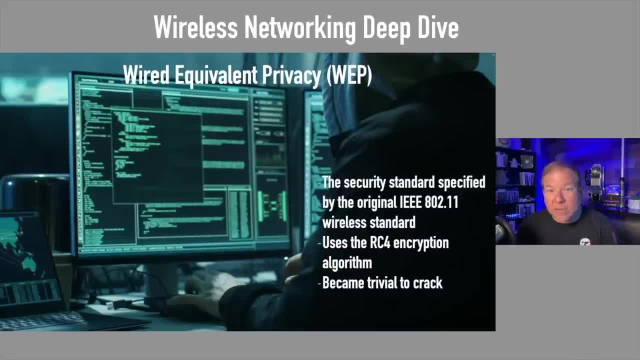 able to determine what the password, the wireless key is within that eight minute period of time. It is very easy to crack. Let's get down to the encryption algorithm that's used. Well, I don't want to beat up on the encryption algorithm too much. The encryption algorithm is RC4. That stands for Ron's Code 4.. 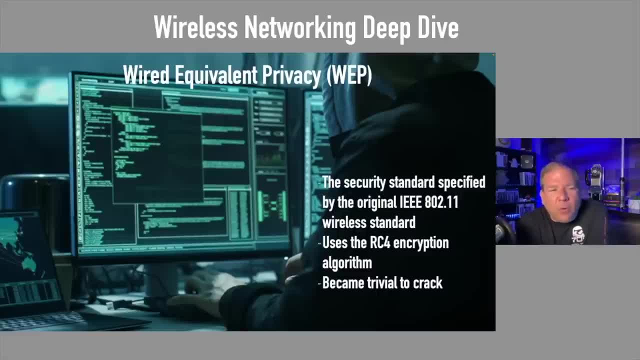 Ron is the developer of it. But RC4 uses something called an initialization vector, an IV. The IV, the initialization vector, is taken together with your wireless network password, your passphrase, and that's combined, Combined with the data. So you've got the data, you've got your password and you've got this. 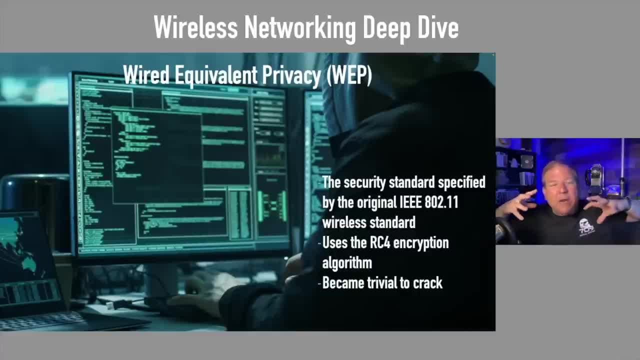 initialization vector. You've got these three parts and they mathematically get all squished together and that's what's transmitted. But the initialization vector, in the case of WEP, is only 24 bits long. And if it's only 24 bits long, that's what makes it so crackable, Because 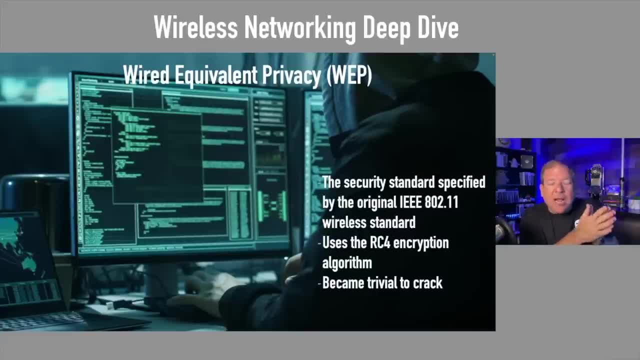 you're going to have more than one. you're going to have more than one data stream and it's going to produce the same encrypted string. They're called collisions, Not the same as collisions in the Ethernet world, But it's a way that we can mathematically determine. 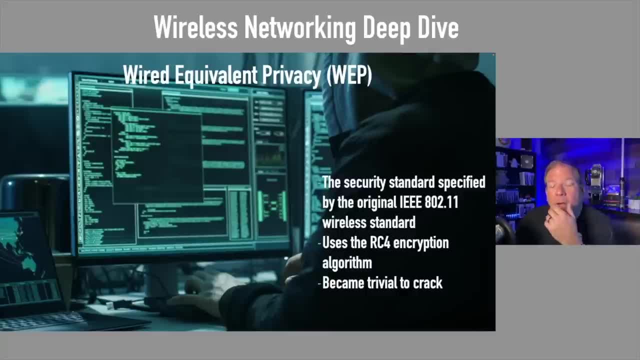 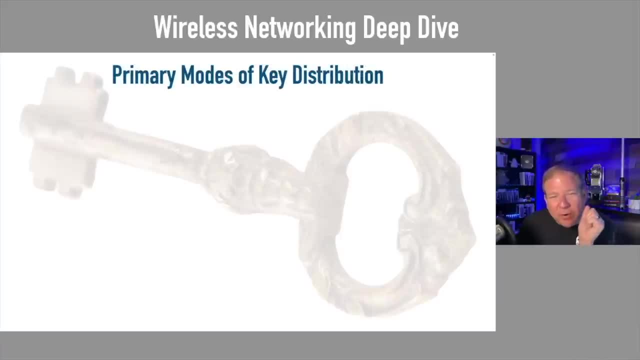 what the password is. So we don't like WEP. We should not be using WEP Now, this key or this password that we're going to be using to authenticate ourselves to the network. that can be given out in a couple of different ways. One is where we go to each device in. 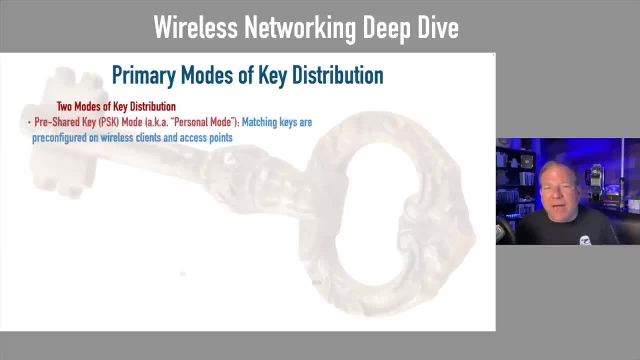 Seride. You type it on your phone, You type it in your iPad, You type it in your access point, And that is called a pre-shared key. Everybody has the same key. It's been shared with you and everybody in the environment is using the same key. This is probably what you would find. 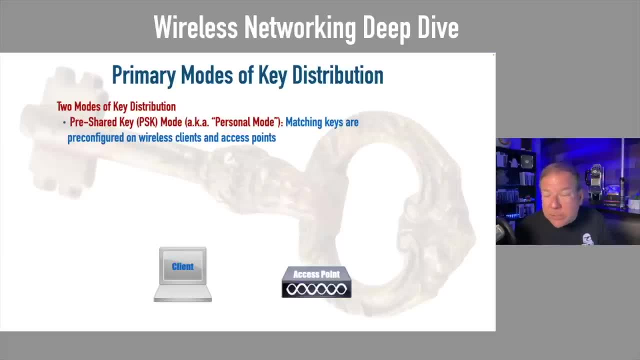 in your home or maybe a small business. It's not going to scale very well to an enterprise because if you had thousands of people in the enterprise, can you imagine a disgruntled employee starts giving the key out, or they leave the company or somehow the key gets compromised. You've got to go change the key on everybody's device. 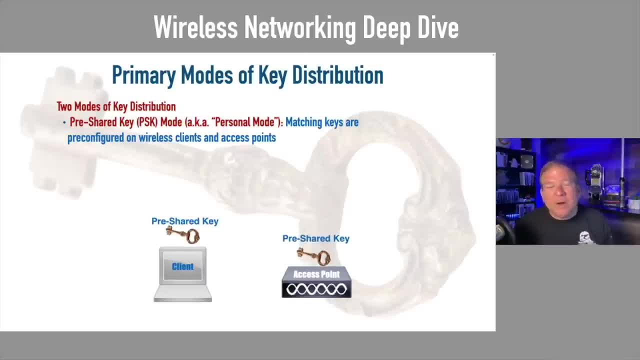 It doesn't scale well. So what do you do for an enterprise? For an enterprise, we're going to be using what's called a key pair. With a key pair, in enterprise mode you're going to have a key or not necessarily a key pair. It can be that. 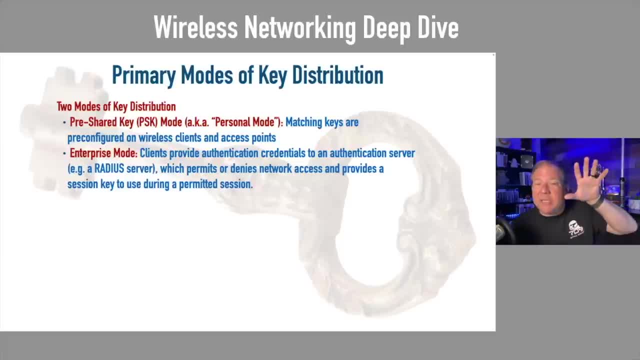 but you're going to have what's called a session key. It's a key used between your client and your access point, just for your connection And it's just for the duration of your session. That's why we sometimes call it a session key. Now, to get that key, you're going to have to 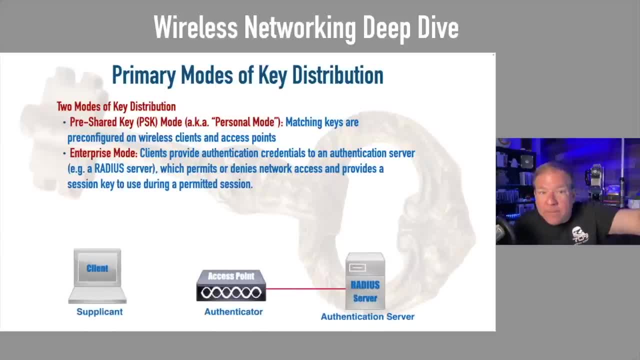 take your client and authenticate on the network. Typically that's going to be with a Radius server or Cisco's server that you might use to do this. It's called ISE, I-S-E, the IDC Identity Services Engine- But you authenticate And if you provide your appropriate authentication, 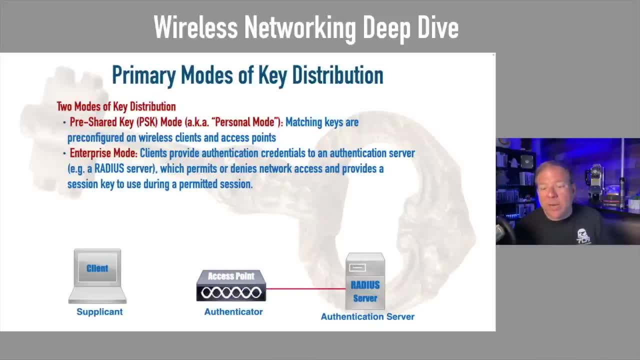 credentials. that authentication server, like a Radius server, is going to say: all right, you've authenticated. I'm going to create this key. It's only going to be good for you and only for this session. I'm going to give the key to the access point. I'm going to give. 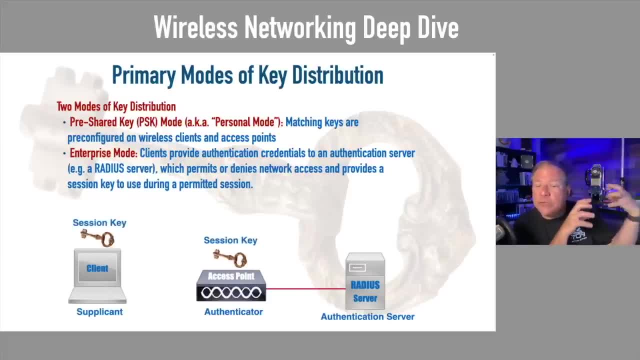 the key to you, So you and the access point. you can use that key for your encryption back and forth between yourselves. So even if you do leave the company, you don't know what the key is. And it's not good for any other session, It was only good for that one session. 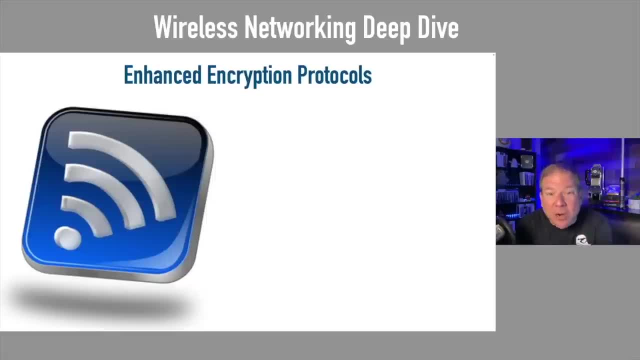 So we've got a couple of ways of getting that key, but we need stronger encryption. WEP is not going to do it for us. So let's take a look at the next evolution after WEP. After WEP- or WEP's, I should say- WEP's implementation of RC4, there was TKIP. 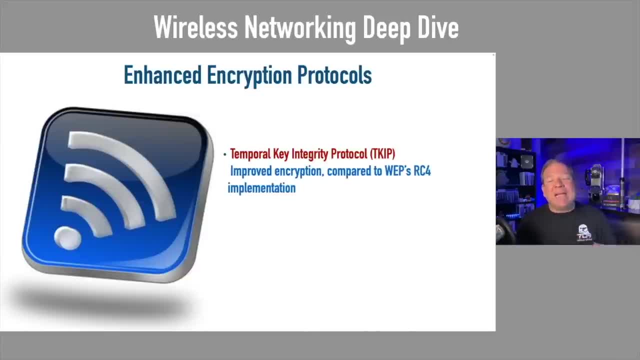 Temporal Key Integrity Protocol. This was vastly more secure than the RC4 implementation used by WEP. However, it still used RC4. You might say what I thought: RC4 was no good. It used RC4 with a much larger initialization vector which made it orders of magnitude. 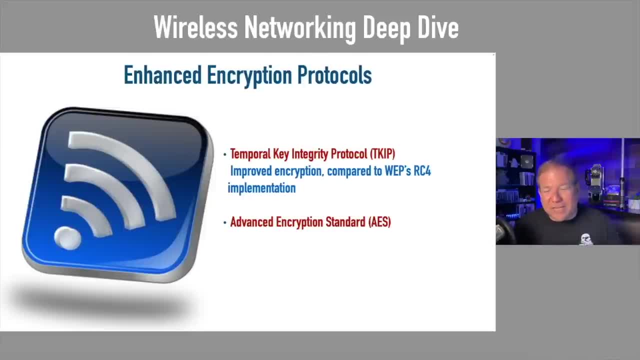 more secure- We'll talk more about that in just a few moments- But even better than TKIP is AES. This is sort of the flagship encryption algorithm out there today, The Advanced Encryption Standard. Could you say that again? What, Wow. 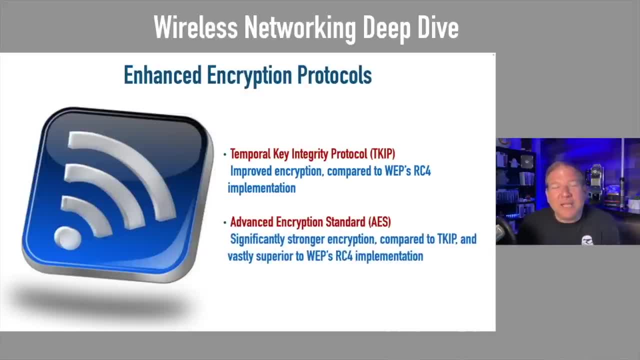 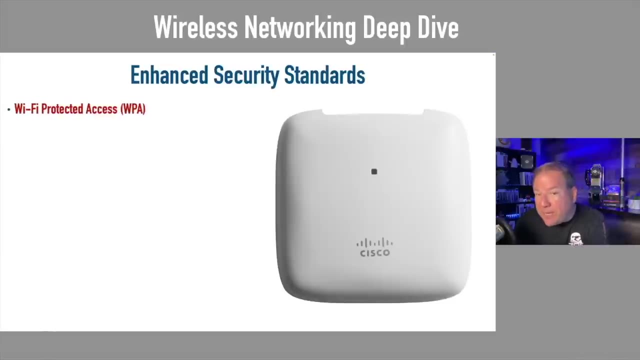 Siri wanted to get Get in on the conversation there on my watch. That was odd. But the Advanced Encryption Standard much more secure than TKIP, much more secure than WEP. And there were these standards that came out where you could say: I want to use WEP or I want to use WPA or WPA2.. WPA is Wi-Fi. 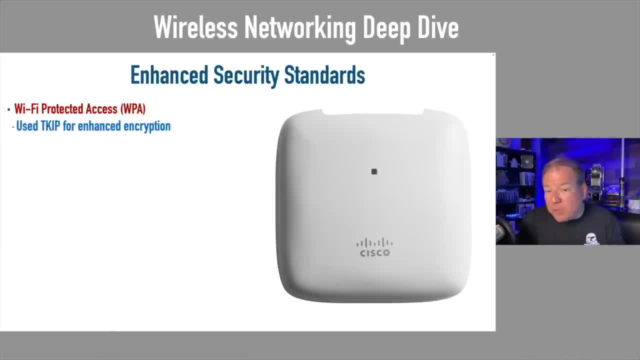 Protected Access. Its encryption solution was to use TKIP. That was better than what WEP used. Now I said TKIP. as great as it was, it still used RC4.. It still used Ron's Code 4.. But instead of using a. 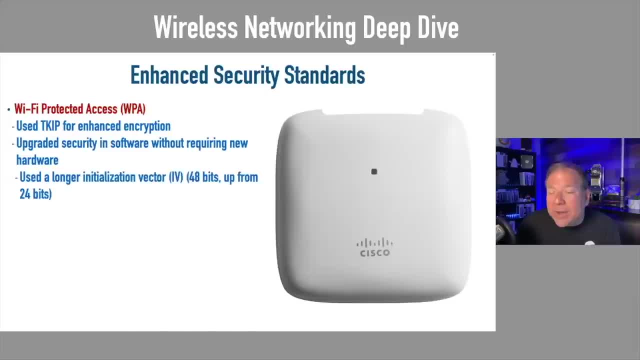 24-bit initialization vector. it used a 48-bit initialization vector And you might be thinking: okay, we doubled it. So now, instead of cracking the password in eight minutes, it takes 16 minutes. That's not, No, no, no, no. It's not twice as secure When we go from 24 bits to 25 bits. 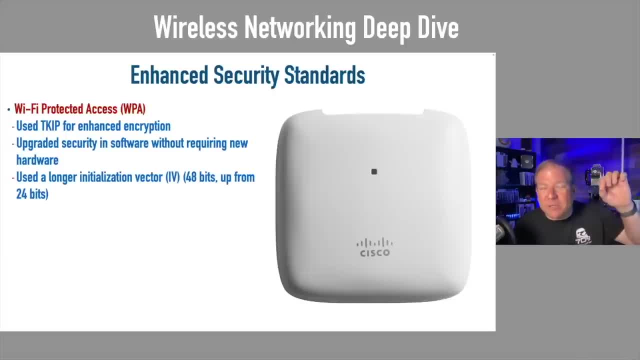 that doubles the security. You go from 25 bits to 26 bits. that doubles the security. By the time you get up to 48 bits. we're orders of magnitude more secure than the way WEP did it. Now you might say: 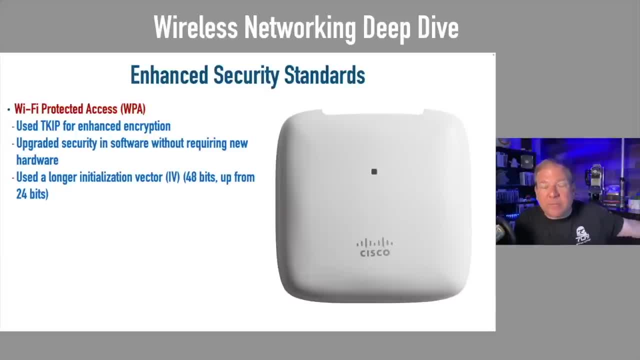 wasn't AES around back then? Couldn't we have gone straight for something more secure? Yes, it was around back then. There were more secure algorithms out there, but we're talking about the early days of Wi-Fi networks. There was so much processing required. 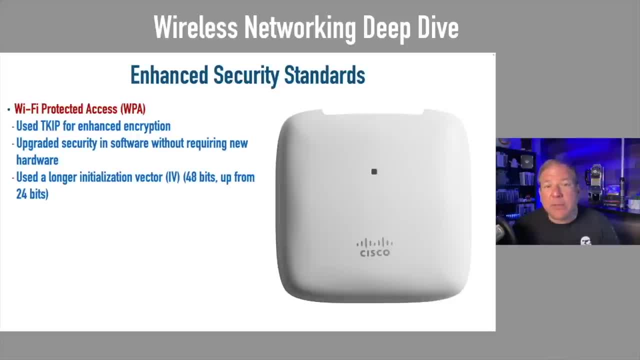 to do the encryption and the decryption. Some of the older wireless hardware just wasn't up to the task of using AES. So WPA with TKIP it was sort of a. It was an interim baby step fix. It was better than WEP but yeah, it wasn't the best encryption out there. 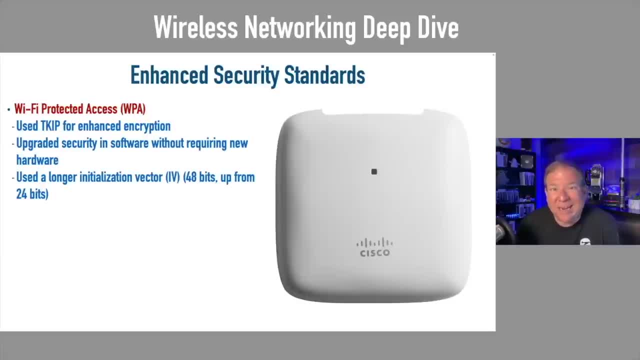 because we had older hardware that just couldn't handle it. Well, around 2006,- well, just prior to that, but around early 2000s- WPA2 came out. Now, the reason I said 2006 is in 2006, in order to 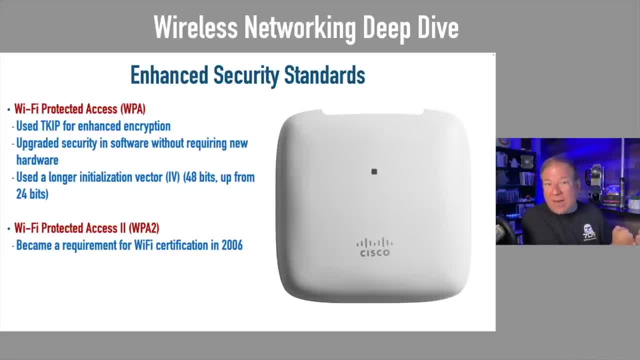 get the seal of approval from the Wi-Fi Alliance to say you're Wi-Fi certified, your device for WPA2 had to support- or rather, to be certified for Wi-Fi, your device had to support- WPA2.. Now WPA2. 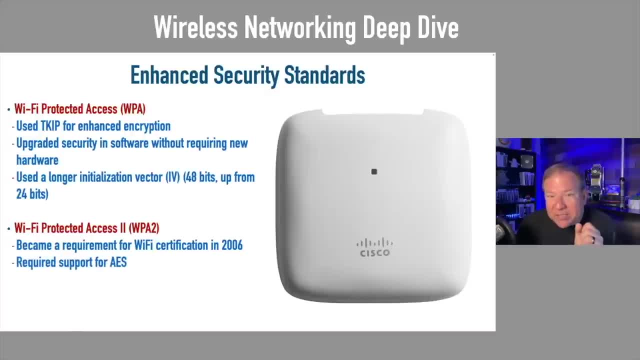 had a requirement to support WPA2.. Now WPA2 had a requirement to support WPA2.. Now WPA2 had a requirement that it had to support AES, the Advanced Encryption Standard. But in 2006,, didn't we still have some older, lower powered wireless hardware out there? Yes, So here's what. 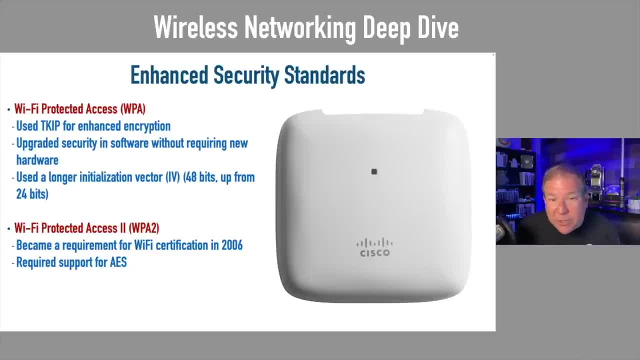 the compromise was With WPA2, you had the option of still using TKIP if you wanted to, Because if you're in an environment that had the older hardware that would just be overburdened with all the processing of encryption and decryption. you had the option of still using TKIP if you. 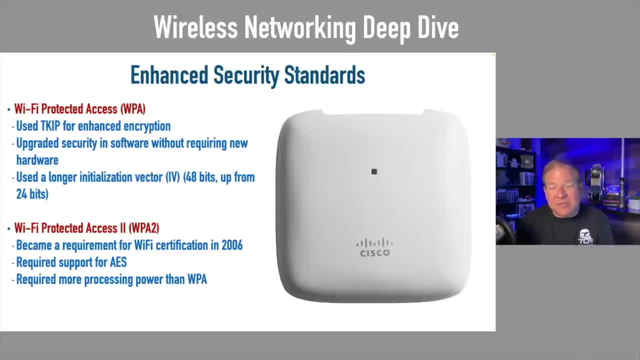 wanted to, Because if you're in an environment that had the older hardware that would just be overburdened and decrypting AES, you could say, eh, I'll still use TKIP. But you had to be able to. you had to. 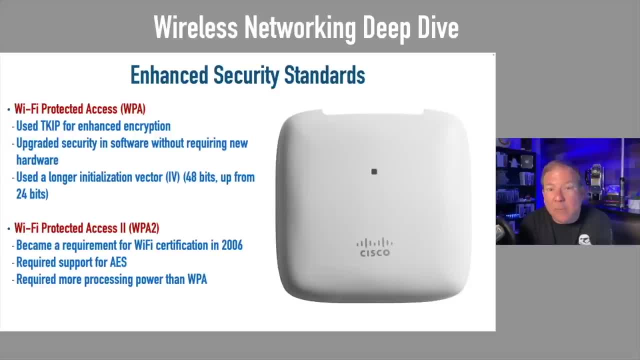 support AES. It had to be available on that device but you could turn it off Or you could say: I'll do both. So my older hardware that can only do TKIP, it'll do TKIP. My newer hardware that can: 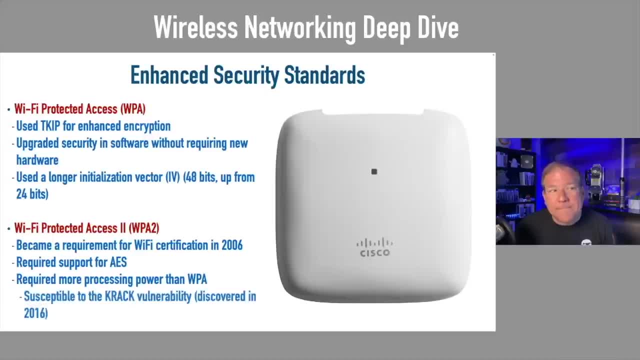 do AES, it'll do AES, But it was. I mean, we're starting to get better and better now, where AES is at least an option, And for about a decade, this was the flagship go-to security standard that you wanted to put. 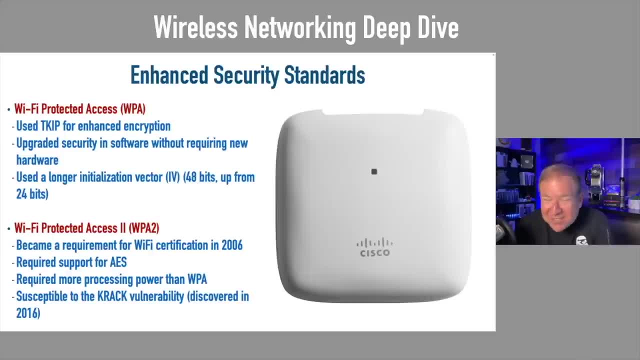 on your wireless access point Until 2016.. Then there was another vulnerability discovered, called the crack vulnerability, that was able to crack WPA2 networks. Now this attack is much more difficult to carry to pull off. I've read the process to go through It's. I don't think I. 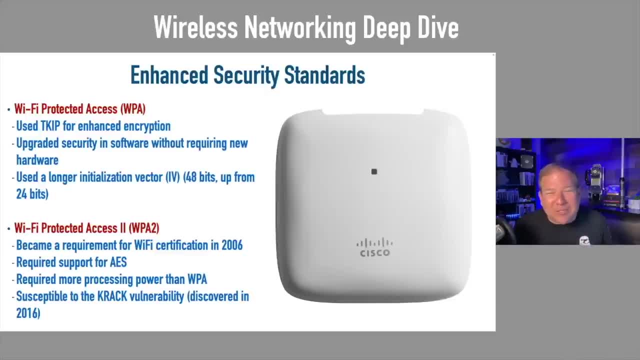 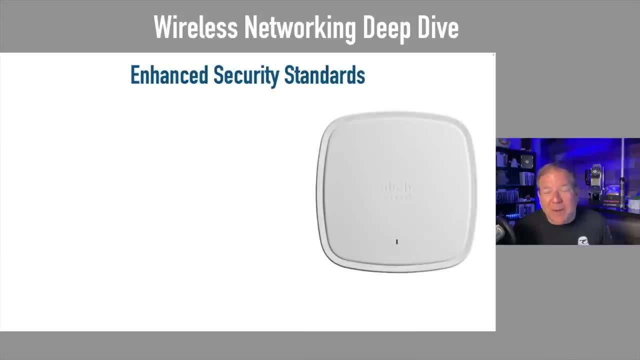 would be able to do it easily without doing a lot more reading and research. It's. it's a difficult attack, but it's out there, and WPA2 networks can be compromised. So what came next? You guessed it: WPA3.. Now, today, this is the flagship, This is the best. 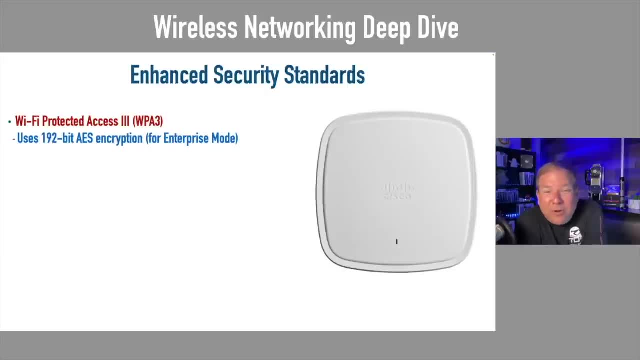 option we can go with, but it's not supported on all of your access points, So WPA2 is still considered pretty good, even though that crack vulnerability is out there. But if you can do WPA3, I'd do WPA3.. 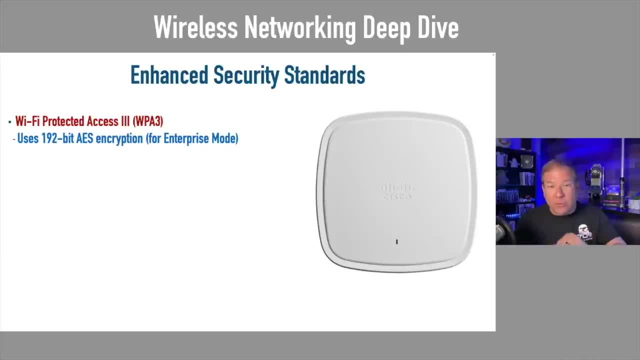 Now WPA3 is even stronger if you're in enterprise mode. Now, remember the two modes of key distribution. There was personal mode, where I I hard code my password on this device and I hard code my password on the access point. But there was enterprise mode where my radius server handed. 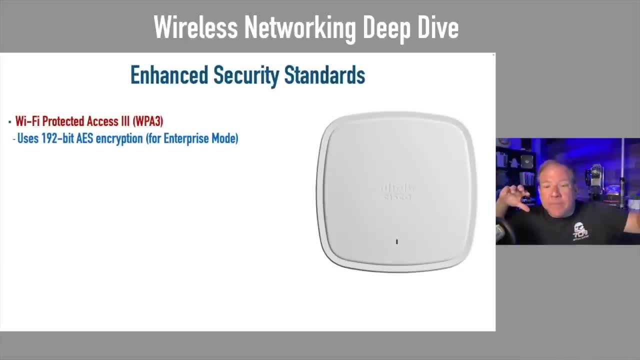 out session keys per device per session. If you're in enterprise mode, if you're using WPA3, it uses a stronger version of AES. The AES we've been talking about up till now was 128 bit AES 128. 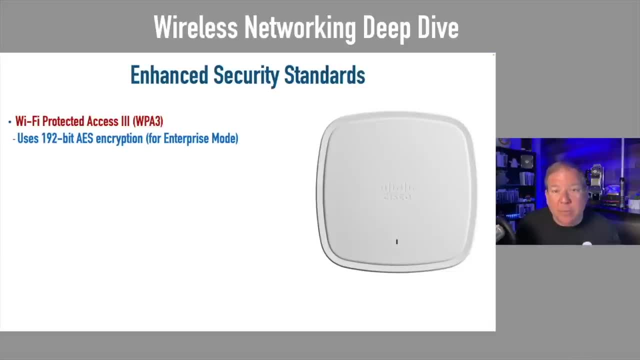 So WPA3 is a stronger version of AES. So WPA3 is a stronger version of AES. So WPA3 is a stronger version of AES. Well, if you're in enterprise mode with WPA3, it's 192 bit keys, So that's a lot stronger. 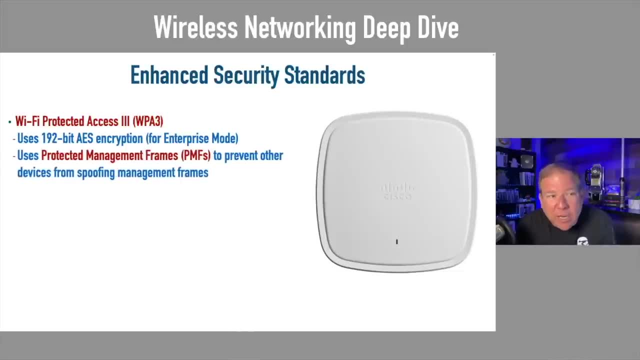 There's also something called protected management frames. Now, if you were to join us for some of our ethical hacking training? in fact, I demonstrate this in some of our training, where I send deauthentication frames to a wireless access point to knock off a client And when that client 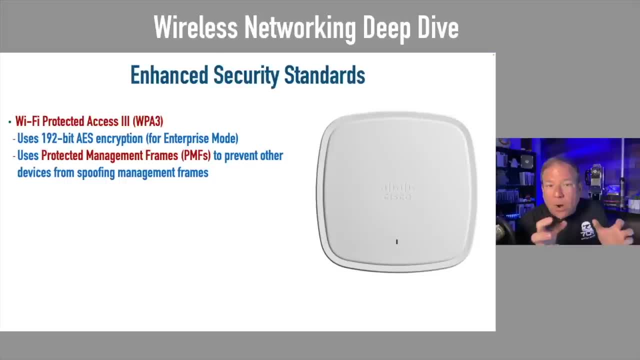 reattaches. I'm sniffing the airwaves with my wireless card and I'm able to watch the four-way handshake as it reattaches. I'm able to take that I run it against a dictionary of well-known passwords, like 14 million well-known passwords, And in a span of less than about 25 minutes. 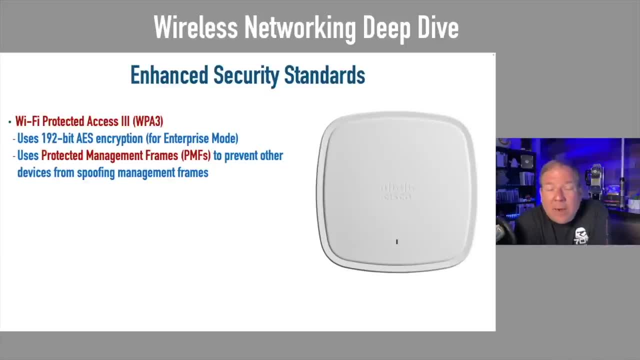 it takes for that attack. I can determine a wireless access points password. WPA3 protects us from that. It doesn't allow me to deauthenticate people. It doesn't trust my management frames that I'm sending in. It also prevents me from taking this device offline. 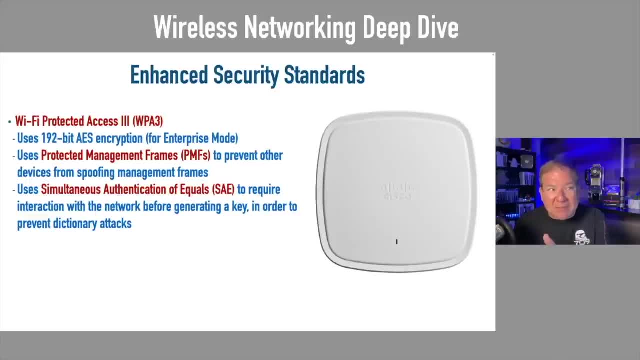 This is called a simultaneous authentication of equals. That name is not descriptive of all of what it really does. What it means is: I cannot take a device offline and just run a brute force attack and say, all right, what about this password, this password? No, I have to be communicating. 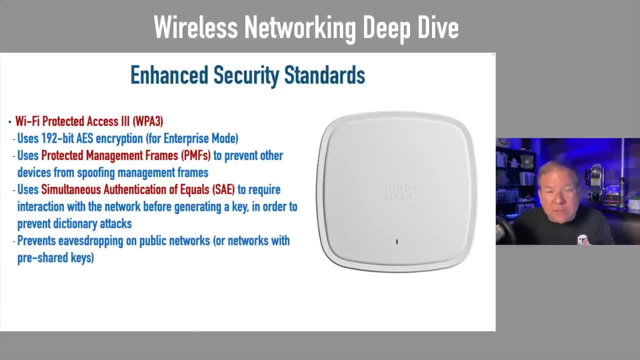 on the network in order to try those password attempts. So it's going to help prevent those brute force attacks And if you're on a public network, like you go into a coffee shop or you're at an airport- and you join without a password. yeah, traditionally people have been able to. 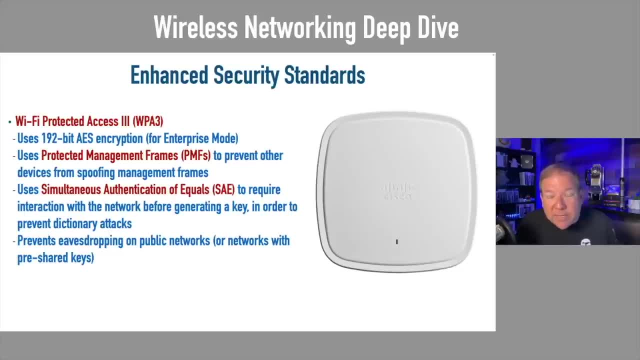 eavesdrop in on your traffic, So it's a good idea to set up a VPN connection when you do that. Here, WPA3 helps protect you on those public networks, And for years- for over a decade. let me see if I can find the button on here. Yeah, here it is. There's a little button. I. 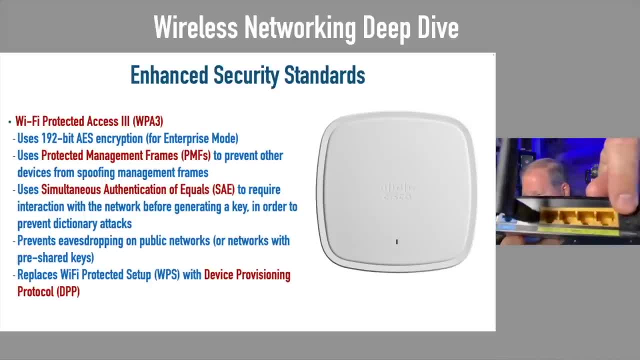 don't know if you can see it on the back of this right there That is a wireless access point, Wi-Fi protected setup, a WPS button That allows me to press that button and I can go add on new additional clients without having to go into the configuration page and type in the pass. It was. 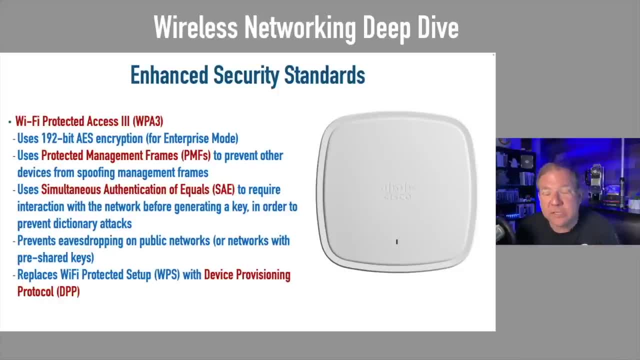 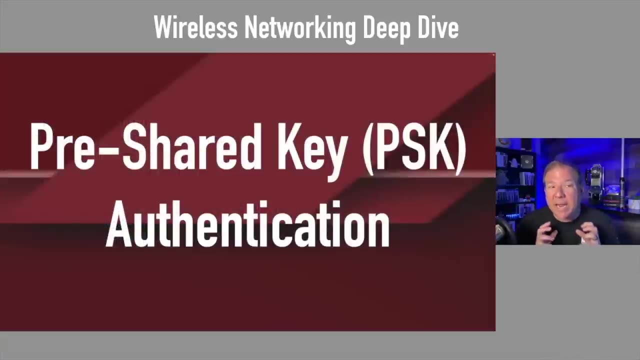 an easy way to add clients to a network. Well, there's a security vulnerability in that too. That gets replaced in WPA3 with something called DPP, device provisioning protocol. So those are how these security standards have evolved over the years. Now let's take a step back and see how. the theory behind it works. So let's take a step back and see how the theory behind it works. So let's take a step back and see how the theory behind it works. So let's take a step back and see how the theory behind it works. 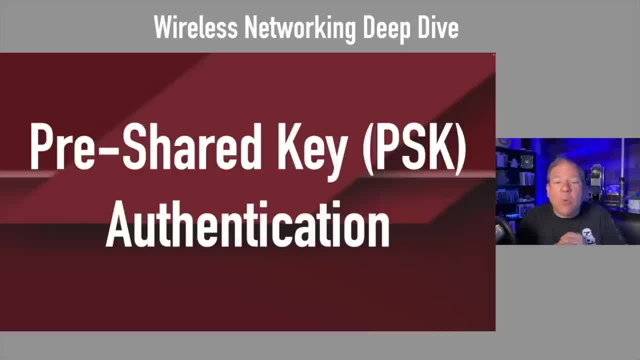 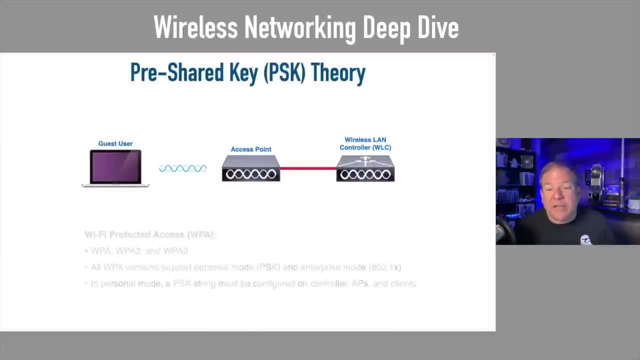 And how to configure. we're going to get into some demos now- how we can configure some of this authentication, starting with pre-shared keys. Pre-shared keys: that's where I go to my client and I go to my wireless LAN controller or my access point and I type in those keys. 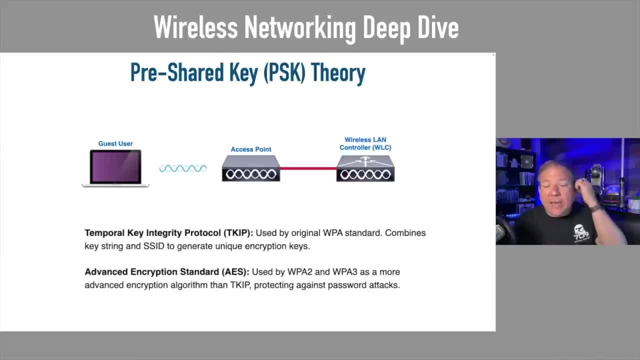 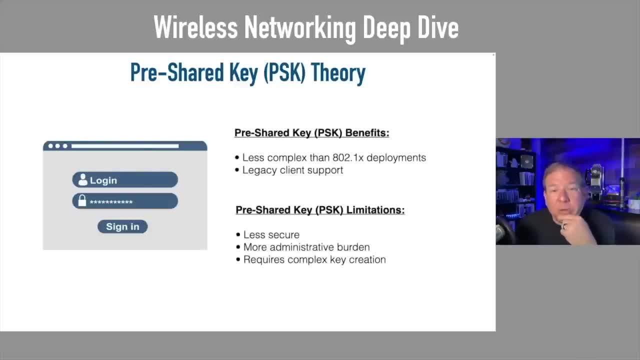 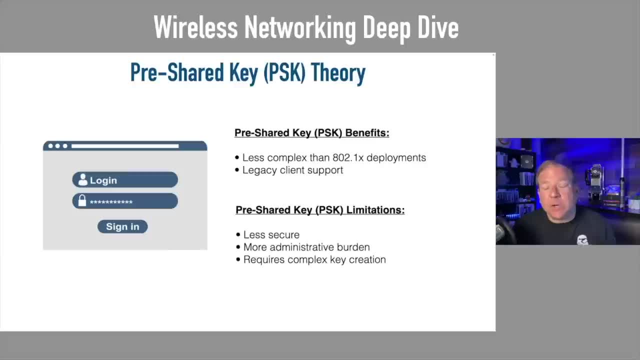 going to demonstrate that for you using Cisco Packet Tracer in just a moment. But with a pre-shared key it's going to be a lot easier to set up for small deployments. You don't have to have an external authentication server like Cisco ICE or a Radius server. You just put a password. 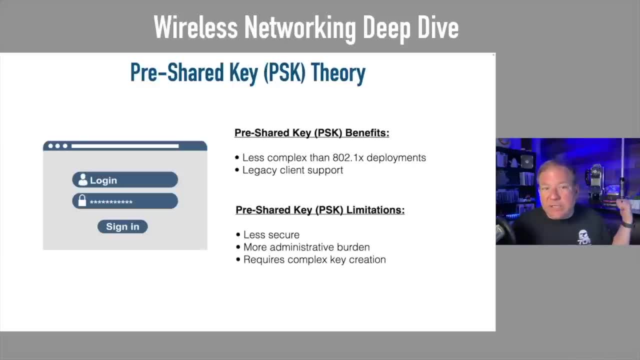 on your devices. It's going to support devices that are older that might not be able to set up out support enterprise mode. On the downside, it's not going to be scalable, It's not as secure And we don't want to use it in large environments But for small environments. 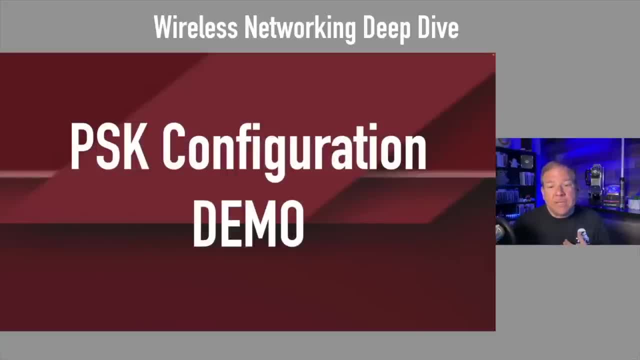 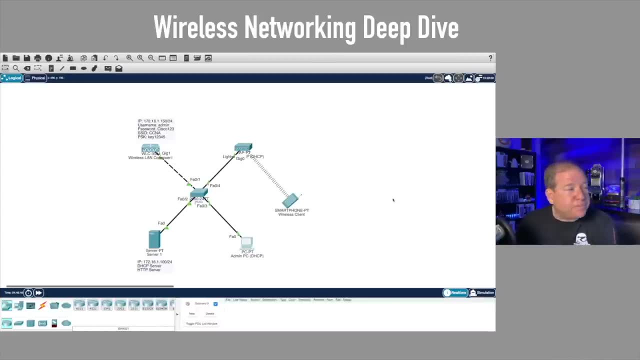 I mean for my home. that's what I'm using. Let me show you how we do this. Let's go out to Cisco Packet Tracer Now. I showed you earlier the link you could use to download this Right now. I've got an SSID called CCNA. 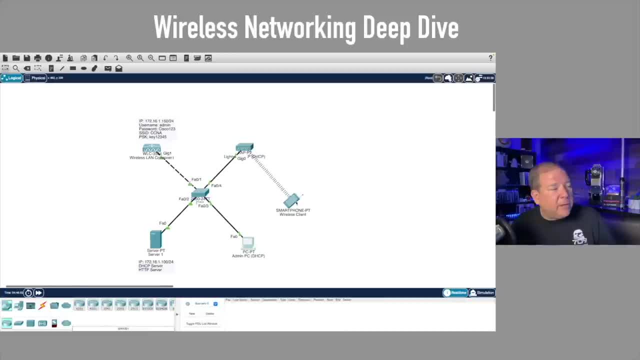 Business Advertising. This wireless phone currently belongs to the CCNA network. What I want to do is I want to go configure another wireless network on this wireless thing controller. Again, this is exactly what the CCNA Blueprint says you need to be able to configure. So I'm 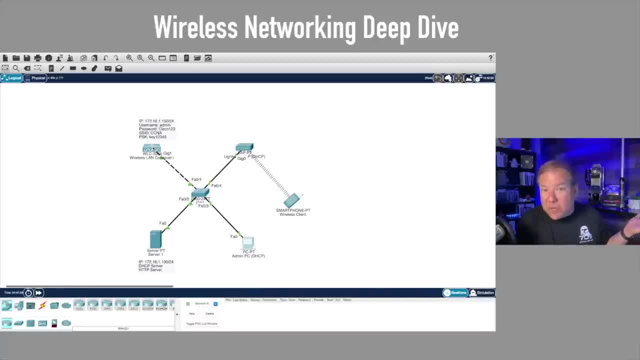 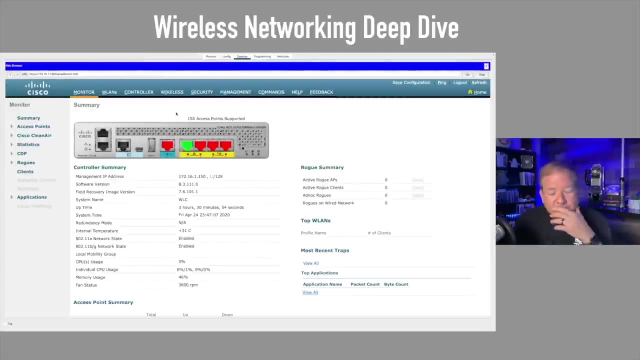 going to walk you through it And I gave you the links to download this stuff so you can practice on your own. So to do this, I'm going to open up a browser on my client, my PC- Which I've already done actually- And we're logged into that wireless link controller. I'm 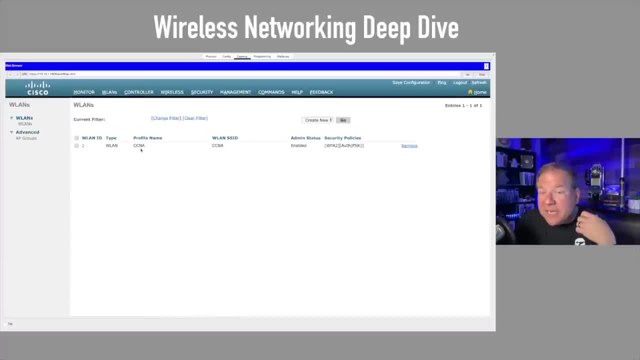 going to go to wireless LANs, And I've already got one called CCNA. Let's add a new one. To add a new one, I'm going to say create new. In fact, let me take my face off the screen. so. 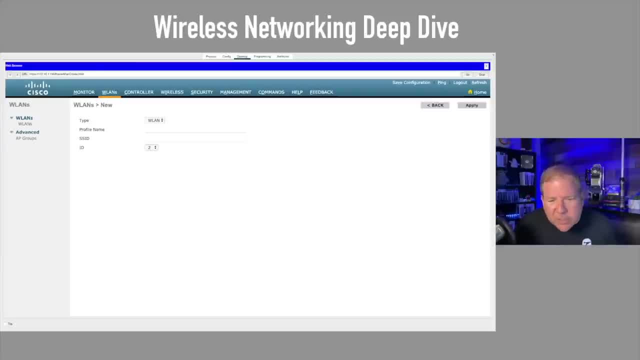 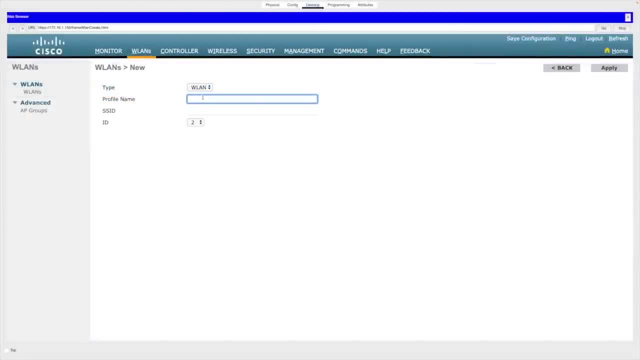 everything will be just a little bit bigger because the writing is a little bit small. Yeah, that makes it easier to see. Now for the profile name and the SSID: the profile name, that's a way that we're going to add a new one. So I'm going to add a new one And I'm going to 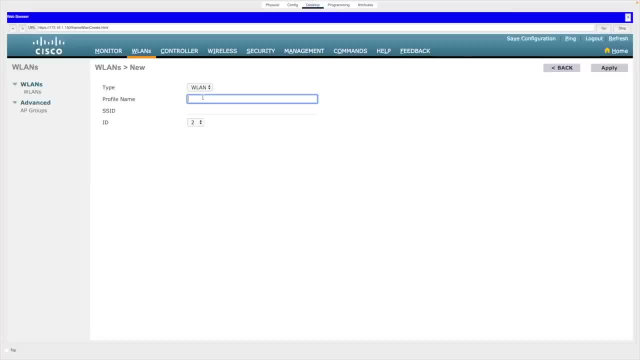 we can search and group and apply policies to things that belong. You could have a headquarters profile or a branch office profile In our case. I just want you to know. this is not the network name, But it could be. In fact, let's just call it. I'll say it's CCNP, But the SSID that I'm 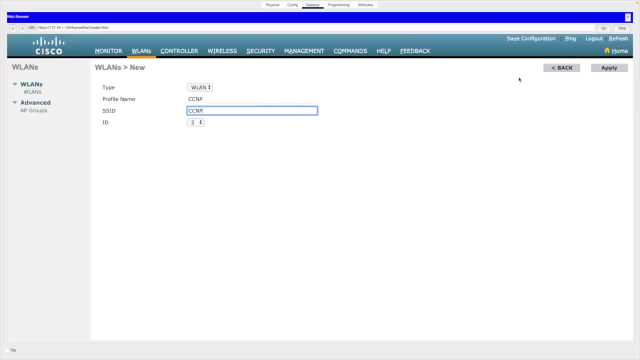 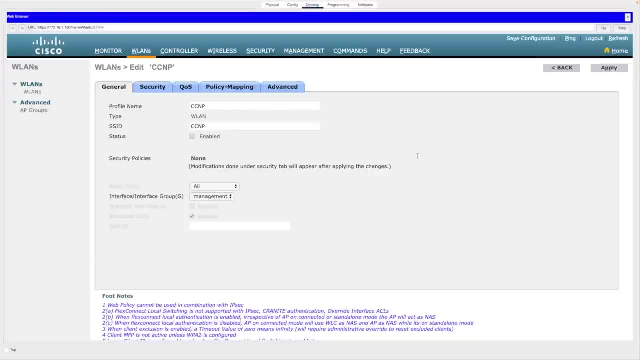 advertising. that's going to be CCNP. So I've created a new wireless network, an SSID, called CCNP. Now here is a big gotcha. Please hear me on this When you're doing this on your own. if I didn't tell you this, 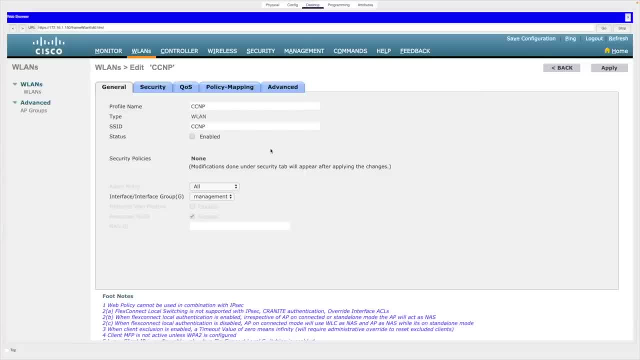 a large percentage of you, I predict, would not get it to work because you didn't check this. enable checkbox. Please make a note of that. You got to say it's enabled. Once it's enabled, we'll apply that. And now let's set up security the way Cisco says we have to do it for CCNA. 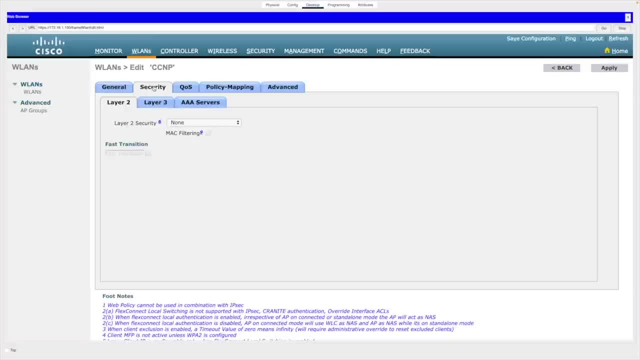 We're going to go into the security tab And we're going to set up layer 2 security using WPA2.. Now this says WPA plus WPA2.. That means either one, So I'm going to select WPA plus WPA2.. And I want to use a pre-shared key. 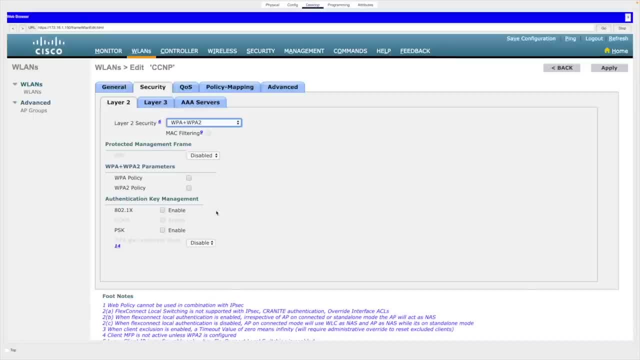 That's what Cisco says. we need to know how to do. So. I'm going to use WPA2, and I'll check that WPA2 policy And I'm going to check pre-shared key. But notice this: When I say yeah, I want to use WPA2, it says, oh, which encryption do you want to use? Remember? 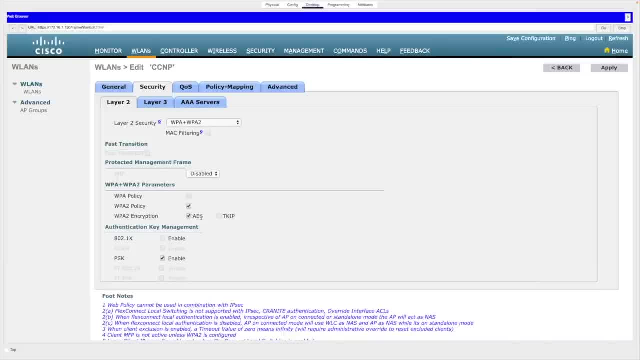 WPA2 had to support AES, but it could also support TKIP or you could do both. I'm not going to support TKIP, I'm just going to leave it at AES. So I've got AES selected, WPA2 selected, pre-shared key selected. Now I'm going to enter. 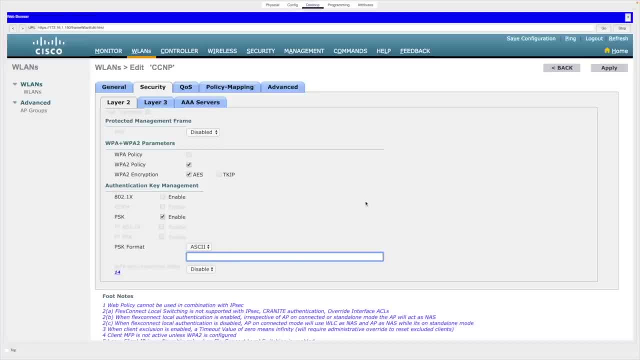 my pre-shared key And I'll just say it's CCNP, all caps 123.. Not a great key, but we'll take it. Oh, I didn't have enough characters in it. Let's see, I'll say CCNP in uppercase and then CCIE in lowercase. Try that. 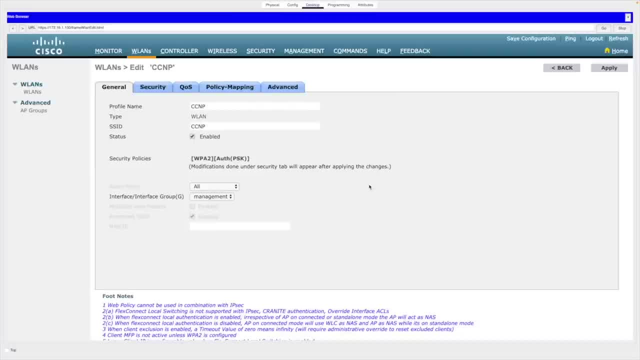 And that just says all right. if anybody's connected this network, you're going to knock them off because you just changed the password, All right. So that's my configuration. Layer 2 security: WPA plus WPA2.. WPA2 policy- AES. 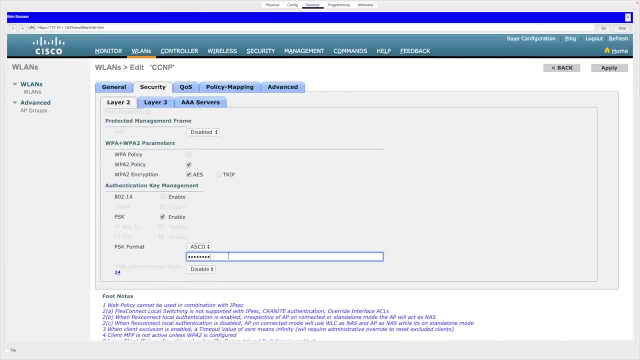 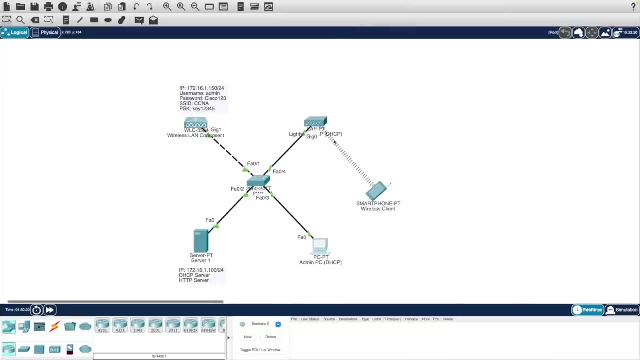 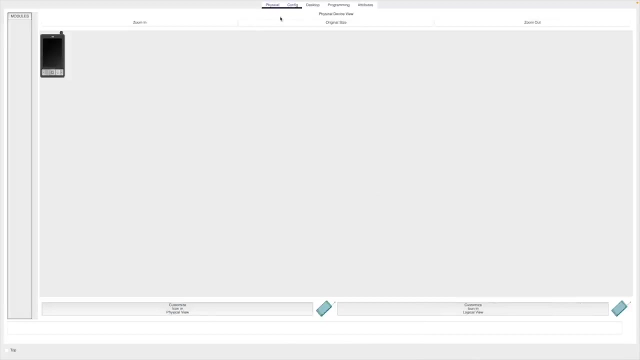 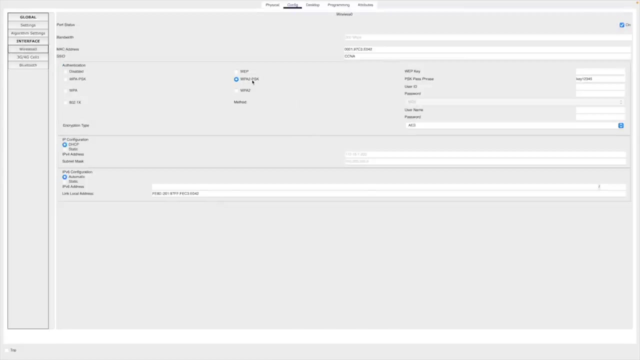 pre-shared key And I gave the key of CCNP uppercase, CCIE lowercase And we've applied that. Let's now go to our phone. Let's see Where is it. Yeah, let's go to our phone And I'll go to config- wireless And let's see if I can use WPA2 pre-shared key, The SSID. 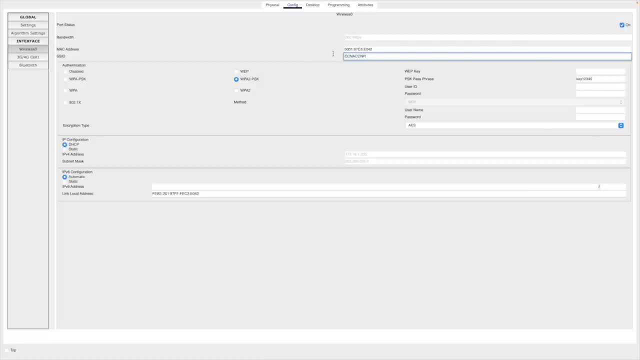 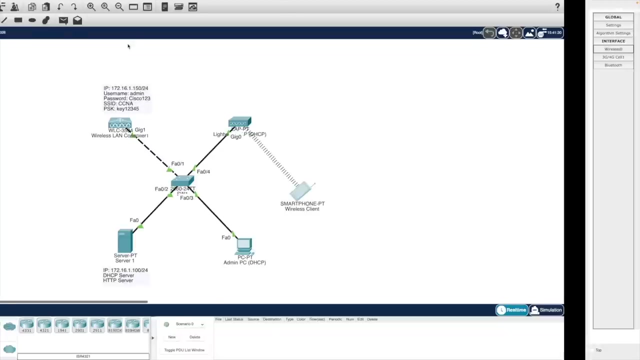 is not CCNA anymore, It's CCNP, And my password, my key phrase, is going to be CCNP P-C-C-I-E, And that should be applied now. Let's make sure it's stuck And let's go back to the phone. It's not connected right now. When it's connected, 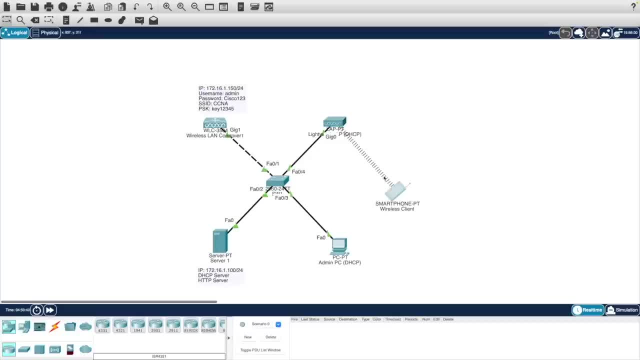 oh, now it is. It took a couple of seconds. I expected it to. When it's connected, we see these dashed lines. That shows that I've got connectivity. So that's what Cisco says you have to be able to do for the CCNA exam. 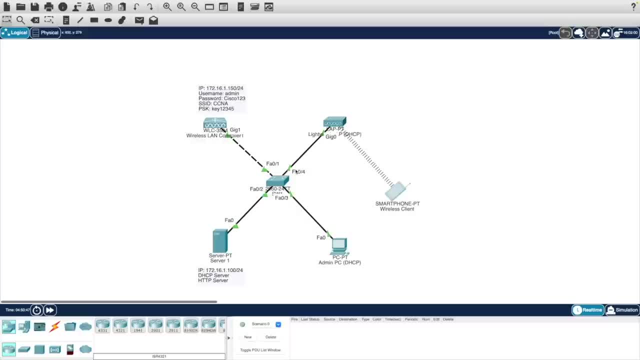 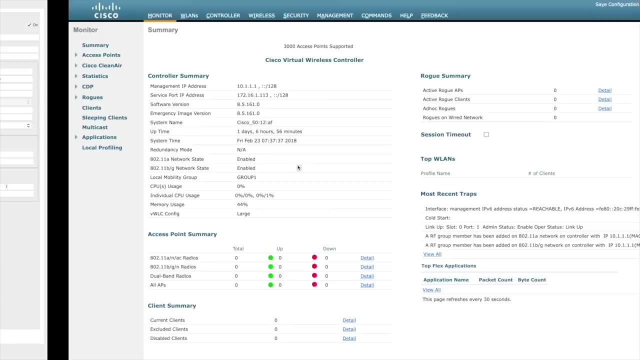 You need to be able to set up a new wireless network. Be sure to click Enable, Configure Layer 2 security for WPA2 and a pre-shared key. That's how you do it. It's that simple. Let's get back to our slides. There we go. There's our slides, And now let's get a little. 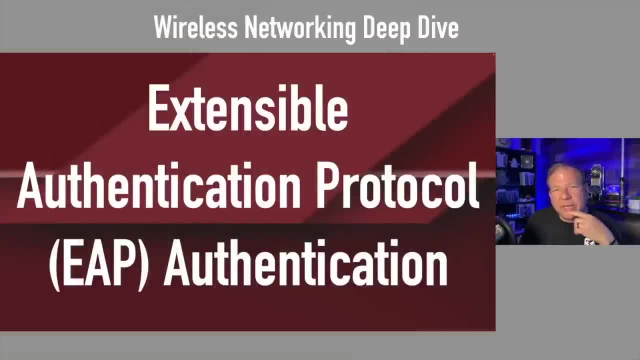 bit more in-depth. Let's take it beyond just pre-shared keys. Let's go into enterprise mode, where we have authentication off of like a radio or a radio server that's going to be handing out these session keys. The way the session keys are handed out can be done in a variety of ways. 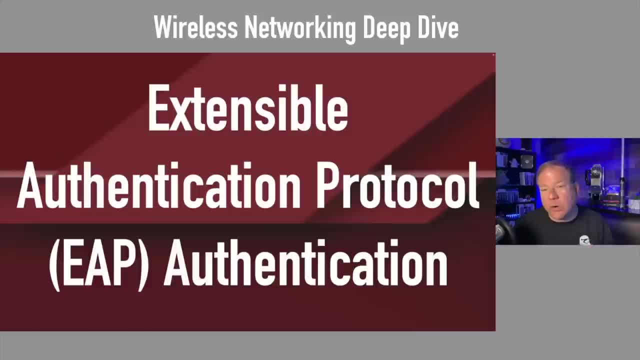 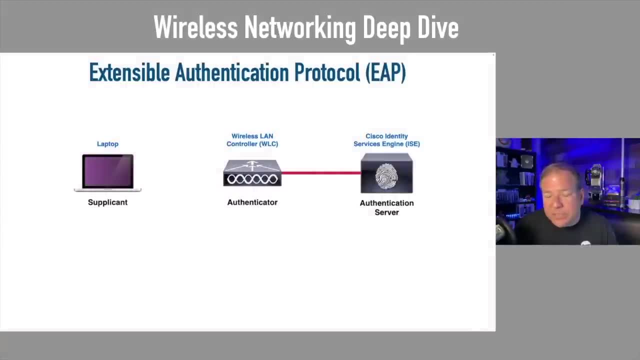 And the ways that that can happen are described with one term for your notes. It's called EAP- Extensible Authentication Protocol, Extensible Authentication Protocol. Now, this is not just used in wireless networks. You could have You could have a computer with a wired connection going into a Cisco Catalyst switch. 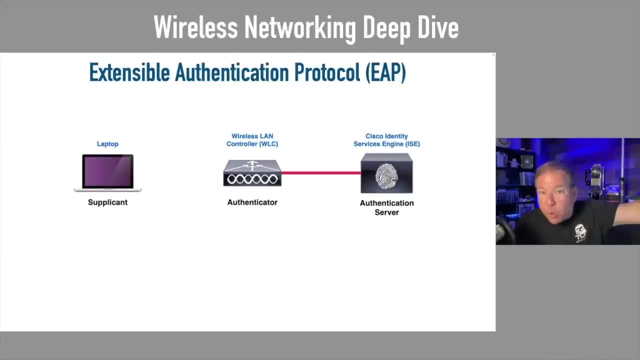 running 802.1X security, port-based security. It would use this as well. It's a way for us to say: I would like to access the network, Mr and Mrs Switch or Mr and Mrs Wireless LAN Controller. 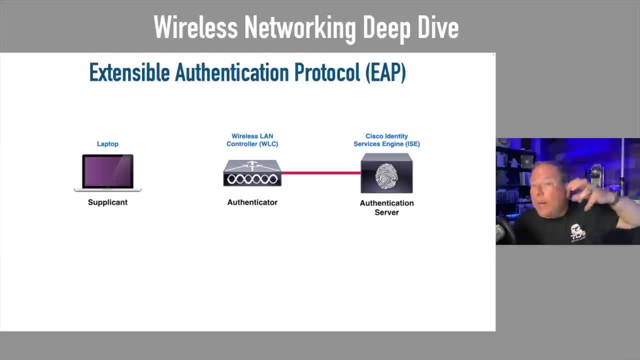 It's going to then take our request relay that request to an authentication network. It's going to then take our request relay that request to an authentication server like a RADIUS server or Cisco ICE, And if we pass that authentication process we'll be given a key to. 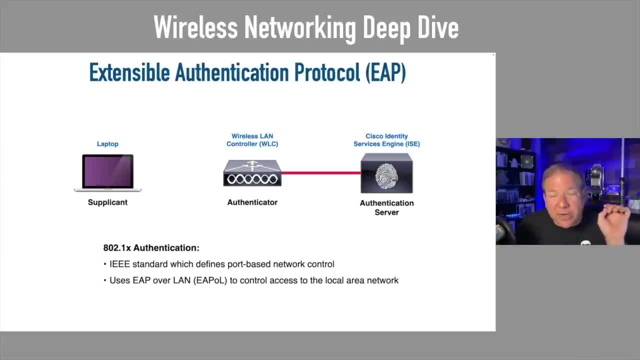 use. Again, this is called 802.1X authentication, not just for wireless. This applies to switched wired connections as well. And for your notes, I want you to know the three components that we have in a .1X network. Number one: we have a supplicant. 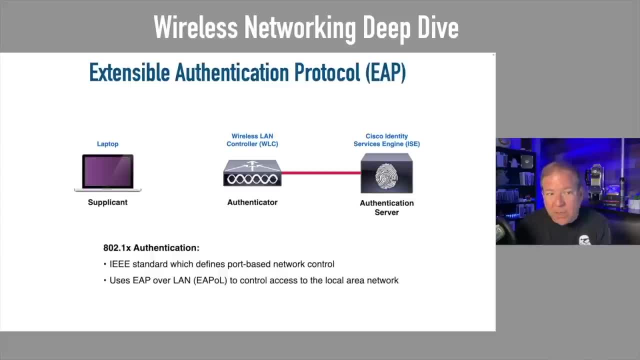 To supplicate means To ask something, So a supplicant is asking for access to the network. The authenticator could be an Ethernet switch in a wired environment, or it could be a wireless LAN controller in a wireless environment. Now I think the term authenticator is a bit misleading. 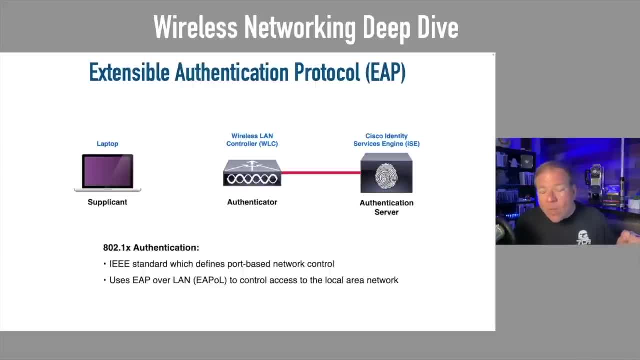 because it's not doing the authentication. I would prefer to call this a translator, because it's not doing the authentication. It's not doing the authentication. It's going to be translating those EAP messages into RADIUS messages as it goes over to the server. 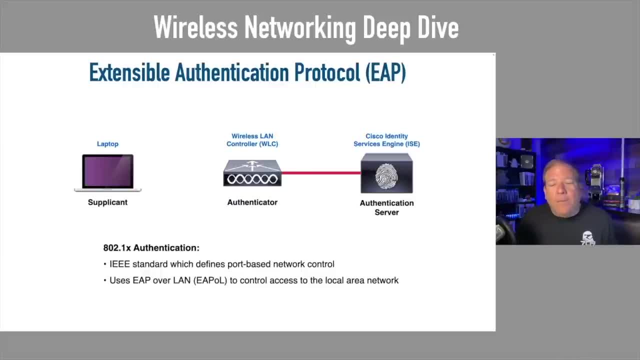 You'll see what I mean in a moment. But the third part of a .1X network is the authentication server. Again, it could be a RADIUS server, It could be the Cisco ICE or the Identity Services Engine server That's going to check our credentials. And here's kind of another breakdown. Those are the terms that 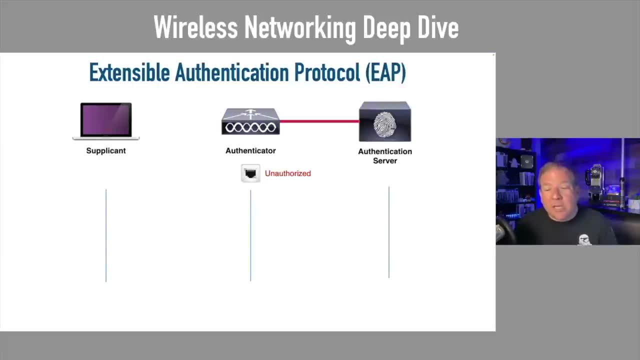 I just gave you. I want to go through the step-by-step process. So, whether I'm trying to connect to an access point or a physical port on an Ethernet switch, here's how it goes step-by-step. My supplicant, that's my. 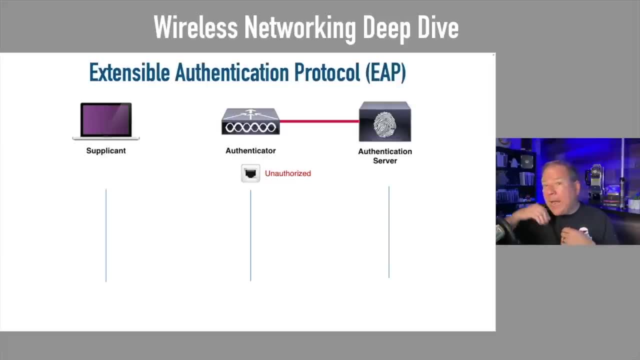 client. either it could say, hey, I want to get on the network. It could send that to the wireless LAN controller, Or on a switch, the switch could see that somebody just plugged into me. I'm going to ask them to authenticate. The point is, the initial message could be coming from the network. 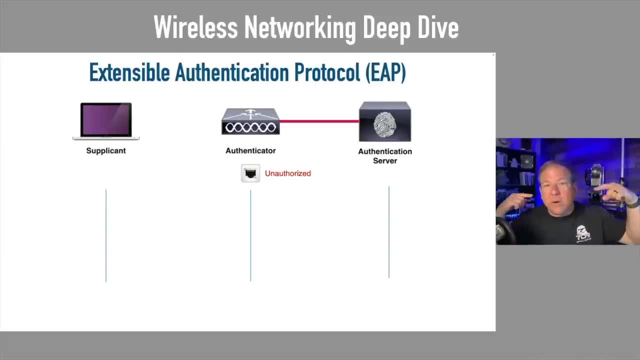 It could be coming from either the client or the supplicant or the authenticator. If the supplicant starts it, it's going to send what's called an EAP over LAN, an Extensible Authentication Protocol over LAN. start message saying: hey, I'd like to connect to the network And the authenticator. 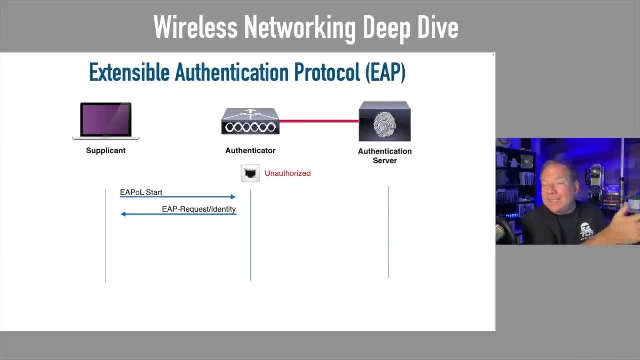 is going to then request the identity of this supplicant. Now, that start message might not have happened if we hadn't done that. So that's going to send an EAP over LAN, an Extensible Authentication Protocol over LAN, And the supplicant says, hey, I want to get on the network. 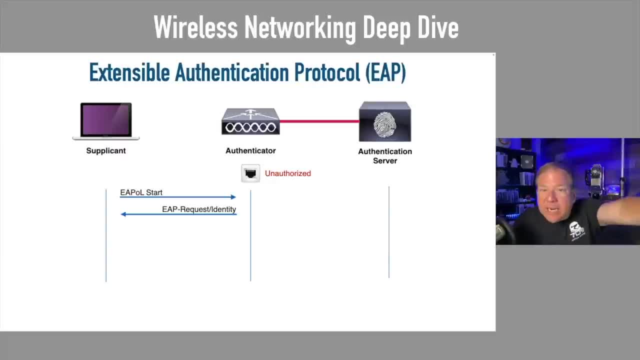 The switch would have seen that port go up and it would have immediately sent out that request identity message. But in the case of wireless, we send that EAP-OL start message And the supplicant says: oh okay, here's my identity, The authenticator which I said I would call the. 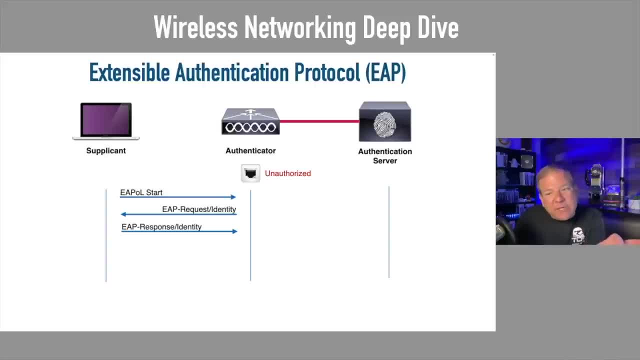 translator. it's going to translate that EAP message into a corresponding radius message and say: hey, I've got this computer over here that wants access to the network. So the radius server sends it a challenge message. To get access to the network, you need to provide whatever. 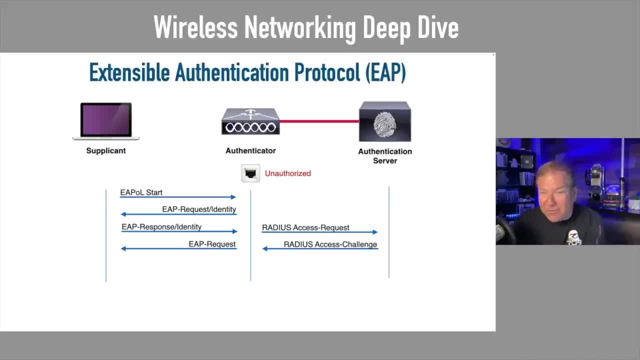 credentials. Well, the authenticator, or I would call it the translator, converts that into an EAP request message saying: hey, can you provide username and password information? we'll say, And that comes back in an EAP response which gets translated. 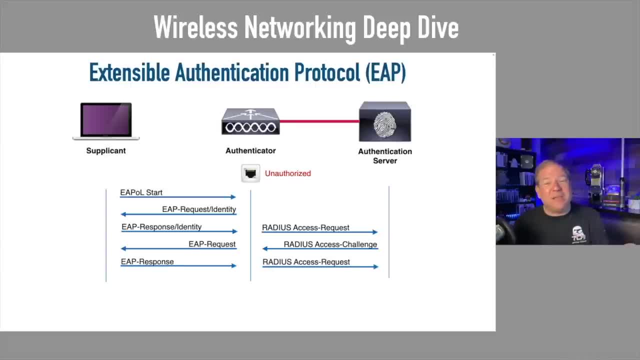 into a radius message Saying here's their response. The radius server or the I server will check that against their database and say yes or no. It'll either be an accept or a reject. Let's say it was successful. We send an accept message over to the authenticator which translates that into an EAP. 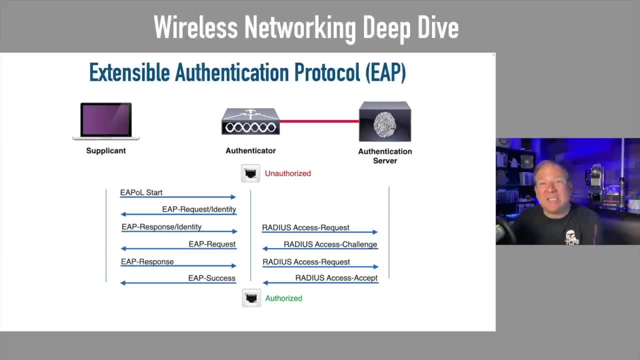 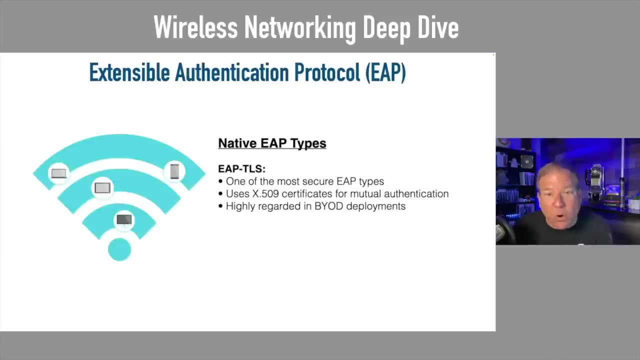 success message. So the supplicant now gets access. They are authorized to talk on the network. That is a generic way of explaining how EAP works. There are different flavors of EAP. For your notes, I want you to know there are two. 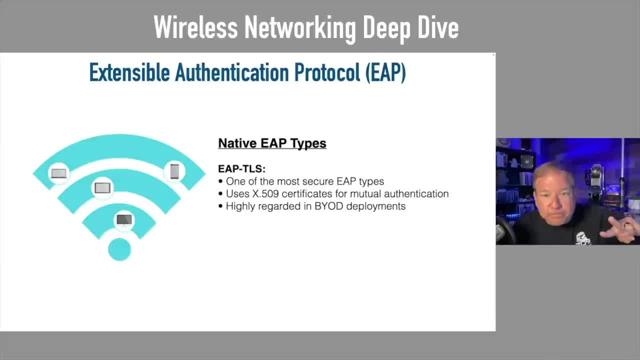 broad categories of EAP. There are native EAP types and there are tunneled EAP types. The tunneled EAP types is: think of that as a protective layer. It's an outer tunnel that's going to protect the other EAP. 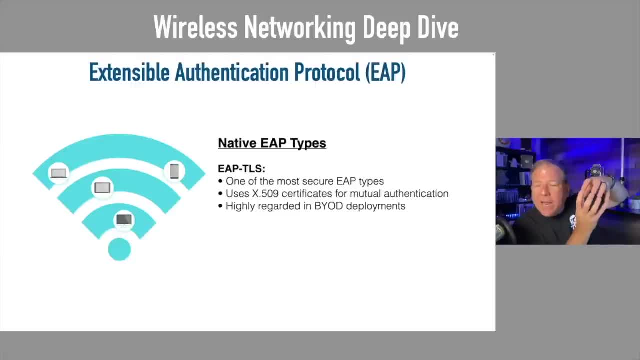 Sorry, could you say that again? Wow, Siri is very active today. It's going to protect the conversation going on by EAP inside of the tunnel, but it's going to protect the native EAP conversation. I'll show you a graphic of: 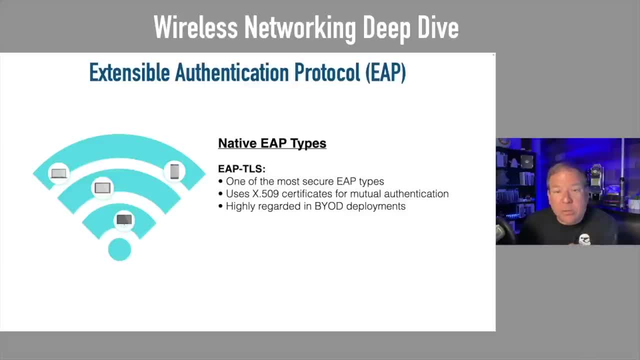 that in a moment, But one of the original and most secure native EAP types is called EAP TLS. It uses transport layer security- Very secure. It does require that you have a digital certificate, though, which means you have to have a certificate. It's a lot to set up. We'll say that. 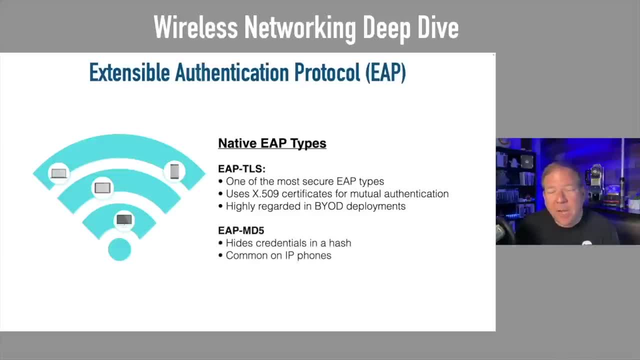 But in an enterprise it's probably worth the setup. Another option that's not as rigorous to set up is called EAP MD5.. Now MD5, Message Digest 5, that's a hashing algorithm. It's going to send the password, not as an encrypted 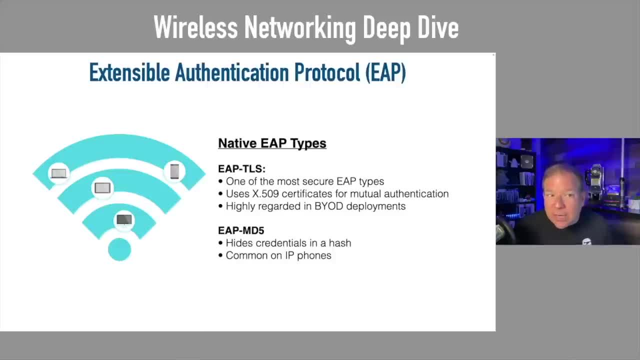 string. It's going to send it as a hash, kind of like a fingerprint. So if both sides have the password and they both create the same hash, then yeah, it was probably the same password. You see this oftentimes on Cisco IP phones. So if you do, join me for the collaboration training. 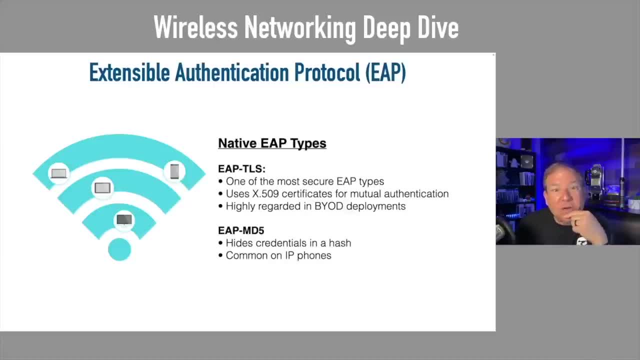 that we talked about our CO core course. yeah, we talk about that. Another EAP type Microsoft developed and it's called EAP MSCHAP- Microsoft Challenge Handshake Authentication Protocol, Version 2.. Why would we want this thing from Microsoft? Well, Microsoft has the most. 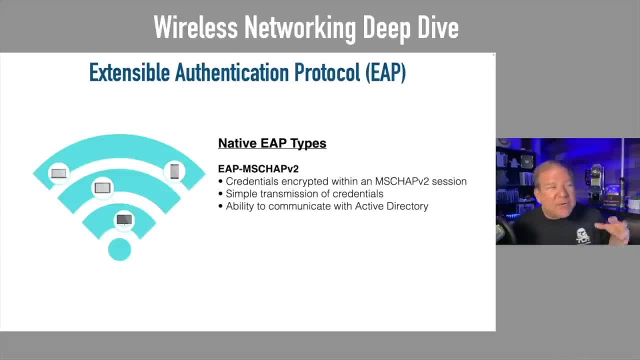 directory out there today, And by directory I mean a shared user database. It's called Active Directory. Microsoft Active Directory is the most popular type of LDAP service we have. LDAP is Lightweight Directory Access Protocol. It's like a database of usernames and passwords, So we can 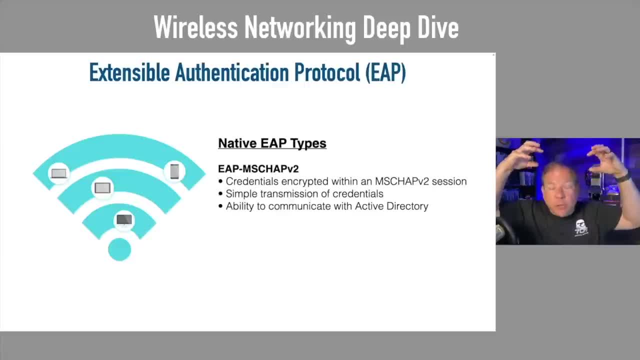 have multiple devices authenticate against a common user database. Everybody doesn't have to maintain their own user database. So Microsoft says: oh, you're authenticating with the network. Why don't you use this existing Active Directory service that everybody else is using for authentication? So if you're a Microsoft, 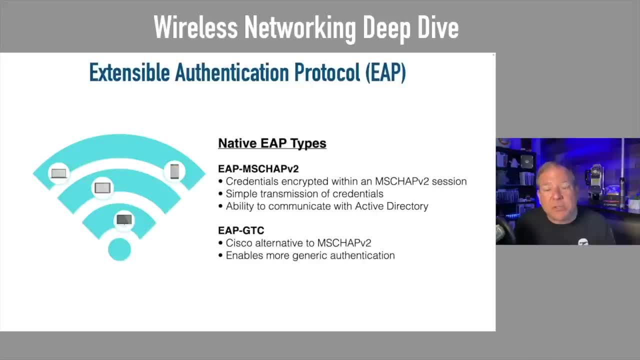 environment. yeah, that might make sense to use EAP MSCHAP version 2.. Cisco came along and said: not everybody uses Microsoft, Let's create something a little bit more generic. So Cisco came out with something called EAP GTC for generic token card. That's going to be able. 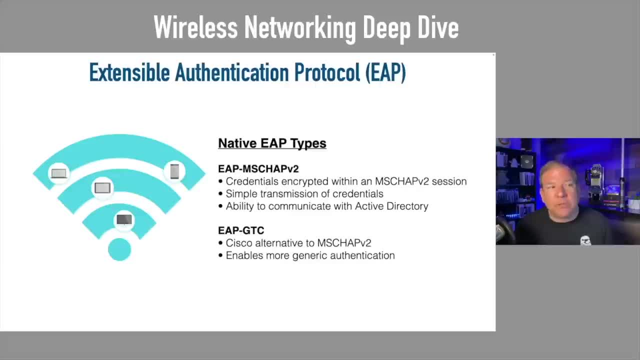 to use more generic authentication, where you might be able to use EAP, GTC for generic token card. A generic LDAP server doesn't have to be Active Directory. Somebody's saying MD5 is really unsecure, isn't it? There's a couple of hashing algorithms out there. 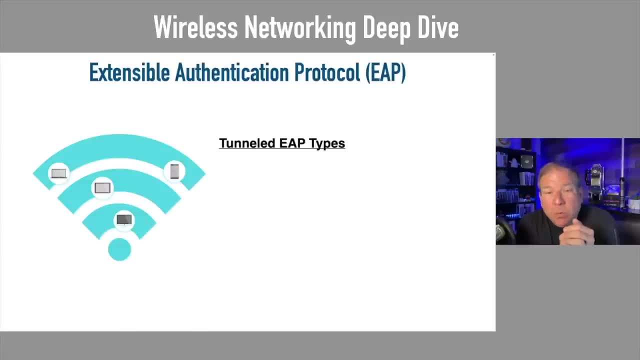 that are fairly popular. MD5 is one of them. The other is SHA Secure Hash Algorithm. Of the two, you're right, MD5 is the lesser secure of those. It's subject to brute force attacks. In general for IP phones it's considered secure enough. for what we're doing with just. 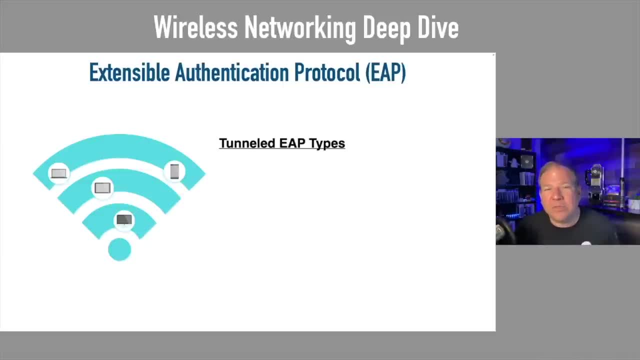 authenticating the phone with the Cisco Communications Manager server. But if you've got strong passwords, MD5 can be very robust if you have strong passwords, If you have a three-letter password- I've done this. We used to break for fun in class when I taught security. we would 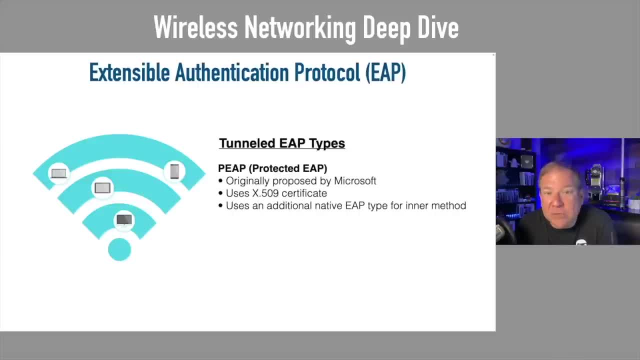 break MD5 hashes No less than two seconds. But those were with very weak passwords. If you have strong passwords it could take years. So it really comes down to the password. but great point Now, those were the native EAP types. If you want to use them by yourself, by themselves, 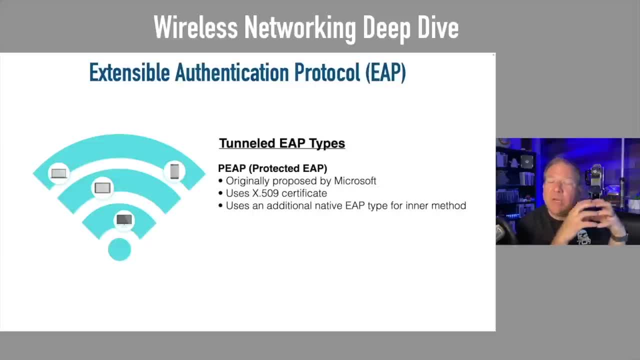 feel free, you can do that. But if you want that communication to be protected by an outer shell, you can have a tunnel that you send those EAP conversations through. And there's this tunnel EAP type- that you can use to send those EAP conversations through. And there's this tunnel. 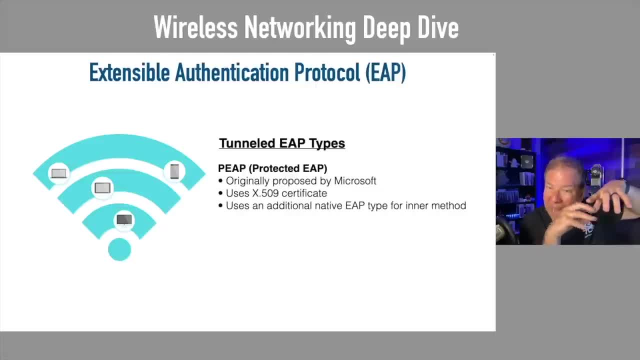 EAP type that you can use to send those EAP conversations through. And there's this tunnel EAP type that will encapsulate, it will envelop your native EAP type And one of those is called PEEP protected EAP. This is something else that Microsoft proposed. Again, it requires a digital 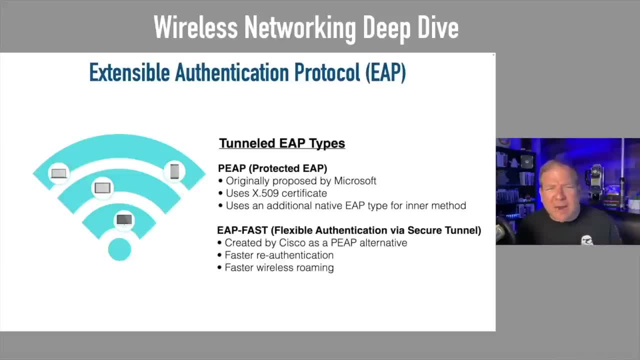 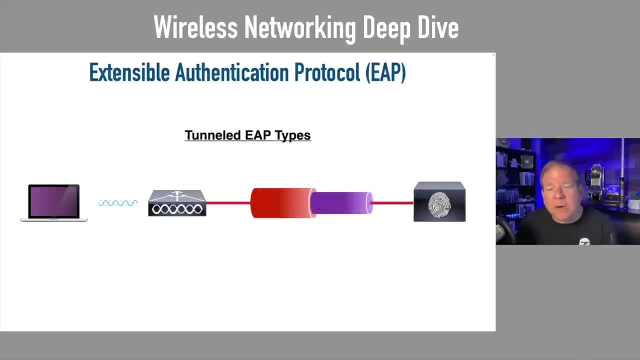 certificate, Cisco's alternative. apparently, whenever Microsoft comes up with something, Cisco says: oh no, we can do better than that. That's not Microsoft specific. So Cisco came out with EAP fast. That's another tunnel, EAP. But here's a great visual of what I'm trying to describe here: The purple tunnel that you see. 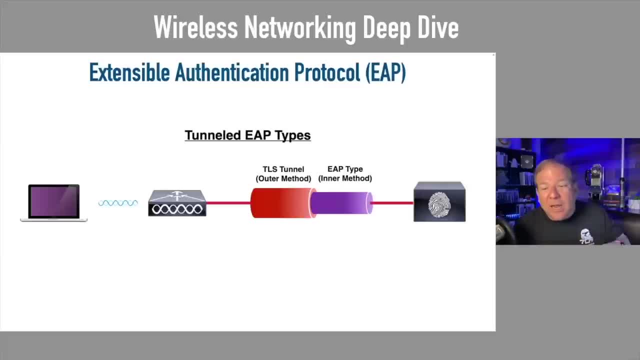 that's where your native EAP types are. That's your inner method. Protecting that inner method is the outer method. Those are your tunneled EAP types, And the examples we gave you of tunnel EAP types included PEEP and EAP fast, The native EAP types that can flow inside of the tunnel. 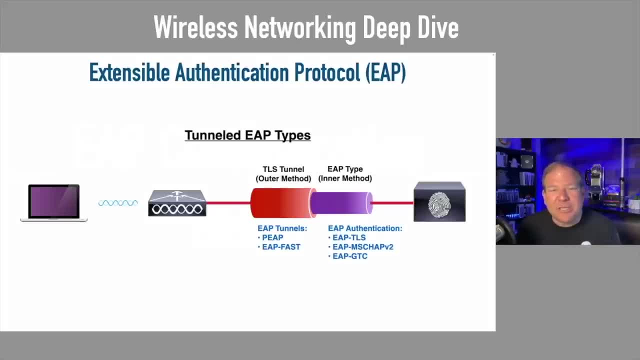 are EAP TLS, EAP MSCHAP and EAP GTC generic token card. Now let me explain this a little bit. So let's start with the EAP token card. Let me I'll make this full screen again for you. 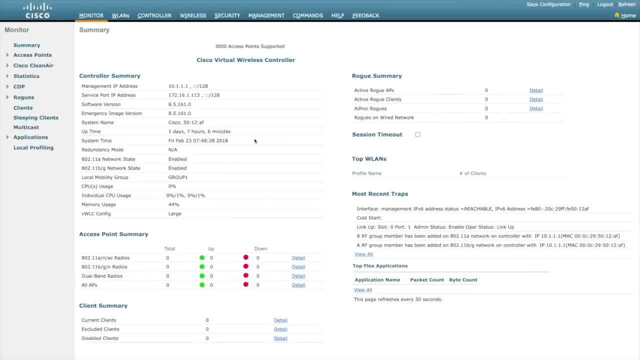 So you can see this, And I'm going to go out to that 60-day evaluation wireless sync controller that I told you about And let me show you how we can set up EAP, something that Cisco says you need to know how to do for the Encore exam. 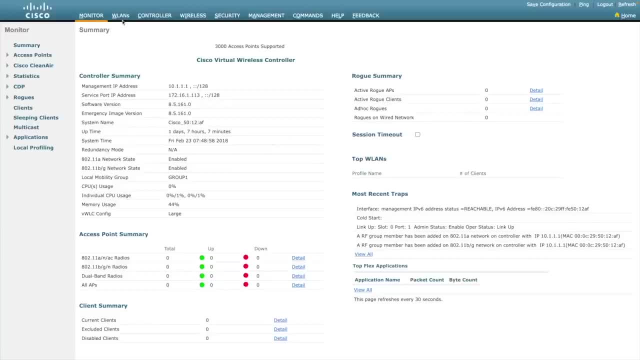 So here we're sitting on this virtualized, fully functional wireless sync controller, And I actually don't have a RADIUS server. I just want to show you how we would point to a RADIUS server if we had one. But here's how we would do it. We would go to the security tab up top here. 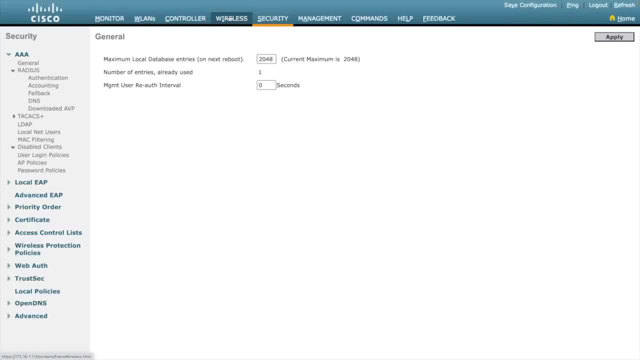 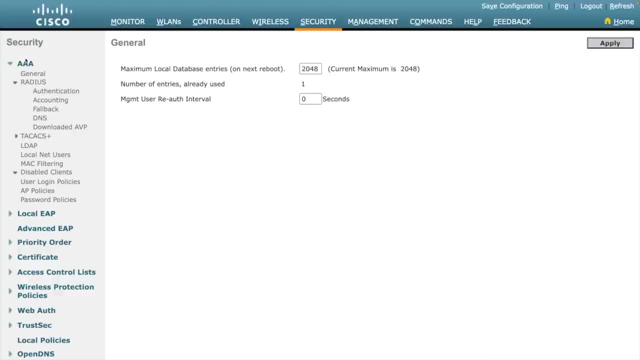 In fact, can I make this a little bit larger? Yeah, that made it a little bit, trying to make it easier to read for you, So that makes it a little bit larger. I'm going under the security tab And then under AAA. RADIUS is a AAA server, That's. 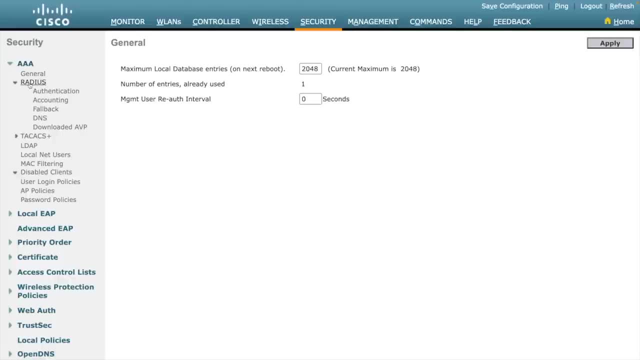 authentication, authorization and accounting. I'm going to go under RADIUS, And then I'm going to go under authentication, And right now, you see, I don't have any RADIUS servers. So I'll say: I want to create a new RADIUS server. Now again, I don't really have one, But let's pretend that I have one. 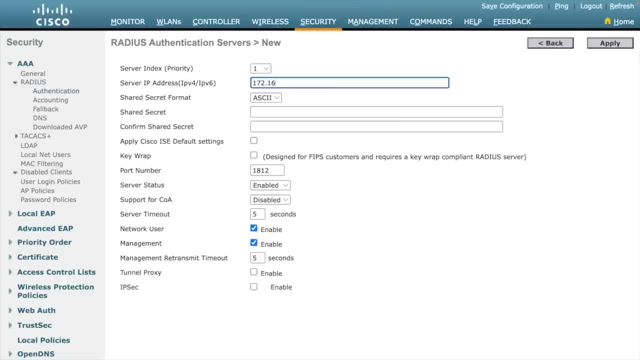 at an IP address of 172.16.1.223.. And I'll give it a shared secret password And I'll just make it Cisco. Now I'm going to leave all these at their default settings. I will mention this one. You want to make sure that the server status is set to enable It should. 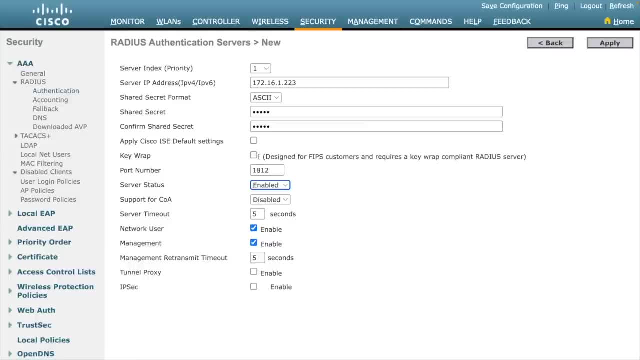 be by default, but it's not going to work. if it's not, I'll mention this one as well: key wrap. I'm not going to do that, But the key wrap option means that the key it's going to be protected. 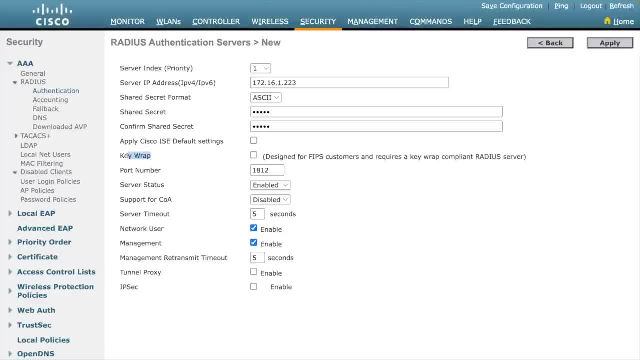 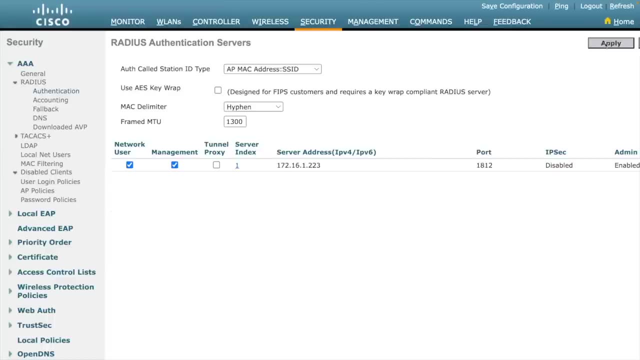 with AES encryption. But I'm just going to leave it disabled, keep everything nice and simple here And I'll say apply. So we've now defined a RADIUS server. Okay, how do I now tell wireless LANs to use a RADIUS server? Let's go over to our wireless LANs. I'll say WLANs. 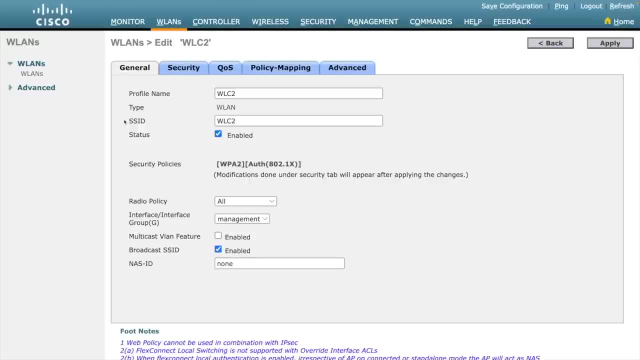 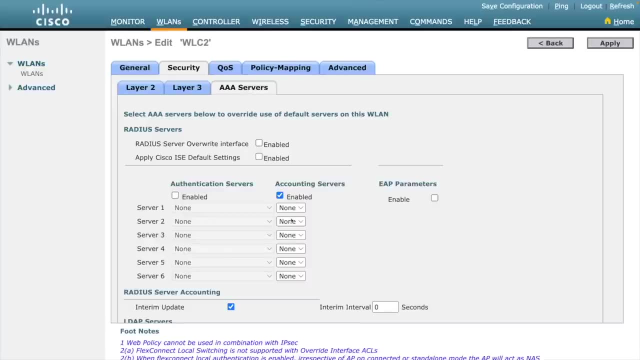 And I've got one created here And under the security tab I'm going to go under AAA servers. Now, right now we don't have any assigned. I'm going to say I want to enable my authentication servers And the server that I just created shows up here. 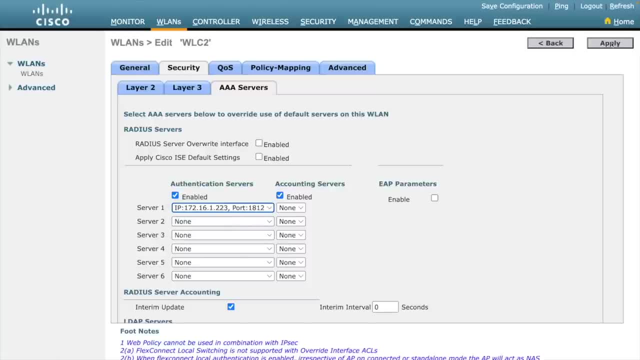 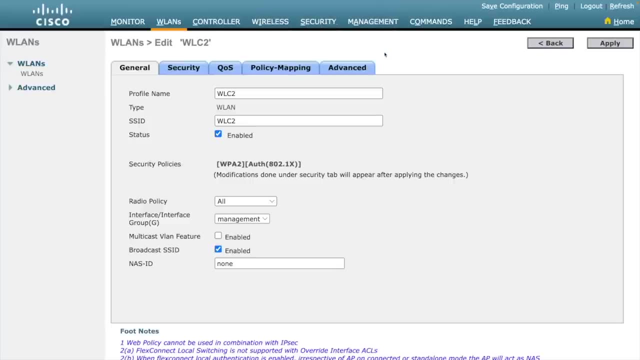 So I'll say WLANs And I'm going to go under AAA servers And I'm going to go under AAA servers And I'll select that And I'll say apply. It's that easy to tell a wireless access. well, to tell all the wireless access points, because I just configured it on the wireless. 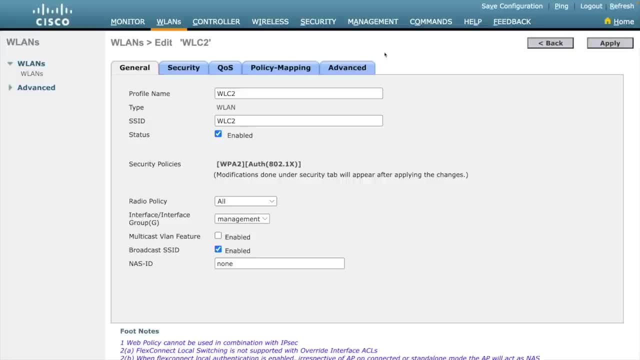 LAN controller. I just told all the wireless access points. hey, I want you to go check authentication against this RADIUS server. Let me show you another option while we're out here, though Maybe. oh you know what, I didn't specify the EAP type. I should do that. 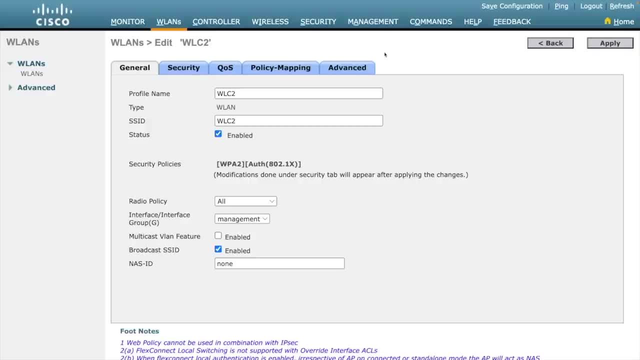 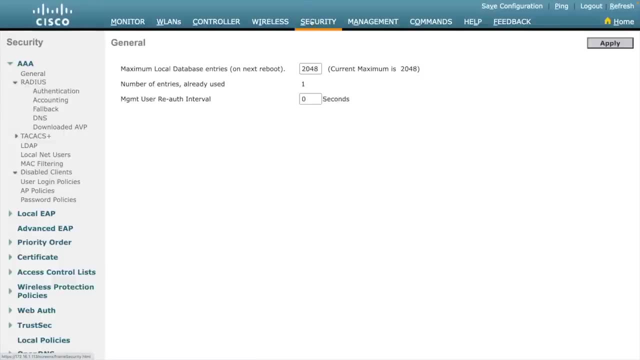 Yeah, let's do that. Let's say that we're going to use a specific type of EAP, So let's go back under security And let's use trying to. Yeah, I'll tell you what. let's do a. let's set up a local database where we're not using a RADIUS server. So I've said: 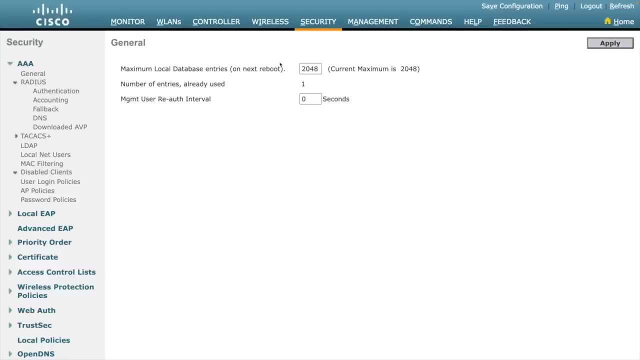 here's how you point to the RADIUS server. Let me show you how we would point to a local user database using local EAP. So I'm going to go to the security tab And I'm going to go into the local EAP that you see right there. I'm going to go under profiles And I don't have one right. 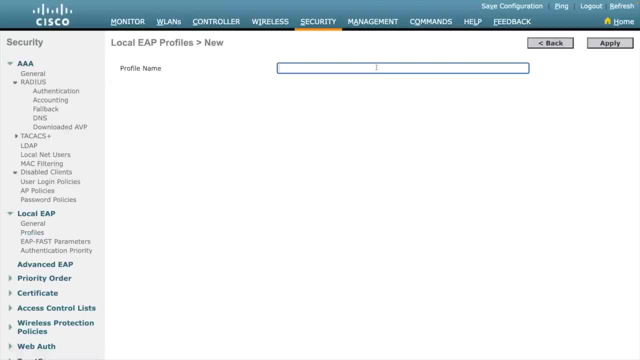 now. So I'm going to create a new EAP profile. This is what flavor of EAP that we just talked about am I going to use? Okay, I'll say I'm going to use. just make a name, I'll just call it local. 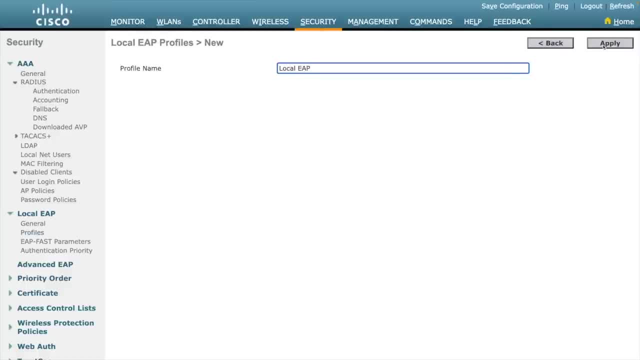 EAP, Not too imaginative, But I'll apply that. And oh, it doesn't allow spaces. I'll say local, no space EAP. And it allows me to select what I want to use. I'll use choose EAP, TLS- we talked about that one. 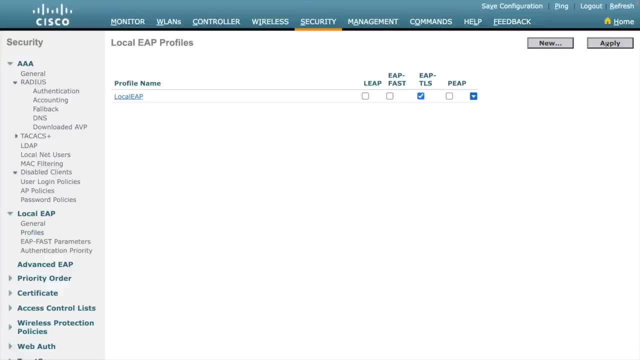 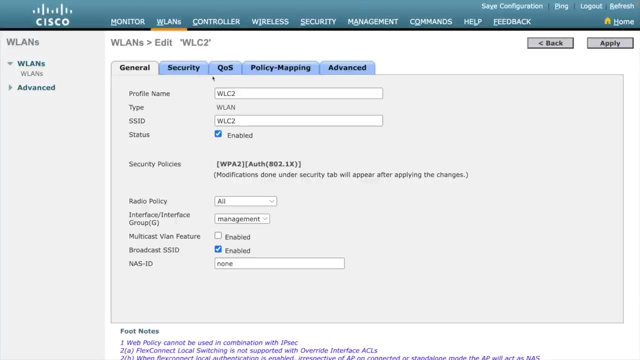 And I'll say: apply. So now we've got this EAP profile, Now let's go apply that to our wireless lane controller. Before I said: use this RADIUS server. So let's go back under security, back under AAA, And I'm going to get rid of this RADIUS server And I'm going to go back under security. 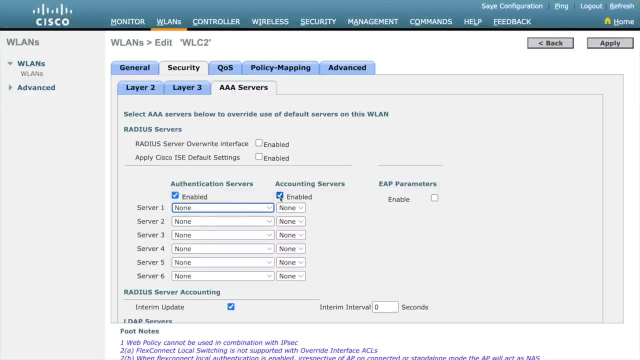 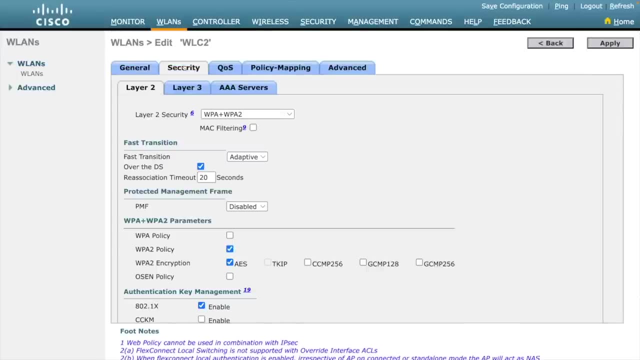 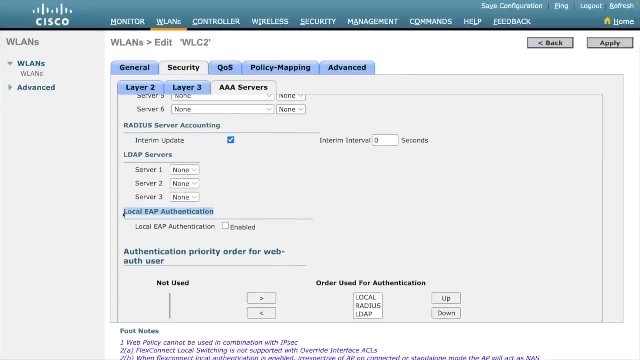 This server that I specified a moment ago. So I've got none. I'll apply that. So back under security, AAA servers: none. But if I scroll down notice, I can specify local EAP authentication. I'm going to enable that. It says: what profile do you want to use? 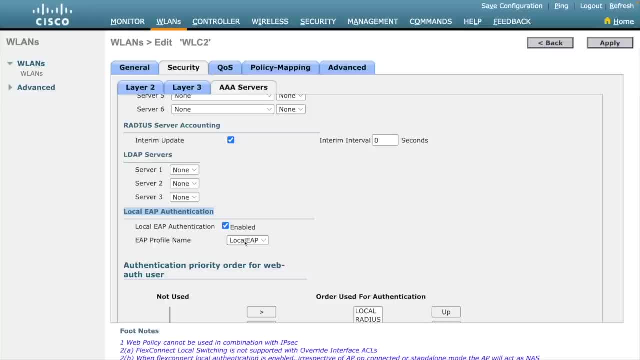 Here's the one I just created. It's automatically populated. for me It's called local EAP. So I'm done, I can say apply And it. now I'm going to go back under security And I'm going to go back. 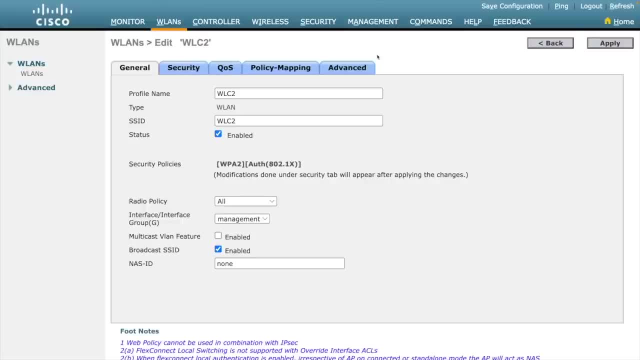 into security And it now says: all right, in order to get a session key, you're going to have to authenticate against a local database, And the type of EAP we're going to use is I forget. what I picked now was no, it was EAP TLS. That's what I picked, But in order to authenticate locally, 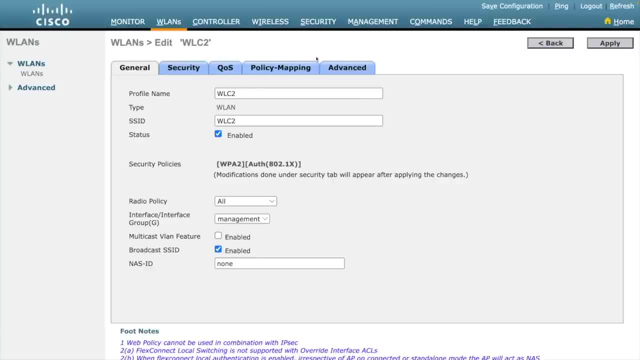 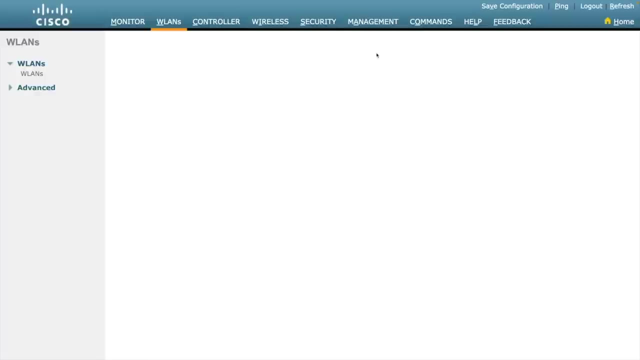 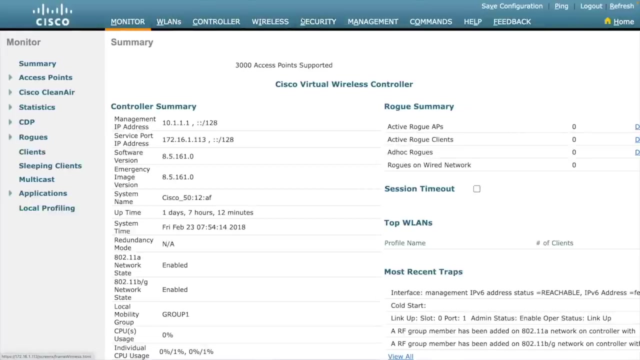 I need to create a user database. How do I do that? Well, to create a local user database. let's go back to where is it? Oh, I'm going to say apply. Let's go back to security. That's what I was looking for. 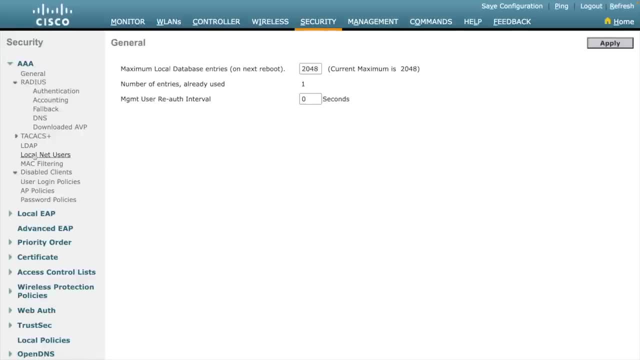 Go back to security And I'm looking for local net users. So I'll say new. I'll say I've got a username of, we'll say K Wallace, I'll give a password of Cisco. I'll confirm the password of Cisco. I'll allow myself to connect to any profile And I'll just 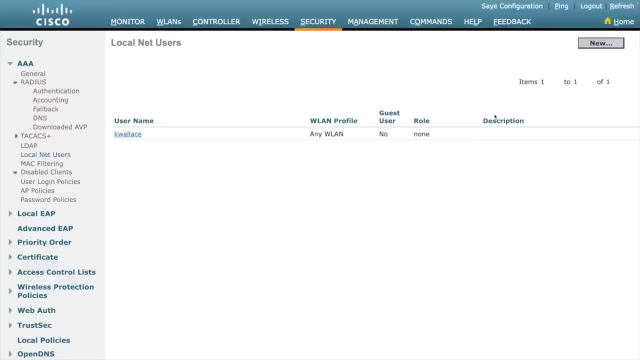 say apply. So here's what's happening now. If I tried to authenticate to an access point, if I tried to authenticate using this wireless LAN controller, it would say: hold on, we're going to use that EAP TLS method And we're going to check you against this local user database. 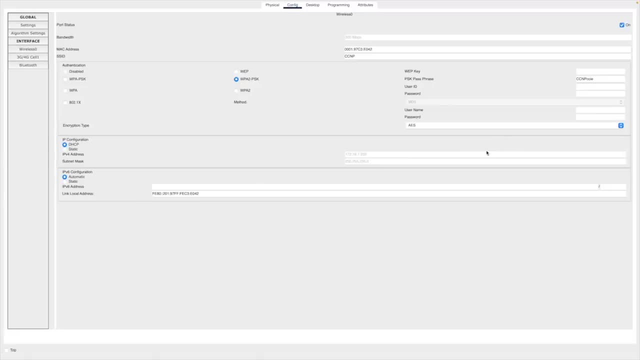 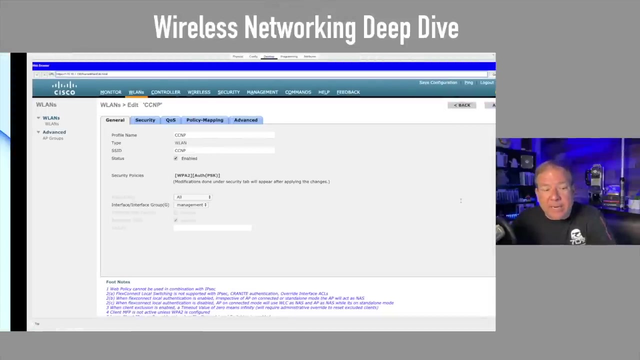 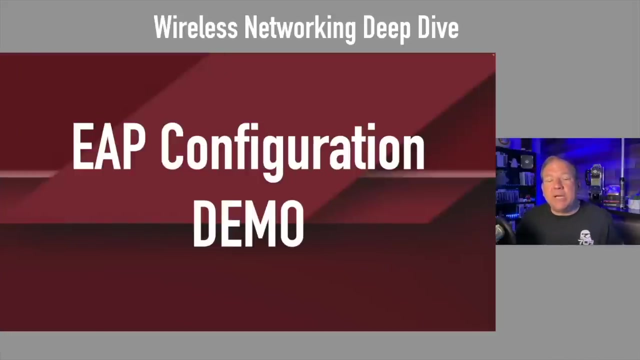 which I just created. So that's a look at. really, that's a look at two different ways of setting up EAP. We did it using a RADIUS server And we did it using- let me find our slides again. There we go. And we did it using a local database. So a couple of ways of setting up EAP. 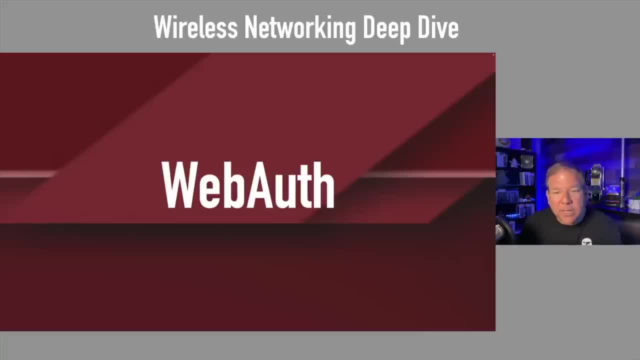 Another way that we could authenticate with an access point is- and you might have seen this in a hotel- where you're getting on their wireless network and you have to agree to their acceptable use policies. You might have to put in your last name and your. 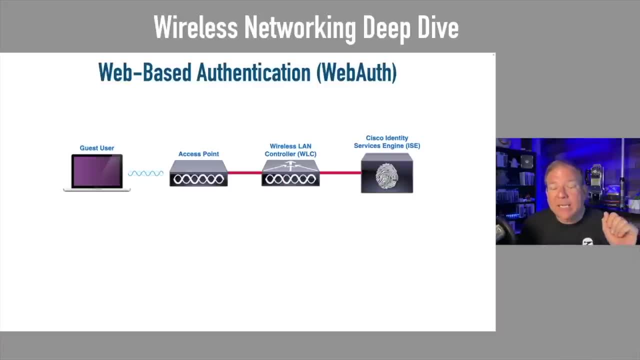 your room number. perhaps You might have seen something like that. It's called WebAuth Here. we don't have to have any sort of client software that's going to be doing authentication with the RADIUS server. We can just open up a browser and authenticate directly through a. 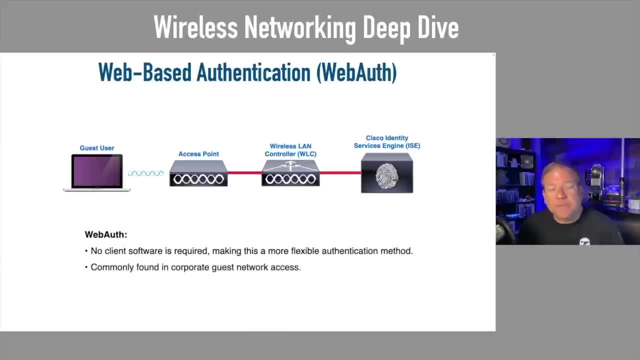 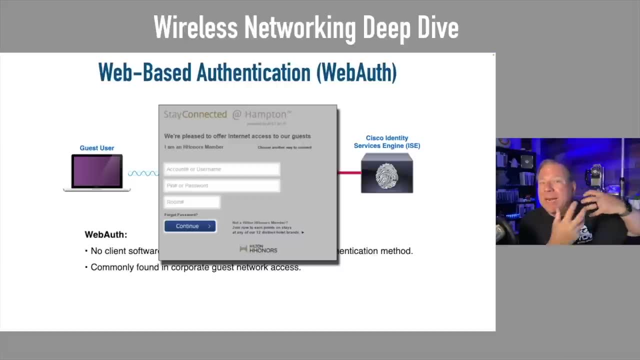 browser. It's going to make it a lot more flexible for the users. This is oftentimes used for guest access. So somebody, you can force somebody getting on the network through your access point. You can force them to a webpage where they have to say: 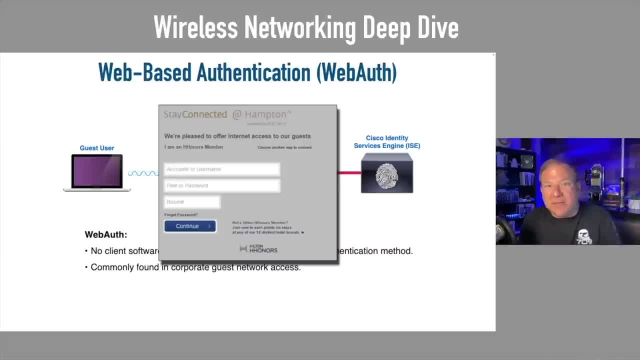 yes, I agree to all these policies. So if they do something in violation, you can say: you agreed. you're going to be in trouble now. You applied to all these policies or you agreed to all these policies. Here we have an example from Hampton Inn. 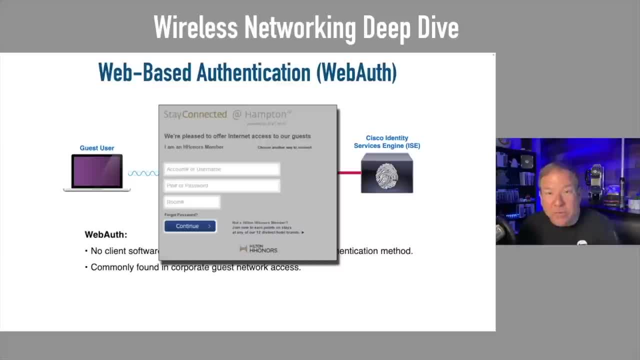 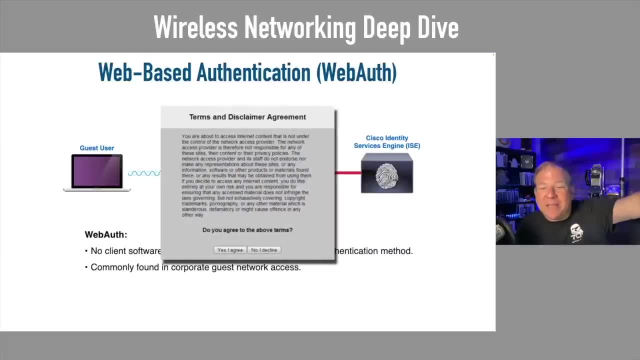 where they might say: hey, what's your username, Here's the password that we gave you at the front desk And here's your room number. All that matches up. You get on the network, but then, instead of getting directly out to the internet, they might make you agree to this. terms of use. 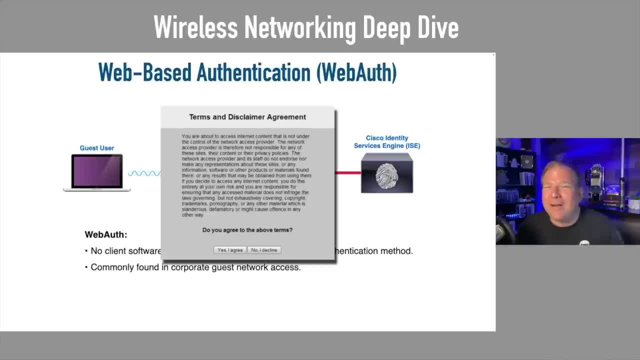 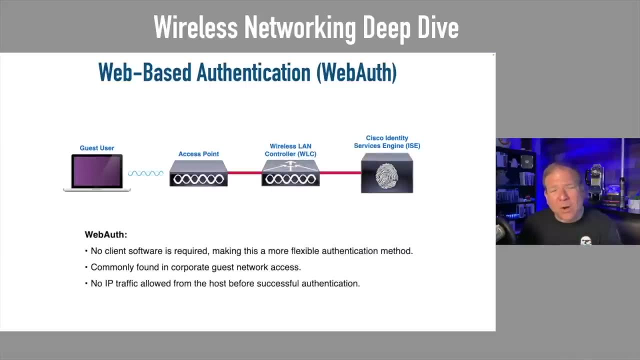 So people don't go in a hotel and carry on bad, illegal activities on the web, for example. So how does this work? It looks like I'm talking to the network in order to be able to get these webpages coming back to me, But at the 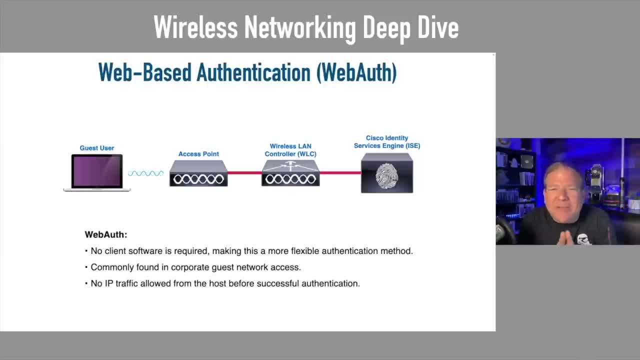 same time, I cannot get anywhere. I want to. The only IP traffic I can get on the network is for authentication purposes, And that's called web auth, And there's a couple of ways of doing this. We could have our centralized radius database with all of our users if we wanted to do it that way. 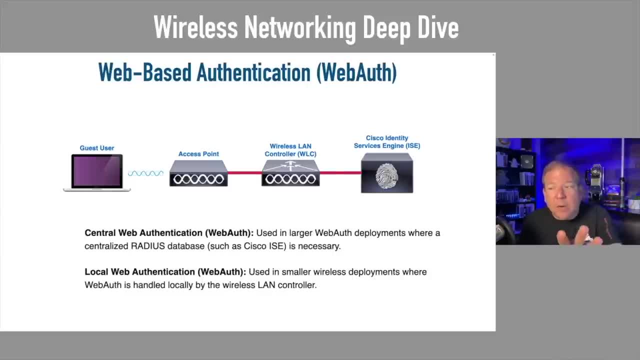 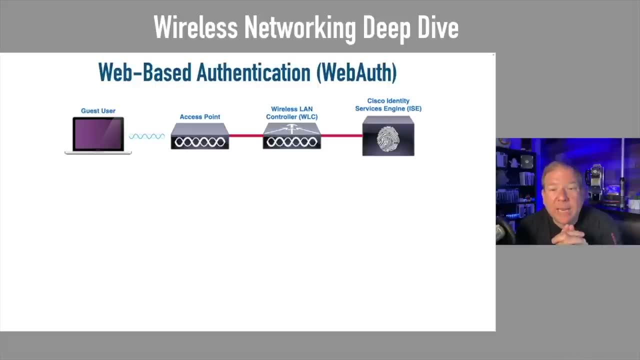 But oftentimes in smaller environments, we could have local web auth. This is where we could have a local user database, like we just set up on the wireless LAN controller, and somebody could authenticate. In fact, I'll show you how we can create the splash page that you would get to. 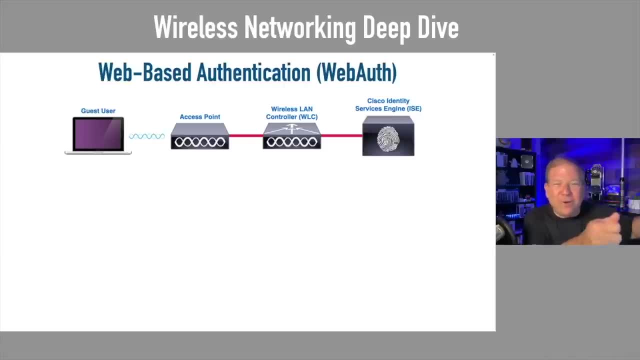 when you connect to- maybe- a hotel's access point. That's the way it works. The guest connects to XYZ Hotel's access point. It doesn't have a lock next to it. It looks like you don't have to have a password, But when you connect to the access, 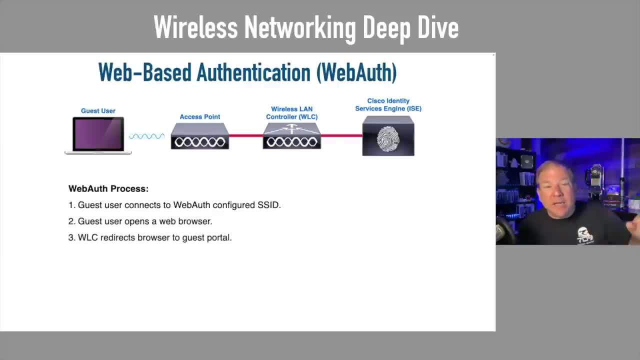 point and you open up your browser, you're immediately redirected to their guest portal where it might be asking you for your room number, your name, things like that. You're going to give your credentials. That's going to be checked against some sort of server, maybe a radius server. 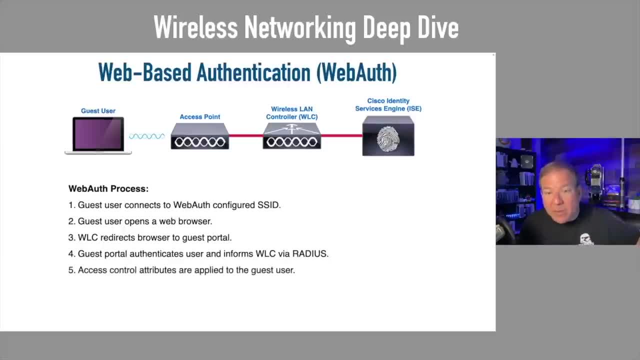 Maybe it's going to be a local database inside the wireless LAN controller And you're going to get policies applied to you that are going to limit you as a guest user. You're probably not going to be able to browse the printers in the back office, So you're going to be given a set of permissions. 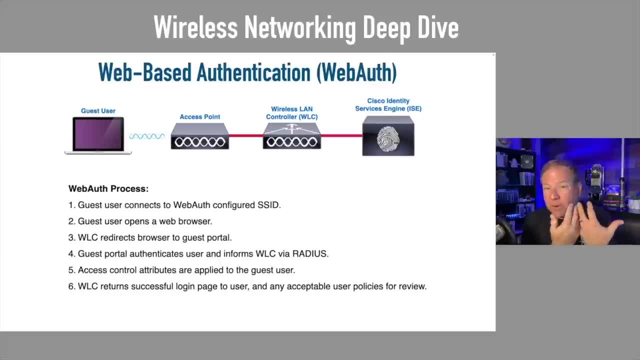 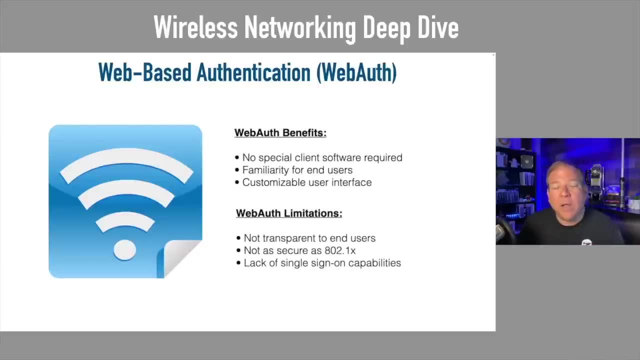 And then, if you give appropriate credentials, you might be asked to agree to their acceptable use policies And then you're going to be able to navigate on the network. The benefits of this: you don't have to have any software installed, You just go to. 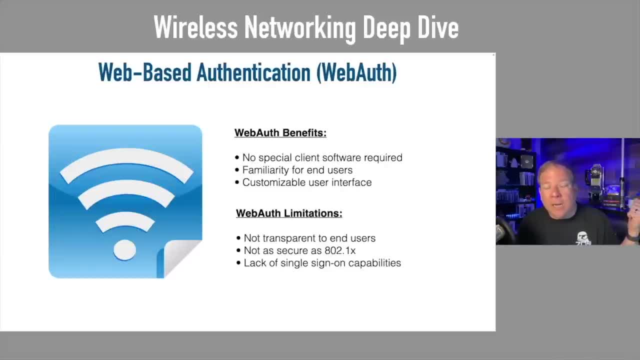 a browser, And it's something that a lot of users are familiar with because they've used it in coffee shops or hotels or airports, And we, as administrators, we can customize the interface, In fact, what a lot of hotels do. they will redirect you to their hotel page, So as soon. 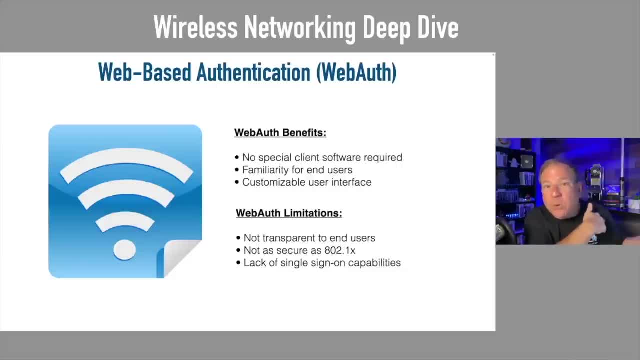 as you get on the network, even though you're trying to go check sports scores on ESPN, you're redirected to the hotel page of all their services and restaurants where you can make reservations. So it gives you information that they want you to receive And then you can go to wherever you want it to go. On the downside, it's not as secure. 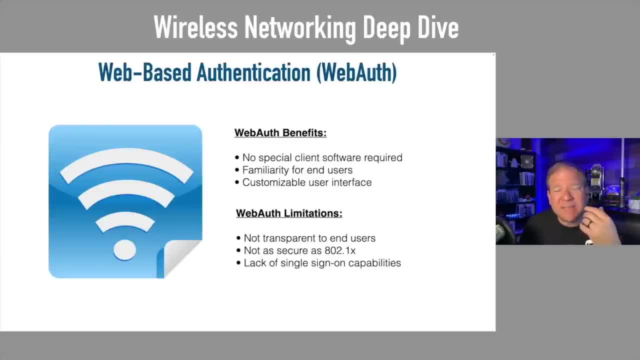 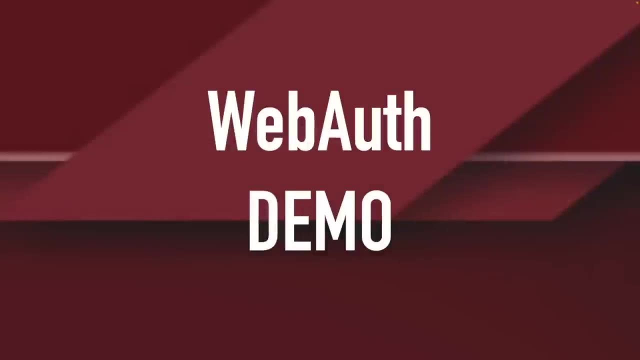 as using EAP and 802.1X, But it's easier for the user in some cases. I want to show you how to set that up. I'll go full screen again so you can see it, But let me show you how to set up WebAuth. 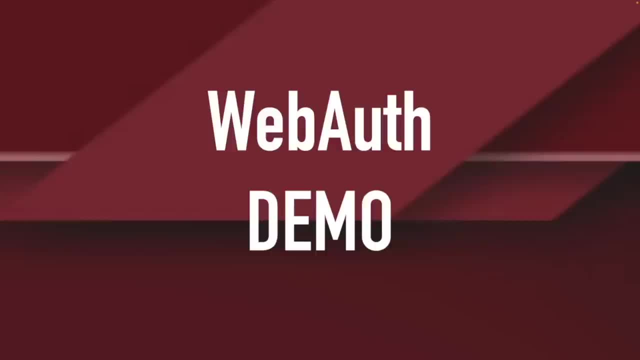 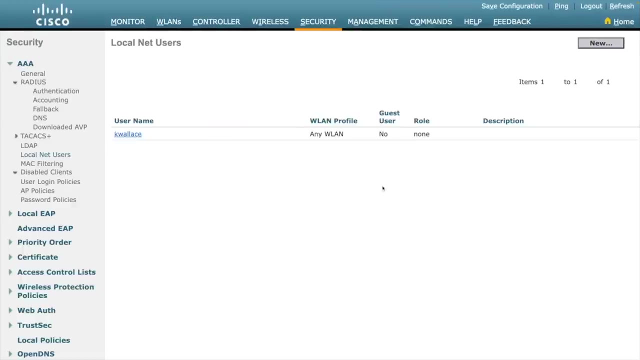 Let's show you how to do WebAuth using that existing local user database that we already set up. So when you say, if you're thinking where are the users coming from, We've already set that up. So let's go back into our. let's go back into our virtualized wireless hand controller. 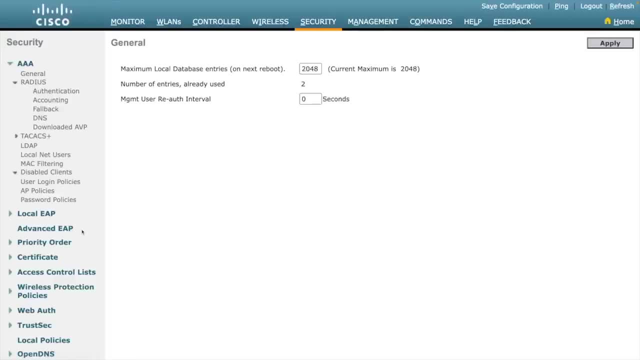 We're going to go to security And on the right hand or left hand side- here there's an option for security. So we're going to go to security And on the right hand or left hand side- here there's an option for security. 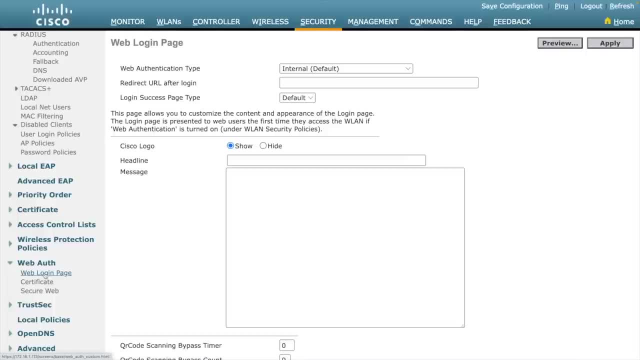 So I'm going to go to the web auth- You see this- and I want to go to the web auth login page. So when somebody connects, we're going to say: here's what we're going to, here's where we're going to send them. Now we could authenticate them internally using the local user database. 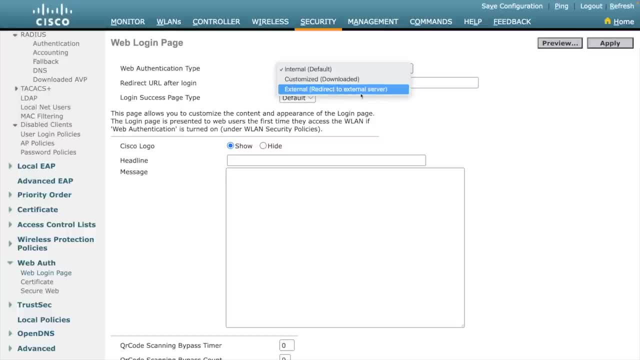 which we've already created. We could send them to an external server, like a RADIUS server. Oh, and we could include the Cisco logo or not. In fact, I'll show you the Cisco logo, I'll show you what it looks like, then I'll take it away. But for the headline, let's say we're connecting to the. 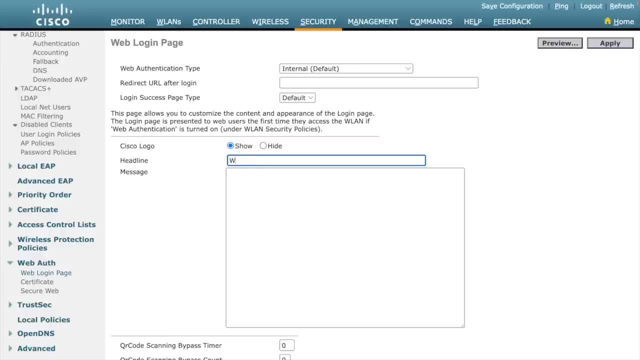 to the kw train network. i could say something like welcome to the kw train capital t train network. and then i can give a message. i could say: please read and agree to our acceptable use policies and i can apply that we could say preview to see what that would look like. 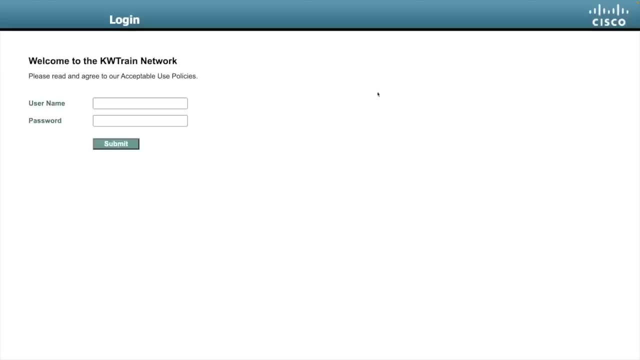 what would that splash page look like? this is what the user would see when they when they connected. they would see the cisco logo in the upper right hand corner, they would see our message and they would be asked for the username and password. let me just show you what it looks like. if i say hide, 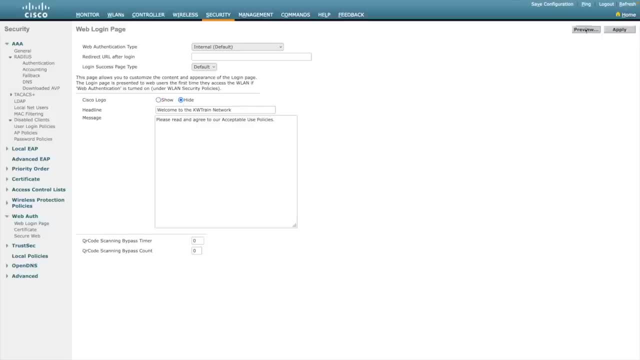 that if i hide the cisco log, uh, login and say preview it's, it's no longer there, as you can see. all right, perfect, now we've- uh, we've got the login page created. how do we tell our wireless controller to use this? well, let's go back under our wireless land. we'll go back under wireless land one. 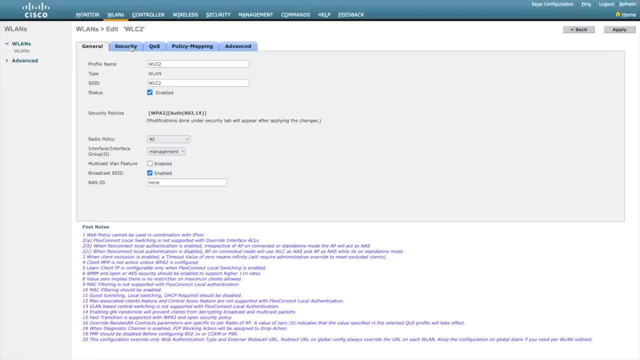 and we're going to go to security and for layer 2 security. i'm really not using layer 2 security at all. i'm going to say none right here and i'll apply that web auth is actually layer 3 security, so i'm going to go under layer 3 security and for layer 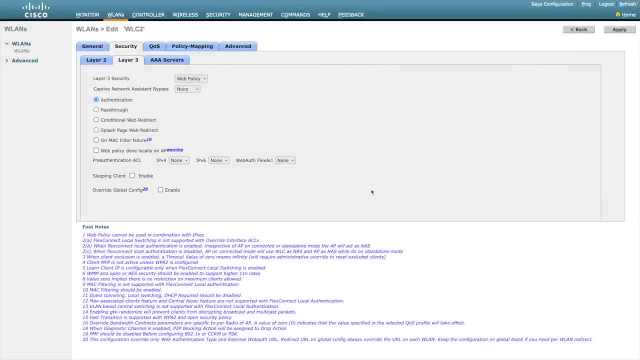 3: security. i'm going to say i want to use a web policy and there's a bunch of stuff we could configure here. i'm going to just leave everything at the default and i could say i want to go to a certain splash page to redirect once i get logged in. 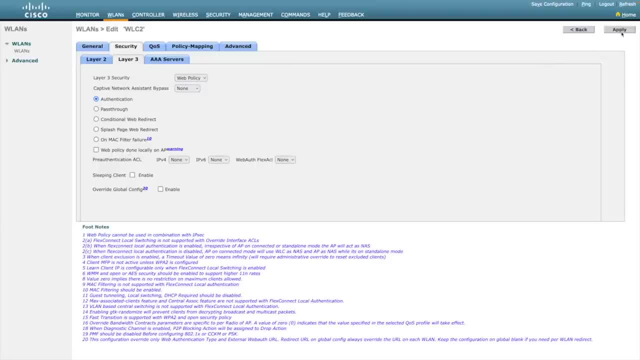 but i'm saying: use this policy, which is what we just created, and i'll say: apply. so. now, when somebody tries to authenticate, they're going to be presented with that splash page that we created without the cisco logo- i think that's the way i left it- and they would have to use login credentials. 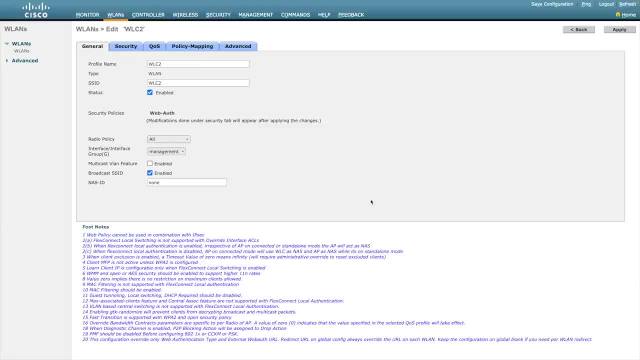 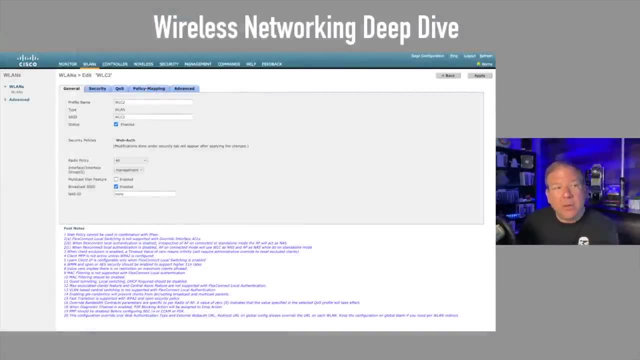 that were found and they would have to use login credentials that were found and they would have to in that local username database. so that is a look. we've now seen four different ways live of setting up authentication. we saw how, using a packet tracer, we saw how to set up. 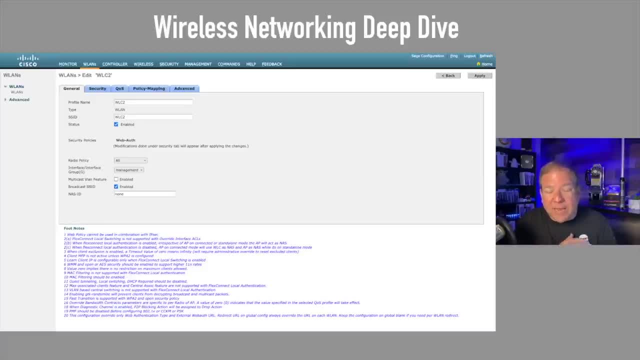 how to set up wpa2 with aes, we saw how to set up eep using a radius server, we saw how to set up local eep using a local user database and we saw how to use this and use a web policy for web off. so lots of different options that we have. now let's get. 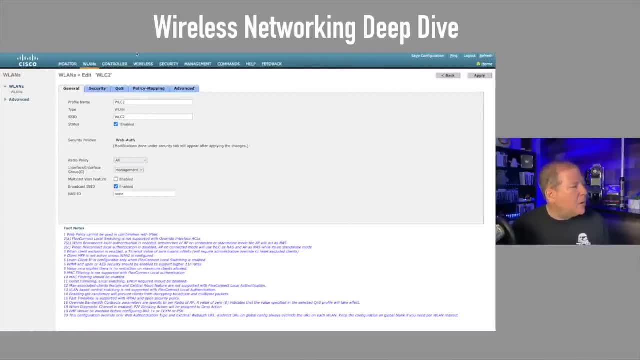 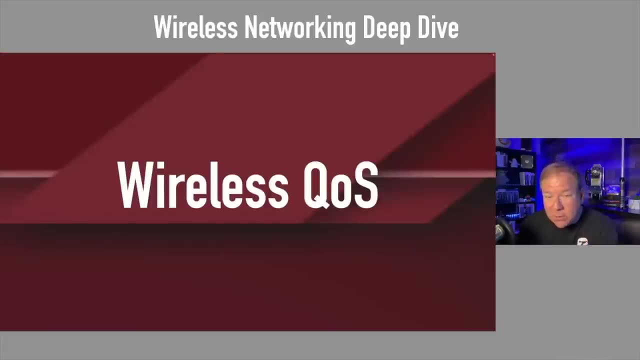 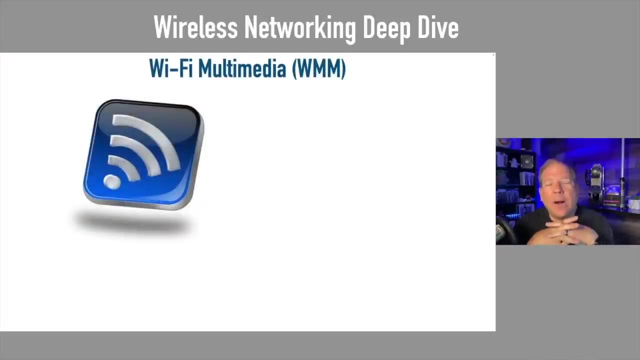 back to our slides. there we go and we want to talk about quality of service. this is an encore topic: quality of service in the live uh, quality of service in the wireless environment. now, if you've joined me for my quality of service courses, i love teaching quality of service and i'm going to 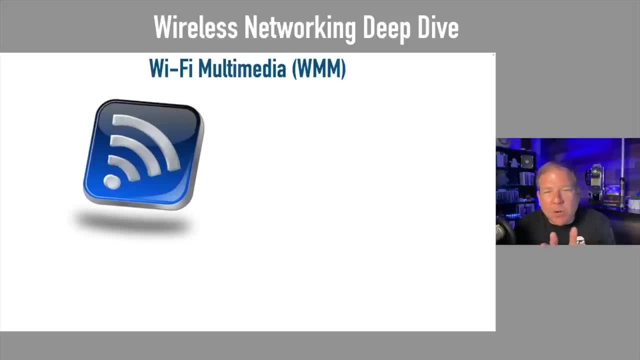 talk about quality of service in the wireless environment now, if you've joined me for my quality of service- and when we talk about quality of service, we talk about different ways that we can mark traffic, and one type of marking that we can do is at layer two and we call it a class of service marking. 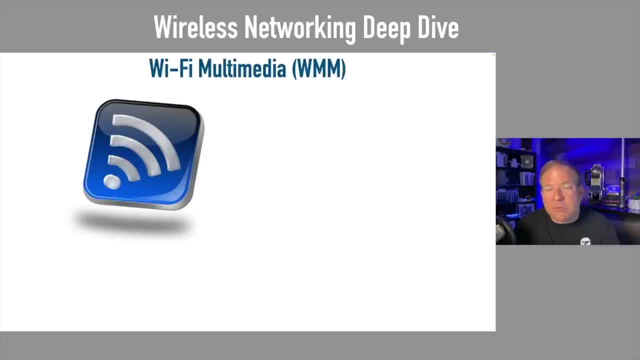 and there are eight values or sometimes we call it a dot one p marking if we're not going over trunk connection. i don't want to review that's a big discussion. i don't want to review all that right now. bottom line is we can mark our traffic with one of eight values in the in the range of. 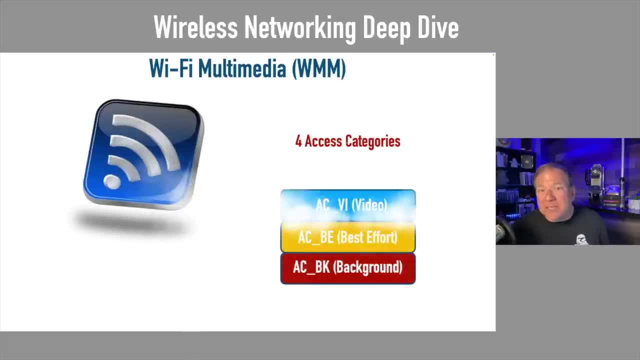 zero through seven. well, wireless is not a service marking. it's a service marking. it's a service marking. it doesn't give us eight categories, it gives us four categories. there's a category for background traffic, a category for best effort traffic, a category for video and a category for voice. 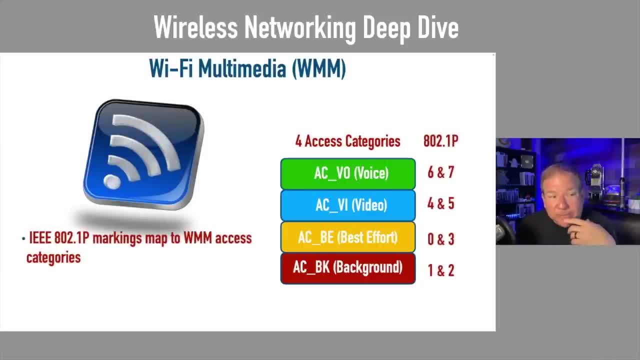 and it's going to take those values of zero through seven that we've previously marked. or cisco phones, they mark them automatically for us and if you're one, if you're have a marking of one and two, you're going to be stuck in the background category zero three, you're going to be stuck in. 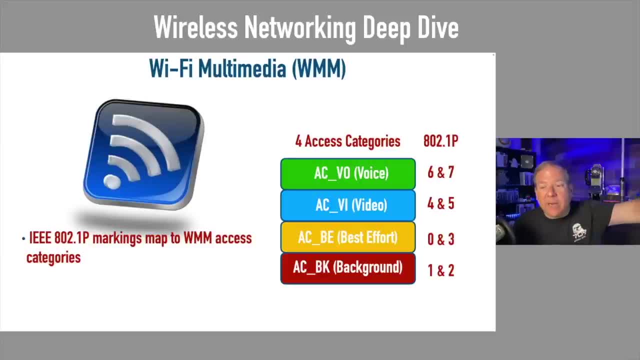 the best effort category. if your voice you're going to be in the background category, you're going to be in- uh, you are. if you're six and seven, you're going to be in the voice category. if you're four and five, you're going to be in the video category. so we've got these four different. 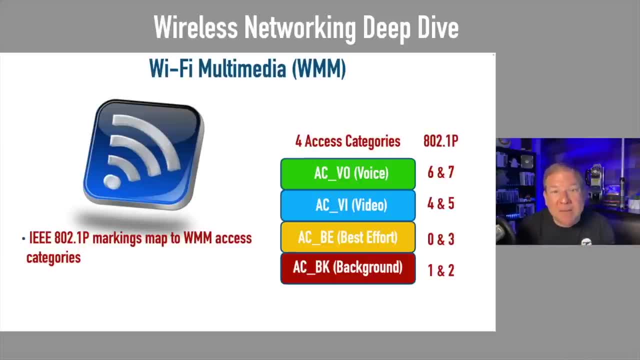 categories of quality of service. what does that mean? how are we going to treat traffic in the voice category different than the best effort effort category? aren't we all just transmitting as fast as we can? yes, but when an access point is transmitting frames wirelessly, it doesn't just send one and just hot on the heels of that first one, as close as it can. it sends a. 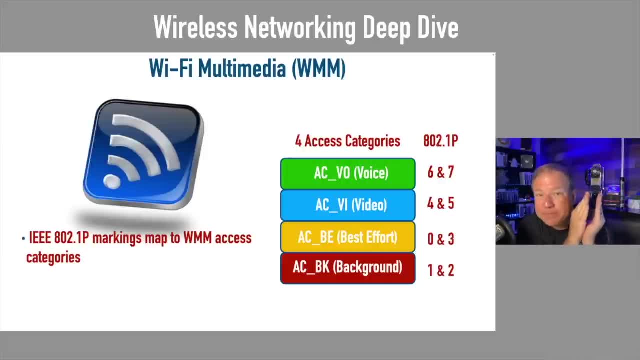 second one: no, there's something called an interframe gap and if there is a collision- uh, because, uh, two people tried to transmit it once, which we cannot do, which we don't have to worry about with wi-fi six, but prior to wi-fi six, we had to worry about that- what we would have to do is: 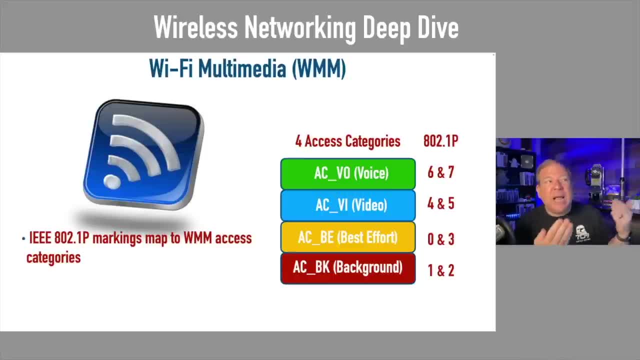 set a random back off time to say, oh, there was a collision, i'm going to wait this amount of time. well, here's the way it works. we're going to do two things to make higher priority traffic get treated better. the first thing we're going to do is we are going to have a more aggressive interframe space. 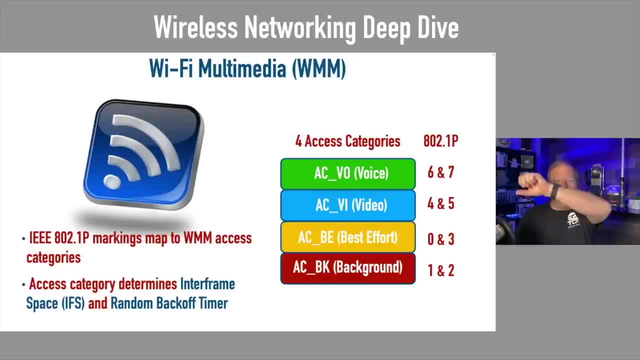 so when i'm sending my high priority traffic, instead of sending one packet and then here's another packet, i'm going to send one packet and just very, very close behind the second packet. we're going to be aggressive in sending those with very little gap and if we do have to back off because 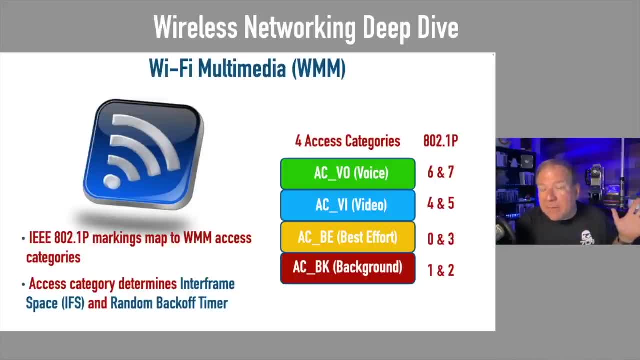 there was a collision collision, the maximum amount of time that I can back off is going to be much smaller for my higher priority traffic. In my lower priority traffic it's going to have to wait a longer amount of time if it experiences a collision. So I'm going to be more aggressive in transmission and I'm going to 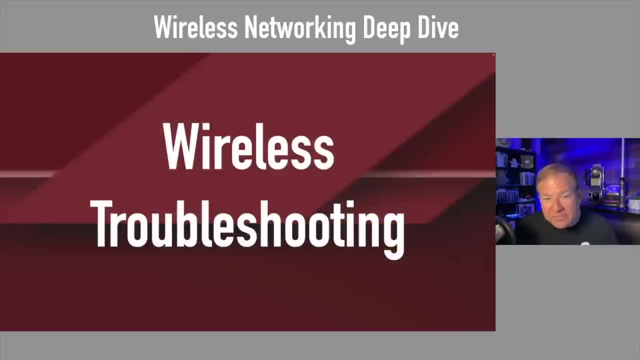 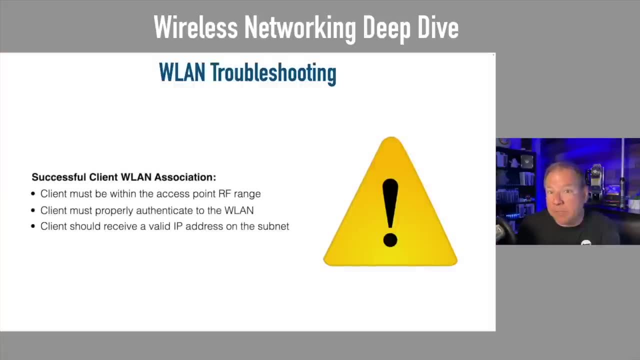 wait a shorter amount of time in response to a collision, And our final topic for today is troubleshooting. Now, when we're troubleshooting, a lot of wireless troubleshooting is common sense. Let's think about this Number one: your client's not getting on the network. 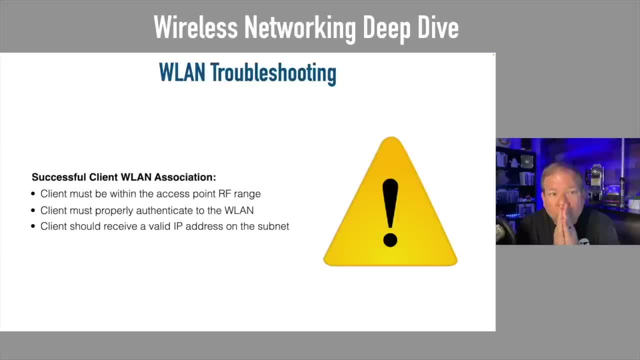 Are they in range of your wireless access point? Some people buy long-range access points thinking that that's going to solve the problem and it can definitely help. But sometimes just because you can transmit with a higher power level, that doesn't mean you're going to be receiving. It doesn't mean your phone out there is going to be. 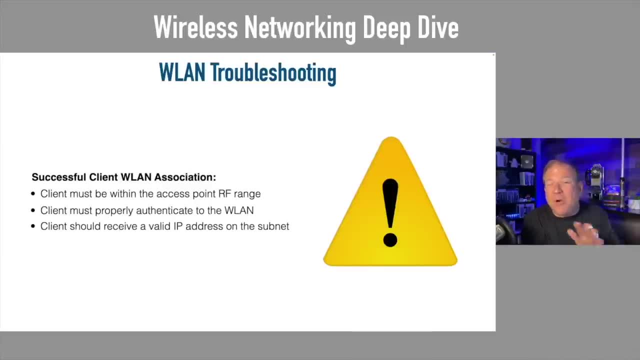 able to transmit. It doesn't mean your phone out there is going to be able to transmit Back to you at that higher power level. Now some long-range antennas. they have more sensitive receivers but not always So. quote-unquote. long-range access points don't always fix it. 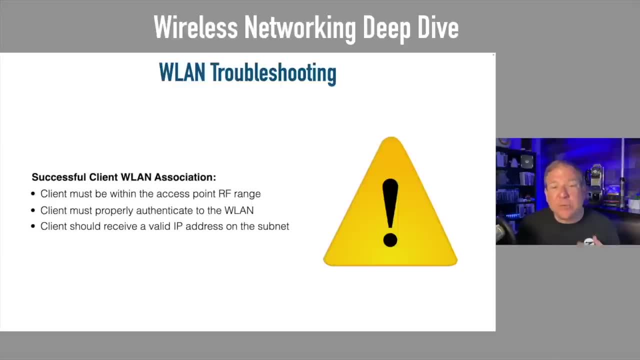 for you. Make sure you're in range. In fact, I like to do a site survey. I will take my little wireless survey tool and I will just walk around the building after I've got the access points in place or just temporarily laid on a desk to see if it's a good place for an access point. 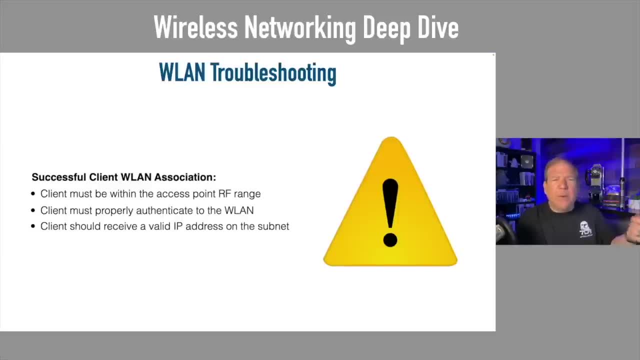 and I'll check the coverage. Oh, that's a little weak here. Maybe we need to check the coverage. Maybe we need to come out from that corner a little bit. Make sure that authentication is set up. There are multiple options for authentication. Just double-check all that. 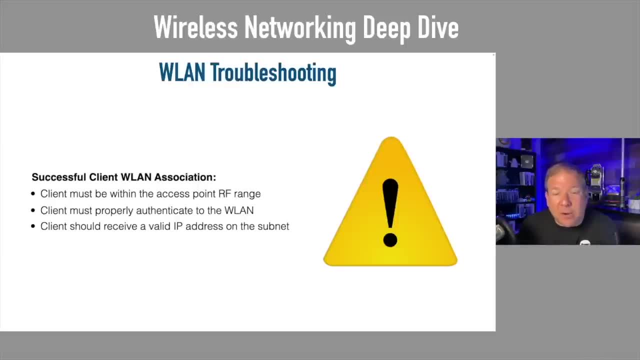 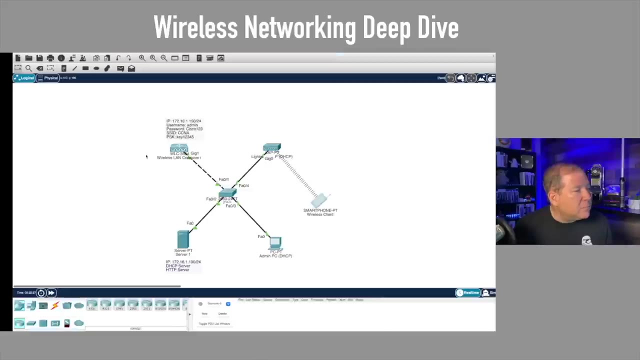 configuration. Make sure that your device is getting an IP address on the right VLAN. Make sure all that is set up correctly. I want to show you some other places you can look to do troubleshooting If we go back out to our main interface here, open this up.